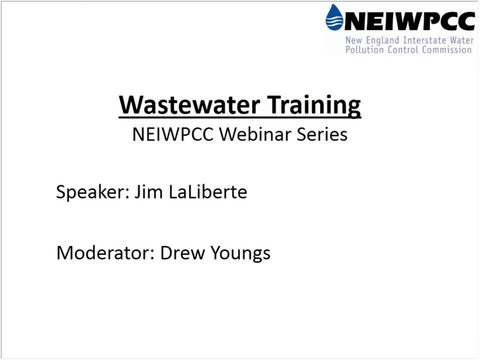 time and thanks for joining us this morning. My name is Drew Youngs and I'll be moderating today's first of three wastewater training- all NUIPIC internal staff webinar series. Kind of a long title but a lot of good information. today Our speaker is Jim Laliberte And I'll 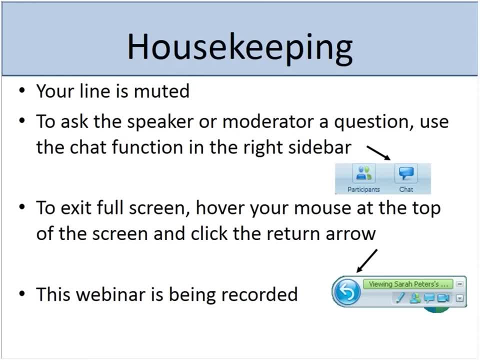 tell you a bit more about Jim before we get started. But before we get into the meat of the training, I just wanted to give you, for those of you that are calling in, some tips on using the system. if it's your first time, It can be a little confusing. Your line is: 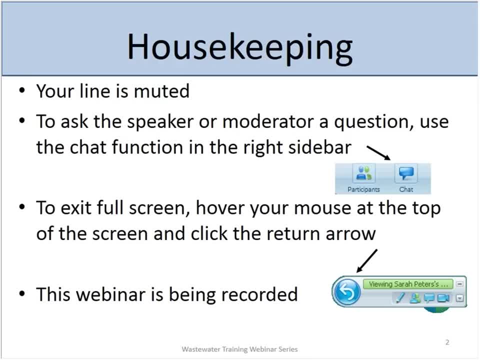 muted so we can't hear you, But the idea is that you can hear us as we move through the slides and chat about them. To communicate with me or to pose a question for the group or to Jim, you can use the chat function. As Jim is presenting today. I'll be keeping. 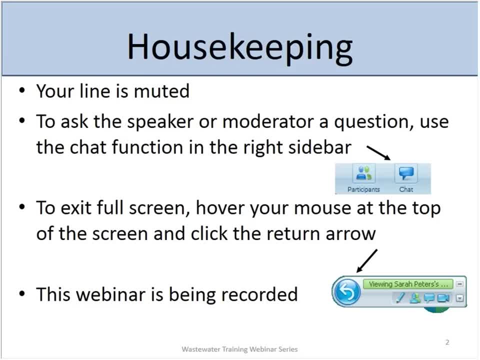 an eye on the questions that come in via chat And when we have, you know, a good opportunity for discussion. when I have some questions coming in, you know I'll ask Jim when it's a good time And you know we'll chat about your questions. 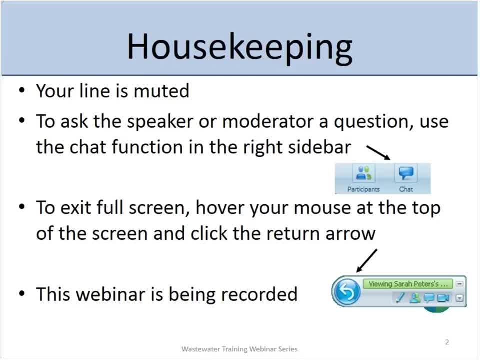 So use that function to communicate with me. You can toggle in and out of full screen by using the arrow function. You just you want to hover at the top of your screen where that green bar should be, And it will give you kind of a drop down menu to navigate the. 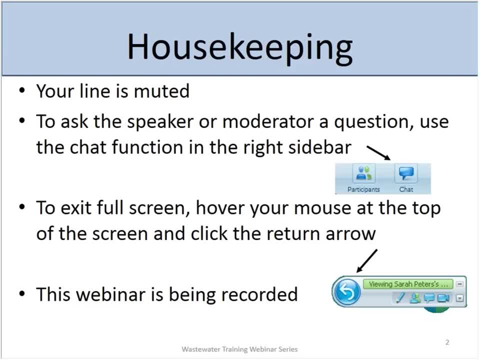 system. We are going to record the webinar, So this will be up, probably on our website in the future. We'll have it in electronic form so you'll be able to access it. You can contact me, contact Jim, contact Tom Groves, And you'll be able to get that And you'll 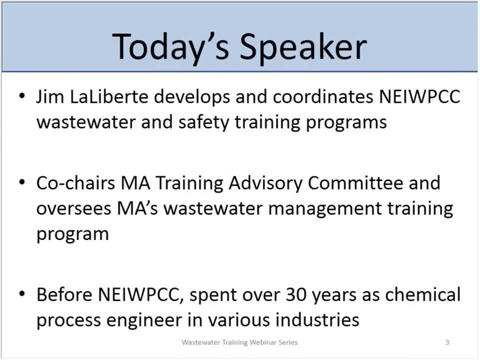 get that information. So a little bit about Jim. Jim works with us to develop and coordinate NUWIPEC's wastewater and safety training programs. He's the co-chair of the Massachusetts Training Advisory Committee and oversees Massachusetts Wastewater Management Training Program Before. 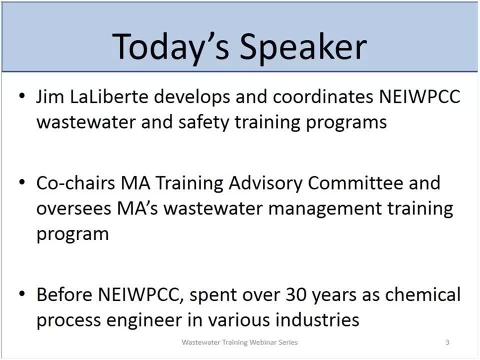 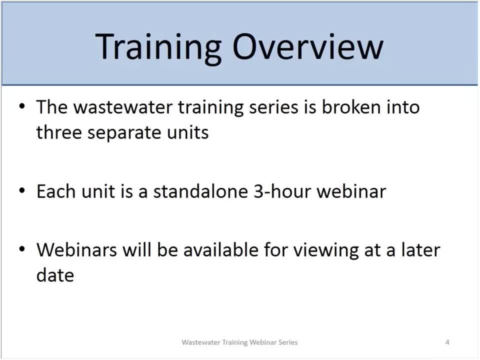 coming to NUWIPEC. he spent over three decades as a chemical process engineer in a variety of different industries. So for the training overview I'm going to use the Jim's, excuse me. this is an overview of Jim's training. It's broken into three. 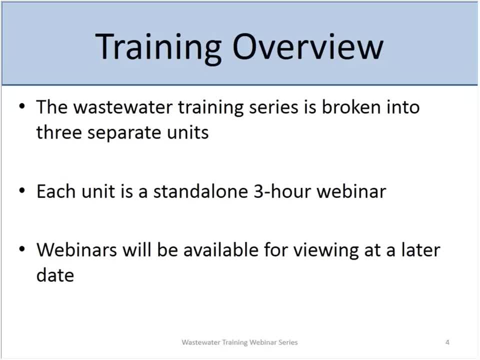 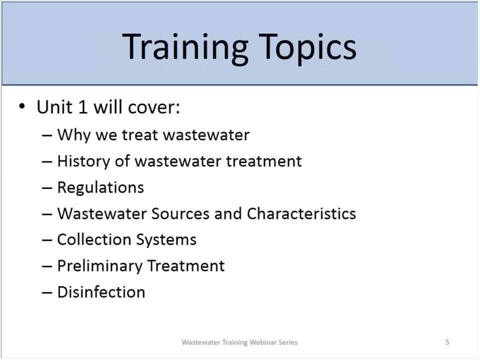 separate units. Each unit is going to be a standalone webinar of about three hours And these are on the three different dates that you're probably aware of And again, they'll be available later as well for you to come back and review. So Unit 1 is Day 1.. That's today. Jim's going to tell us about some reasons why we treat. 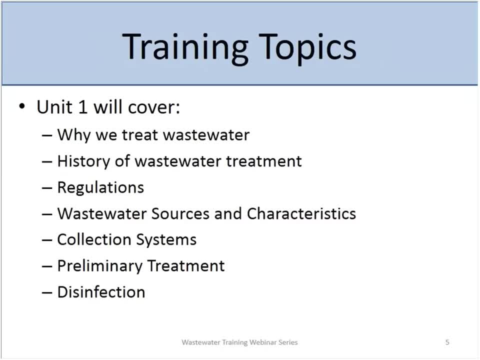 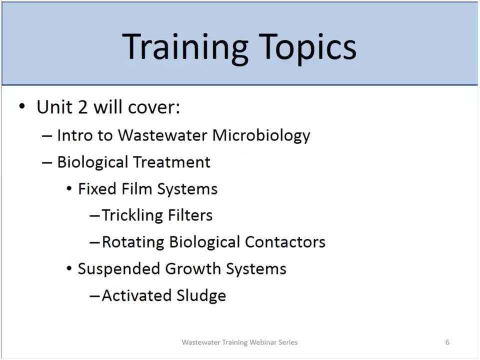 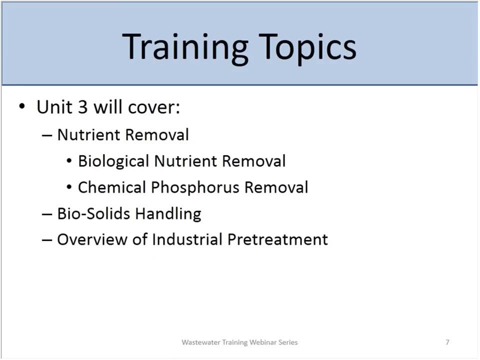 wastewater: the history of regulations, wastewater sources and characteristics, collection systems, preliminary treatment and a little bit about disinfection. And then Unit 2 is Intro to Wastewater: Microbiology, Biological Treatment. And Unit 3, which is Day 3 in February, will. 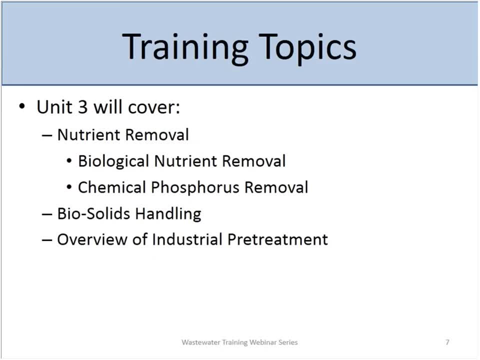 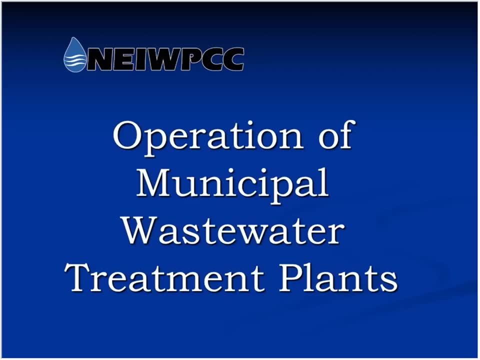 cover nutrient removal, biosolids and an overview of industrial pretreatment. So, without further ado, I'm going to go ahead and hand it off to Jim. Thank you, Drew. To expand a little bit on the topic, what Drew was telling you about myself outside of outing me for over three decades? 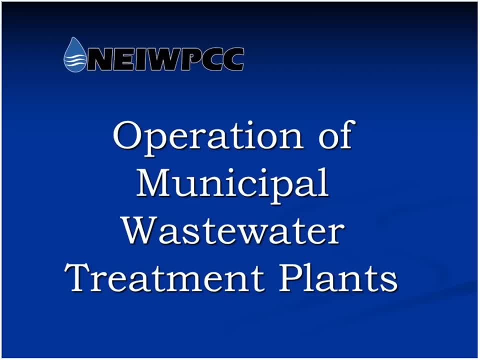 of work, actually a chemical process engineer by degree and got my career started with sugar, which is a long way from dealing with wastewater, But nonetheless I fell into the wastewater field pretty much by accident, the way most people do, working for a small chemical company. 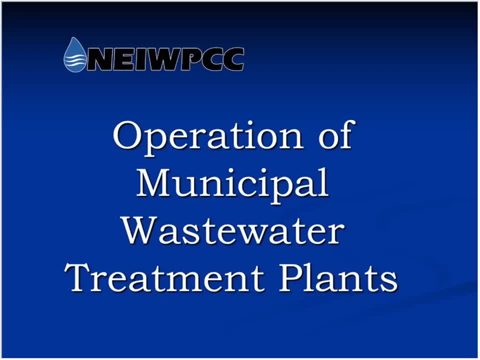 in National New Hampshire And they actually had a wastewater treatment system, which is what they were doing, because they were direct dischargers of their effluent to the Merrimack River. Y'all know what that direct discharger is. What is it? 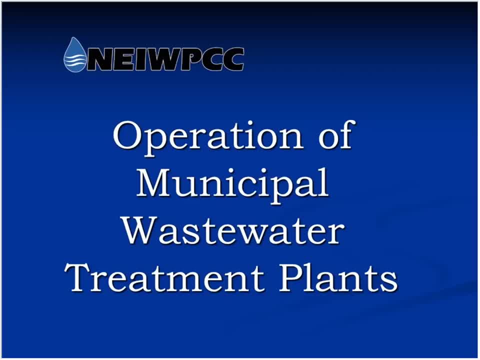 You mean the wastewater into the river Right. We were going directly into the Merrimack River And at the time I took over the process they'd been operating for about five years. They had a NPDES permit and I imagine you all know what NPDES stands for- And at that 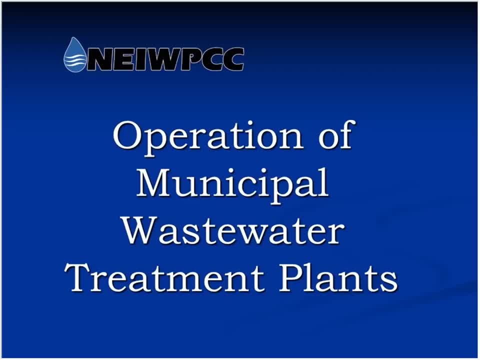 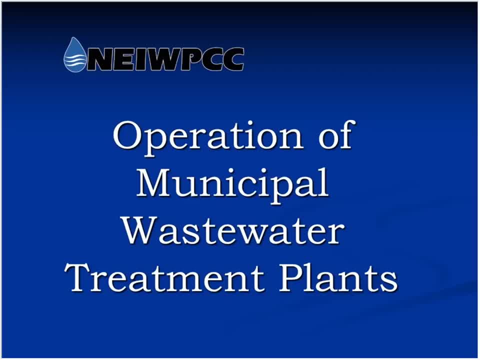 and they had a NPDES permit and they had a NPDES permit and they had a NPDES permit. They were just chugging along nicely and getting away with it. In New Hampshire, the regulations were a little weird. Since we weren't really dealing with domestic waste, it kind of fell. 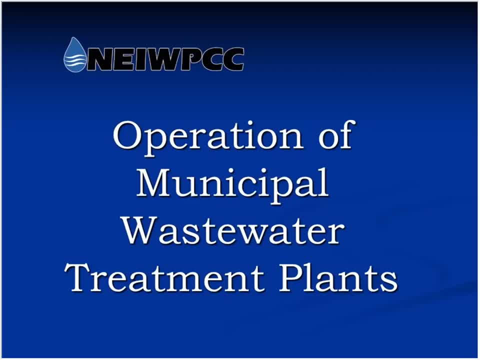 under the radar. We still had a state permit, We had the NPDES permit And we ran an activated sludge process, much like most municipal systems, And I felt that, since I was going to have to learn all this stuff very fast, I might as well be certified, And I went through the 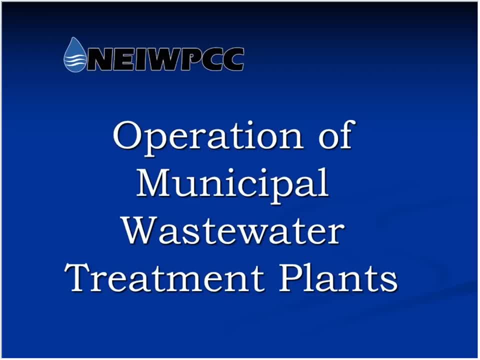 process of eventually getting a grade four, which is their highest. I currently hold a five combined down here in Massachusetts. Massachusetts is a bit different from most other states in that they have industrial certification And at the combined level of five and six here in Massachusetts that means I could work in an industrial facility. I could work. 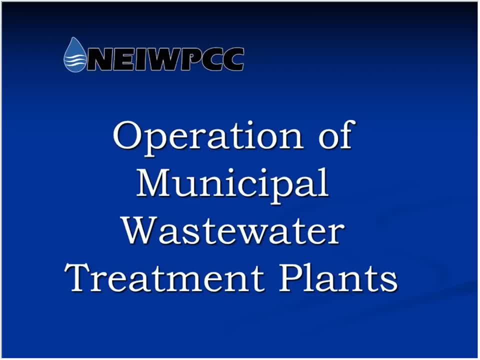 in a municipal operation. That being said, I got thrown into it very quickly. I found it to be a very fascinating field and economists having to play with it, But nonetheless this is a lot cleaner. So what we're doing through this program is: 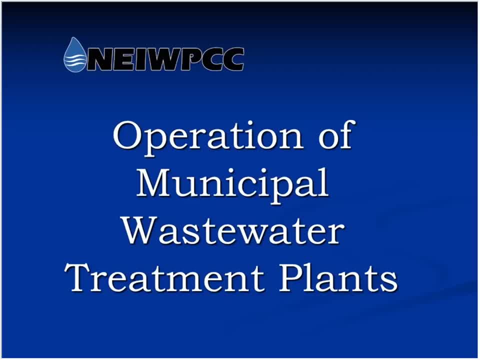 basically a boiled-down version of what I normally do over a six-week period, one day a week for six weeks For people that are getting into the business and wanting to become certified. I also do a higher level one, an intermediate course of people advancing up. 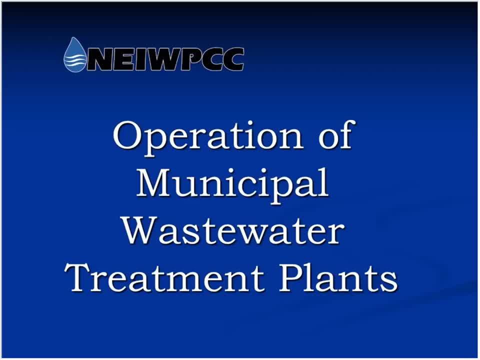 through the grade levels, So I'm jumping over a lot of stuff that you really don't need to know, But you're going to get a good overview of what you're going to be doing And you're going to get an overview of what goes on soup to nuts- in a municipal treatment plant. 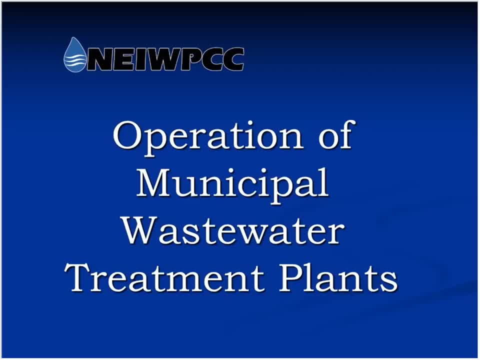 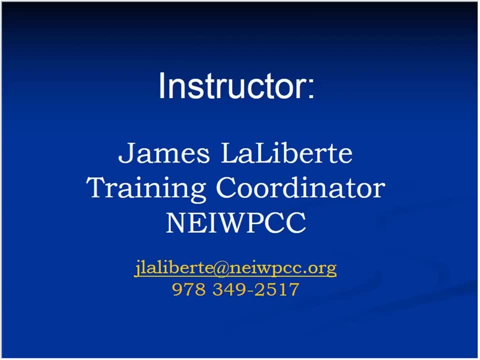 various types and give you something to go on When you're doing your work, relate back to how this may or may not affect what we're doing on our end of the pipe. So again, lastly, this is my email address, my direct line to my desk, if you have any. 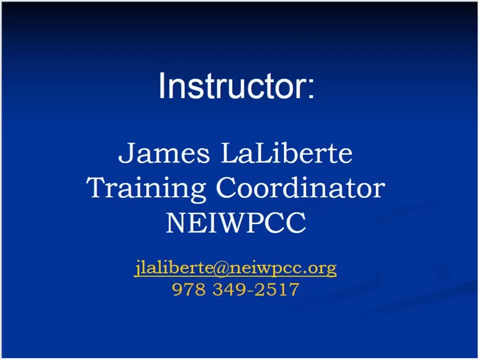 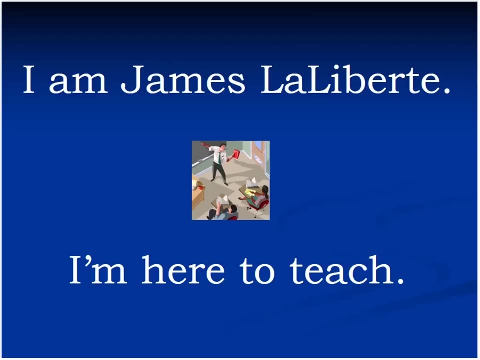 questions about wastewater treatment or anything like that. We've got a lot of people here, primarily out of New York State, so you guys run a little bit differently in your certification process than what we do here. So again, this is my deal: I get up and we go through the. 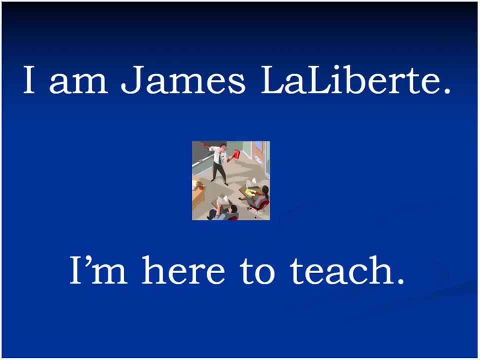 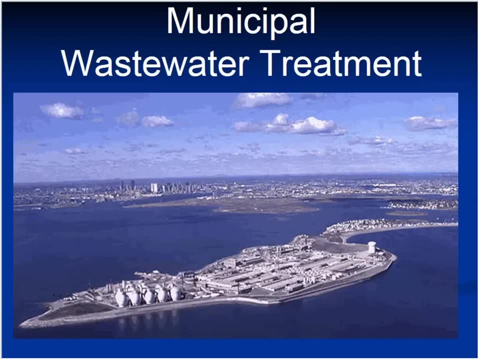 room and find out who's around. That's a little bit difficult in this current circumstance, but you know about me and how I got started and why I'm the guy in the front of the room. So we're going to talk about wastewater treatment Again. this morning. I'm going to go over a 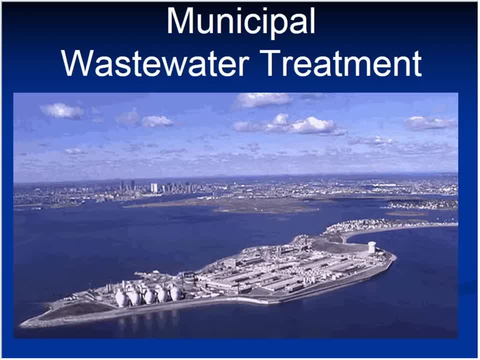 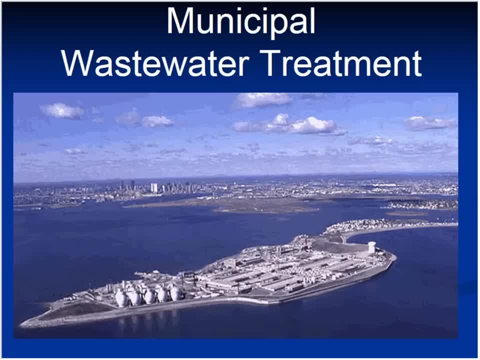 This particular plant that you're looking at now is Deer Island in Boston, Mass. Deer Island is one of the largest facilities in the country. Typical day is about 350 to 400 million gallons. The highest number I've seen go through the plant was we had some very 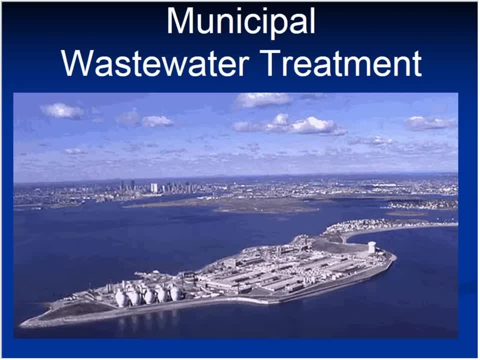 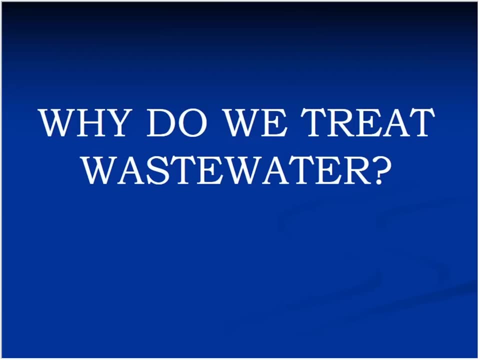 heavy spring rains about almost 10 years now And the highest number I saw over there was 1.3 billion, the difference being a billion gallons of rainwater going through the plant is about 2.9 billion gallons. What are we in this business? Why do we even have to? 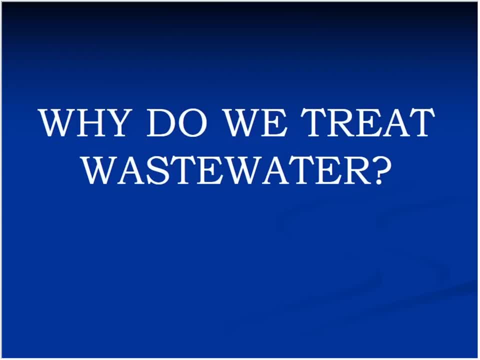 deal with this stuff. Civilization went on for centuries without any wastewater plants, without any septic systems or cesspools or any of that kind of stuff. Why do we have to do this? Population growth, Population, growth, Population. Well, that certainly exacerbated the situation. Everybody wants clean water. 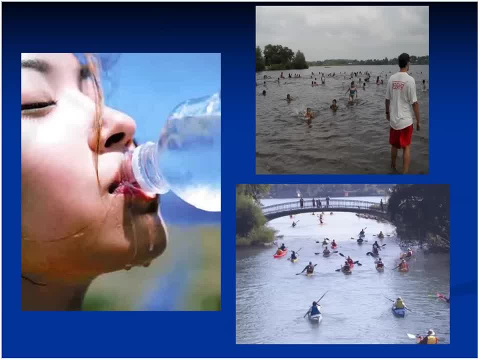 and I don't want to be the only one who wants clean water. Everybody wants clean water. You want to be able to go out and go canoeing or swimming in the lakes and the streams. It's also a part of drinking water protection. part of it too. 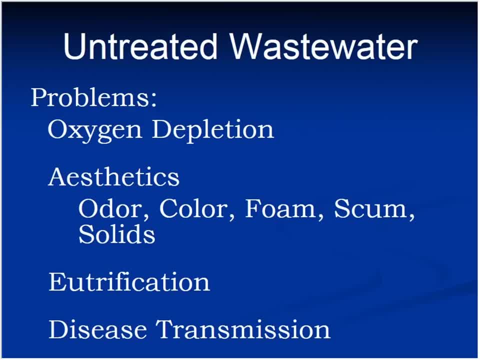 Untreated, this water is thrown into the rivers and the waterways. We're going to have oxygen depletion. Basically, the river is going to die off. Aquatic life can't survive. We're going to have odors and scum and it's just going to look nasty and be ugly. 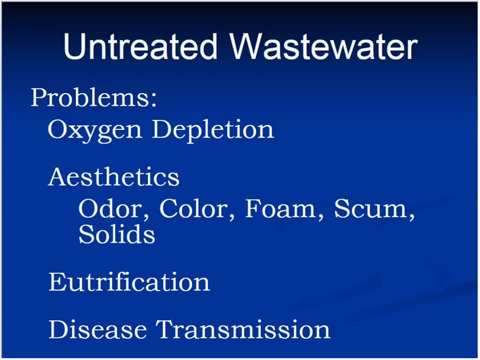 and you're certainly not going to be able to drink it. The issue that we're dealing with to a large degree now, as we move forward with technologies, is the problem of eutrophication. Eutrophication is when you throw a lot of nutrients into the river water. 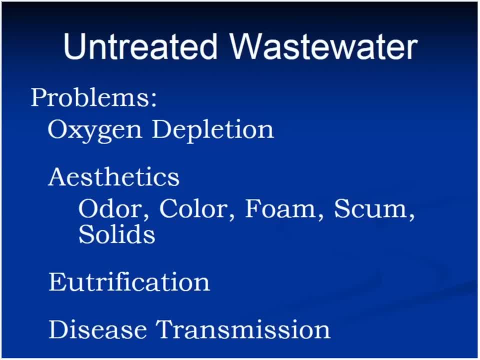 and you help grow aquatic plants, Algae and weeds and all that they slowly take over. And really the biggest part of our business- we really want to look at it from that standpoint- is we're in the health business- Disease transmission. 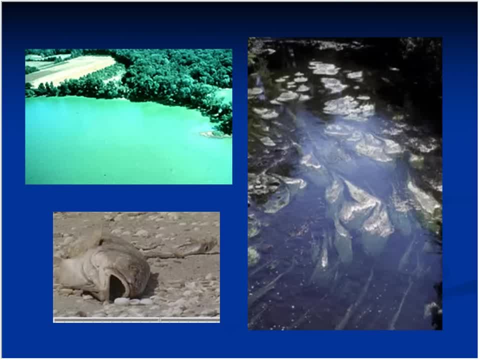 Waterborne, Waterborne diseases. Again, this is what we're trying to avoid. Fish kills. Amomia toxicity could generate that. Green ponds. That's eutrophication, That's a problem that we deal with And just nasty looking streams. 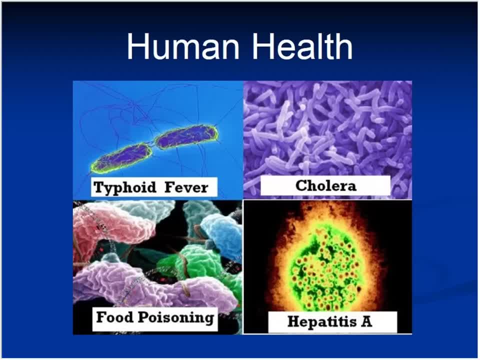 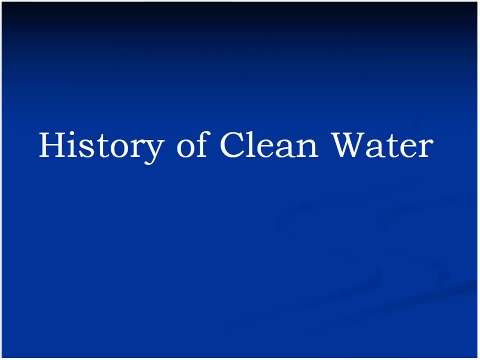 Again, these are the problems we're trying to deal with: Eliminating waterborne diseases. The largest reason for population growth to the degree that it is now is because of wastewater treatment and the improvements that have happened over the past hundred years or so. 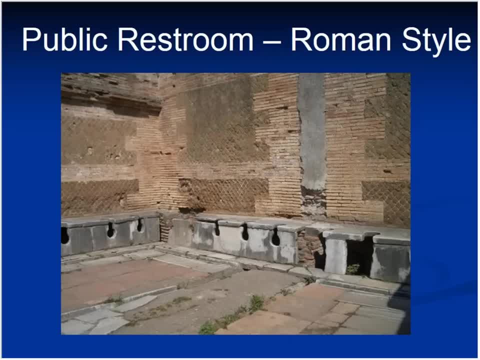 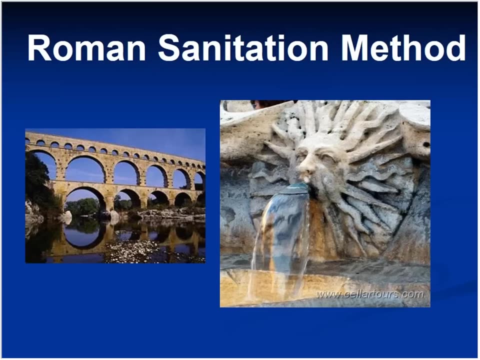 But again we go back a long ways with efforts made to deal with waste, Human waste- largely. Again we go back to days of Roman empress. you know, early days, AD, Public restrooms and all that Tough on a cold morning, but what are you going to do? 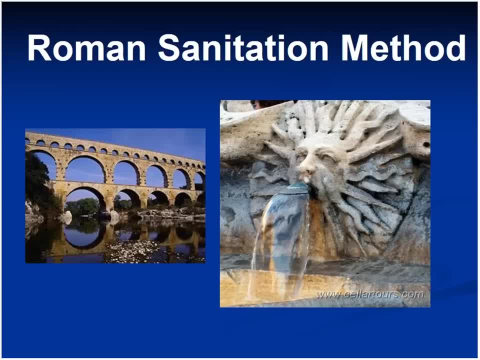 But really Rome 50, 60 AD. Rome brought in over 2 million gallons of water each day from the mountains, The aqueducts. you had all the nice fountains. It was very pretty, but its real purpose was to flush the waste out. 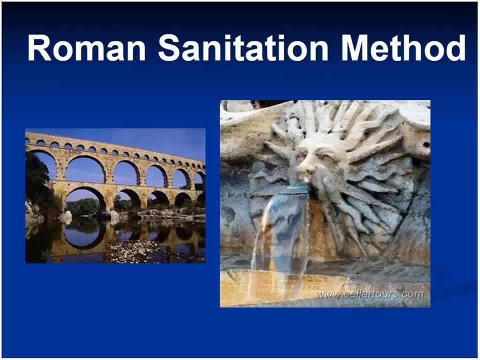 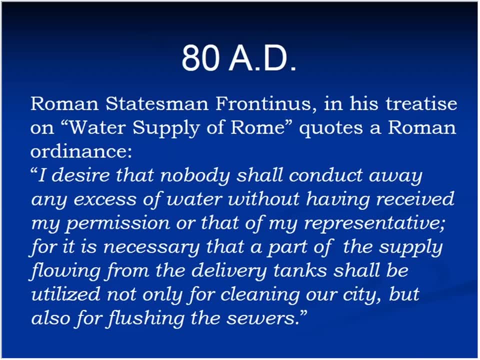 get it to the river and make it go away. That was wastewater treatment for centuries. Get it out of town, Let it be somebody else's issue. Even then they had concerns over control of water. We had old Frontenus here. 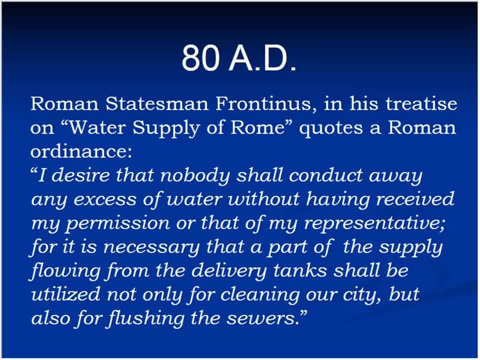 He was the guy in charge of water back in 80 AD. He could do anything without checking with him. Necessary that a power supply flowing from the sewer tanks be utilized not only for cleaning the city but for flushing the sewers. That was treatment back then. Over and away, As time went on, we did have that population growth. You had started to have some really dense inhabited cities and stuff And again they would put ditches in the middle of the street. They were actually starting to put the concept of sewers to take stuff away. 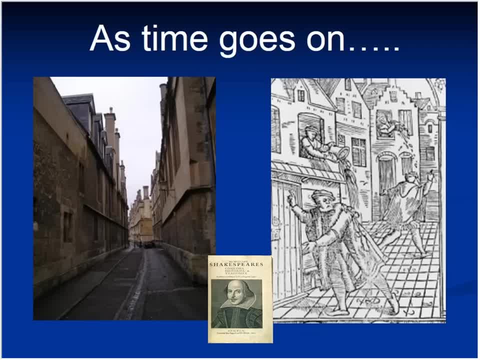 But again, it was still just to get it to the nearest river and have it flow away. I've got Shakespeare up here Because the time of Shakespeare, right around 1600,, the island of Great Britain really only grew its population because of emigration from continental Europe. Left to itself, the island would grow its population. Big cholera outbreak, Boom, Typhoid, Boom- Same thing. It just went back and forth and had no real growth. Early days of the United States. all you needed was some land. 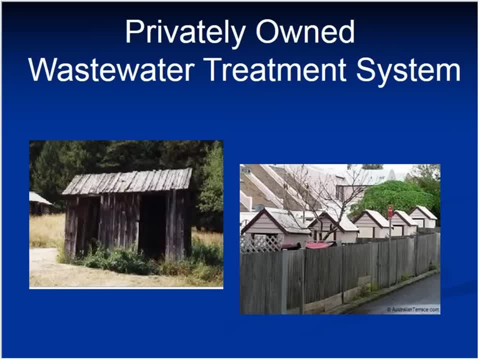 You'd dig a pit over in the corner, put up a nice little shed, You were good to go. And even in the populated cities there were back alleys. They had all the privies just lined on up. And actually, if you remember, Shelley, 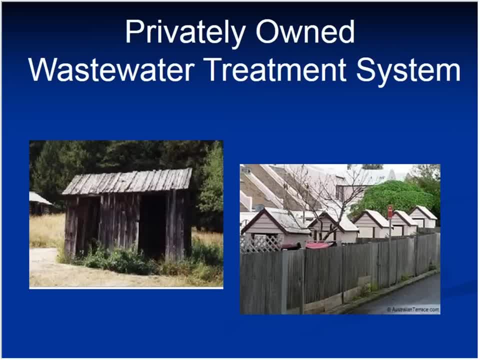 somebody came in and showed their license for night soil. Yes, Night soil was the industry. People would come in, clean these things out, and they would do it during the night And then they'd use it for fertilizer later on. That's where night soil actually came from. 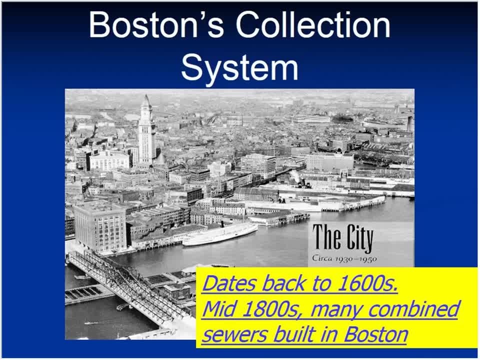 The version of septic hollers I guess you want to look at Again. as time went on, populations grew, You'd see big cities. Besides sewering Back in the 1600s, we have some sewers. 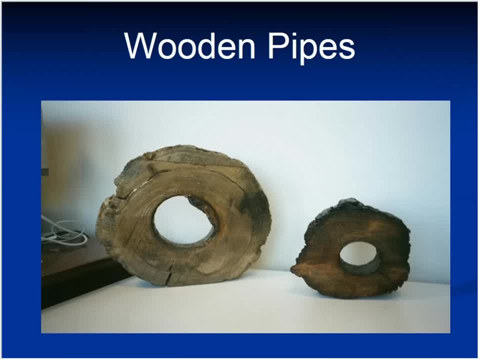 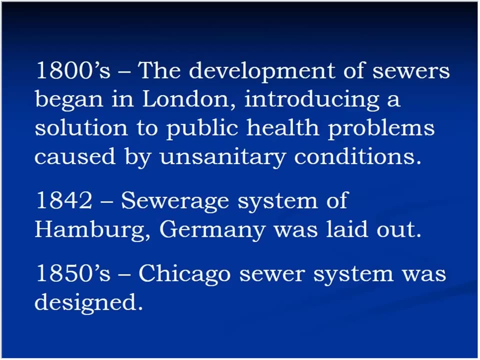 Even in the Boston area they still dig up wooden pipes that were found for use in transporting water, transporting waste into the harbor, just to get it out of town. No real treatment, Just move it out of the way. It's really part of the 19th century. 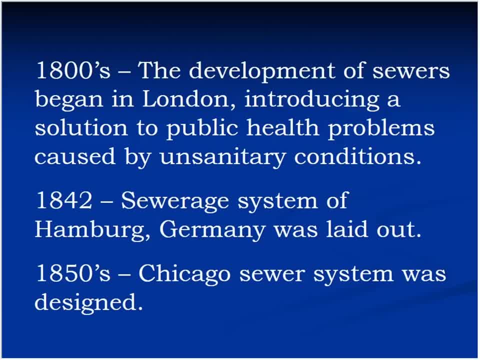 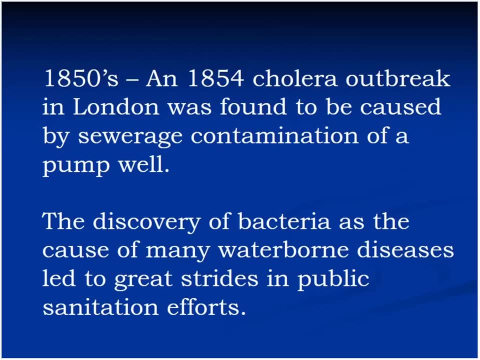 It started to have some issues, Had a big outbreak in London. It really started to open up some eyes. Science was advancing at that time. Microbiology and other stuff was developing. We got a lot of sewers were being put in, But we had this big cholera outbreak in London in 1854.. 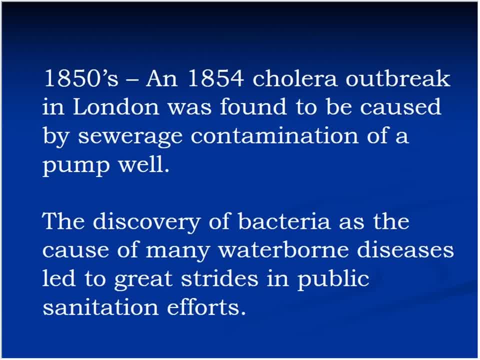 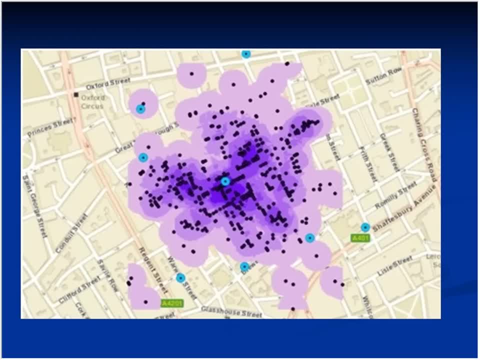 And a fellow by the name of Dr Snow was the guy that actually made the connection And they found this well pump that was in the city of town. He studied all of the cholera incidents around this particular area and found that this one, well, this little blue circle here. 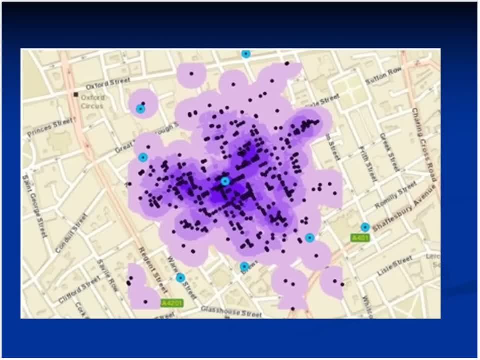 in the center of all this mess seemed to be the problem, And when they investigated they found that the well was actually less than three meters away from a cesspool And it was leaking in, And anybody that lived in the area was using that for water. 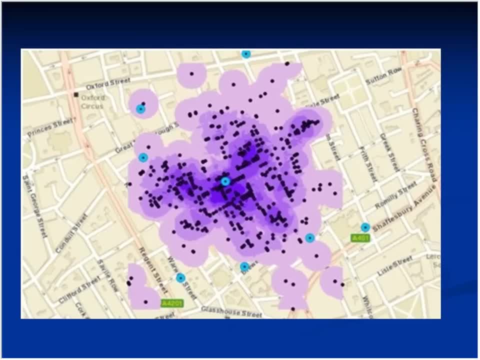 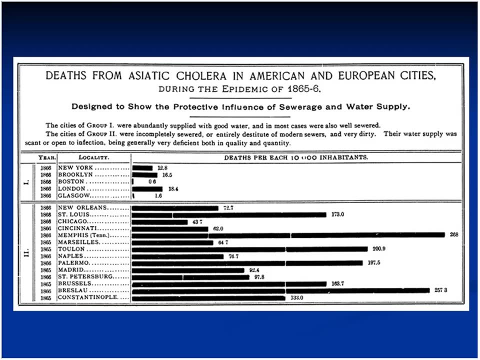 People were walking by. That's why you had some of these outlives. We're all getting contaminated from that. They realized that they had to really separate these two items and not let them get together Again with sewering and smothered material. 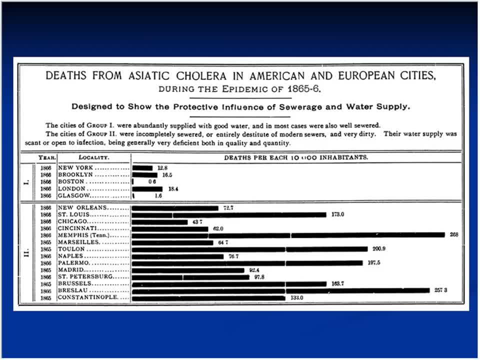 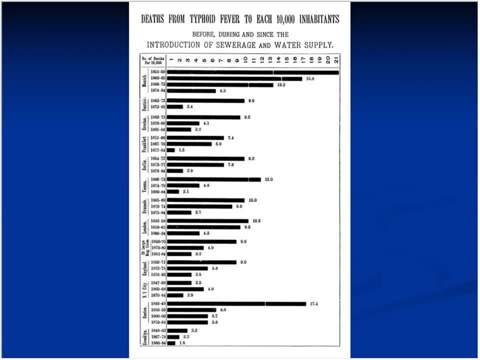 look at sewered cities as opposed to unsewered cities in terms of cholera deaths. They changed because now it's not so prevalent. You have all these cesspools all around town contaminating drinking water And if you look at individual cities as they sewered over time, 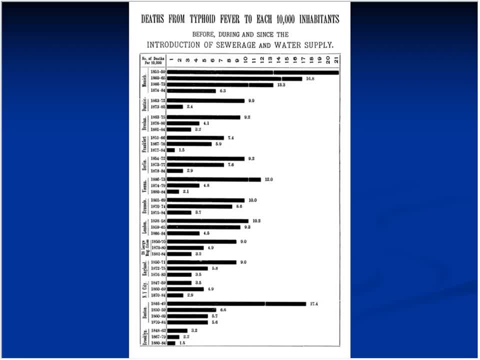 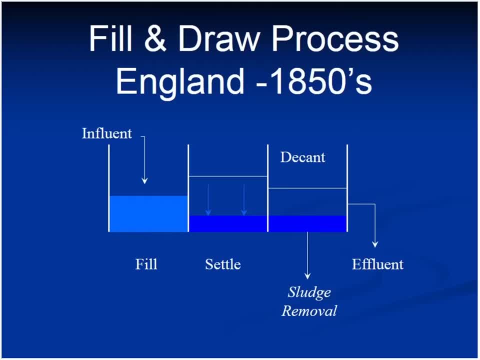 typhus deaths all dropped off considerably Well, they started to realize that you had to keep them separate, But they still weren't really treating. It wasn't until the latter part of the 19th century that in Britain they came up with this process. 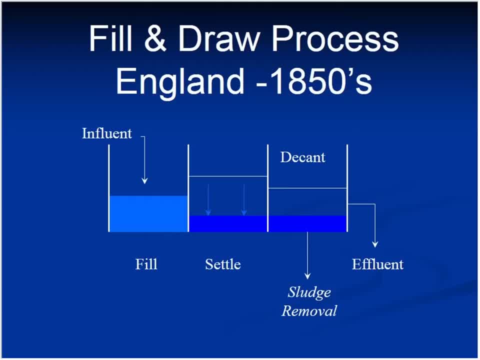 that they called the salt till it dropped. Basically, they'd pump all the water into a tank and let it sit. The solids would settle to the bottom of the tank. The supernatant looked relatively clean. They'd take that and throw that in the water. 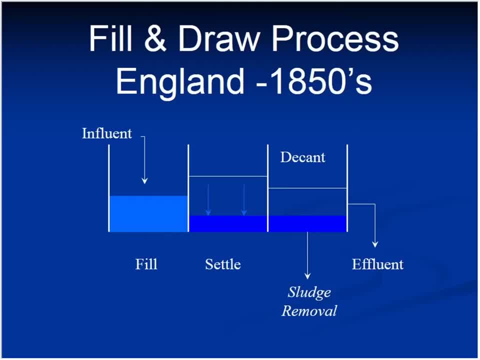 The sludge that would be removed on a regular basis was then taken off to use as fertilizer. That was all well and good and they were doing a pretty decent job, except for the fact that this liquid that they were sending off to the river. 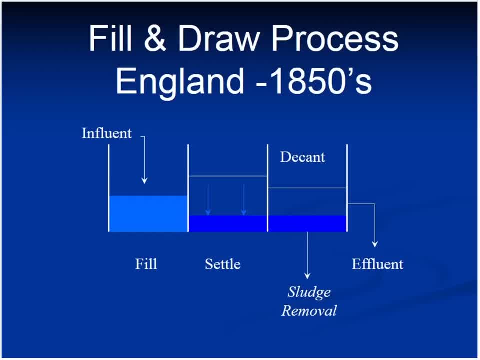 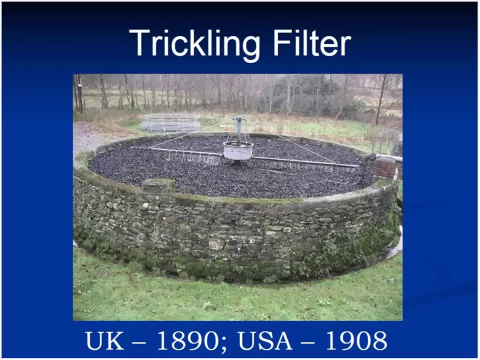 still contained about 60% of the BOD of the wastewater. because it was soluble, It didn't settle out as a solid. Around 1890, they developed what's called a trickling filter, And this is actually a real method of wastewater treatment. 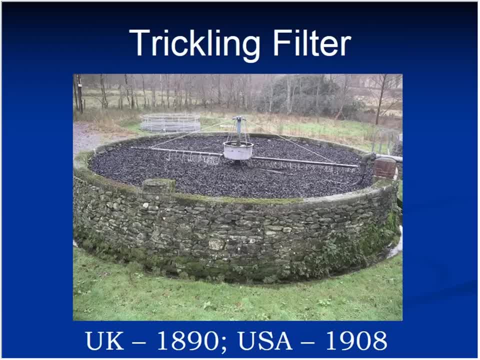 What we've got here is a nice little thing all built of stone and stuff. So you've got a tank, You fill it with some sort of a media- whether it's rock or broken bricks or something like that- You pump the water in. 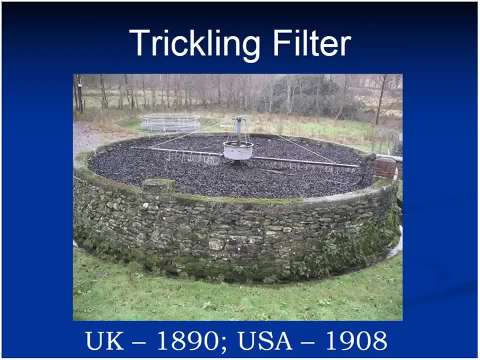 let the water trickle down through that media. Organisms live on that media And, as it sounds, one man's waste is another man's treasure. Well, that's food to them, All this wastewater. they would break down the BODs that trickled through this unit. 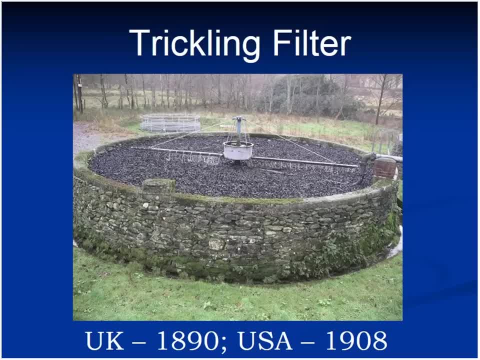 So you had a very low BOD coming out of this thing When we talk about trickling filters. we'll talk in much more detail about this next week. It's not a filter in the traditional sense. Think of it as a BOD filter. 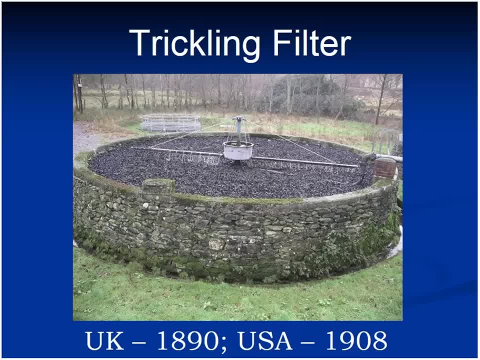 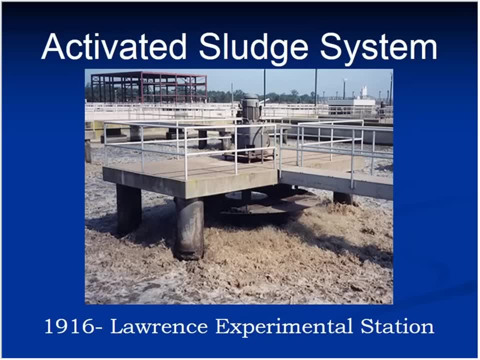 In fact, you're going to have more solids coming out of this than actually go in, And this idea was brought across to the US a little after the turn of the 1900s. Now the activated sludge system, which is the most common method used today, 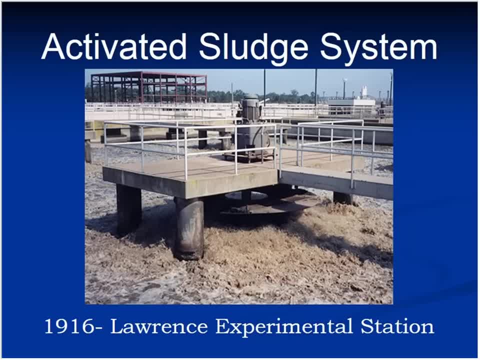 a lot of that development work was done here in Massachusetts over at Lawrence Experimental Station, And this is where you really have the optimum amount of control over what's going to happen in your process. You can do all sorts of things with these organisms by manipulating their conditions. 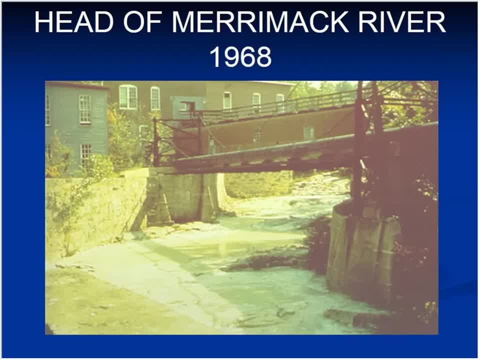 It's a very common method, But even at that there was not a lot of regulation forcing anybody to do this sort of thing. Rivers were still just dumping grounds for waste, whether it's domestic waste, industrial waste. This is. you can't quite see it. 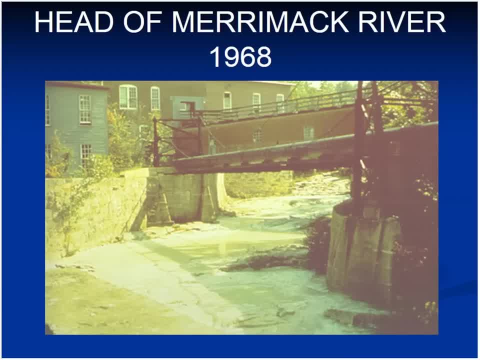 but this is the Merrimack River. Oh, there you go. Cool. Thank you, Drew. This is actually up in Franklin, New Hampshire, where the Winnipesaukee and the Tumajewasek come together to form the Merrimack River. 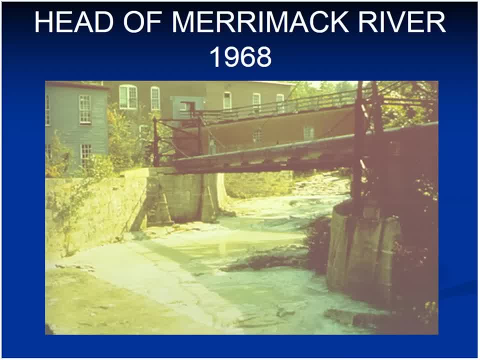 And it's an old slide, as you can tell. It's pretty well yellowed out, But still there's no fly fishermen, There's nobody tubing, There's nobody swimming. That water is barely looking like water. Nasty, nasty stuff. 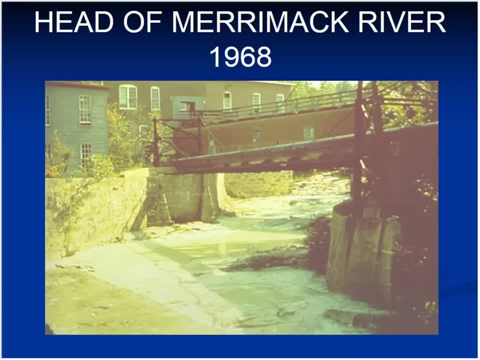 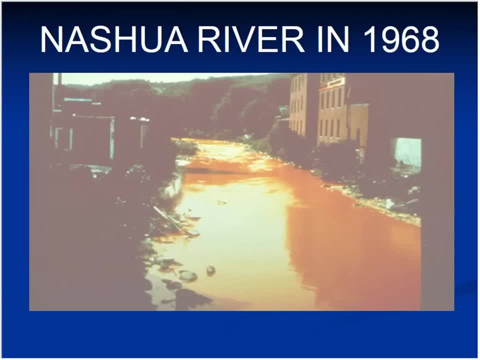 And that isn't even 50 years ago. This is the Nashua River. Yeah, I'm from Nashua. I remember the river looking like this. The mill was making red paper that day. Oh, is it close up there? I actually had a job in a mill much like this one. 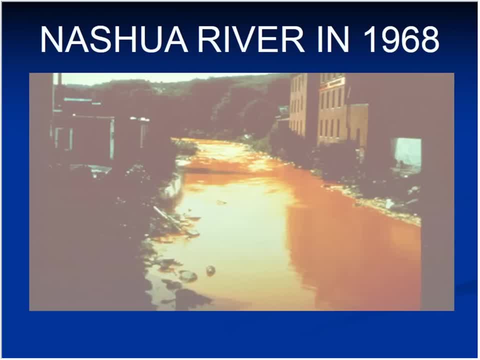 you see, on the right alongside the river, It was right. in downtown Nashua- Excuse me, And the plastics thing- we had a fellow who put together all of these dyes, powdered dyes, to mix with the plastic for whatever it is we were producing that day. 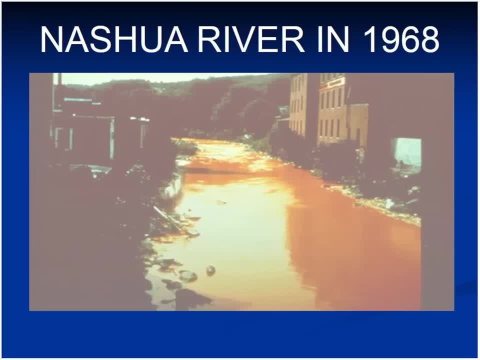 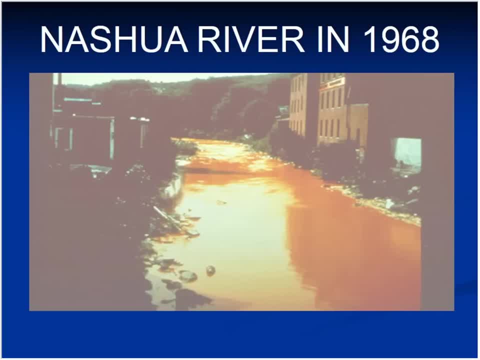 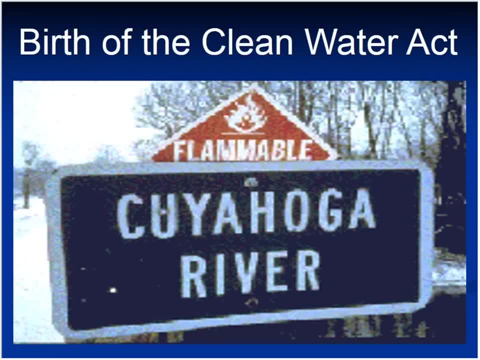 a little bit more time. there was an incident out in Ohio. This is the Cahova River and we got our flammable sign. A bit of a joke, but not really. 1969, Cleveland, Ohio. The picture on the left. 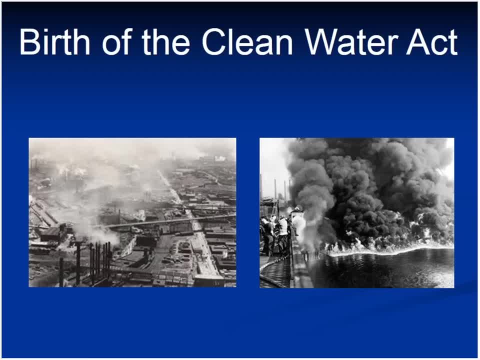 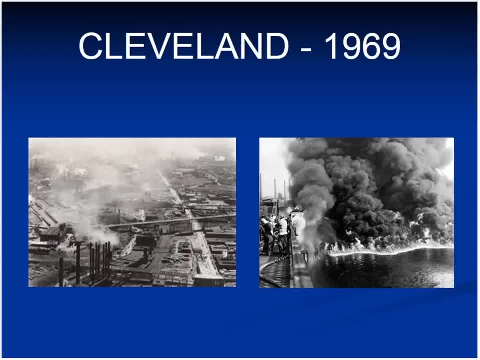 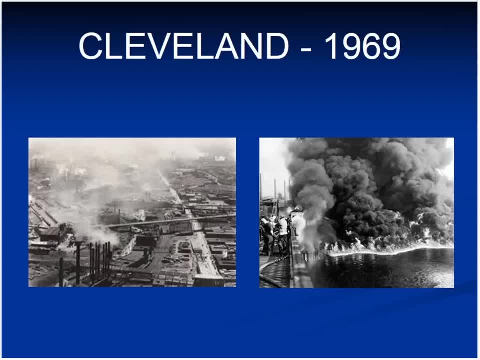 Big industrial area. When you crossed the bridge over the Cahova River and you looked out and you see this, it was the stereotypical picture of pollution of every sub you think of. And one day the river caught fire. Fire lasted about 15 minutes. 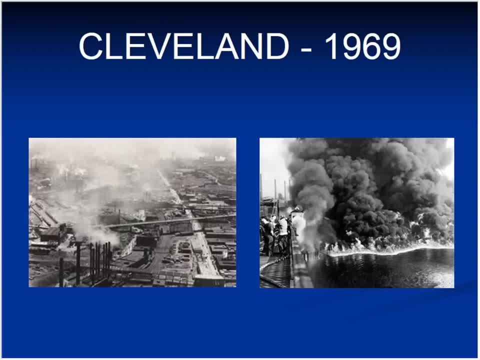 It wasn't a big deal. It wasn't the first time the river had caught fire. It wasn't the first river to catch fire, But it just happened to happen at a time when the environmental movement was really starting to get some wheels and, I think, a lot of. 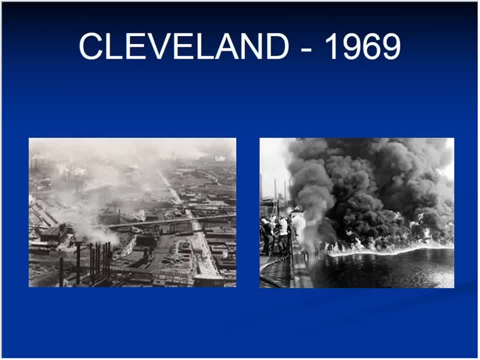 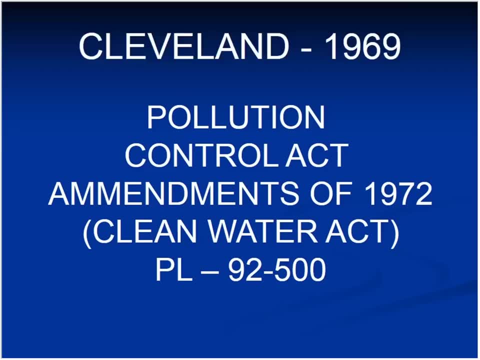 I guess the residents And they finally came across this picture, and that was the turning point for us. Our rivers will burn. what else do we have to wait for before we finally get something? As a result of that, we ended up with what we call the Clean Water Act, an amendment. 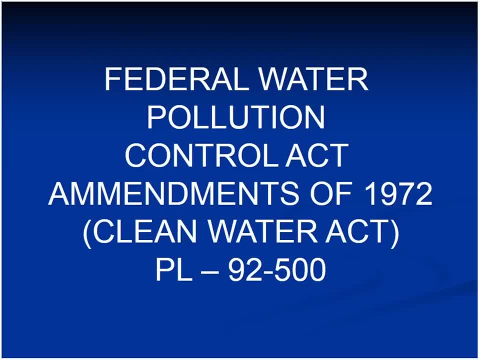 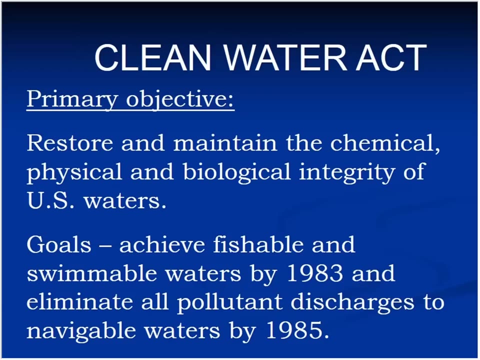 to the Federal Water Pollution Control Act of 1972, Public Law 92-500, which brought in billions of dollars for training engineers, training operators, building plants, upgrading green plants, easily turning over the whole aspect of wastewater control, And their challenge was to make them fishable and swimmable by 1983, and eliminate all pollute. 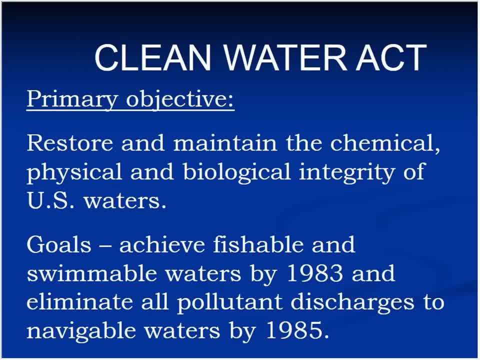 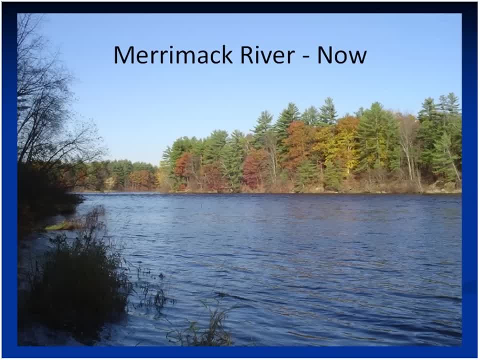 discharges, which is a pretty lofty desire to down the waters by 85. And they did that very, very well. It went over very fast. This is the Merrimack River now. I live just a mile up the hill. 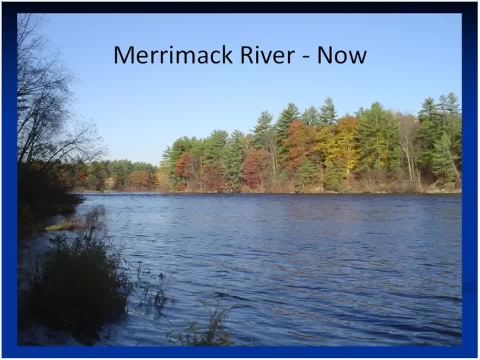 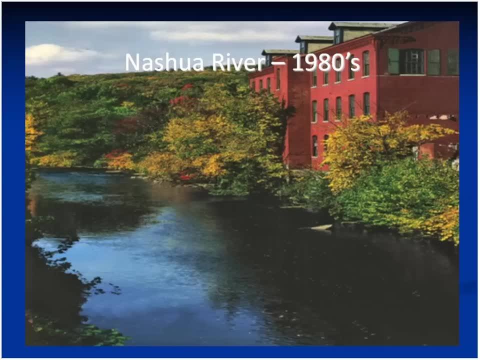 People are jet skiing and fishing. Lowell's got a swimming beach on the Merrimack River. The National River is a scenic waterway. now They have fishing tournaments. It's a beautiful thing. I like to go kayaking on it. It's very nice. 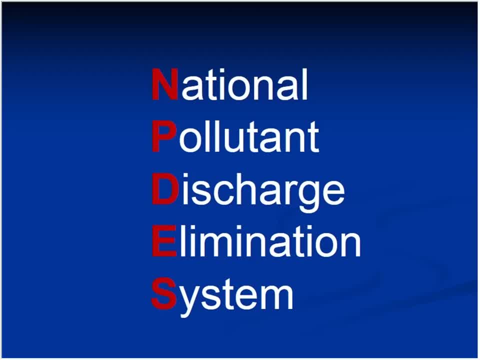 So, again, what came out of the Clean Water Act is the National Pollute Discharge Elimination System. That's what regulates all discharges for the waterways of the US. Any treatment plant that is a direct discharger has a NPDES permit, whether it's a municipal. 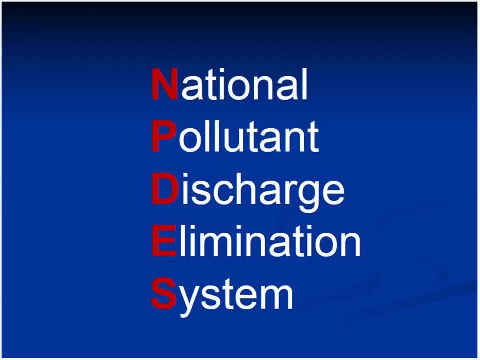 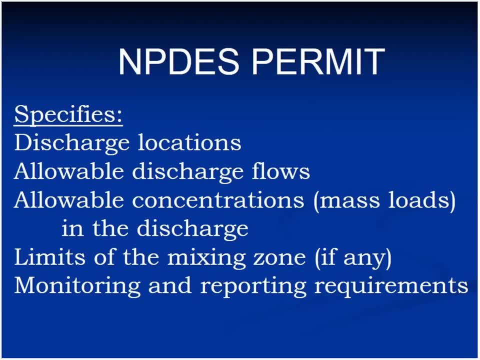 plant or an industrial plant- I had one because I was a direct discharger, even though I wasn't a municipal operation- And permits- and take a look at a permit. now they just get larger and larger and larger with the stuff that's being thrown in there where you can discharge what your allowable. 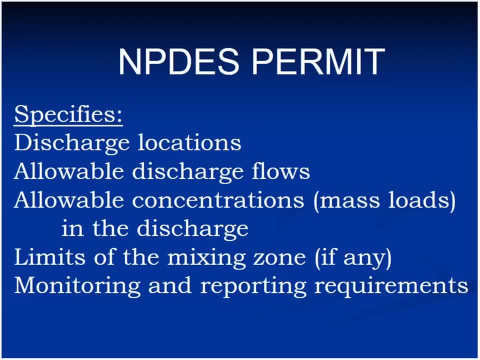 flows are all sorts of stuff. They break them down by seasonal limits for various things. It's very important that operators understand what's going on there. They've got to monitor and report. All of that is laid out there. It's very, very detailed. 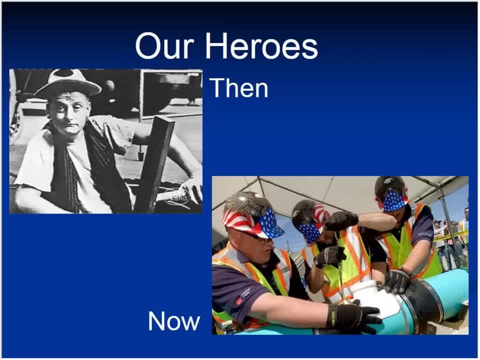 This is being in this business is kind of strange. when you talk to people, You familiar with. this guy up here in the upper corner. The more I teach, the fewer people know who that is. What do you know? That's Ed Norton up there in the upper left corner. 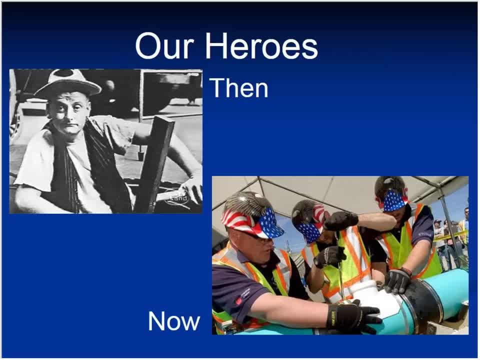 Ed Norton was on a TV show with Jackie Gleason called The Honeymooners And he is a. He's the only sewer worker ever to be on TV. You know the show with the sewer workers. they show the difference. Ed was a great guy. 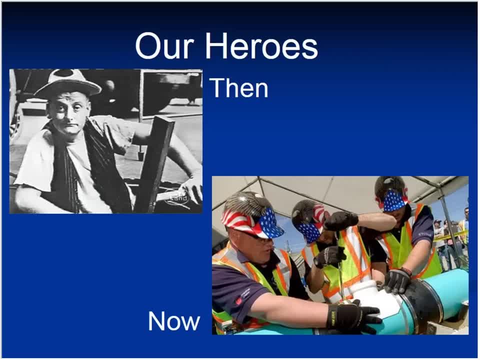 But you know, if you wanted a friend, he was right there with you all the time. But he was about a four-watt bulb And when you tell people what you do, that's kind of What's the matter with you. 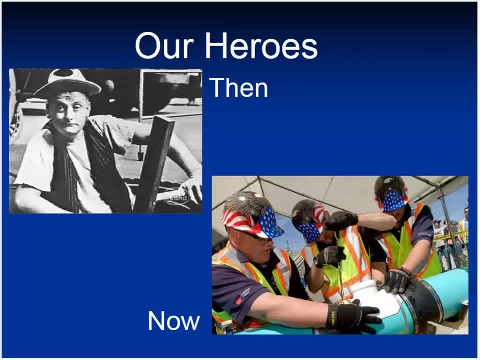 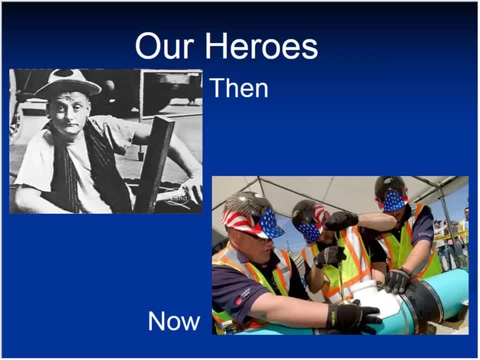 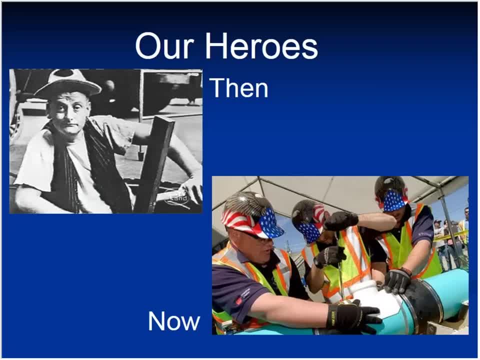 We just did it in conjunction with NIWIA last spring. It's a competition between operators in five different categories and it's really quite something. We get a chance to go to WEP or even to the spring meetings- something to watch. these 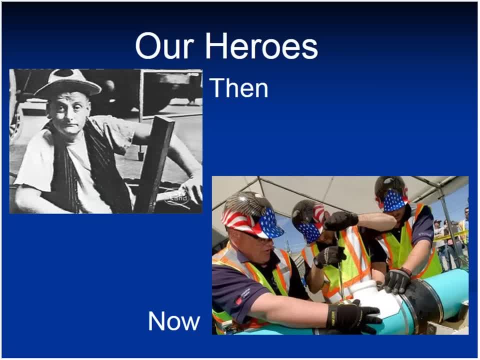 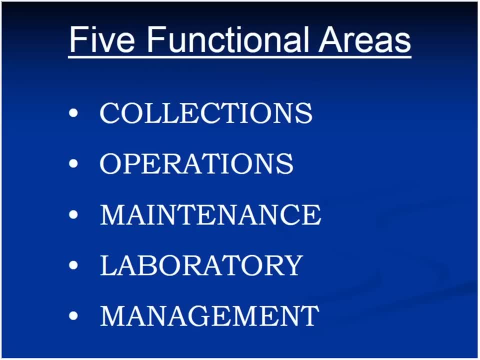 guys go to work. It's quite a bit different from here to there the amount of technology involved in this business. So we look at wastewater areas that people get involved in. We have the collection systems. Collection systems are what we used to call sewers, but sewers is kind of a nasty name. 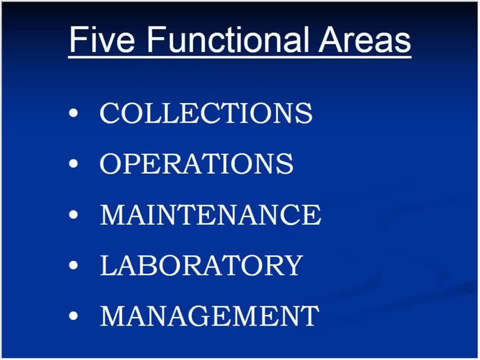 now. so we call them collection systems Operations. that's where all the fun is, if you ask me, is maintenance. the lab, which does a lot of the analyses for the operation, helps a lot with process control. and certainly there's the management, which is why we developed our management training program to try to 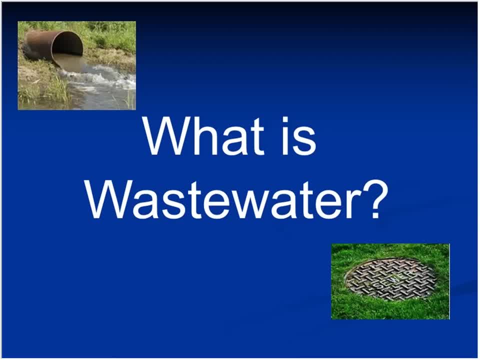 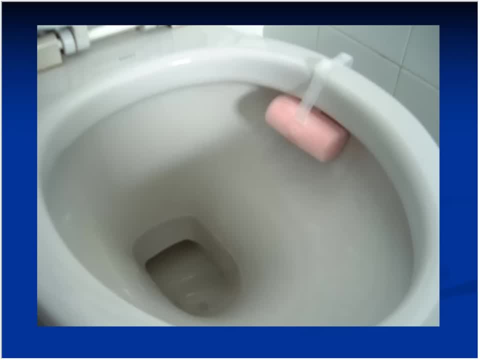 drive people into that position. So when we talk about wastewater, you kind of know what it is, but really, if we break it down a little further, what are we talking about? You don't have my sound there, but we know what goes down there. 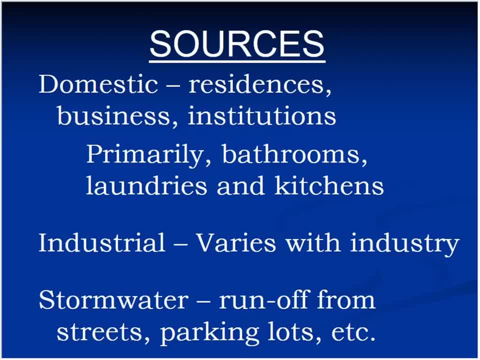 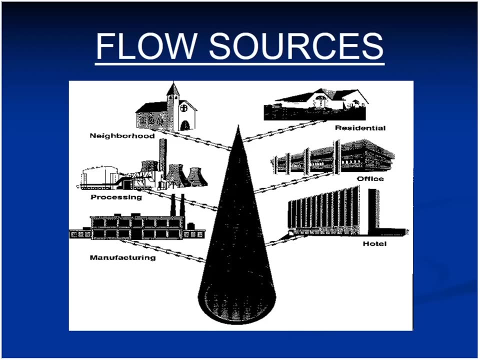 Domestic wastewater is from residences, schools, commercial establishments, industry. We also have in most communities we have stormwater mixed in with our wastewater. As much as we'd like to separate it, we still have a lot of that getting in there. 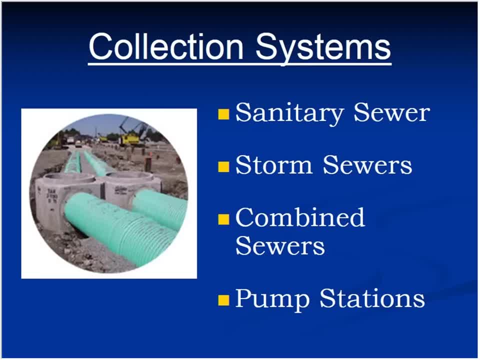 Again, it pretty much comes from everywhere. We talk about collection systems. we have a sanitary sewer which will handle domestic wastewater from houses, from industries and what have you. You may also have storm sewers which are totally separate. Ideally, every town should have a separated system. 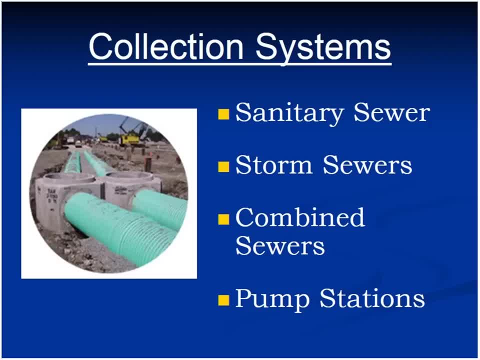 Rainwater is just water. It really doesn't need to be treated. We don't need the extra volume going through a pipeline. We don't need to go through a plant, just wasting some money on it. But again, we're in an old part of the country where if there's a pipe on the ground, you 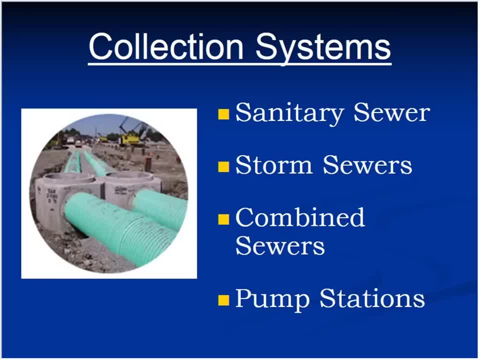 might as well use it. So we have a lot of cities that still have a lot of combined sewers. That means everything goes into one pipe, and that's why New Orleans has that extra billion gallon of rainwater. We also have pump stations. 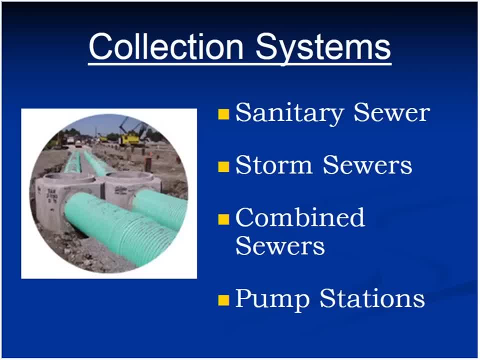 We're not living in flatland Illinois. We've got to get over the hills, So we've got pump stations out there to help get us over those high points. When you look at what's in there, it's a lot of different things. 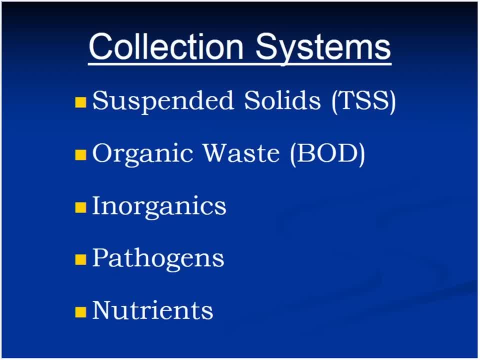 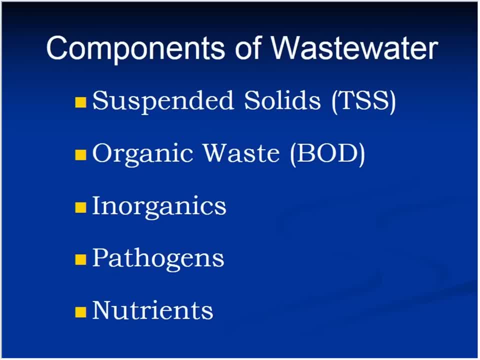 oxygen demand BOD and total suspended solids- TSS. In the initial NPDES permit these limits were set at 30-30, those two prime things that they were out to reduce. We have some amount of inorganics. 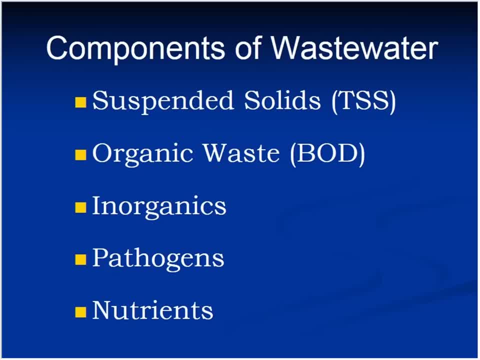 Those are dealt with through a preliminary system. try to remove those as much as possible. We also have the pathogens. Do you know what the pathogens are? Disease, Disease-carrying bacteria. We don't know who they are, so we treat all of this water as though it's pathogenic, disease-carrying. 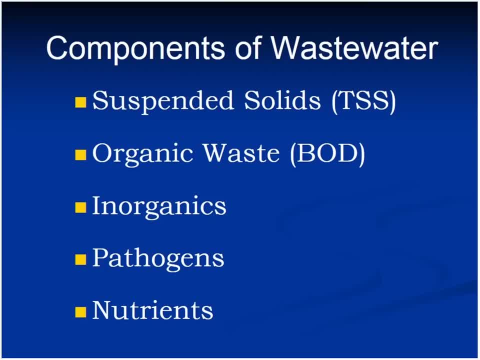 So we've got to be very careful. It's one of the concerns in working on these facilities. And we also have the nutrients. This is the big issue now, because we did a very good job on reducing BOD and TSS. That's a pretty simple job really to reduce BOD and TSS. 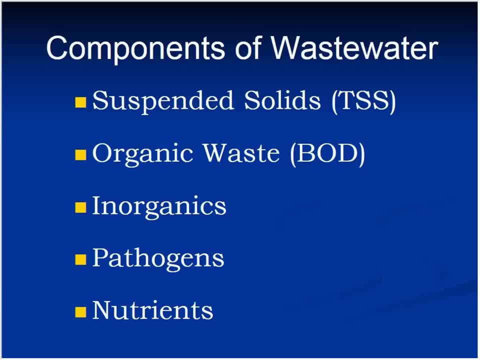 So we've got to be very careful. Thank you, That's a pretty simple job really. The nutrients is a whole other issue. We're talking about nitrogen and phosphorus. Those are the components that cause the eutrophication. You might have grown up in an area where, down the road, you had a nice pond that you could. 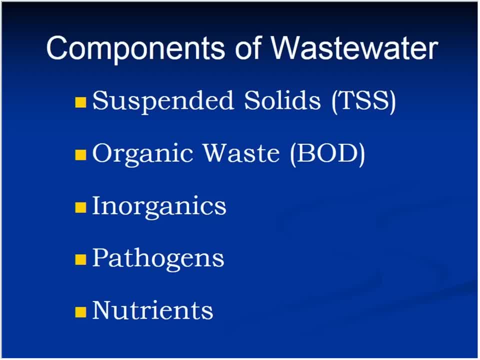 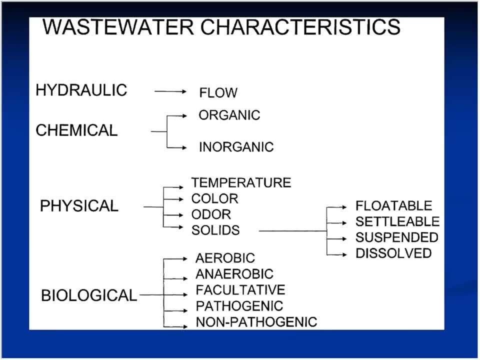 use all summer long and now it's just a bog because it's filled up with weeds and everything. They die off and slowly choke over there. So four components of wastewater that we have to consider. First of all, the hydraulic. We talked about the hydraulic component. 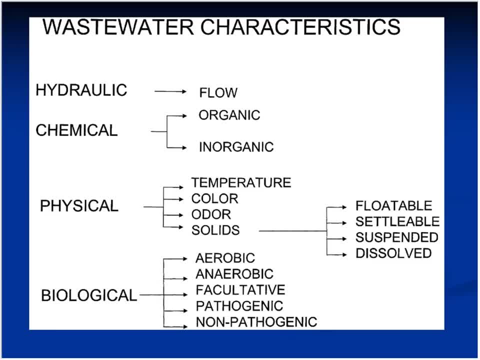 We're talking about the flow to the treatment plant. Chemically, we have largely organic matter we're concerned with. We also still have to be concerned with some of the energy, Physically, temperature, color, odor, And we have solids, and solids of various types. 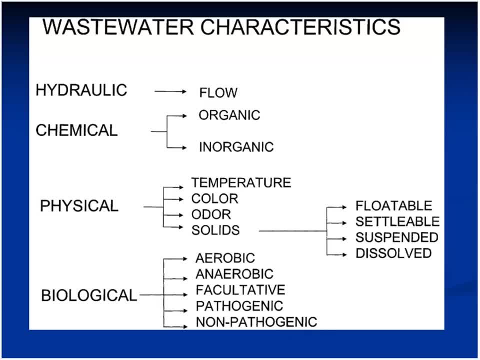 We have floatable spettable, suspended, dissolved. We'll talk about these in a little bit more detail. From a biological standpoint, we have organisms that work under various conditions. We have a lot of different types of organisms. We have a lot of different types of organisms. 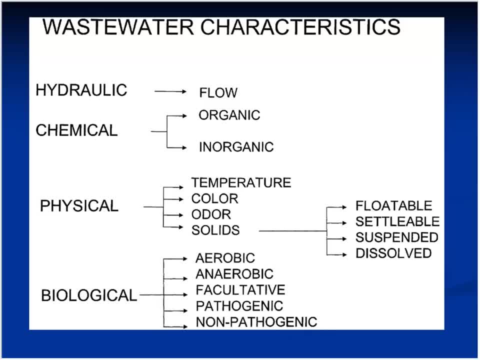 We have a lot of different types of organisms. We have various situations. Largely, we deal with aerobic bacteria. They like free dissolved oxygen in order to survive much the way we do. We also have anaerobic bacteria who function very well in the total absence of oxygen. 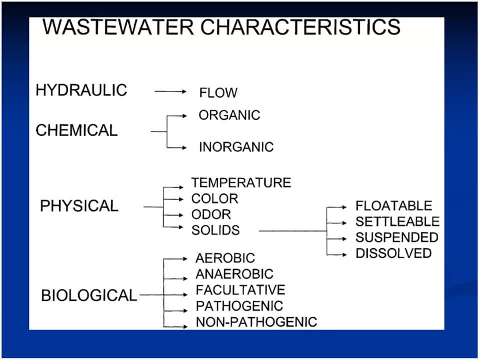 We try to avoid that as much as possible because they tend to stink the place up. But there is a time when they work to our advantage, so we may do that at some point. But largely we talked about this middle one here. facultative bacteria. 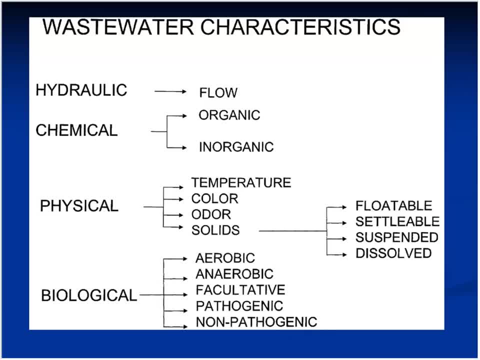 They'll adjust to the situation. If you have oxygen, terrific, they'll use it. If you don't have oxygen, they'll find another source of energy. And of course we have the pathogens and the non-pathogenic. So hydraulically we talk about the floor of the plant. 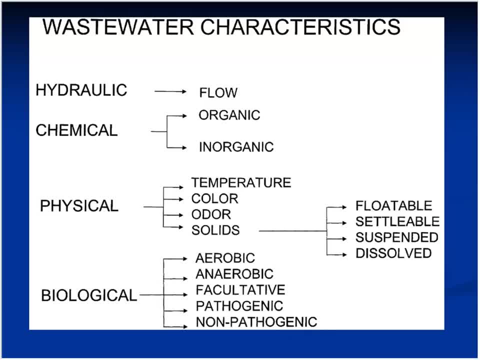 Just you yourselves, probably 60, 70 gallons a day. When you encompass everything else we go into work and everything else that happens through the course of the day, that's about 150, 160 gallons a day. That's the amount of oxygen that comes out. 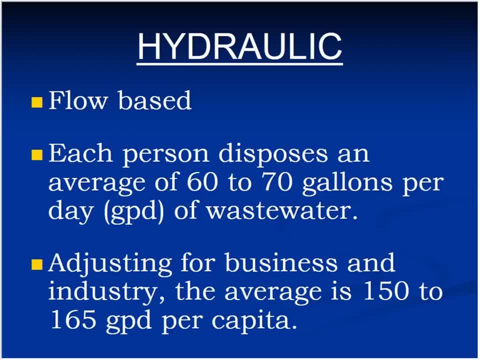 That's a lot of oxygen, And how much oxygen do you need to be able to use? How much oxygen do you need? How much oxygen do you need to be able to use? How much oxygen do you need to be able to use? 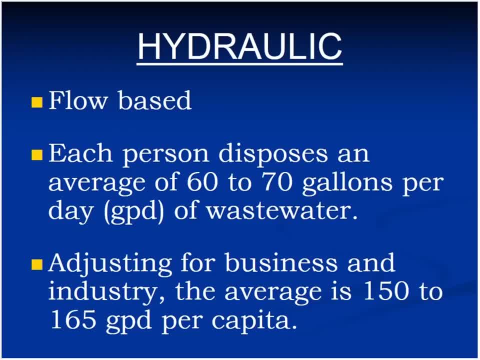 How much oxygen do you need to be able to use? When we talk about the flow to the plant, just you yourselves? probably 60, 70 gallons a day, When you encompass everything else with going to work and everything else that happens throughout. 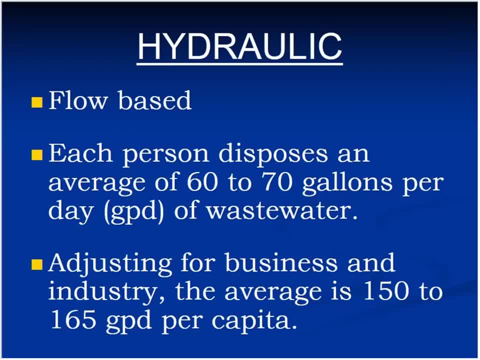 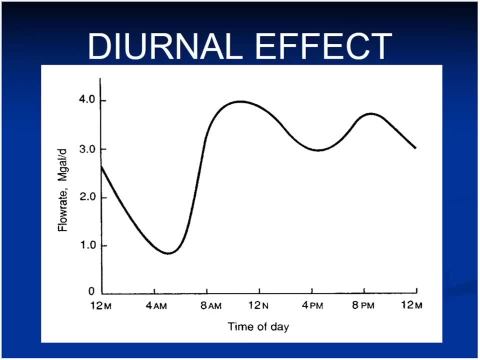 the course of the day. that's about 150, 160 gallons a day per person. So if you know how many people are in town, you can kind of guess the size of the system. What this particular graph is showing you is what's called the diurnal effect. 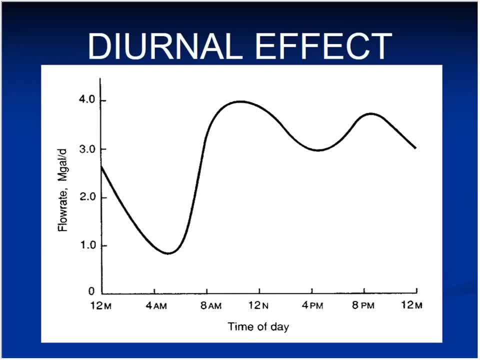 It reflects the flow to a treatment plant based on the activities of people over the course of the day. What you see here is, if you start here at 12 midnight, we've got a flow rate of about 2.6 million gallons and it just drops off steadily down to about 5 o'clock. 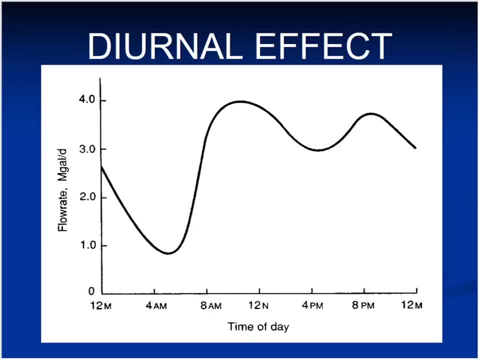 Everybody's home and in bed. You've got some 24-hour operations, late night at Taco Bell and that sort of stuff, but not much is going on, So the flow drops off. Then, at 5 o'clock, what happens? The alarm goes off. 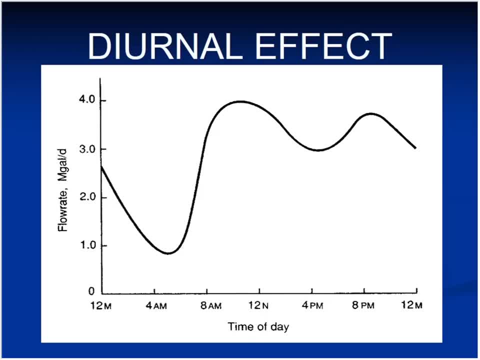 You've got to get up, You've got to get the kids ready for school, You've got to take a shower. Dunkin' Donuts is backed up into the street and everything else. The flow goes up dramatically up to midday. 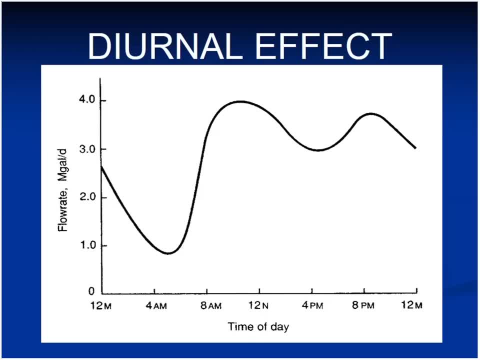 It peaks off a little bit. I guess people are taking a siesta or something. but 5 o'clock at night now you've got to do the laundry, You've got to give the kids a bath. It bumps up again and then slowly goes up. 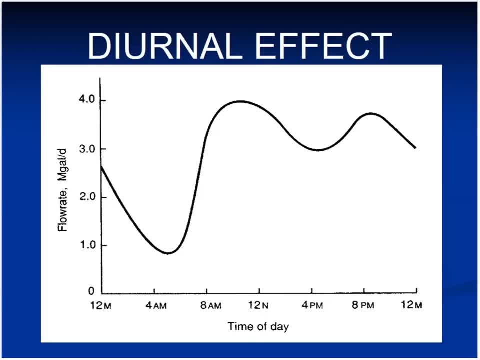 This will vary considerably depending on the size of the facility. In a small town you see something as dramatic as this In Deer Island. it's basically a flat line. They get stuff 35 miles away from Framingham, so it really balances out quite a bit. 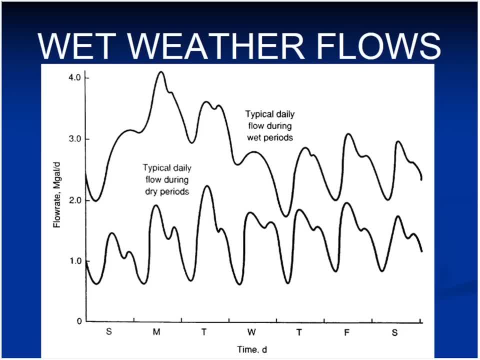 What we're seeing here is the difference between. the bottom line is you can see that same sort of diurnal effect going over the course of the week. The upper line indicates what happens during the rainy season: All that additional rainwater getting in requiring you to work that much harder. 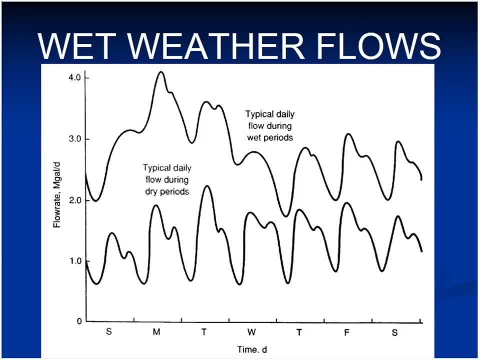 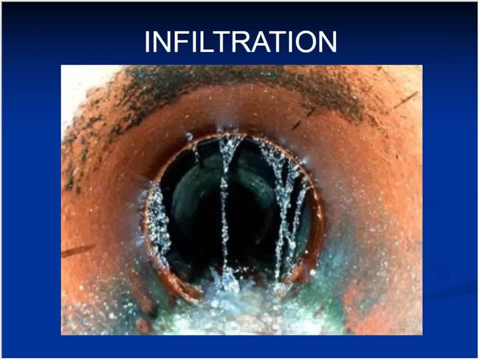 But basically, you're treating the same amount of consistency, You're treating the same amount of constituents, except for the fact that a lot of it's just water. This is the problem. Two things that are causing that issue, even if you have a separated sewer system, is what? 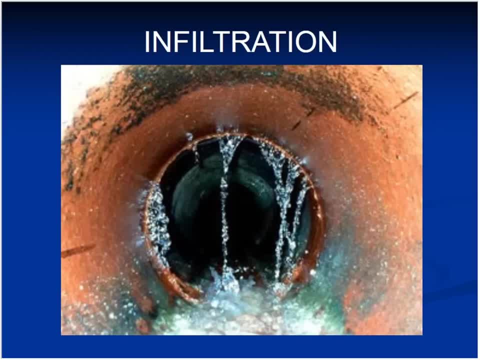 we call I&I First. I is inflow. Inflow is a result of poor condition of your collection system: Cracked pipes, broken pipes, poorly installed pipes, bad joints. Rainwater comes percolates through the ground as you want it. 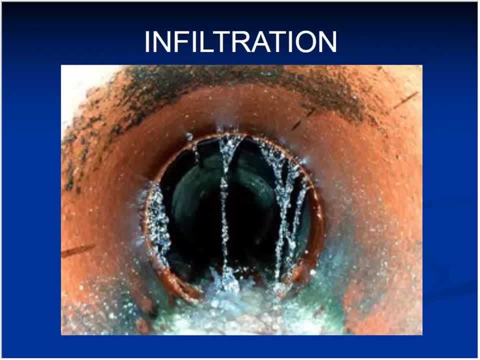 But then it sees this big 36-inch pipe. that's just open space. It's a whole lot easier to go in there than to fight its way through the gravel And it comes, And that's just extra flow of the plants make life harder. 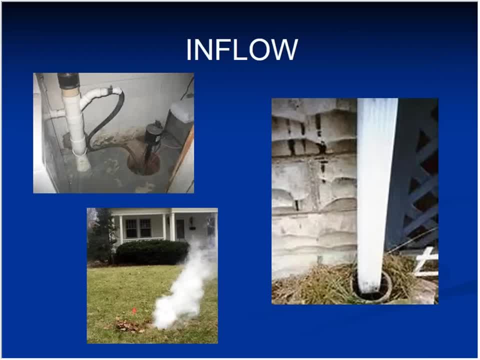 Really that's infiltration? Yeah, It's inflow. Inflow is illegal connections. Roof gutters are very important, A very common thing throughout the Boston area And a lot of work done to remove those things. Some pumps that are hooked up into your waste system should not be there. 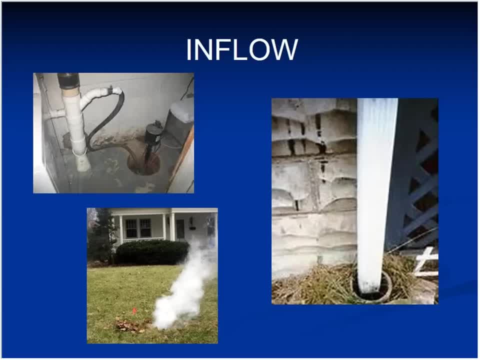 It should just be pumped back outside. And this is this bottom picture with the smoke coming out of the front yard- is a technique that collection system operators will do from time to time to tie the tap down to legal connections. So they'll put a little smoke bomb in the sewer and see where it comes out. 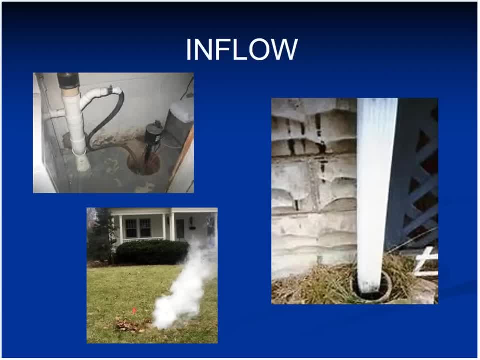 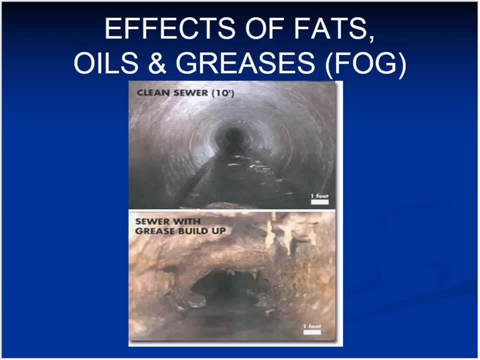 It could be quite humorous. The other issue- that is an issue, a problem, particularly during heavy rain periods, is what we refer to as fat soils and greases, or fog. Grease and oil should not be dumped down into the system. Baking grease should not go down there. 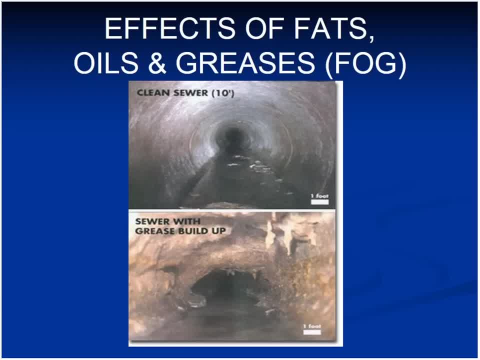 You don't say, well, I'll run the hog water, throw a little down there and chase it out. At this point it's going to hit some cold pipe and just play it out. The top picture is a nice clean pipe. 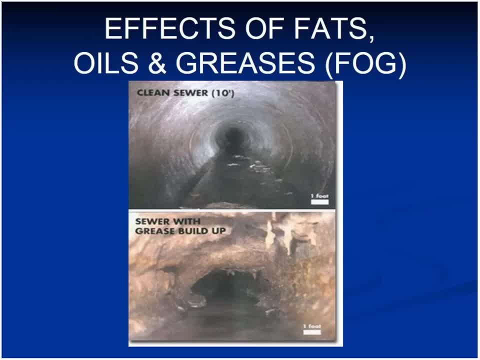 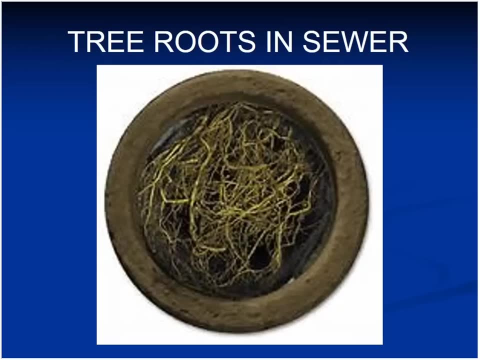 The bottom one is after years of being down the street with the clam shack and whoever The thing is. as that pipe diameter clogs up with grease, its ability to take flow is greatly reduced. So when you do get the big rain, you've got a problem. 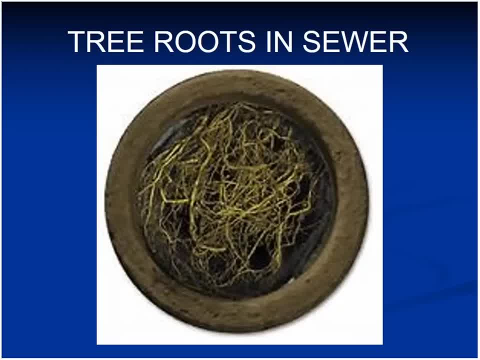 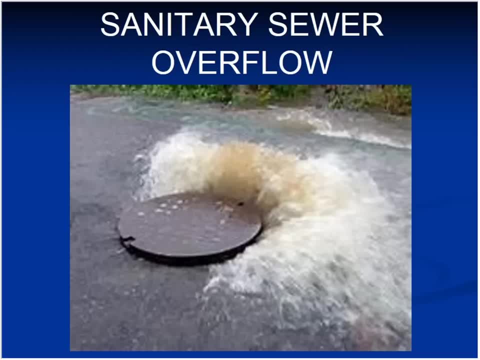 Three roofs And what is being done? that's what happens when the big rain comes and it can't fit through that pipe anymore. For any number of reasons, That is a violation. That's a sanitary sewer overflow. The permit does not say you can discharge there. 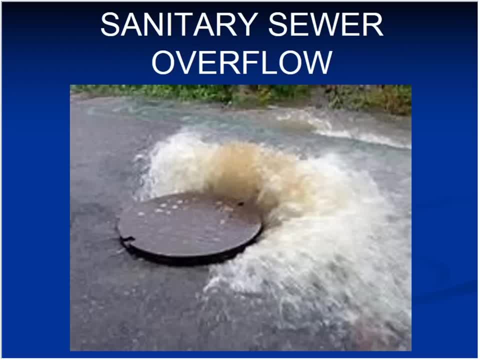 And really, when it comes to fat, soils and greases, it's actually the homeowners that have the biggest problem, much more so than a lot of the restaurants, though they can be an issue. Restaurants have grease traps installed, not always installed properly. 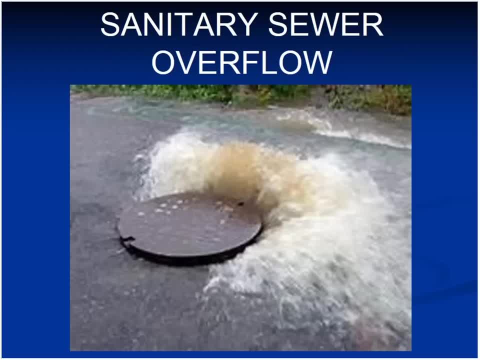 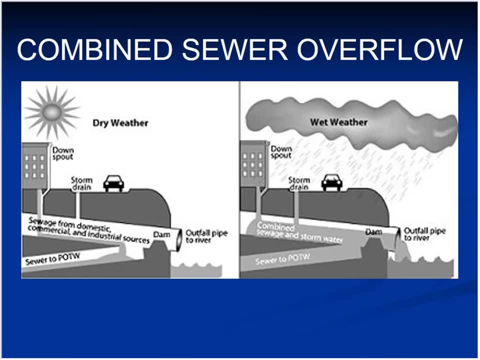 They're inspected generally by the health department, who doesn't necessarily understand how these things work, So that could be an issue for them. Here we go, Not good. You may have heard the term combined sewer overflow. This is a situation that's installed in a collection system in order to protect the plant during extremely high flows. 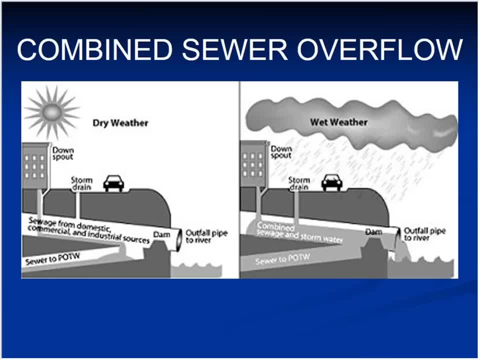 When you think of it, and we'll learn about these guys next week- but we're dealing with single-cell bacteria. Ninety-five percent of the organisms in the world, including wastewater treatment, are single-cell bacteria And if you just triple the flow through a plant, they can't swim upstream that well. 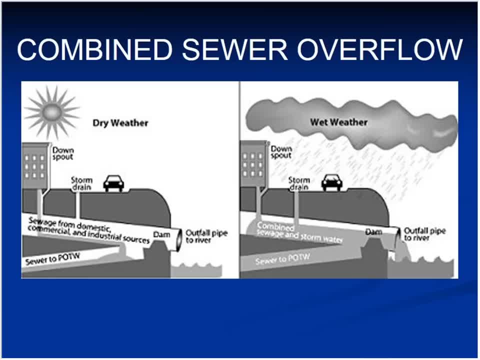 And if you don't protect your plant, you're liable to lose all of your bugs to the river. It's not a good thing. So in a high-flow situation- combined sewer overflow and what we see here is the dry weather- your collection system is built such that your typical flows will hit some sort of a barrier. 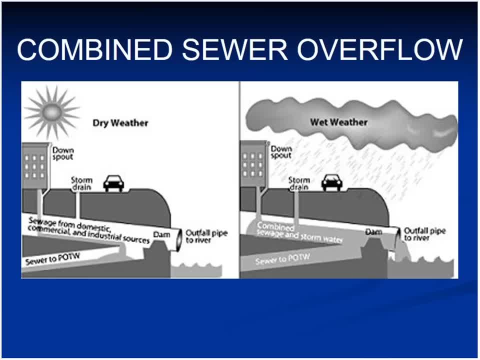 and continue on to the POTW, publicly owned treatment works. the treatment plant, But in extremely high flow. it will allow a certain amount of that to go straight to the river. Unfortunately, what that generally does is it causes all sorts of grief with the residents. 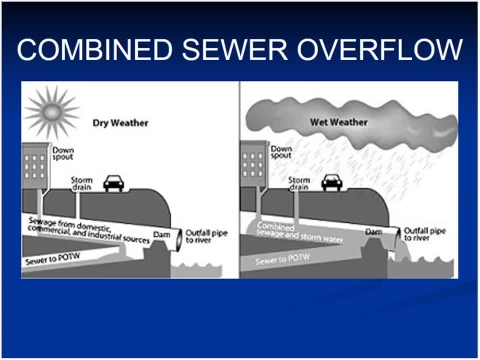 It shuts down swimming beaches from time to time It can be Folks out. in New York State you can look at the Gowanus Canal a bit Kind of tells you what's happening there. If you ever saw that video it would be really nasty during a sanitary. 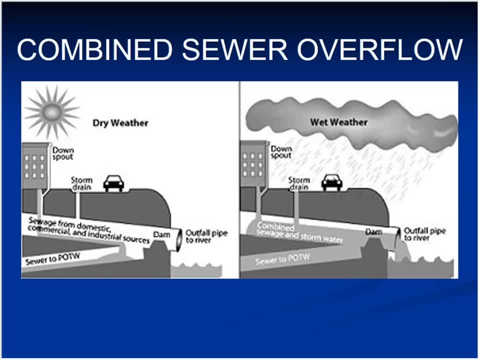 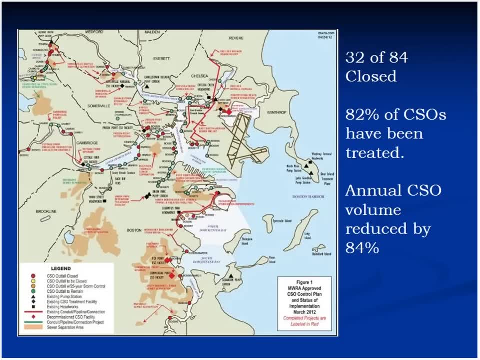 Combined sewer overflow. Increasing leaves are being set up. This is the Association of Boston. how many they had and they've reduced them. They've closed 32 out of 84, at least at the time of this slide, Reduced quite a bit. A lot of them are being designed so that they actually have some amount of treatment. They'll remove grits and solids and they'll also disinfect. So you're not maybe putting water out there, but at least you're taking care of the pathogens. 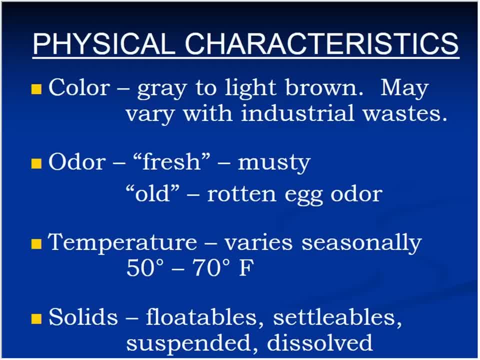 And the whole collection system is being put under scrutiny through a process that we refer to as CMOM: Capacity Management, Operation and Maintenance. It basically says that you have to maintain your collection system. You have to inspect it on a regular basis, find those leaks, cut out the tree roots and all that stuff. deal with the grease issues. 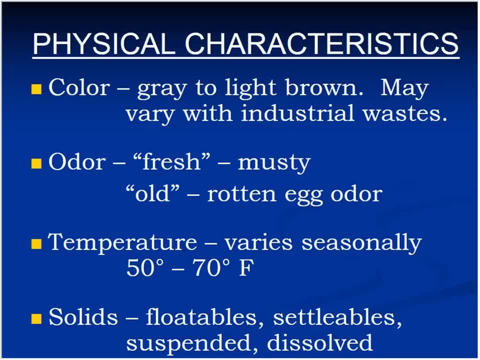 There's been increasing enforcement on that end over the past several years. Physically, when we look at this water coming into the plant, it's typically a gray to a light brown. It can vary depending on what industry it's putting in there. 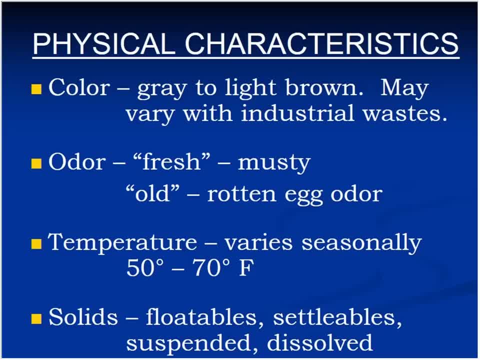 When it's fresh it has a musty odor. You can imagine that I should not be obnoxious. If it's got that rotten, eggy smell, then it's definitely old And that can happen for a variety of reasons And it has to be dealt with. 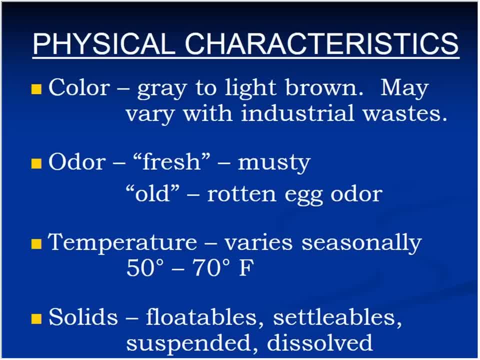 From a temperature standpoint, we get what we get. It's a lot of water. We can't heat it. We can't heat it up, We can't cool it. This time of year the water coming into the plant gets down close towards 50 degrees Fahrenheit. 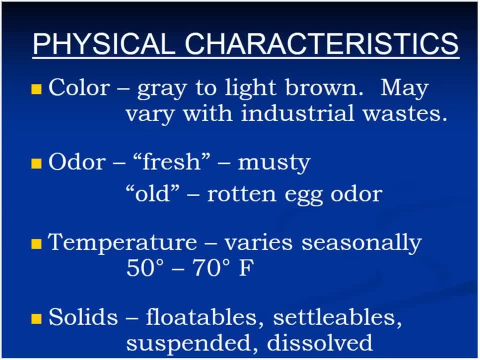 Pretty well insulated, but still the cold will get down there. Summertime it's up around 70 degrees, And what that does to us is we have to operate our plants slightly differently in the wintertime than we will in the summer. 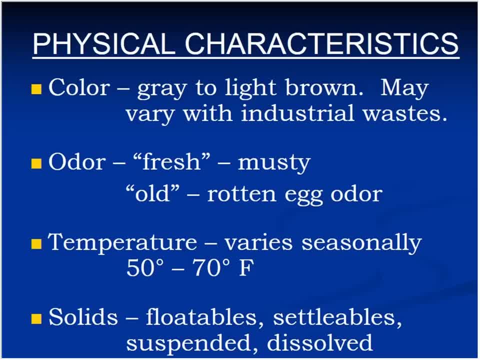 Because, much like us, bugs don't do as well in cold water as they would in warm water, So we have to adjust to that as the seasons change And again, from a solid standpoint, we have floatable, settable, suspended and dissolved. 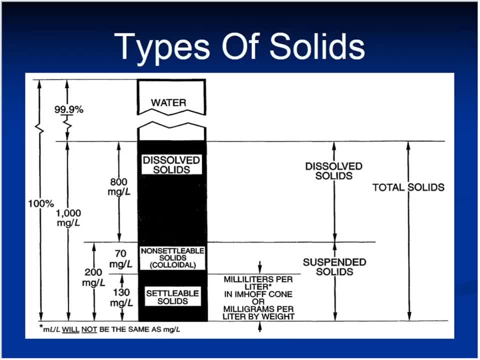 If we were to take a one-liter sample of our wastewater coming into the plant to do a solids analysis of it, you would find that really 99.9% of that inflow is just water. All of this work is done for one-tenth of one percent of what comes into the plant. 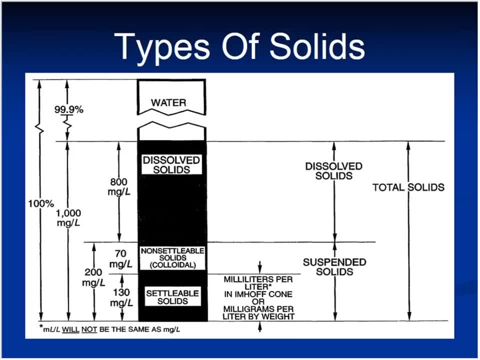 We have settable solids. These are solids that if we take a sample, set the jar on the bench and let it sit there for about a half an hour, they're all going to drop to the bottom of the jar. The non-settable solids. 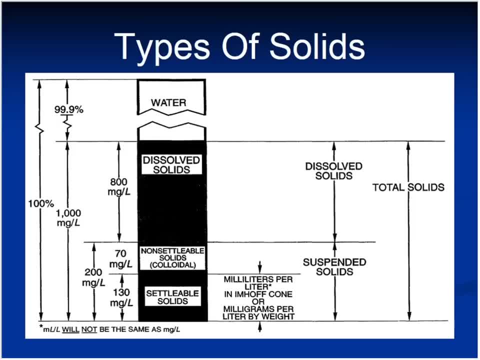 that stuff is just going to hang there and make that water look murky, no matter how long it sits. Colloidal material is very small, same density as water. It's got no reason to go up down sideways And then we have a larger portion of dissolved solids. 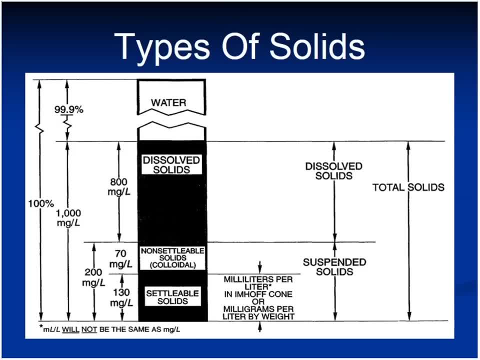 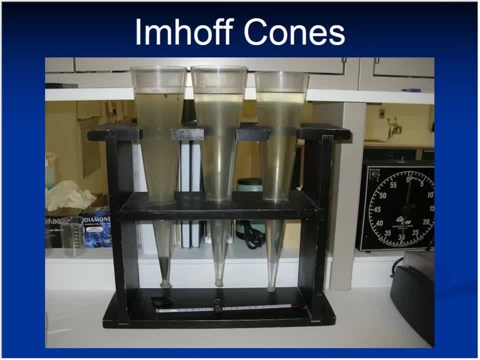 Soluble material that doesn't settle out, doesn't filter out. That's where we really rely on the organisms to do the work. You see in this picture is Eimhoff combs. This is how we test for settable solids- Basically a one-hour test. 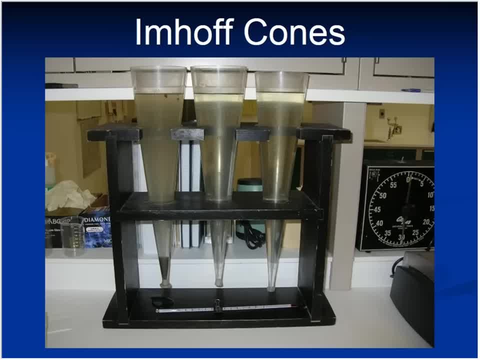 Put a one-liter sample into the cone, Let it sit for 45 minutes. At that point you take a stirring bar and just gently rub the wall to make sure nothing's clinging. You give it another 15 minutes and it's a direct read. 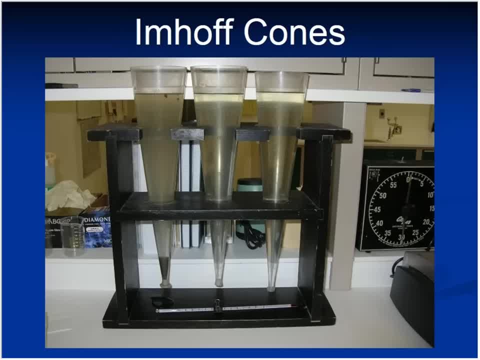 You can see what's coming into the plant. That's the bottom portion. Those are the settable solids After primary treatment. there should be nothing there. You can remove those quite easily. You get a little bit of floatable stuff, But we have no measurement for that. 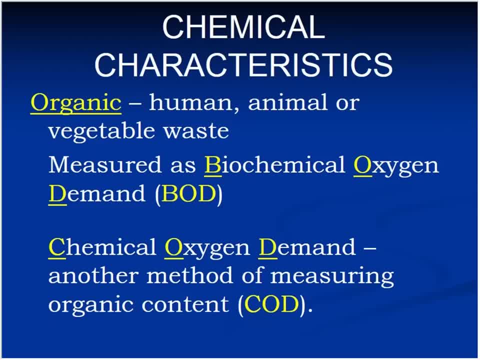 Organically again dealing with human waste, animal waste, whatever you grind up in your kitchen sink disposal, all comes down to us, and it's measured as biochemical oxygen demand. Biochemical oxygen demand is an indicator of the organic strength of the wastewater. 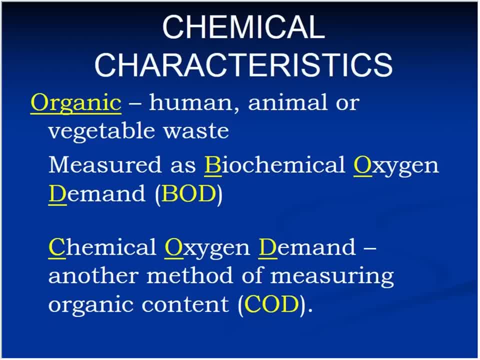 It's not a real thing. It's kind of a weird test. It's a strange way to run an operation. Another test you can do to get some ideas to the strength of the organic matter in your wastewater is a chemical oxygen demand- COD. 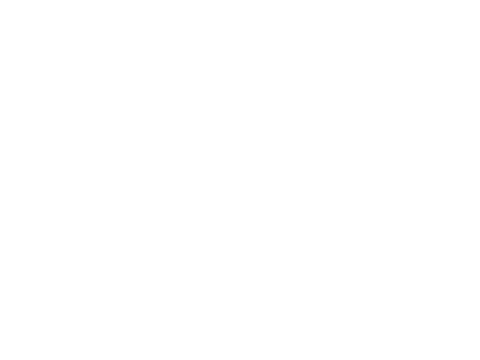 COD is a chemical digestion of organic matter, The difference being a BOD test, which is a five-day test. Take a sample today. We're going to prepare it. put it in an incubator at 20 degrees Celsius for five days. 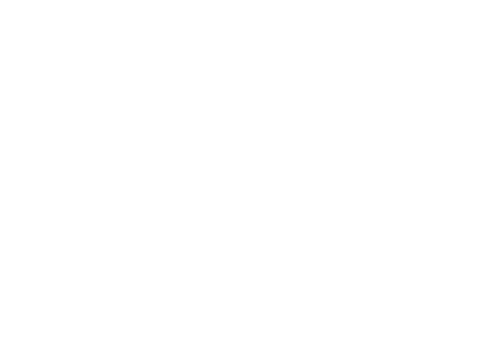 It has to be in the dark. You don't want to generate any algae growth, because algae is. We read the amount of oxygen in this sample before we put it in. We read how much is out there and we do a calculation. Again, this is a permit limit on any treatment plant. 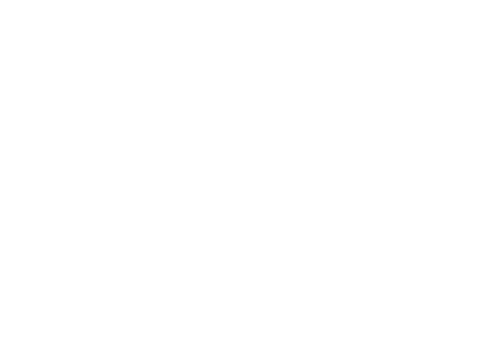 The weird thing is you find out five days from now that your plant is in trouble. Not a fun way to run A COD. you can get an answer in about three to four hours. My operation was completely different in that I had seven different production areas. 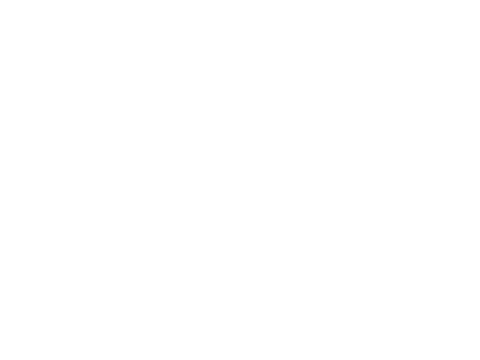 that could drop anything at any time of day. I couldn't wait five days to tell if I was in trouble or not. We ran CODs on a regular basis. By and large, EPA wants to stick with VODs as their test solution. 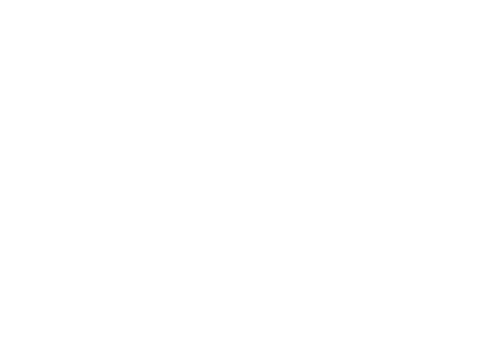 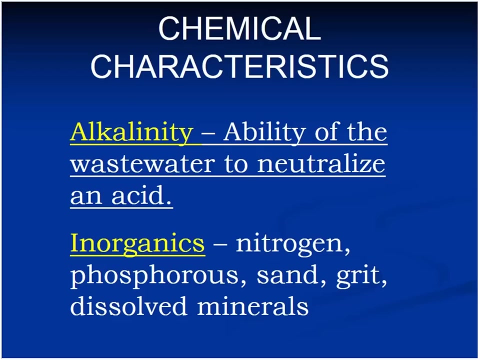 We have a lot of things to worry about. A certain amount of alkalinity coming in. We may need to adjust that from time to time. We'll talk about when that's required. In organics we have nitrogen and phosphorus. Those are the nutrients we're going to be dealing with. 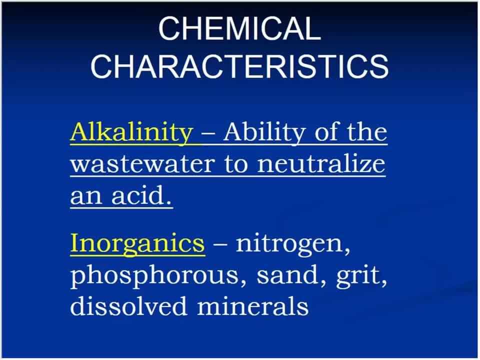 Sand and grit This time of year, particularly in a combined system. we've got salt and sand thrown all over the streets, Then it rains. It all comes into the plant. We've got that extra load in That's coming in. 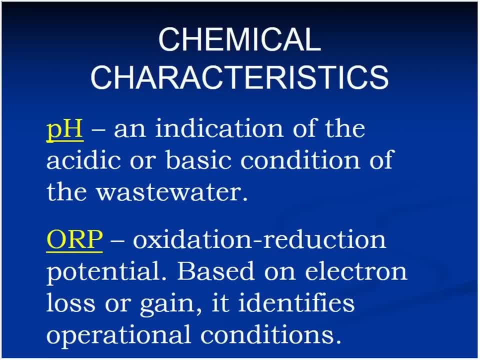 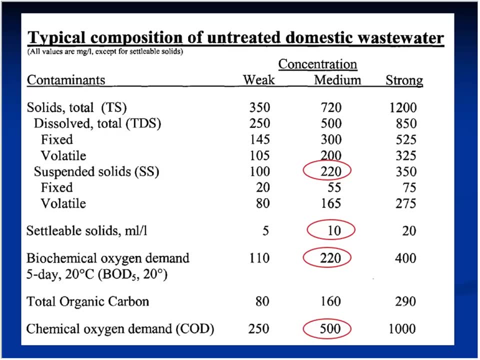 pH doesn't vary too much. We have to maintain that. Make sure it's in the proper ranges for the various operations we're doing, whether doing nitrification or phosphorus removal, ORP. some plants are using that as a method for control. 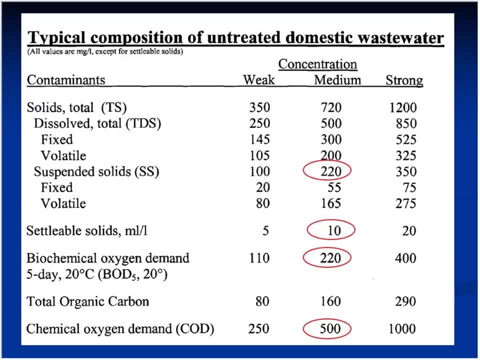 Look at total analysis of wastewater coming in. There's a medium suspended solids coming in On average somewhere around 200 milligrams per liter. Milligrams per liter, parts per million- pretty much interchangeable. Think of it that way. Our settleable solids: a small amount. 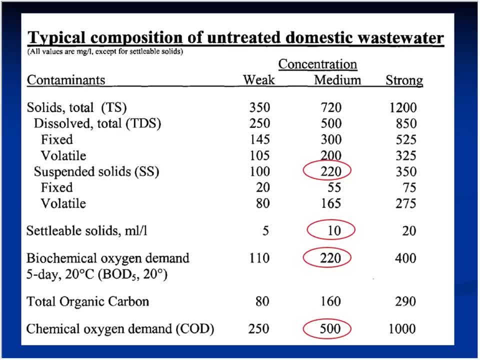 Our VOD. this varies considerably from community to community. Some are down to 150, some are up to 300. It's also a part of how tight your collection system is. That's typical range Somewhere: 150 to 300 is pretty normal. 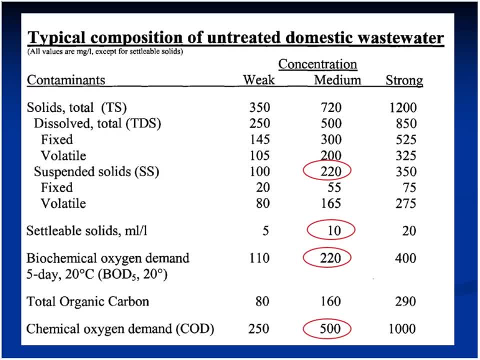 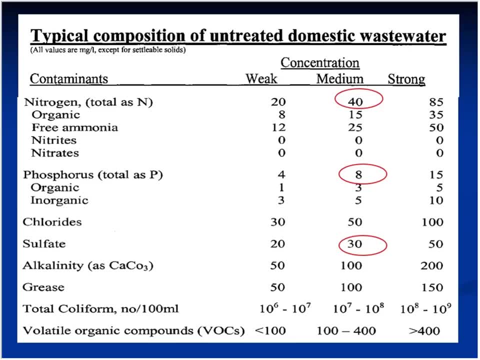 If you did a COD you can build up a relationship between the two. They can get some meaning out of that Nitrogen coming in at 40.. We're going to have to get down to very low single digits. Phosphorus: not a big number, but what we're looking at now is 0.1, 0.2.. 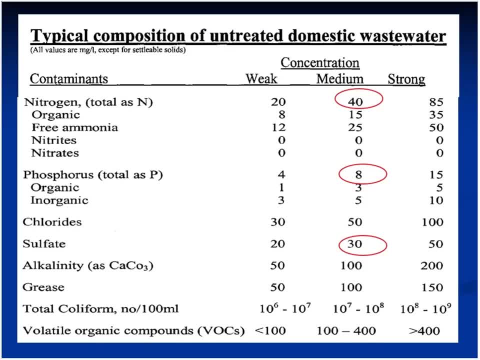 100 parts per billion. Not easy to do. Sulfates- Sulfates are only a problem towards an anaerobic situation, because that's where that rotten egg smells. in This one right here is one of my favorite ones. This is total coliforms. 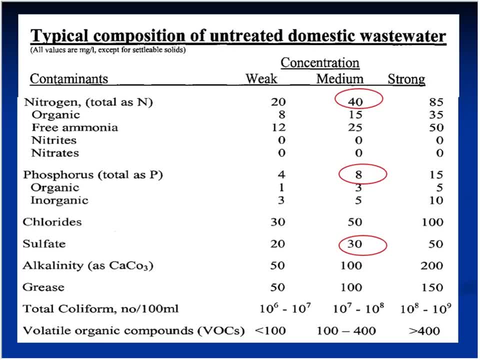 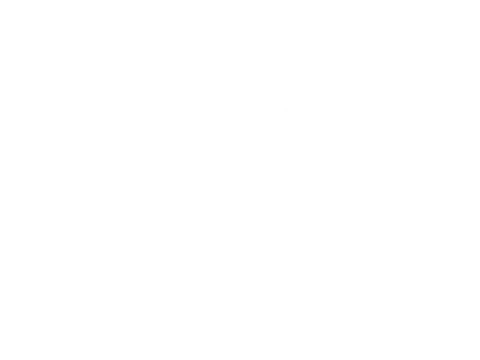 Coliform are a particular bacteria. We use them as an indication of various things Disinfecting if we've done a good job. They're very prolific, They're everywhere, They're in the ground. You probably carry around a few billion yourself right now. 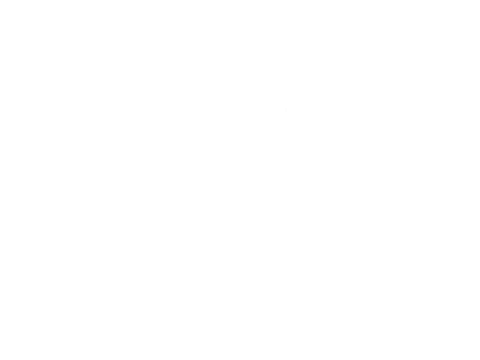 But this is what's coming in In 100 mils, Basically a shot glass. We have a shot glass. We've got, let's see, that's, 10 million to 100 million organisms in that one little. Have you ever seen those probiotic pills? 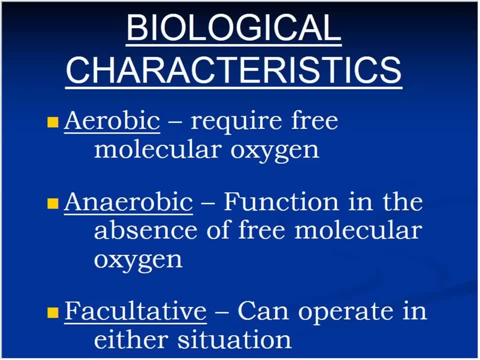 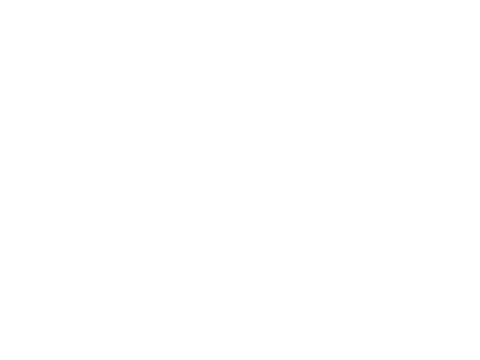 It's like 10 billion in one of those capsules. We try to keep conditions aerobic as much as possible. Aerobic bacteria use free molecular oxygen. They do a very good job of that. They do a very good job of that. Anaerobic bacteria: when all oxygen is gone, they're going to turn on that and that's. 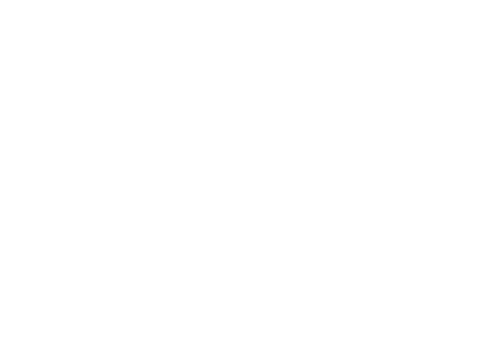 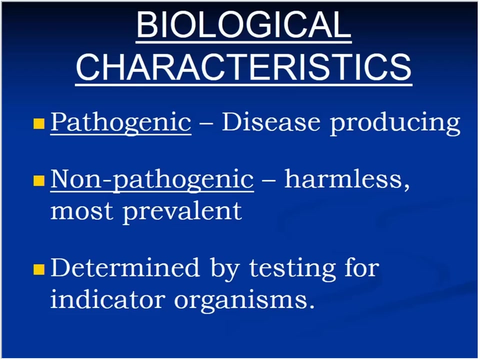 when things get kind of nasty. Facilitative organisms can go back and forth, and that's what the majority of them are. Talk about our pathogens. There's no way to tell who's who. We just assume they're all bad and deal with them as such. 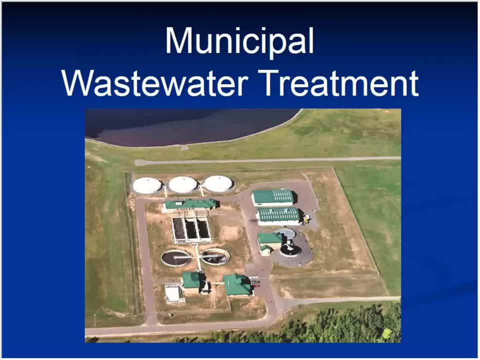 So how do we do this? Who's who. It's what a treatment plant is. Here's a term: POTW- Publicly Owned Treatment Plant. It's a nice little small one. I couldn't tell you where the heck it is, but it's a nice little plant. 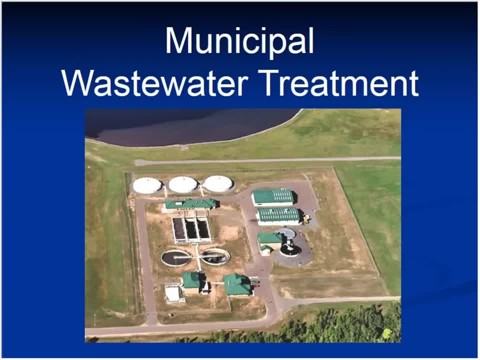 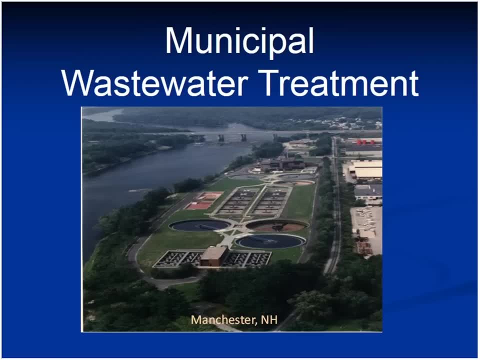 It's pretty compact, probably doing a million million and a half a day, something about that size. This is Manchester, New Hampshire. It's a 32 million gallon plant. It's right up there along the Merrimack River. If you ever flew out of Manchester you went right by this. 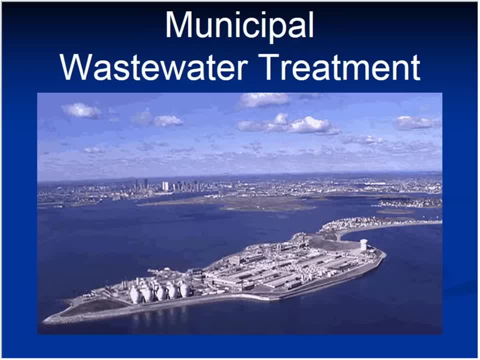 And then there's Deer Island with 350,000 gallons a day, 350 million gallons a day, Huge, huge complex out there in Boston Harbor. You can take tours of this place. It takes quite a while to walk around it. The unfortunate thing about it is you really don't see much of the water. 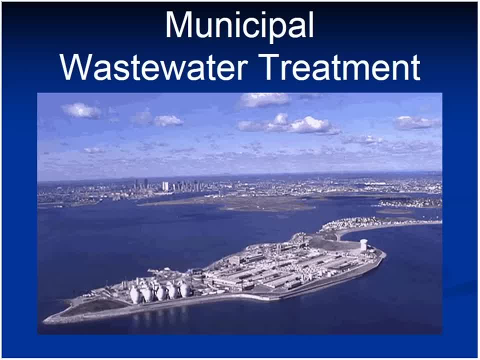 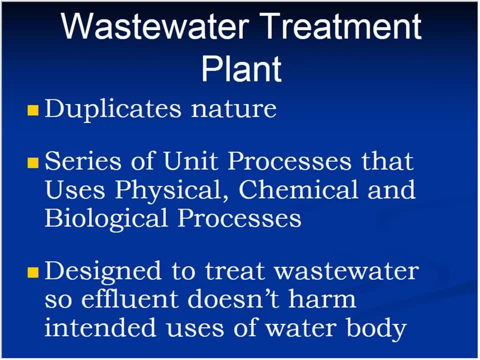 Most of the water you see is Boston Harbor. It's all largely closed system until the very end, right before it discharges out to the bay. So really, all we're doing with this process is what nature would normally do. We're just a little smarter, a little faster. 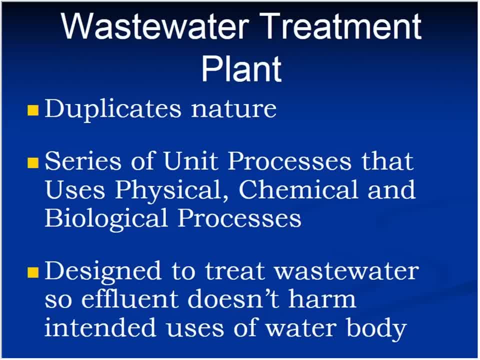 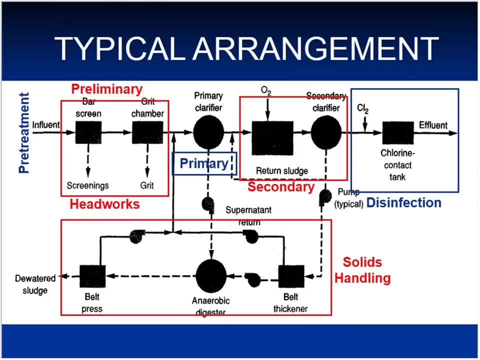 We don't have time and patience, as nature does, And we've got some physical, some chemical, but largely a biological process, And plants are designed to treat the wastewater, so our effluent does not harm the intended use of the water body to which it discharges. 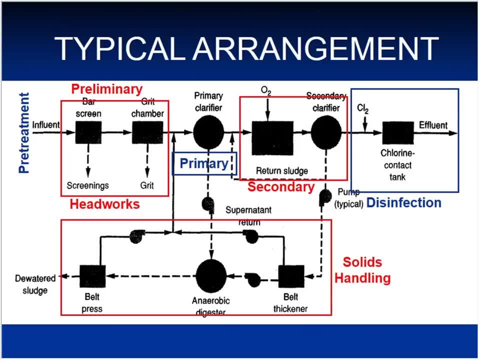 So what you see here is pretty much a basic flow diagram of everything that would happen in a treatment plant if you did everything. Everybody follows the water line, which is the arrows that run across the top of the page. Everybody's going to do that on one device or another. 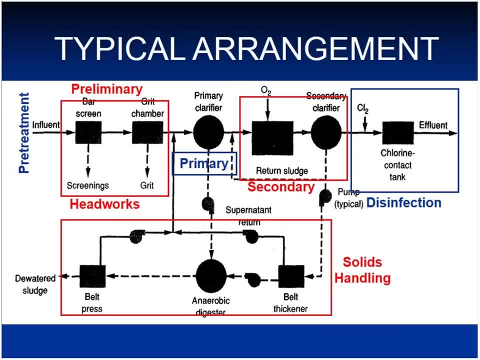 And there's a lot of different ways that this could be done. This bottom portion varies considerably from plant to plant. Dealing with the solids that we take out of this wastewater is quite difficult. It's quite a bit of work, Largely a physical operation with some chemistry thrown in to facilitate it. 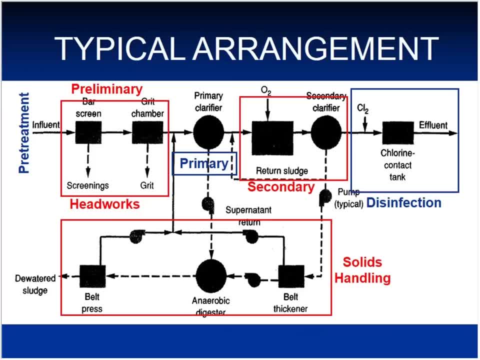 But it takes a lot of equipment and small plants don't necessarily want to invest that much money in equipment that they don't run continuously. Larger plants will do that. Everybody's got to go to a point where they're going to thicken up their material and then 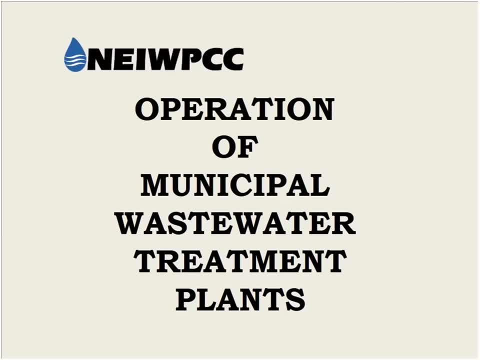 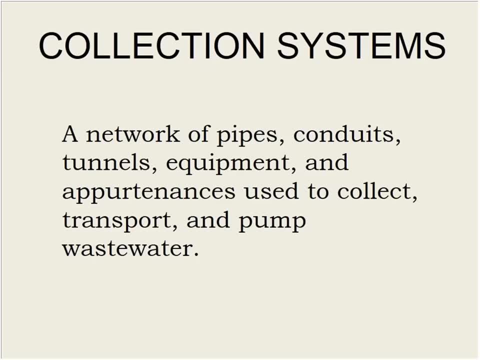 they may send it to a large plant to have them finish it off. I've never seen that before. All right, So we'll break down and get a little more detail on some of these things. Our collection systems, again, network of pipes, tunnels and conduits designed to take. 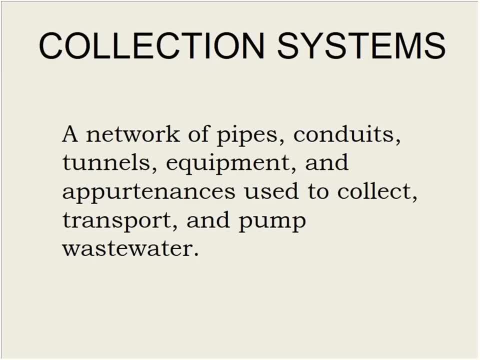 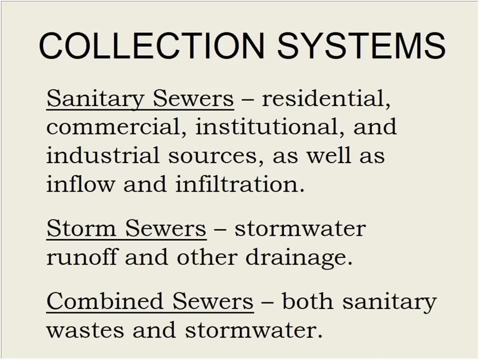 the wastewater from the source to the treatment plant. Sanitary sewers, residential, commercial, institutional, industrial and whatever squeaks in where it's not supposed to go. Storm sewers are just storm runoff Ideal That should be separated and go straight to the river. 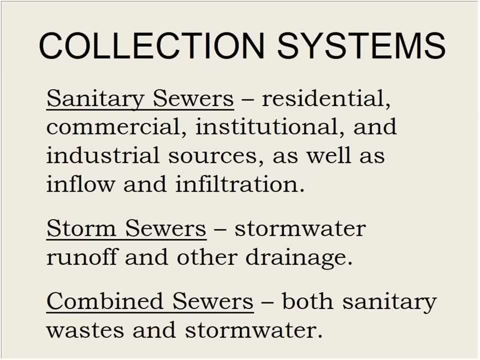 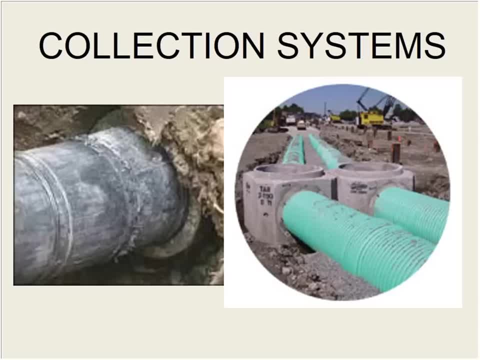 You'll find a lot of them have been labeled: Don't dump this, that or the other thing down there, because it's going straight to the river. But again, we still have a lot of combined sewers out there. Again, there's various types of piping going on out there. 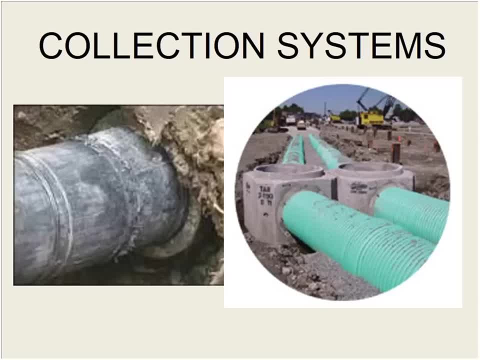 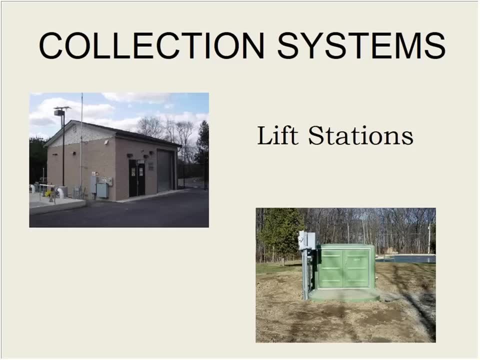 There's concrete, There's steel, There's plastic- All work done. You'll drive around. You'll notice little units like this from time to time. They're just little pump stations. What this is is: you've got a sewer system in some part of town, but then you've got 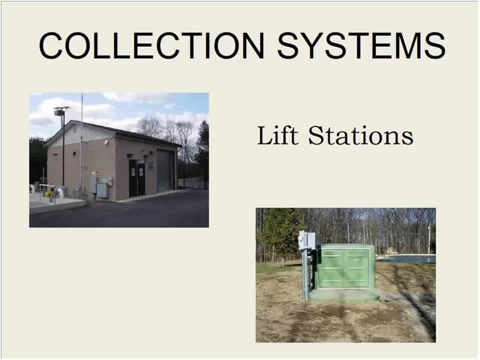 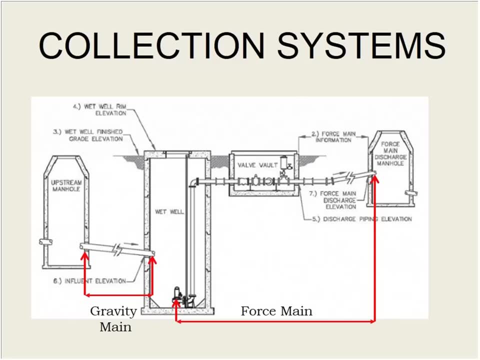 to get over the hill to get to the treatment plant, so you're going to have pumps in there. This is showing you some of the aspects of a collection system. By and large, engineers will do their best to have this water flow by gravity. 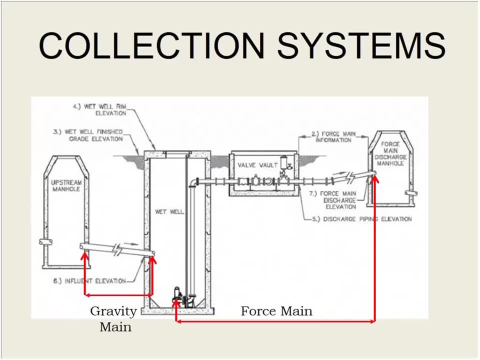 Let gravity do its job, Let it run downhill. That's what we call a gravity main. We've got a manhole and the piping between this manhole and the pump station or what have you just runs at a certain slope so that we maintain flow by gravity. 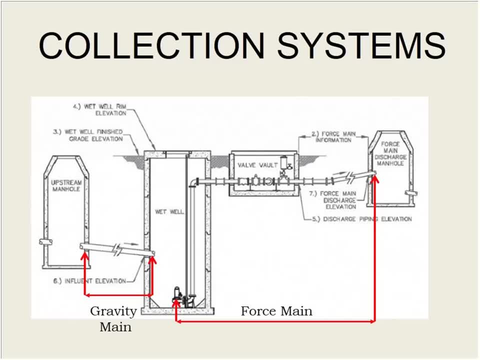 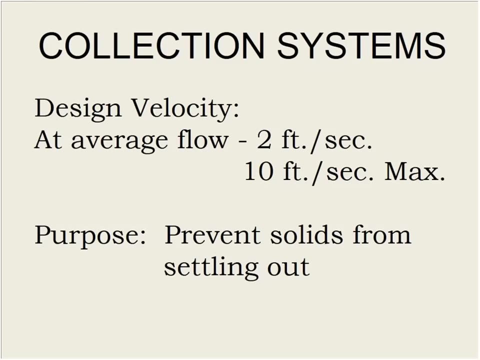 Once we get into that pump station, we have to go over that high point. Now we've got a pump. This system is under pressure. We call that a force main. There's parameters for these things. We design these collection systems to operate whether it's a force main or a gravity main. 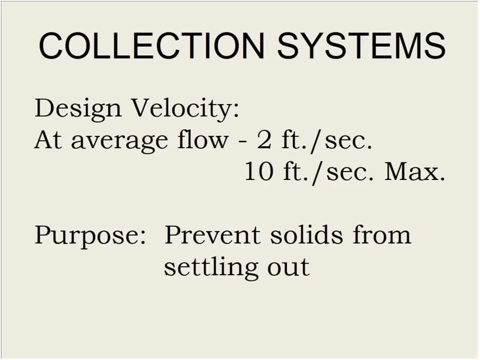 at a certain velocity, an average of two feet per second. We want that velocity because anything that gets into that system we want to make it to the treatment plant. So solids are in there and if our velocity is too slow they settle out in the pipes. 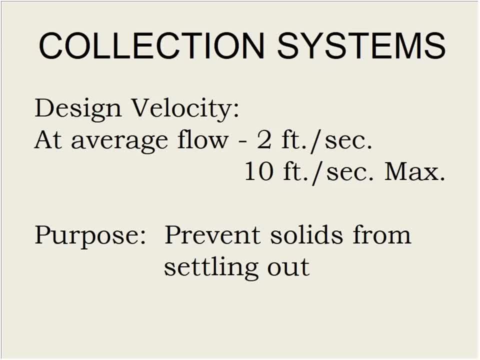 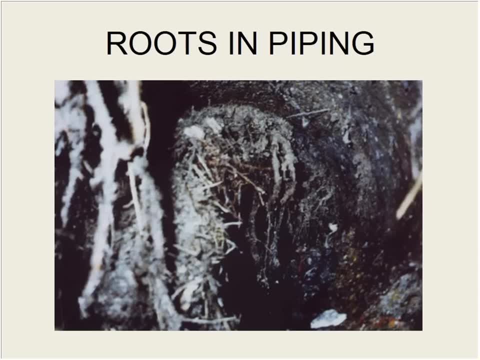 They clog things up. It's not good. So we want at least two feet per second to get that stuff going Again. CMOM in Massachusetts. We've got a pump station. CMOM in Massachusetts now has updated all of their regulations such that they have CMOM. 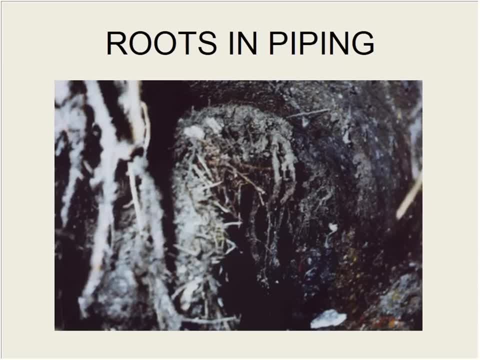 wording in there. The CMOM regulations started being developed back in the 1990s but never got approved by Congress, So they just kind of hung out there and they were kind of a gray area for a long time. Now EPA and the states have started to put them into actual NPDES permits requiring plants. 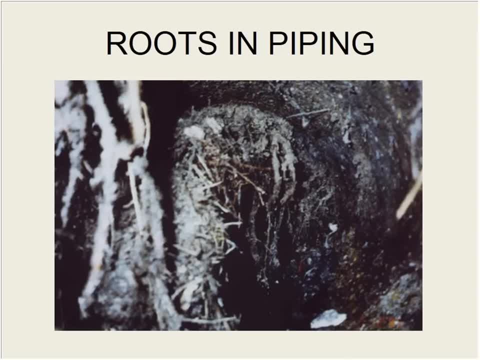 to do it. If you read the MAS regulations, there's about two and a half pages in there just dealing with the CMOM issue on mapping out your system, how often you're going to TV it, how often you clean it, jetting and all that sort of stuff to deal with situations like this roots. 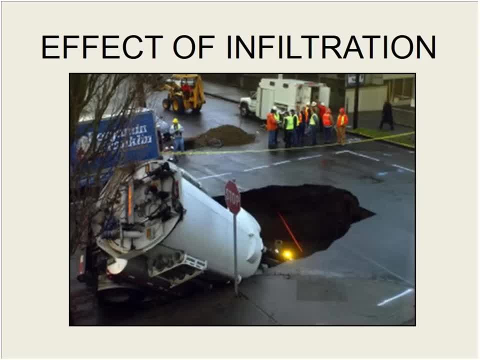 and stuff like that Infiltration. I just saw one recently. I just heard about Detroit and that whole neighborhood that was sinking in. Well, that is infiltration. You think of it? I've got a bed or a broken pipe, So every time it rains, water flows into that pipe and every time the water flows into 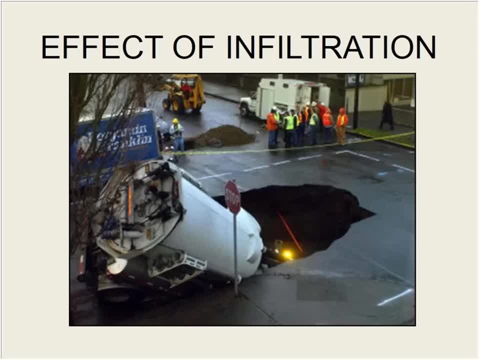 that pipe. it takes some of that soil with it too. At some point there's no soil left to support anything that comes down the street and Honda Civic drops through the street and goes away. It actually happened up in Nashville a couple of years ago. 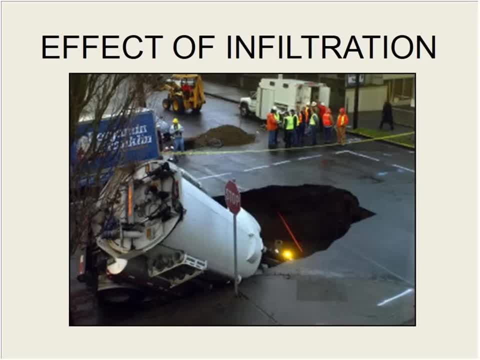 Fortunately it was early in the morning so there wasn't much traffic. It went down the street. The street opened up, Boom God just dropped into it. If you went by on Sunday afternoon you'd never know anything happened. They just filled it back in and paved over it. 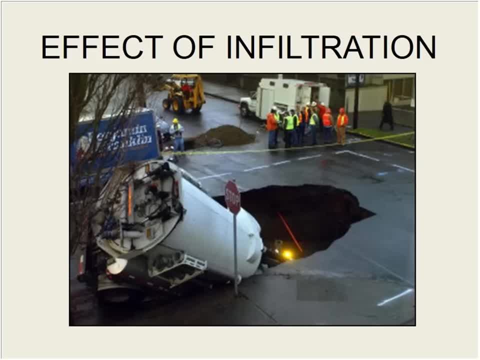 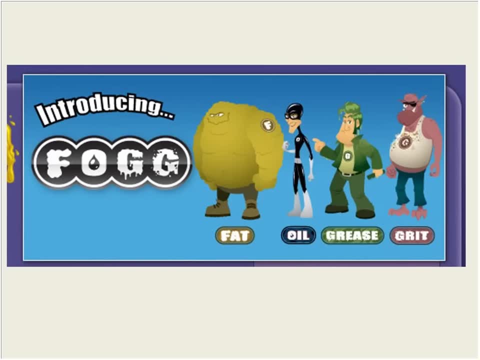 Never fixed the pipe. What do you think happened? two weeks later It opened up again. Lost another car. They said, hey, we've got a broken pipe, We've got to fix that thing. That soil is in green Big issue. 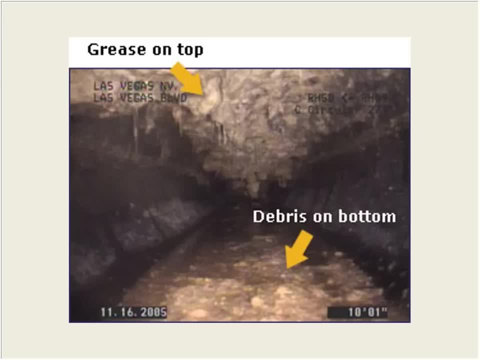 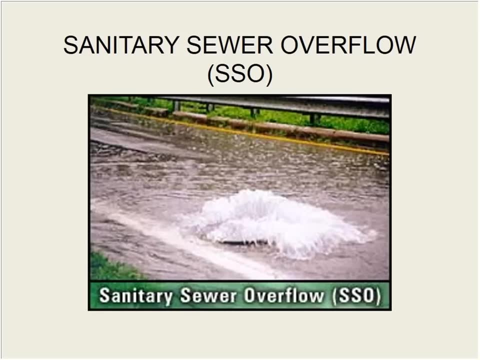 Again, it rides on the surface of the water. Every time water rises up and hits the coal pipe, it just sticks and slowly chokes up that pipe and we end up with this situation. This also not ends up in the street, but also may end up in people's basements and all. 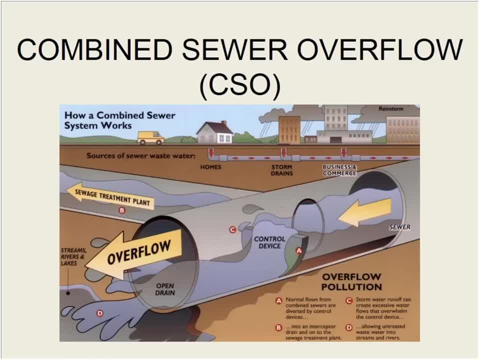 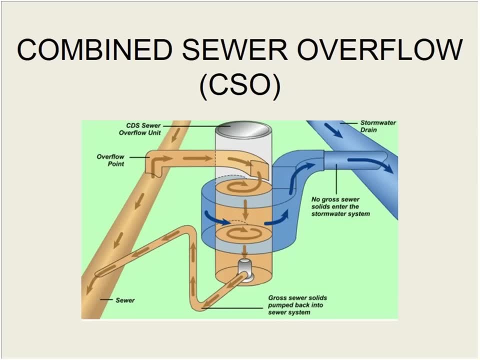 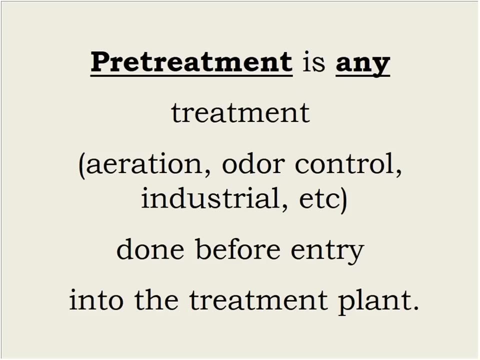 that stuff Very expensive, fix for it. We talked about people that combine sewer overflow operation. This is showing you one that's set up with a cyclone system so that it takes out the grit. It may also get disinfected before it actually discharges down into the system. 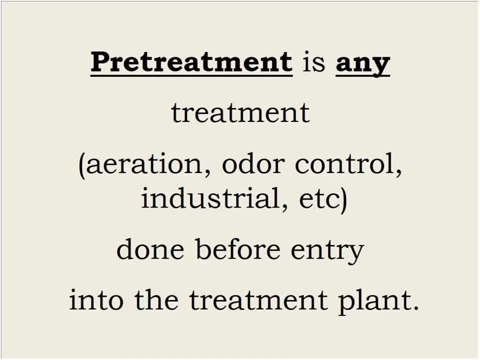 Here's the term: pre-treatment. Pre-treatment is a process. Pre-treatment is any treatment that's done to wastewater outside the confines of the POTW. If the city is dosing lift stations with sodium hypochlorite or potassium permanganate to keep 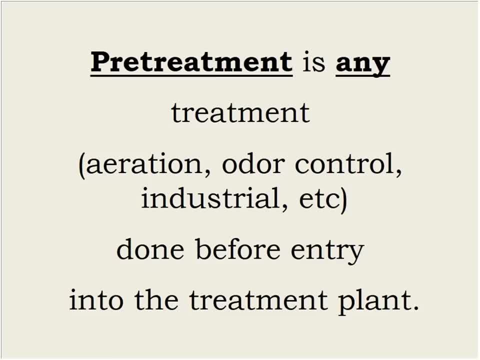 odors down. that's technically pre-treatment. They do that because you go into. as towns expand, they put in 150 houses and there's a pump station. Everybody goes to work. All that stuff just sits there all day. The thing of it is, from the moment you flush, the bugs are at work. 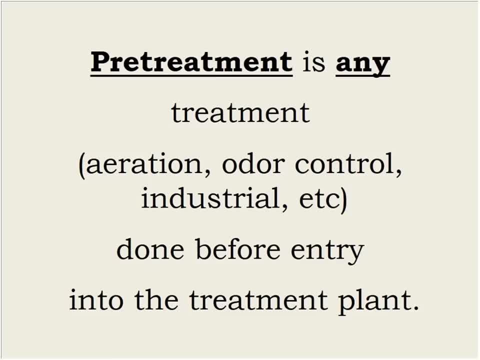 They've got food, They've got the bugs. You help put them there, They do their thing. The oxygen system slowly depletes and you start to go anaerobic and those lift stations just sit there all day because nobody around is flushing anymore. 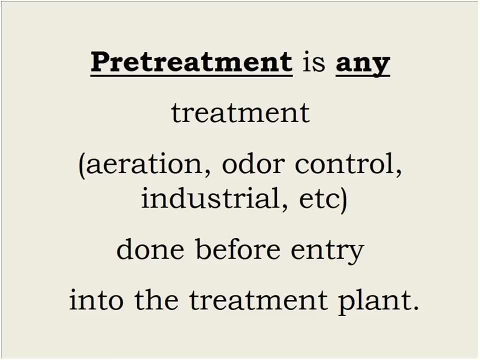 They get kind of smelly. so they've got to dose them back. Technically, at least in Massachusetts it should be done by a certified operator. Industry has to pre-treatment, It has to pre-treatment, It has to pre-treatment. 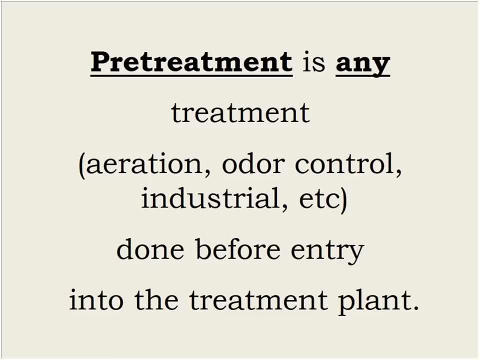 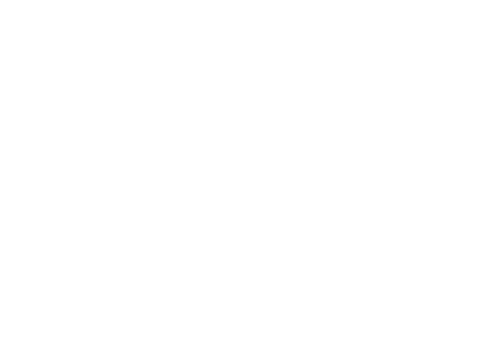 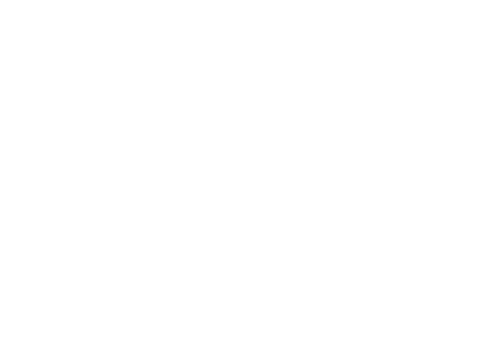 There are chemicals, There are metals that are not beneficial to the operation of bacterial treatment, and those have to be kept out of the system. So that comes under the category of pre-treatment. The towns, and we'll talk about the whole system. a municipality has a pre-treatment. 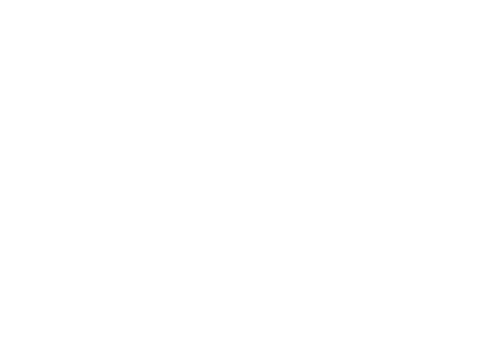 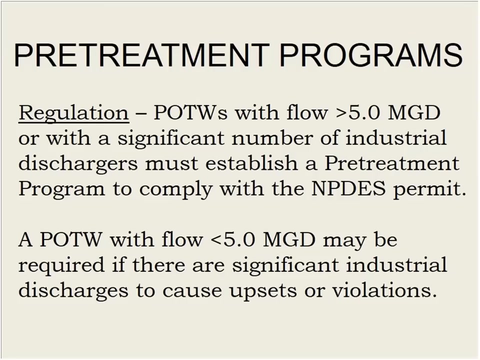 program where they actually oversee industries, write them permits and monitor them to make sure that they're not sending stuff to the plant that will be detrimental to their operation. That's pre-treatment. Any facilities- this is part of the NPDES permit- any POTW with a design flow of five. 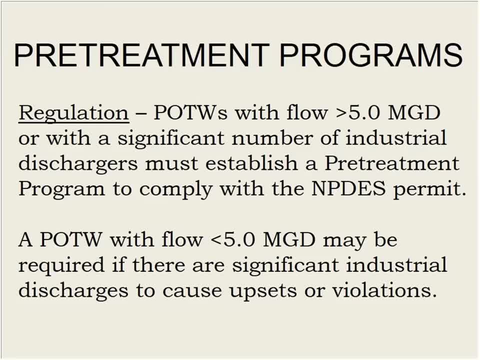 million gallons a day or better, has to have a pre-treatment program in progress. They have to have one. If you're less than five, they may make you have one. if you have a significant industrial user in town, that could really blow out your plant. 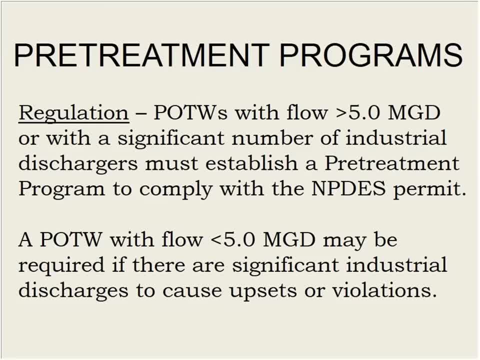 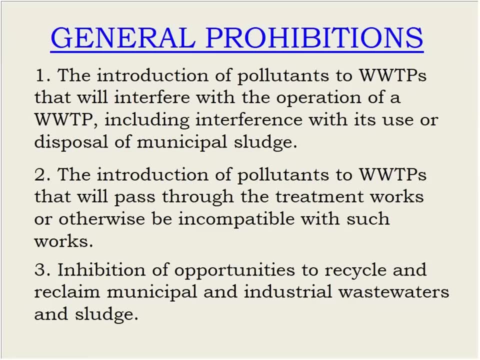 I've got a two million gallon plant, but I'm getting 150,000 gallons a day from XYZ Chemical Company. I have to make sure that I'm watching them on a regular basis to make sure they don't do something. Okay, Again, Clean Water Act of 72 initially targeted municipal operations. 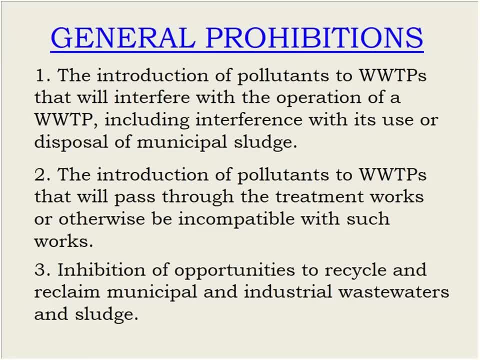 Amendments to the Federal Water Pollution Control Act in 1977 started addressing industries. We spend a lot of money making these plants nice, make them operate well. industry's still messing things up, so we've got to take care of that. They started addressing them in 77 and again in the 80s. 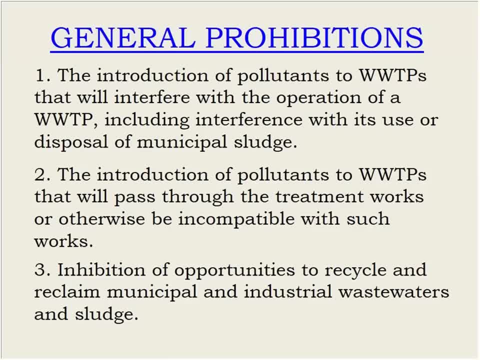 They came up with what they called general prohibitions. These are things that industry cannot send to a POTW. Again, it's a general prohibition: the introduction of pollutants to a treatment plant that will interfere with the operation of the treatment plant, including interference with its use. 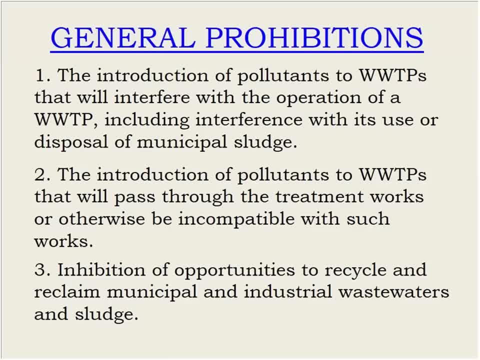 or the disposal of municipal sludge. They can't send anything in there that will be bad for the organisms. mess up the way they work, or mess up the way you get rid of your sludge When you boil it all down. what happens in these plants? 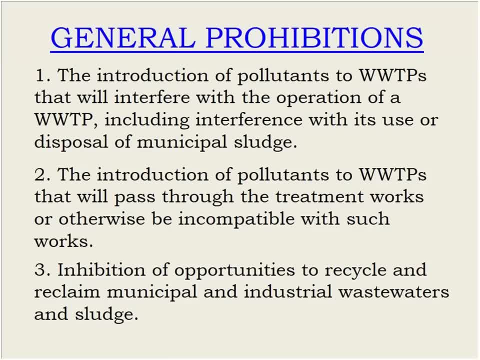 We're taking the pollutants, We're taking organic matter that we refer to as BOD and we're going to turn it into bugs. Now we have to get rid of all those bugs. We have to get rid of these things somehow. I'll give you a situation that happened up in Plymouth, New Hampshire, in 2003.. 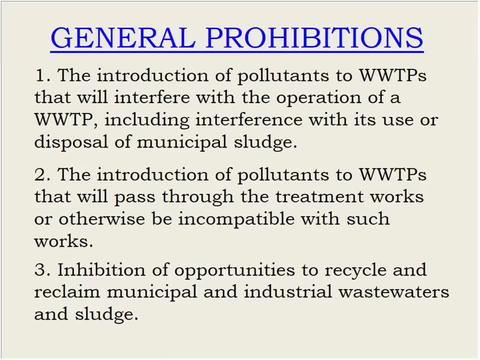 Dry cleaning operation lost some of its dry cleaning fluid to the sewer. It blew out its plant. It killed the bugs. He had no treatment plant. So right there he's in trouble because if you cause the treatment plant to go in violation, 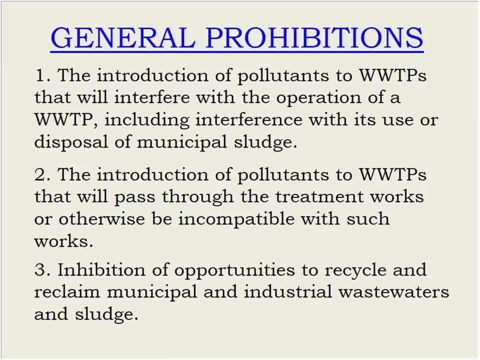 you're responsible for it from an industrial standpoint. The other problem was by New Hampshire's hazardous waste mixture rule, all of the sludge that was in their system at the time, whatever thousands of pounds that may be, was now hazardous waste because it had that dry cleaning fluid in there. 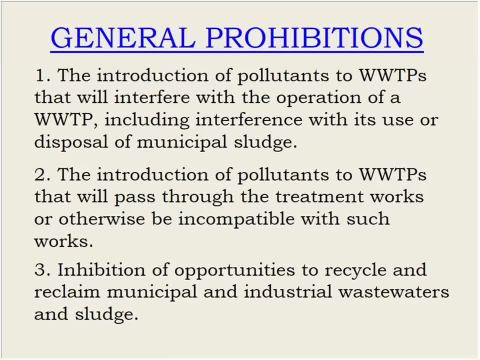 It used to be an expensive problem at that point You can't do that Introduction of pollutants that will pass through, basically big long-chain organic molecules. We've got eight to 12 hours in a treatment plant. It's like you're sitting down with a three-foot subway. 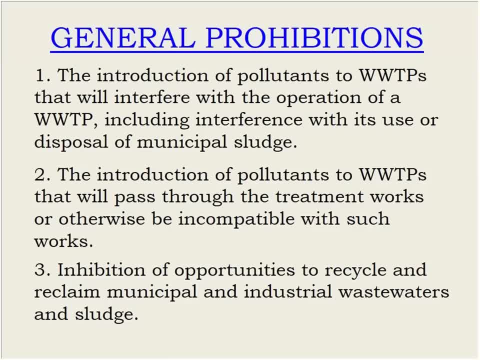 You're not going to get that done in lunchtime, but you're going to do it in a while. They can't treat it all in eight to 12 hours, so it just passes through untreated ends up in the river. That's a no-no as far as industry is concerned, and this one basically rehashes the first. 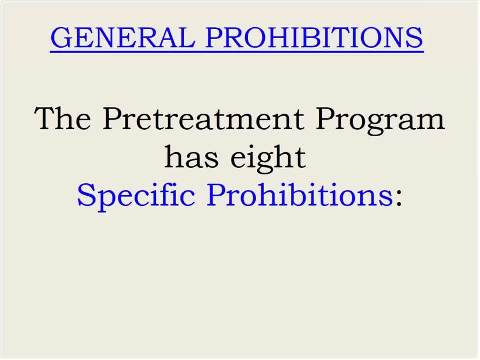 one. They're recycling the water or the sludge. Well, general prohibitions. any lawyer could dance around a general prohibition. I could probably do it if I wanted to. so I said, okay, we'll be more specific. These are things that cannot go to a treatment plant. 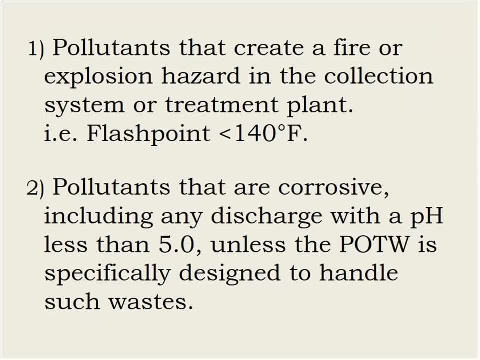 Pollutants that create a fire or explosion hazard. anything with an open-cup flash point less than 140 degrees Fahrenheit. solvents, fuels, that sort of stuff, stuff that go boom, Anything that's corrosive, including a discharge with a pH drop. 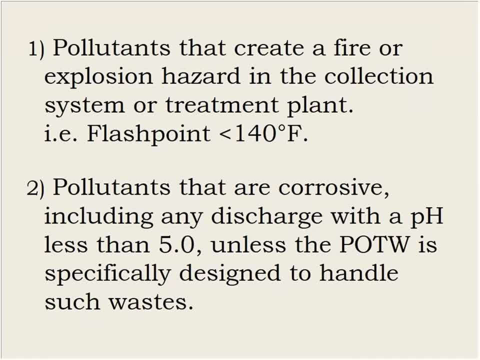 That's EPA rules. Massachusetts set the limit at 5.5, and no upper limit. This is Louisville, Kentucky. I left Kentucky in August of 1980, so I just missed it. You can see some holes in the street. 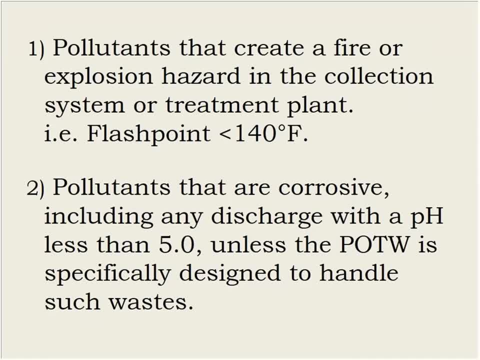 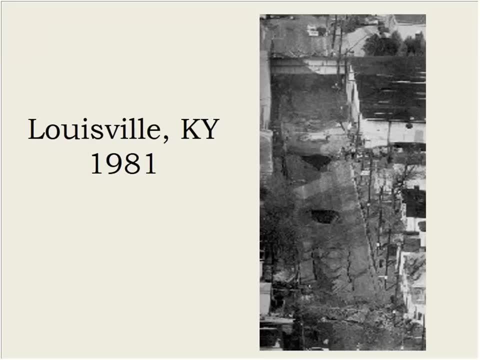 There's a Rawson Purina has a plant in Louisville, Kentucky, making some sort of chow, horse chow, dog chow, cow chow, I don't know, and it's part of the law. It's the law. 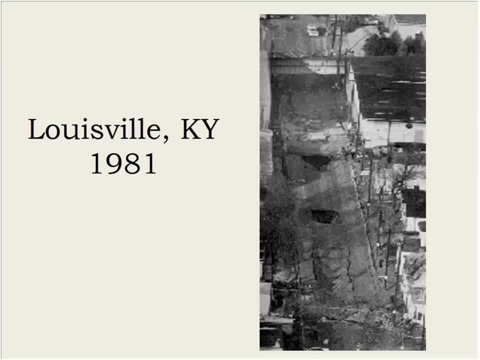 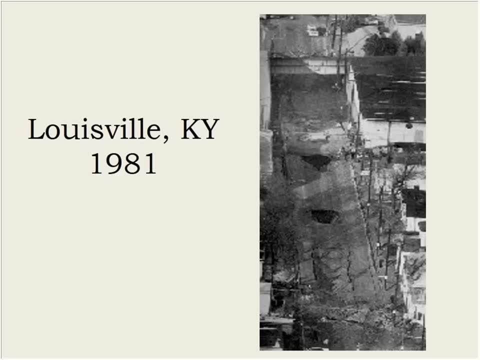 It's the law. It's the law. As part of the process, they extract a lot of soybeans. To extract a lot of soy beans, they used hexane, which is an extremely volatile solvent. Well, they lost a few a pixane to the sewer. 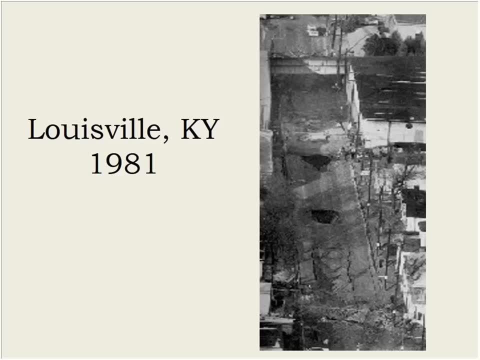 Being lighter than water, it floats on the surface. there's enough oxygen around And it's a true story. Two ladies on their way to breakfast that morning drove over a manhole. Something on their car provided the ignition source and manholes for two miles went boom. 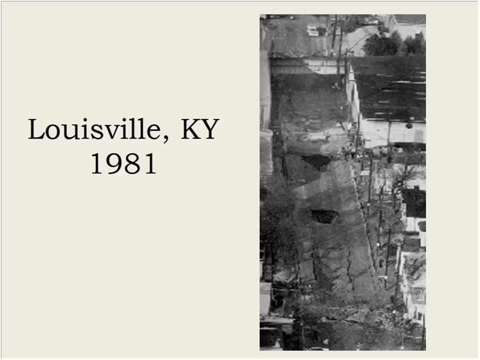 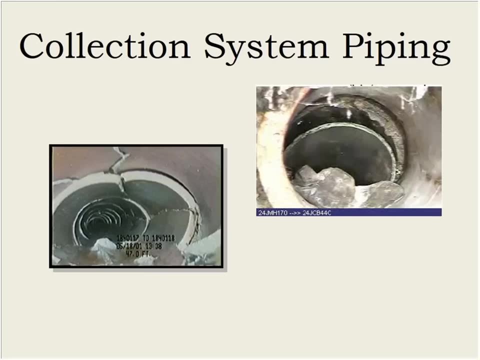 boom, boom. It was cool. There was a traffic helicopter in the sky at the time watching the street flow up. Can't do that. Not a good thing. Low pH: Largely to protect the collection system, in addition to protecting the organism. 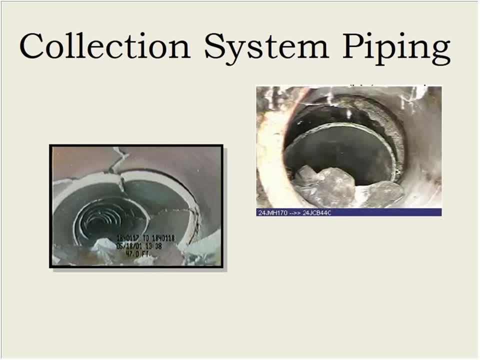 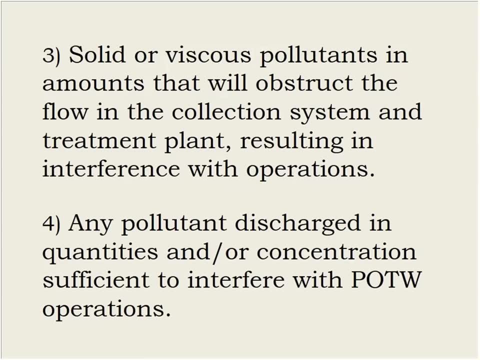 OPHs. The pipes rot out, Boom. Next thing you know it's another truck falling through the street. Solids or viscous pollutants: The amount that obstructs flow in the collection system or the treatment plant. Nothing that can plug up the piping. 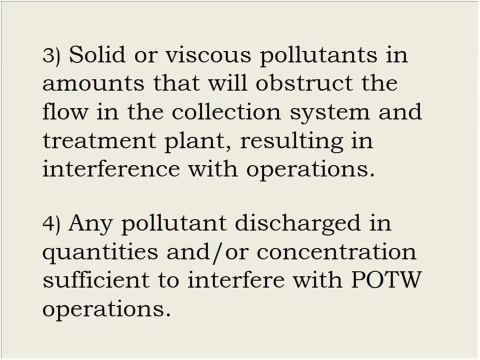 I go to the extreme saying: take our friends out in Deerfield at the Yankee Candle They got a batch of candle wax they don't like. They can't just send that to the sewer. Any pollutant discharge in quantities, concentrations that will interfere. 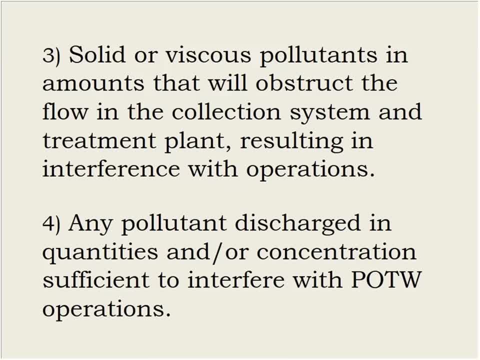 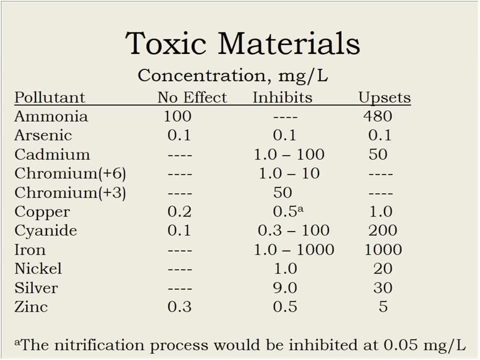 Again, metals: certain organics can't be discharged with that down there It interferes with the process. Metals primarily are the biggest problems. Atmium: You start to inhibit the process. at one pot per million You're into a total upset of 50.. 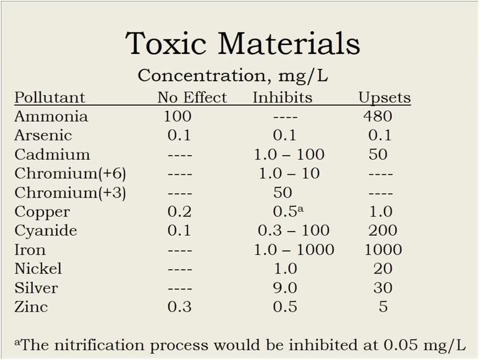 Nickel- Nickel is pretty low too. Zinc: Half a pot per million Doesn't take a lot to really mess up the bugs. They don't like that stuff, So that is. prohibited Discharges with temperatures above 104 degrees Fahrenheit. 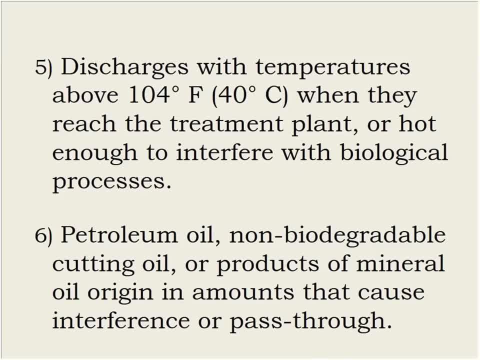 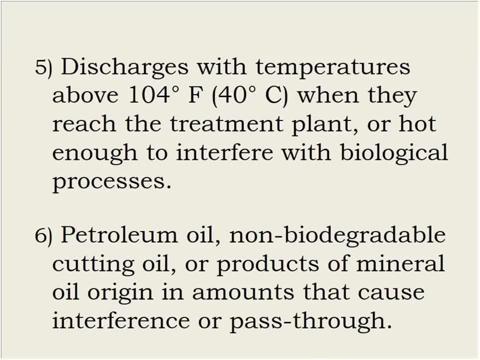 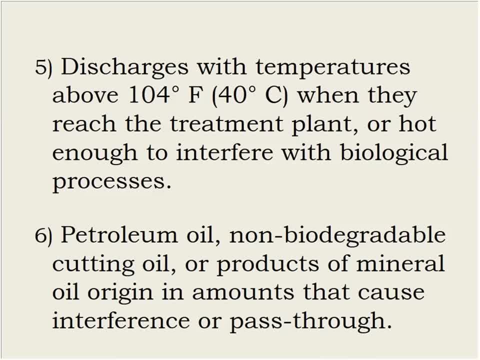 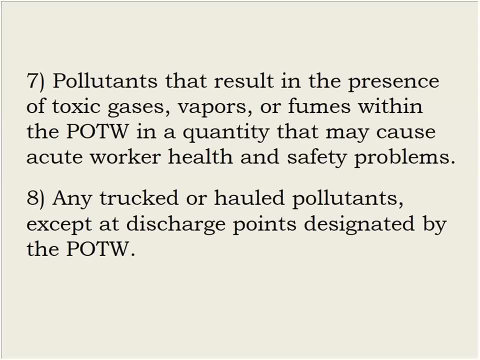 The ones that are low pH And the ones that will just pass through. Petroleum oil, Non-biodegradable cotton oil, Big organic molecules Just pass on through Anything that causes a safety issue for the operators of the collection system, And this one's for the midnight hauler. 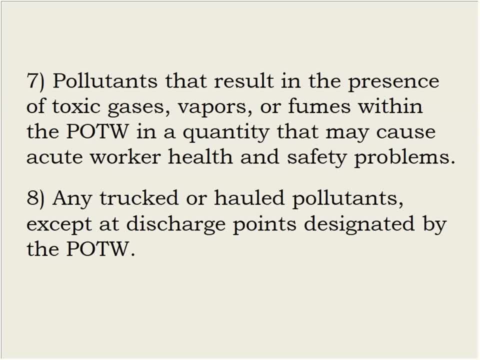 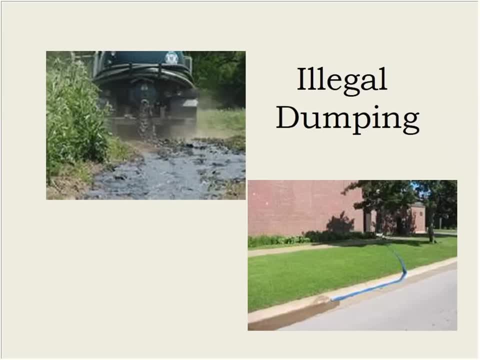 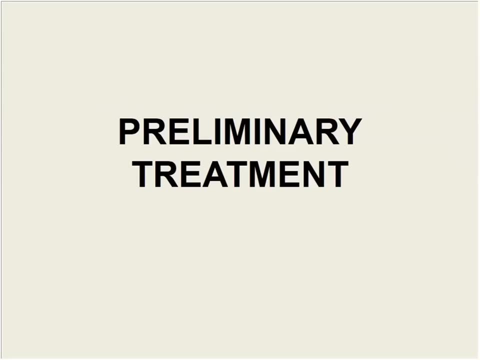 Truck to haul pollutants, except at discharge points designated by the POTW. That's not designated by the POTW. Unless you're in Jersey, You can always go to the POTW All the way through. So I think it's good, Good times for us. 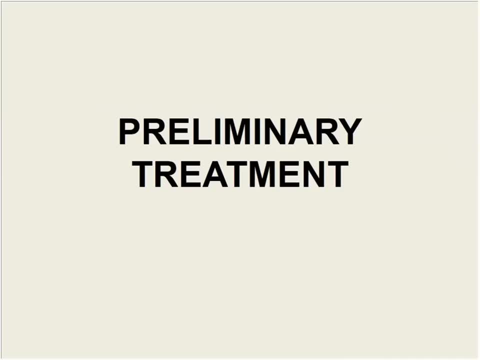 How are we doing Any questions there? Yeah, so just a friendly reminder, folks, you can use the chat function in the sidebar. I don't have any questions yet, But feel free any time to shoot me a question. and when Jim takes a break like he has never. 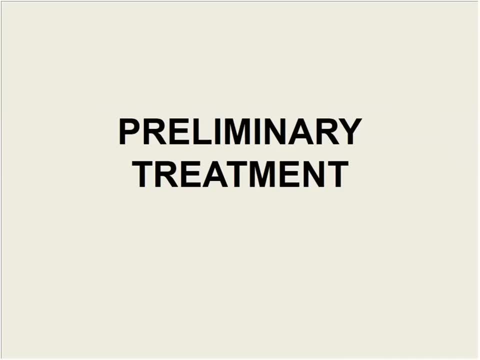 done, we can fill those questions. So again, you just want to hover your mouse at the top in the green bar, Click exit full screen And you can use that chat function to ask questions. I don't know if you want to take a quick break now or keep going. 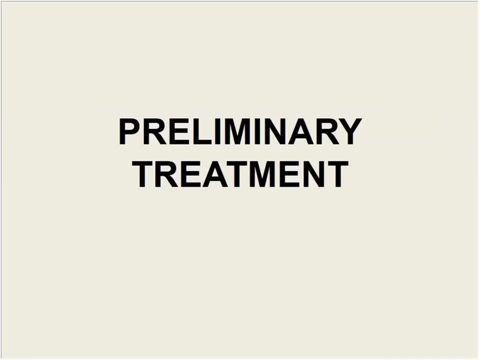 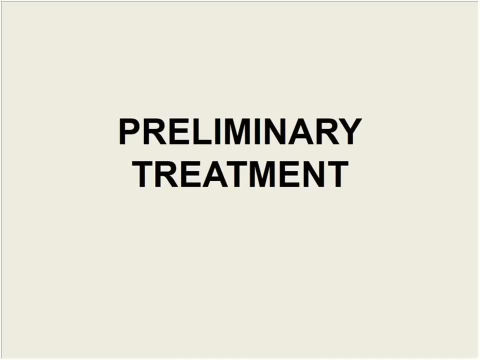 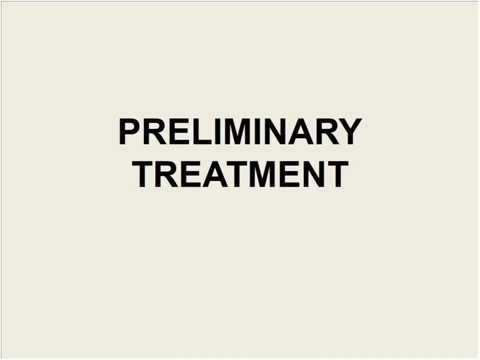 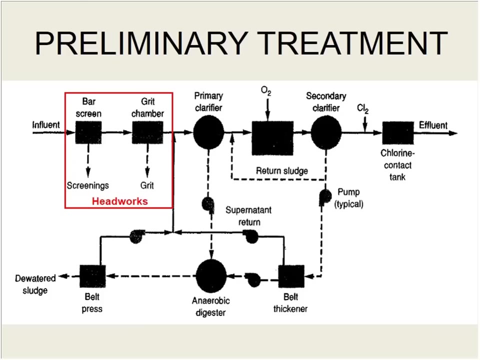 So we're going to talk about retreatment. that's outside the POTW. Now we're inside the plan. the first step that we have is what we call preliminary treatment. That's where we are on our flow chart, Right, Bart. 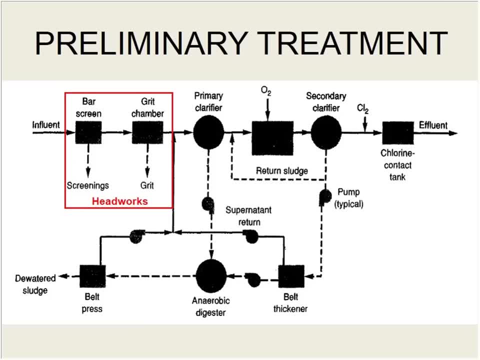 This is the section of the plan we refer to as the head works Right Again. if you think about it, this wastewater has traveled some distance, been on the sides of your town Again. Deer Island's traveled 35 miles from Framingham just to get to Boston. others are 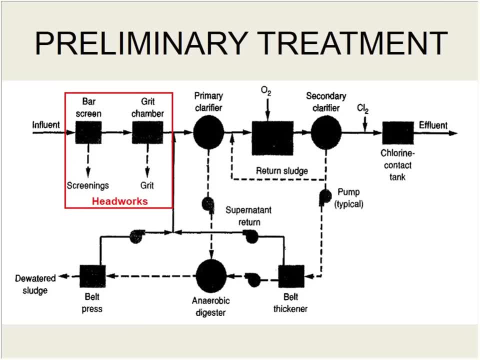 smaller but, depending on pumping cycles and stuff, this is the first time this water sees the light of day. It's been confined to the collection system. all this time The bugs have been doing their thing. The oxygen levels are at varying degrees of functionality. 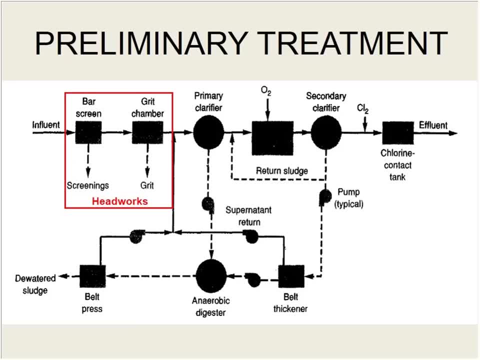 You may have none, at which point the stuff that comes into the plant will smell pretty badly, tend to be pretty dark in color because it's non-septic. Other stuff should be especially gray to light brown and shouldn't be all that obnoxious. 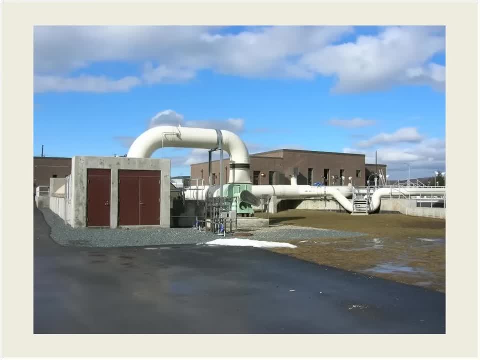 First time it comes up today. This picture is showing you FedWorks building off of there, on the right at Upper Blackstone Water Pollution Abatement District. This is the first time it's coming up today. This is a regional facility here in Massachusetts, just outside of Worcester. 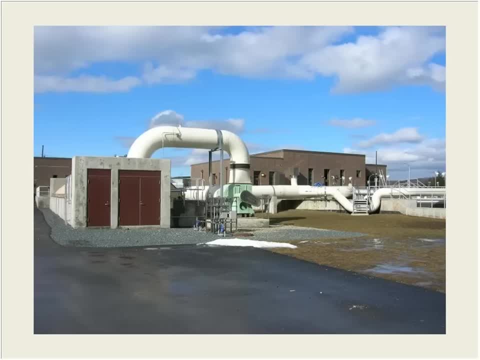 It's a 100-million-gallon plant. It actually has two FedWorks buildings. The one you see on the right is the one that operates all the time, then the older one that's barely visible on the left is there for high-flow conditions. 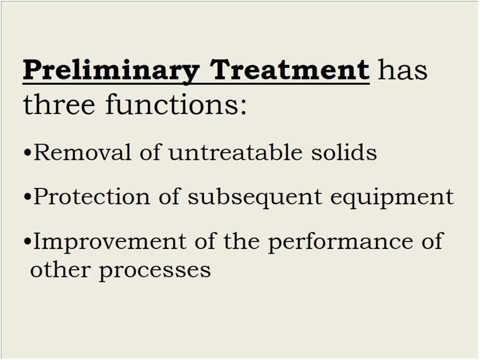 So preliminary treatment is there to remove untreatable solids. We're essentially running a biological process. We've taken out things. There are still some things. Bugs can't eat them. When I'm talking about bugs, I'm talking about single-cell bacteria. 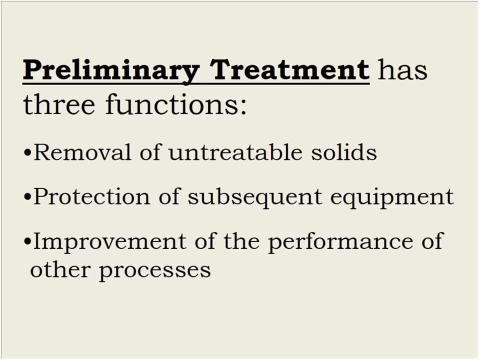 They can't eat golf balls, they can't eat 2x4s, tin cans, cup caps, whatever. and if you talk to anybody that works in the collection system, if it'll fit through a man hole, it'll show up someday. 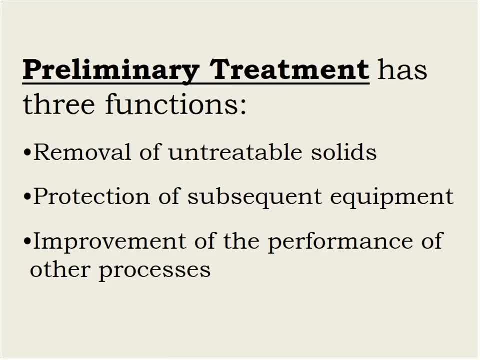 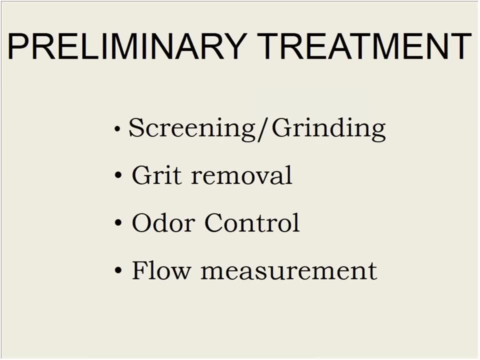 Washing machine cups. We also want to protect equipment. If stuff goes in it could ruin pumps, clog up piping. We don't want that to occur And as a result, it improves the operation. various methods that we deal with screening or grinding. we have brick removal, the separate. 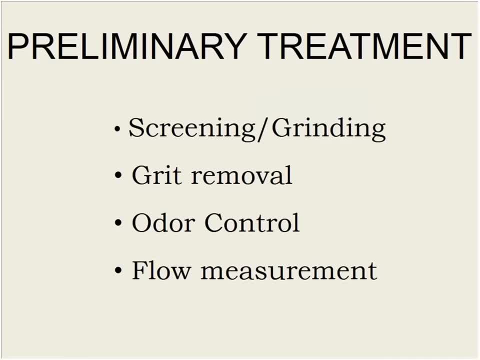 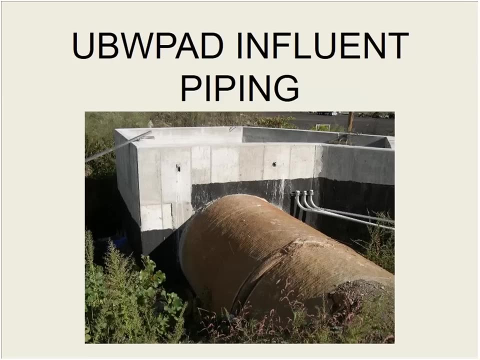 item all together. it's also again because this is the first time this stuff comes to the light of day. we're going to have some motor control, because it can be quite nasty, and we're also getting to our flow measurement. we need to know what's going on well again. ideally, things are. 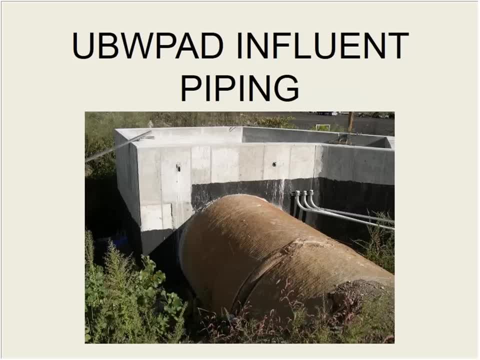 going to flow by gravity but depending on the geography of your location, that may not always be possible. this is the influence line to upper Blackstone, 72 inch line coming in. they're very fortunate. all their water just flows by gravity, doesn't have to be pumped, but it will keep on. 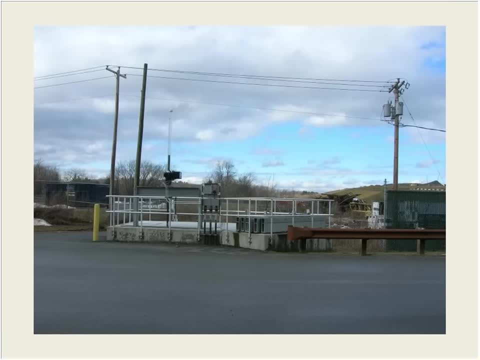 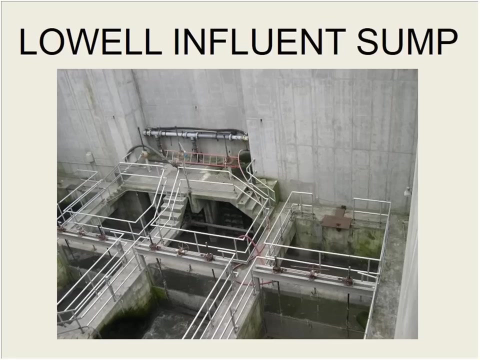 running downhill. this is the vault once it was all closed up. we have a vault here that allows it to go to either of the two headworks buildings, depending on flow rate, and it's enclosed for odor control bowl. on the other hand, their wastewater comes in about 30 feet below break. this needs to be brought up to ground level in order to start. 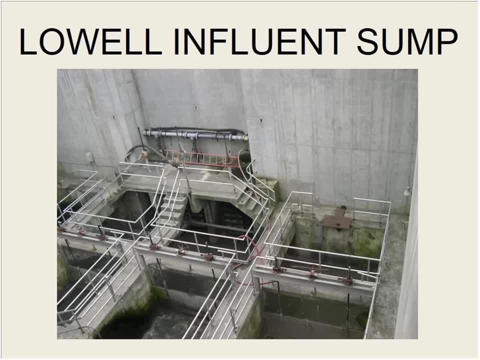 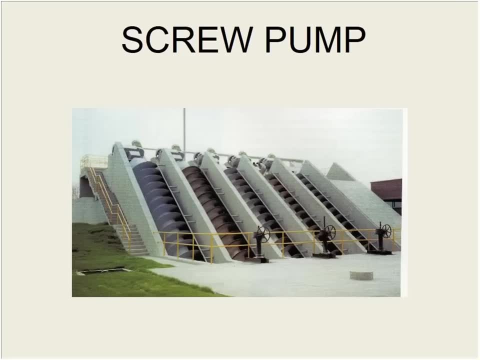 working with it. it's totally open and if you drive by there on the right day you're going to get quite a smooth flow. so these are just set up that way and this is a typical method of raising that incoming wastewater. in a facility such as that is with this screw pump. screw pump can deal with anything. 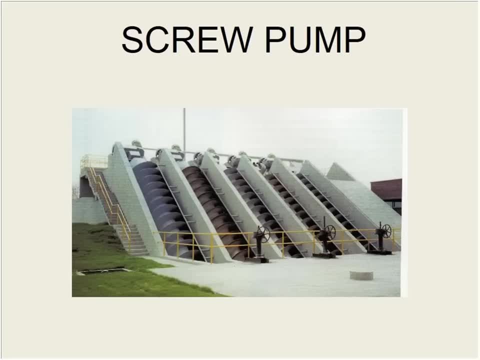 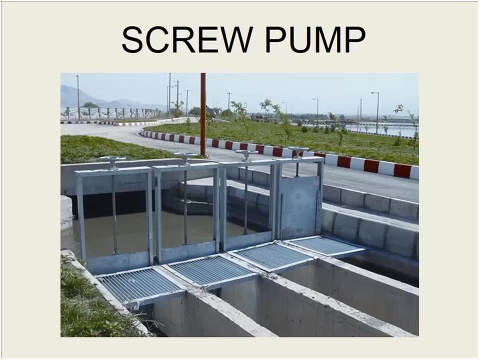 that comes in with the influence. it'll just drag it right on up the hill because it's just a powerful machine, it doesn't clog and it'll actually chew up some of the stuff. as it goes, these situations, they are generally closed for both safety and odor control. this one is open for some other reason. 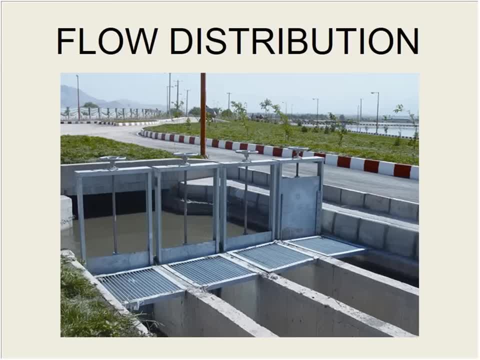 so we talked about velocities through a collection system being generally at two feet per second. we're still at that level as we come into the plant. now, the plant will have multiple units for treating, and the reason for multiple units is you want everything to run within certain 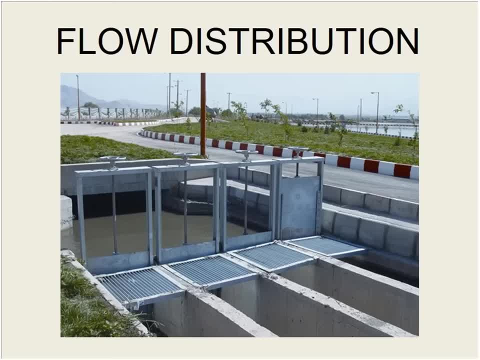 parameters. so I may need a lot of units online during a high rain event and I may need very few during August, when I haven't seen rain in six weeks. so we have to have some method of controlling our flow distribution through the plant. we run in those ideal ranges all the time. this particular one's just using slide gates to allow. 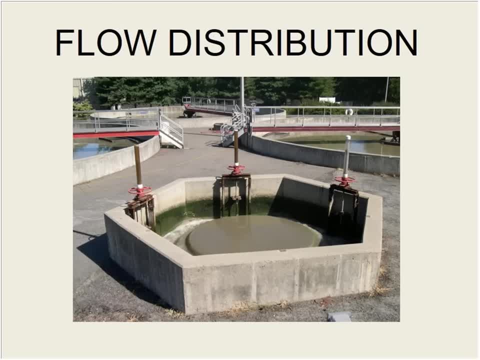 water to go to any number of channels. this is in Billerica. their incoming flow comes in through this. they call it a blossom close up from this pipe, and then they've got three different valves, depending on how many clarifies they're going to operate again. this is just to keep things within. 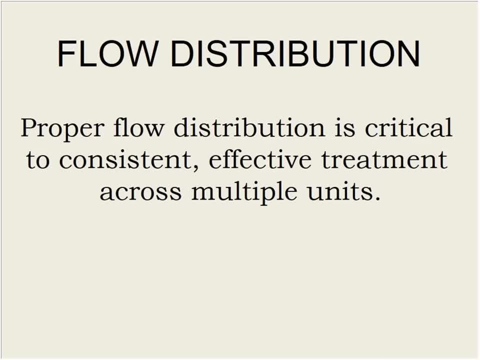 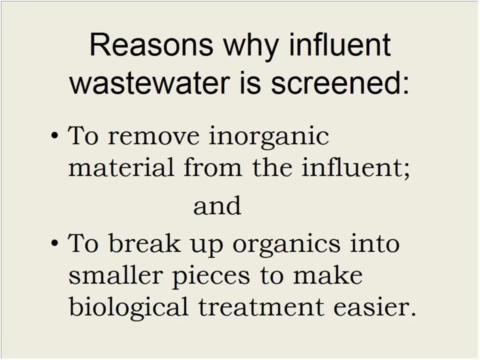 our prescribed operating ranges. so talk about screening. screening is the most common method of dealing with incoming material and we're going to remove inorganics and large stuff that will jam up pumps and stuff. we don't want things that are going to settle out in our 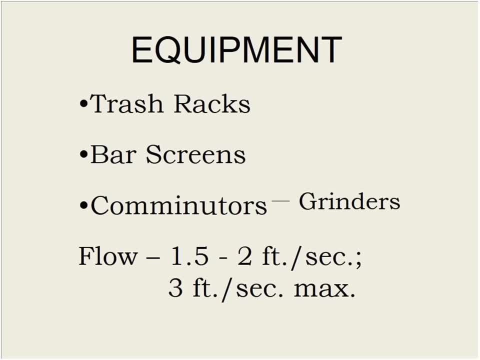 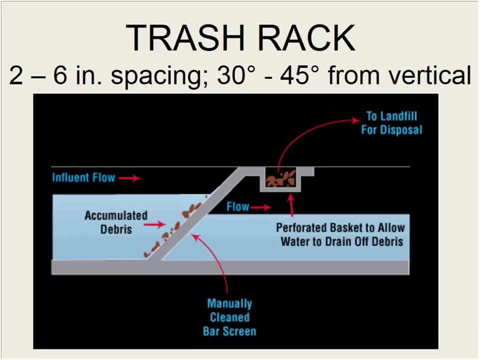 treatment plate tanks and such. so we have trash racks, we have bar screens, we have grinders also. we'll talk about those together. we're still running at essentially that same velocity. we still don't want anything settling out. this is a trash rack. these are so tough and these you may find in Lagoon systems or very small. 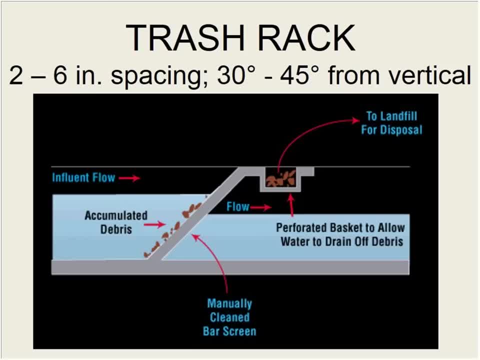 operations, but the principle is kind of the same. we've got a series of bars that set at an angle to the wastewater coming in and their space- the trash rack- is very crude- two to six inches. so some big stuff will still flow through here, but anything that doesn't fit between those bars gets. 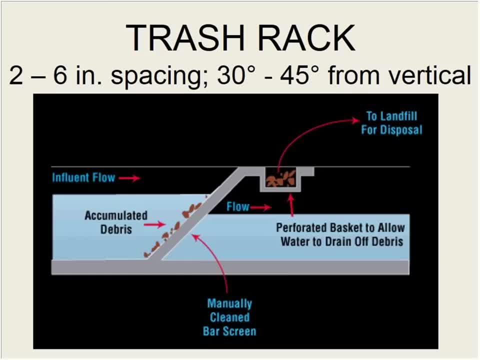 caught on the bars and for the trash racks, the manual operations. somebody has to go out and actually remove that stuff physically with a rake or some mechanism. the unfortunate thing is these things tend to be outside quite often and they're going to plug. usually during the rain event, we flush everything out of the sewer and that's not a great place to 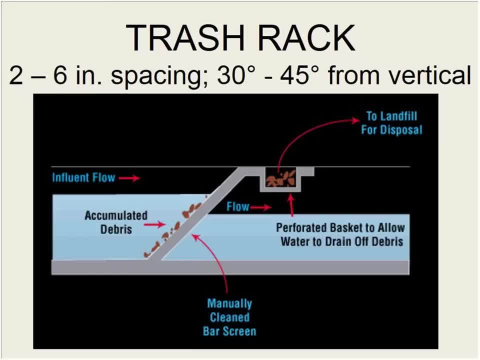 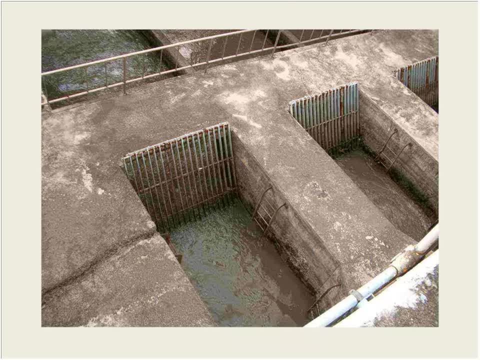 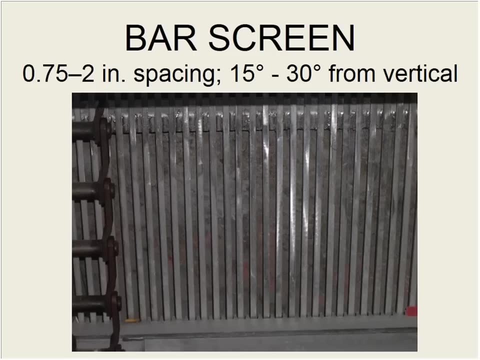 be during the rain event. so there's a picture of a trash rack- very crude screening operation. there we go now. bar screen, which is a little more common in most plants, is much finer: a quarter inch to about three quarters of an inch, so it's fairly tight. these are pretty hefty steel bars they have. 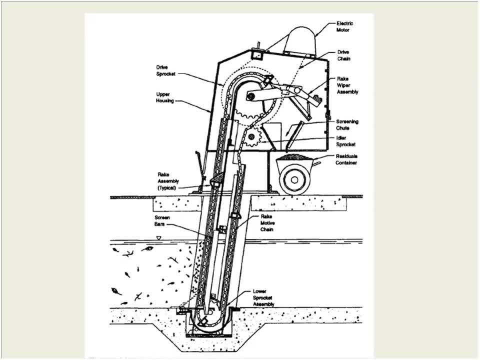 to take the resistance of flow that comes through the plant instead of being mechanic, uh, manually cleaned by some poor guy going out there with a race. and again, these channels can be about 15 feet deep. they're automatically cleaned. got a cleaning mechanism. it's got a rake that'll just. 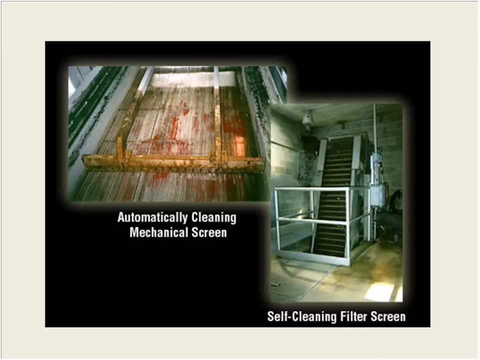 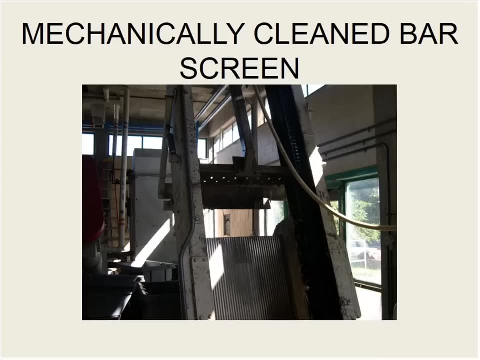 drag this material off and clean it up. you can see one of the rates there. there are different types up there. as it drags the material off the bars, you're going to have a big flat plate. we want the water to come off these things and drain back down into the channel. a couple of reasons for. 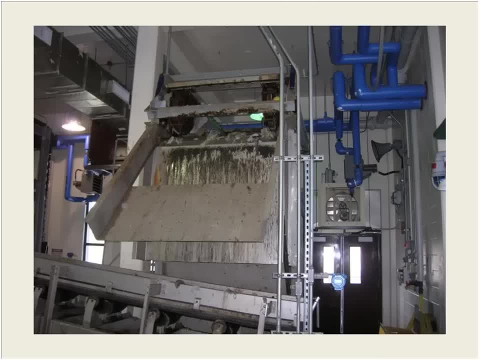 that okay, back into the discharge here. the material that comes off these is ultimately going to go to a landfill, easy to dispose of. but landfills are getting very particular and a lot of ways they don't want excess moisture. we have the drain plate to help keep the stuff in the system. they're 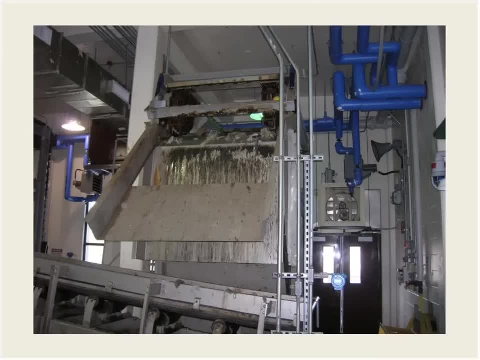 concerned about what we call vector attraction. vectors are nice new word for pests, rats and flies and Seagulls and that stuff, so they have vectors. they don't want to have that stuff because if we just send this stuff off loaded with organic waste, that's going to be bad. you're very good work. 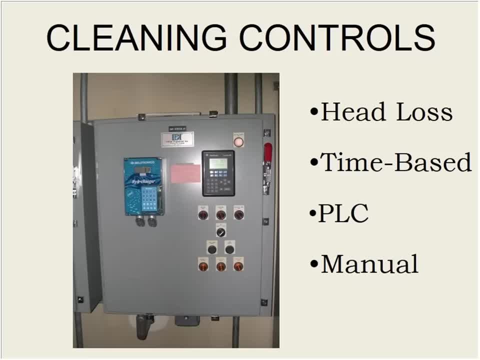 Now, as far as cleaning these things on the automatic systems, they generally work off what we call head loss. Head loss is the difference in water elevation upstream and downstream of the screen. As that stream clogs, water backs up upstream. It has to be able to get around the stuff that's clogging. 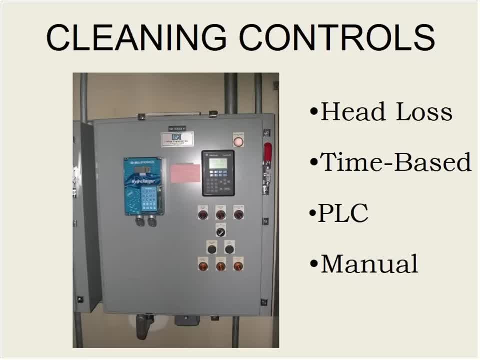 We want to keep that at a minimum. This is a control panel for Nashua. They have this blue device here. on the left part of the panel is a level device- ultrasonic level device that measures the height of the water. upstream of the screen. 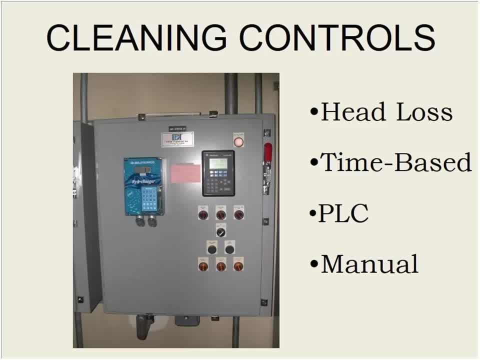 We've got a little PLC in here that's going to control the operation of the cleaning mechanism. It's set up generally as a time-based thing. It's going to run 15 minutes out of every hour. The PLC will control that It's 10 o'clock. 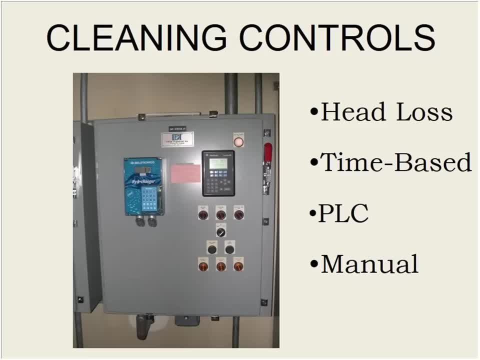 It will run the cleaning device for 15 minutes, then shuts down until 11.. That's all well and good, But now we get a rain, event comes in and we're starting to flush stuff out of the collection system, so the screen clogs up faster than it would normally do then. 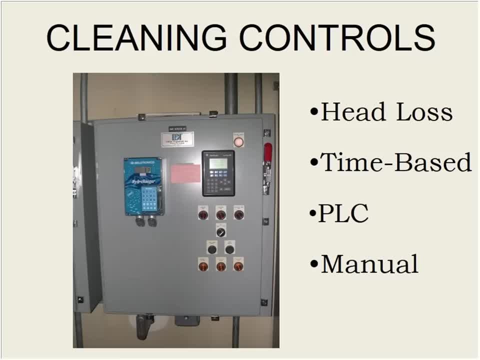 So that's where the ultrasonic level device comes in. It's set at a certain level that says, if it hits this, we don't care about the time anymore, It's time to clean the screen. So that works as a backup, so that we don't plug the whole thing up and have the water. 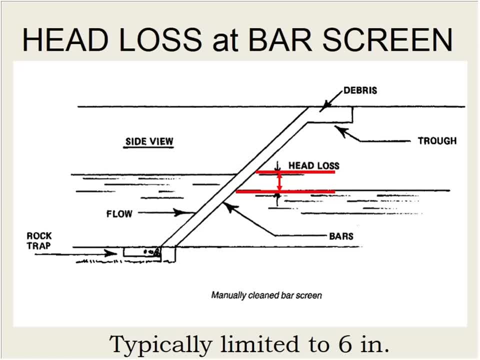 up on the floor. That's typically the way these things are set up. Again, that's that head loss that we looked at. We don't want it to be too big. Again, we want our velocity through the system to be fairly consistent. so, if I wait and 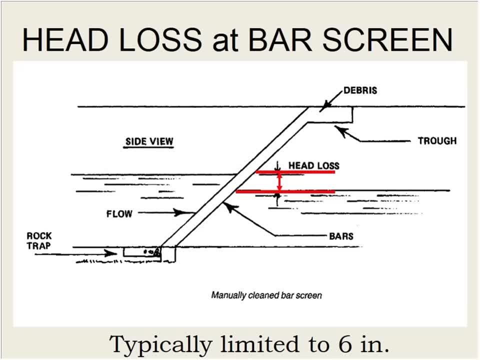 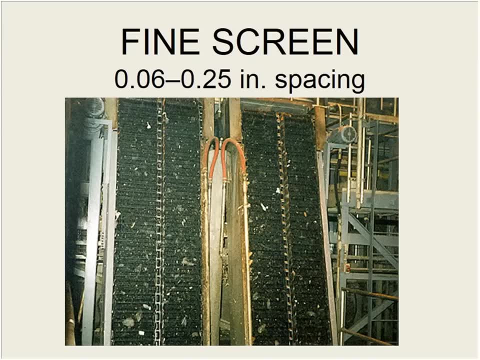 let it build up, build up, build up and then I clean it. I'm going to get this big flush of water running through there, and that's not what we want. There are some that are classified as fine screens: very, very tight spacing. 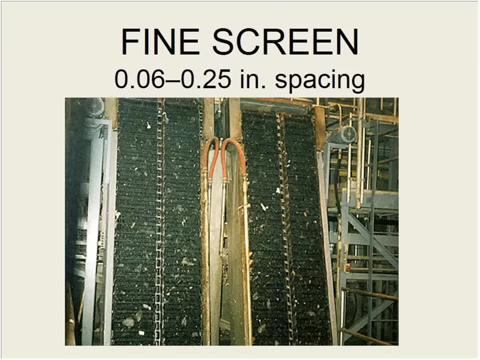 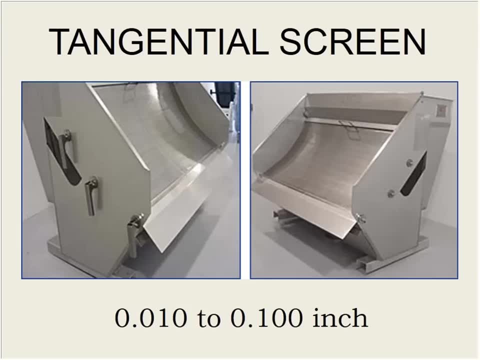 These can actually replace the subsequent process of primary treatment. You need a good, strong backwash to keep them clean, but it's starting to be more and more prevalent. Here's another method that can be run. This is a tangential screen or an arc screen. 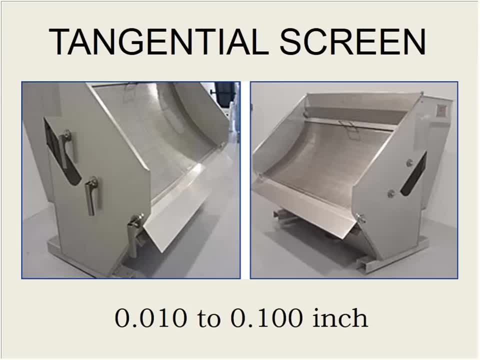 The water just comes up and flows over this, and what we have here is this isn't really a screen, but a series of triangular-shaped wedge wires, very closely spaced. As the water flows over it, those wires act like a blade and just shave off a little bit. 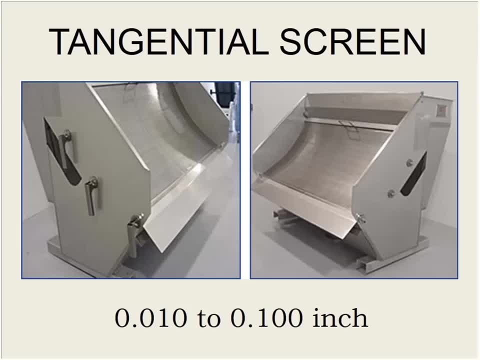 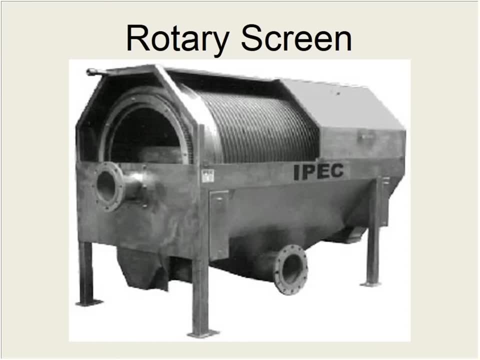 of water. The water passes through, the solids stay on top of this and eventually just discharge off the end. here Again, very tight screening, Something that's been really important. I'm going to go back to this. Okay, This is relatively new. 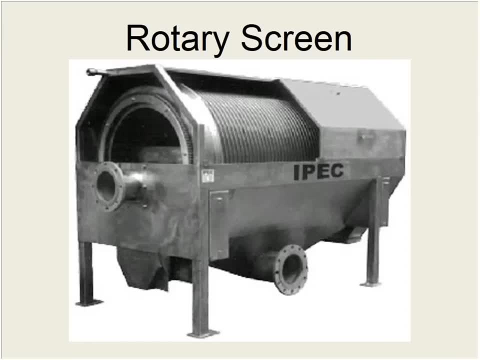 The past 10 years or so, we're starting to see an increase of these, our rotary screens. Your flow comes in. There's a manifold inside this screen. We've got a big rotating drum with a mesh screen on there and as the water overflows, 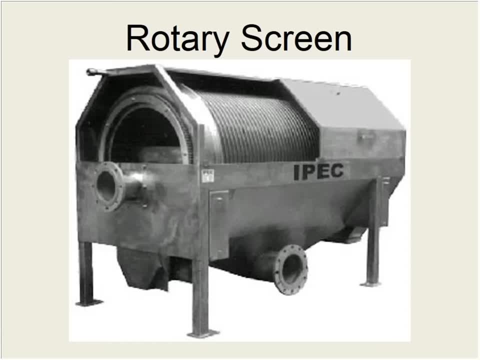 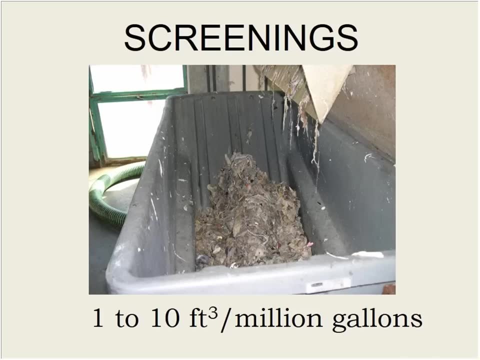 the water will pass through the screen, come out nice and clean and the solids stay inside and eventually get discharged off the end and our screenings. it varies considerably depending on what's going on. It's changed a lot. This is a picture. 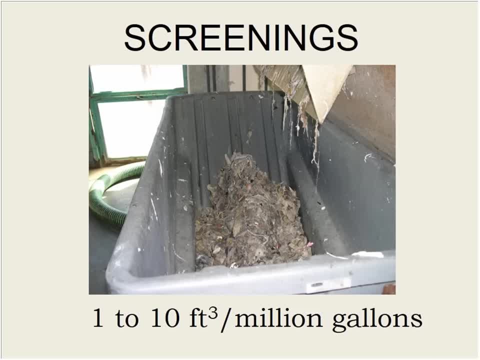 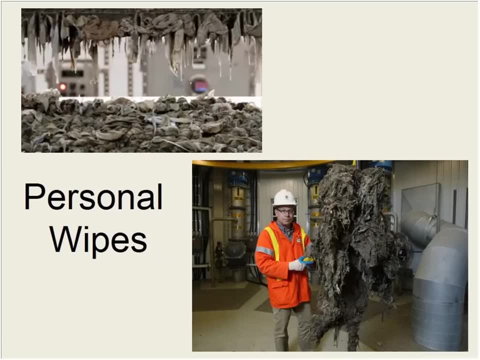 This is a picture from about 10 years ago. out in Billerica. We've got a lot of stringy, weird stuff that shows up, but today this is what we deal with. Oh God Again. I've been watching this over the past 12 years and it's amazing how it's changed. 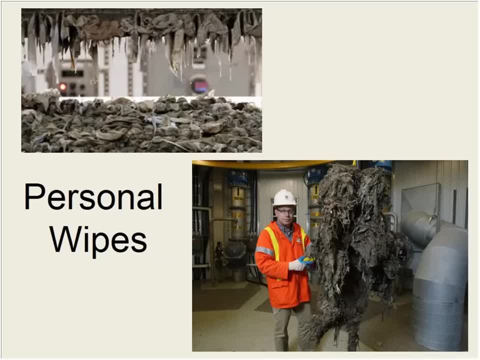 and this is just. we have these monster blobs in the collection system now from all these wipes. It's just huge, Absolutely huge. Stuff comes off by tons. Okay, Thank you, Thank you, Thank you. You're supposed to have a little diaper pail in your bathroom for those things. 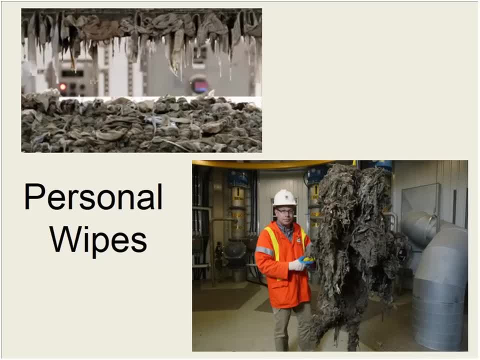 Are those the ones that are supposedly flushable? Yeah, They're flushable. Golf balls are flushable if you've got the right toilet. Flushable really doesn't mean a whole lot. Yeah, Those really should not be in the system. 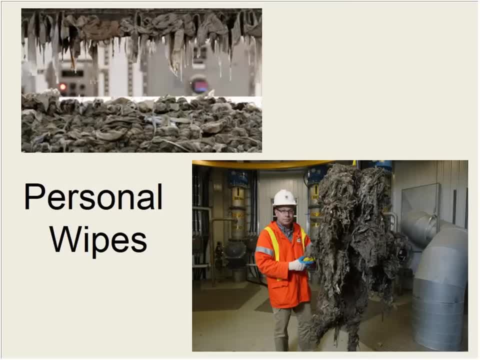 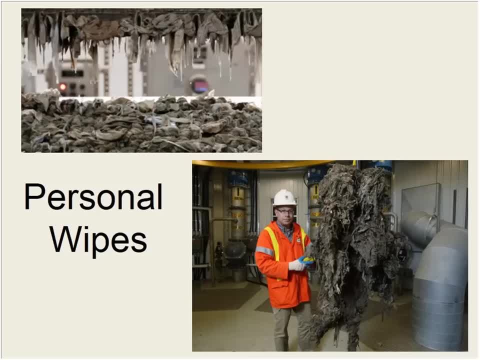 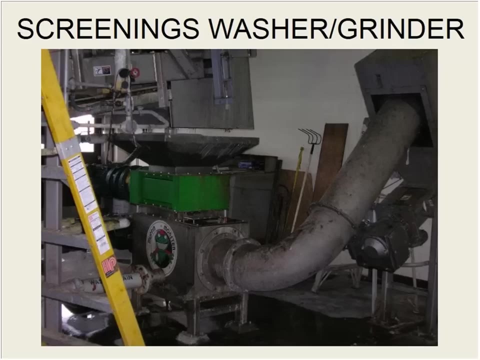 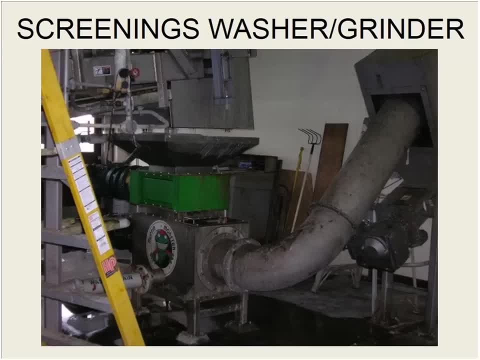 At upper Blackstone. the material comes off the screens. It's a belt conveyor to get into this unit here. This is called the muffin monster. It's a big grinder. This barber has a little tubing around the top- sprays water. help wash off any organics. 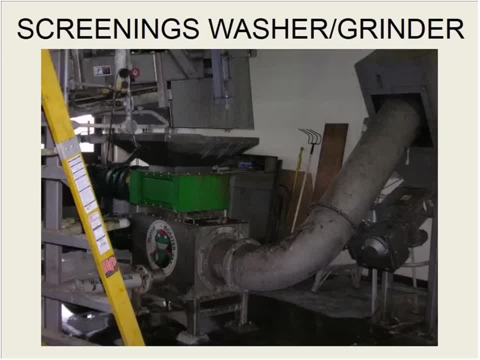 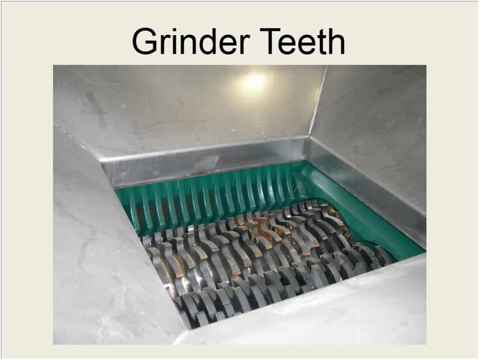 from the screen. This thing grinds everything up and then this is a pump that will squeeze this material and push it out to go into a roll-off bin. squeezes all the water out. The water goes back into the system and stays there, carrying the organics over with it. 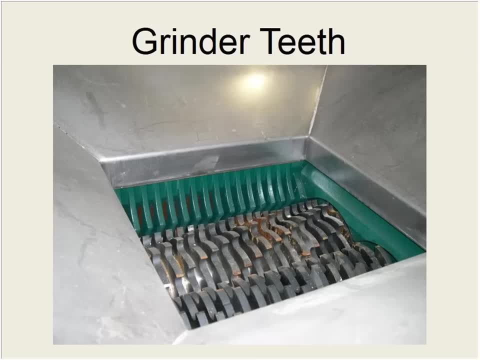 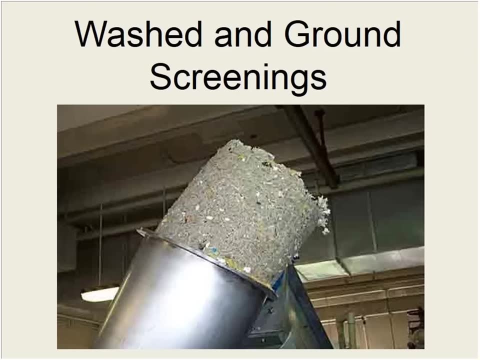 This will grind up pretty much anything. If you throw a hunk of asphalt in there, it will get chewed up. If somebody you're not fond of, this will take care of it, and this is what comes out at the far end. 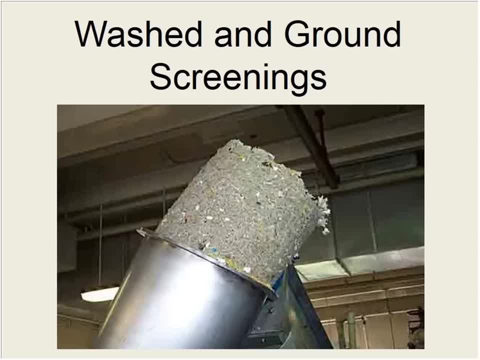 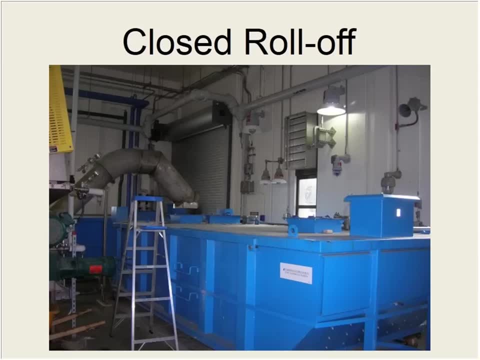 It's very water-consuming because it's really squeezed the water right out of, it goes off to the roll-off and not a big deal. What do they do with that? Do they burn that? What's that? Do they burn that? 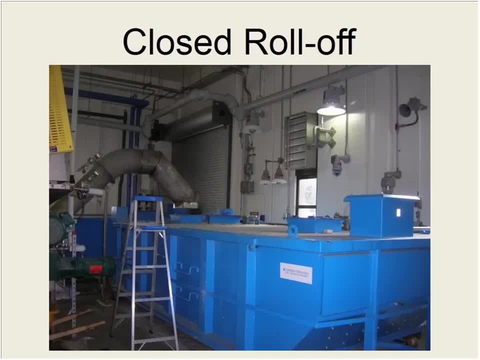 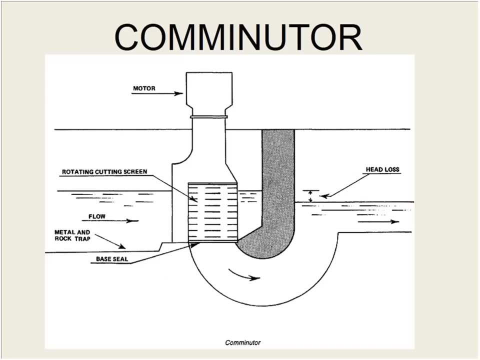 No, it goes to the landfill, It's buried And it's a nice covered roll-off. Even that's part of the odor control. Now, grinders are basically the same thing that you might have in your sink. You've got an incinerator or disposal unit in there. it's the same stuff. 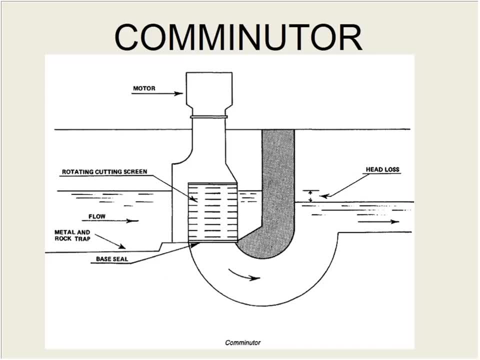 Same kind of a principle. Water's going to flow through. here. There's a series of bars with certain spacing. Anything that passes through the bars is fine, but if it doesn't, it's going to get chewed up by the grinder. 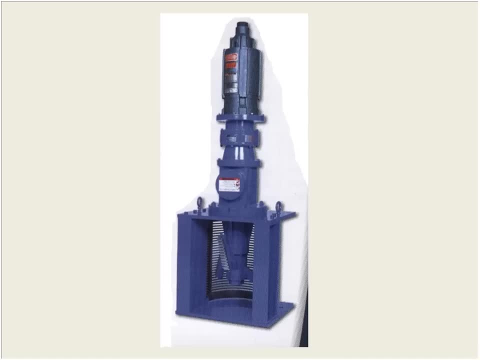 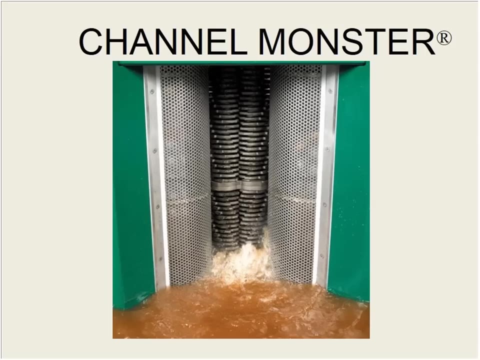 It just keeps going and chews it up until it passes on through. In other words, it's just like that other unit we saw. You can throw pretty much anything in there and grind it up. So the difference between this and screening is screening actually removes this material. 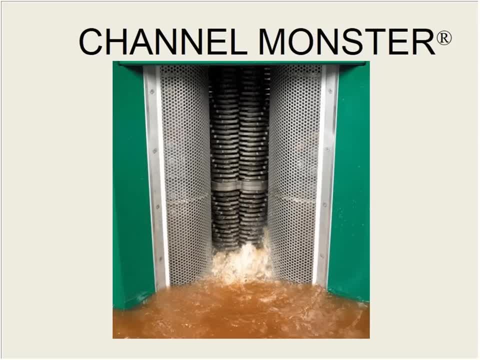 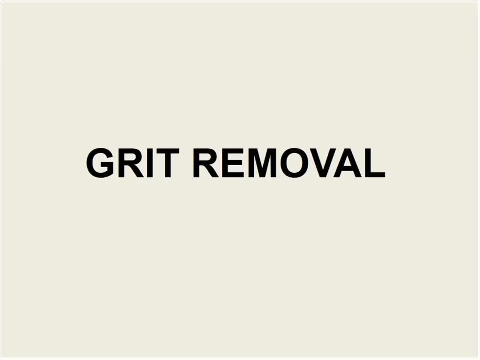 and you can send it out to a landfill. This doesn't remove anything, It just chews it up and you have to deal with it later on. Now, grit, sand, coffee grounds, cinders, whatever type of material that's the inorganic. 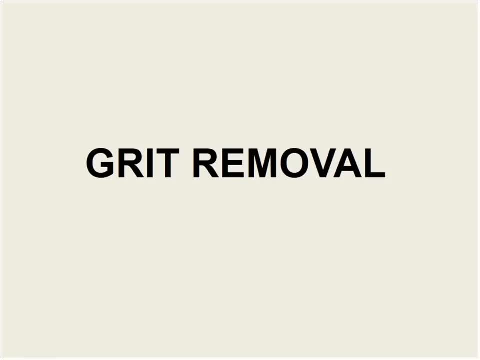 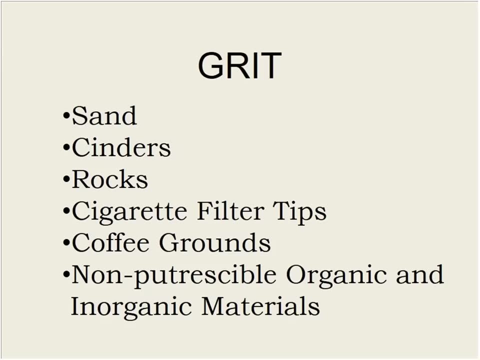 type of material. We'll pass through all of these screens and grinders, but we need to remove it because, again, the bugs can't eat this stuff. So that's the next step in our preliminary treatment: All of this material needs to be removed. 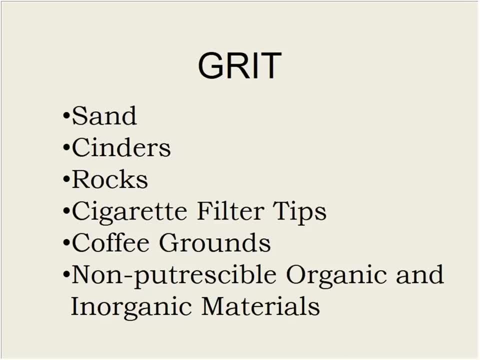 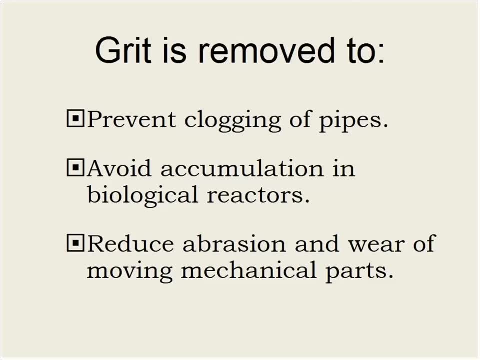 It needs to come out Non-putrescible material. So again, this stuff is particularly nasty because it tends to be very abrasive. It will eat up pump impellers and pipe elbows and valves and all that stuff clogged pipes. 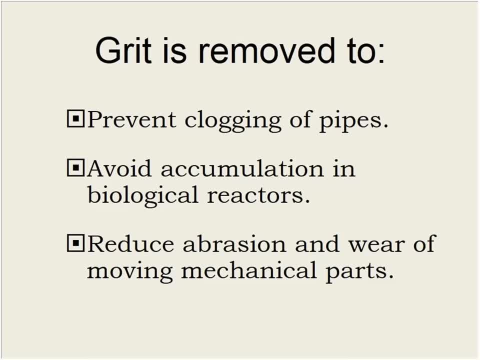 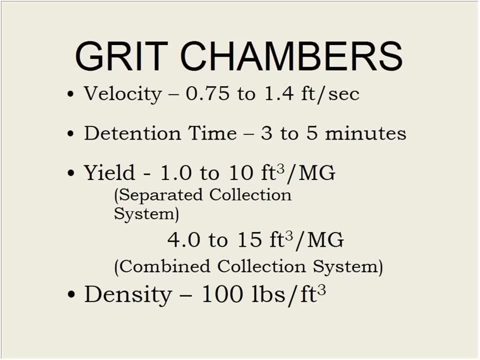 that will settle out in tanks and take up space that we don't want. So we want this out of there. So now again we're in control. So we're actually going to slow the velocity of this water down from our 1 1⁄2 to 2 feet. 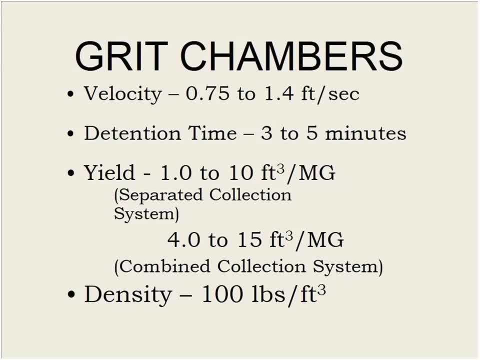 per second we had through screening, down to about 3⁄4 to 1 foot per second. We're going to slow it down just enough so that the dense material can settle, but any organic material which is still lighter can stay in suspension. 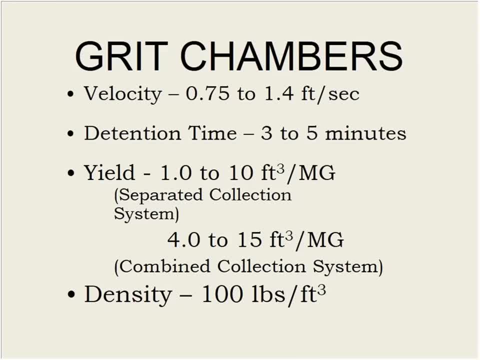 We don't want that settling out. That has to go to the bugs. So 3⁄4 to 1 foot per second. Cut that full in half, And we do that just by expanding the area we're calling. The one thing about this business is: you cannot stop it. 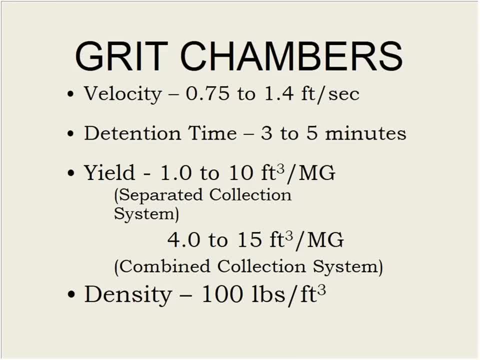 No matter what's going on, No matter what's going on in your plant, this water keeps on coming. You can't close the valve and say, well, I'll fix this, Slow it down, I don't have time. It keeps on coming. 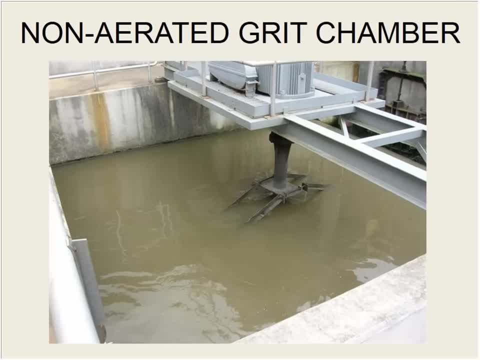 Again, very dense material, about 100 pounds per cubic foot, so it settles quite readily. This is a non-aerated grid chamber. Again, we've just expanded the area of flow, slowed things down so that the grid can settle out in this chamber. 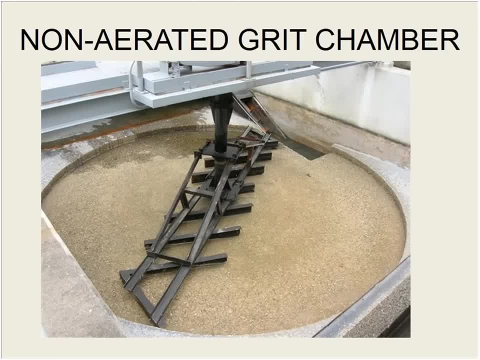 And it's going to settle down into this area And on a timer. So the grid mechanism is slowly going to plow it down into that little sump you see up in the upper right corner there, And then they've got a screw conveyor to drag that material out of there. 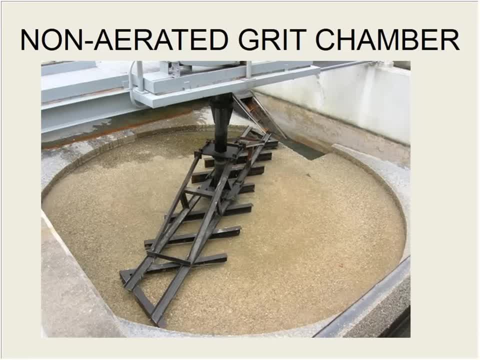 The thing about it is this could be Yammer's mask. They've got a system like this: The material comes in, goes through their flow meters, goes directly into this. Again, it's old wastewater, so it can be rather odorous. 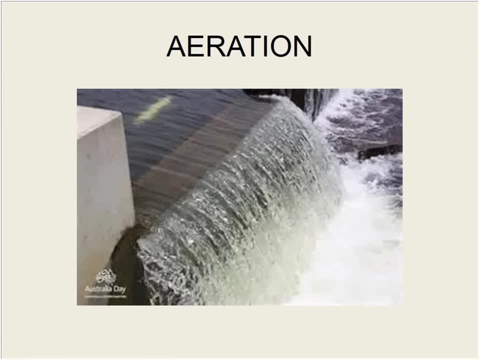 So it's going to settle. So one way that we try to do, no matter what our system is, we want to get some oxygen back in this water to shut down any kind of anaerobic operation. or even some of the faculty, The ones that are non-aerated grid chambers, tend to have a drop afterwards. 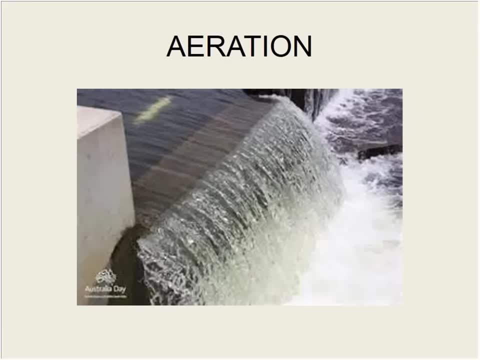 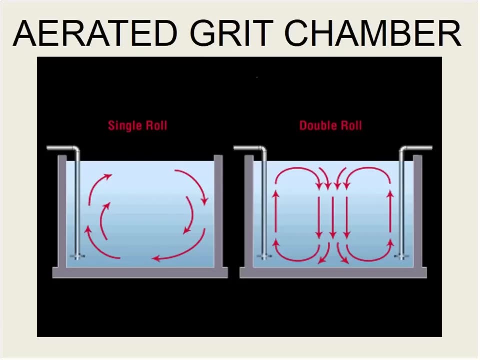 It's going to flow over a dam. drop a couple of feet, That's just enough to aerate that. very well, get it back up and shut down any anaerobic activity. Now this picture is depicting an aerated grid chamber. This is where we're actually going to pump air in. 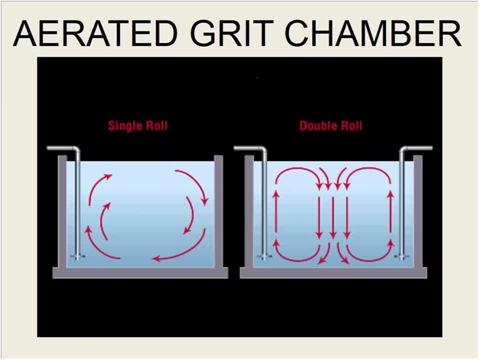 It has two purposes: We're going to freshen the wastewater, It also facilitates the settling of the grid And you see, the pipe over here on the right-hand side is going to inject air and it causes kind of a swirling action inside the chamber itself as it moves through. 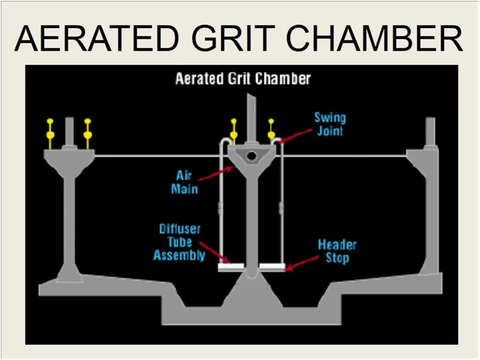 It changes the apparent density of the water, so the material settles more readily and freshens it up at the same time. Down at the bottom of this portion here you're going to have some sort of a removal system, a chain and bucket or chain and flight system to take it away. 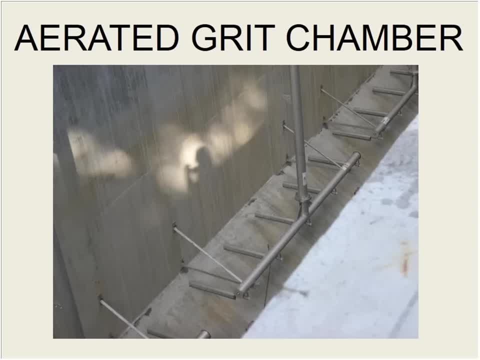 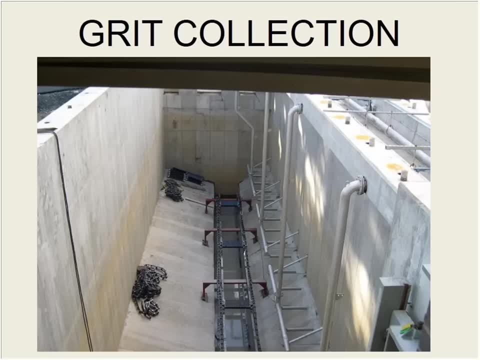 You've got to drag this stuff out. So this is upper Blackstone, when they were going through their renovations. You see the aeration pipe here on the side And then down at the bottom is the chain and bucket system. It's going to drag the grid out of this unit. 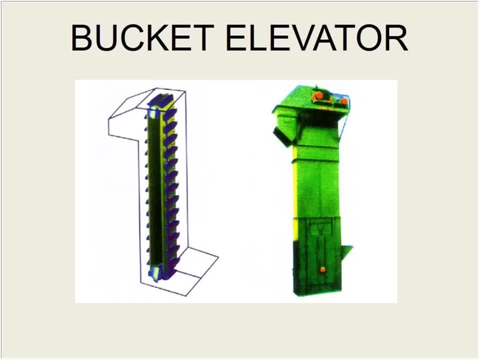 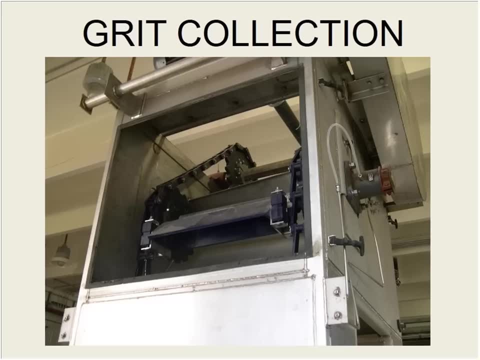 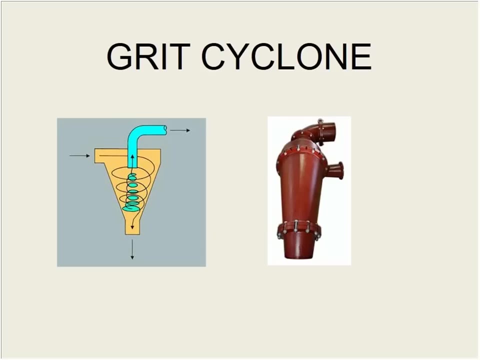 Brings it inside. We've got a bucket elevator. It's just a continuous belt with these buckets in there. It hoops up material and then flings it out of the top to wherever it needs to go- See the bucket. Some facilities, instead of doing this method, pump their grid out of the chamber and run. 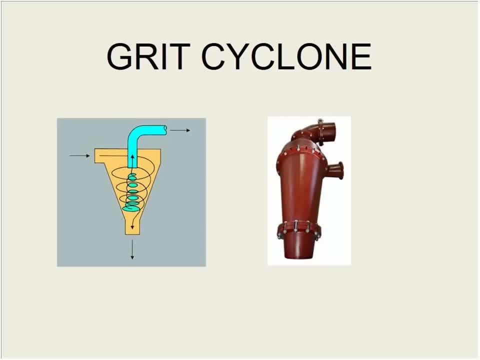 it through a cyclone. Cyclones are very good for concentrating solids. The material comes into this cone-type device, comes in tangentially. The material spins around. The solids go to the wall and get pushed down towards the bottom apex. Clear water comes towards the center. 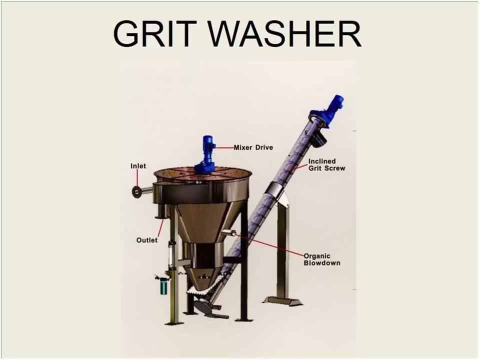 The solids go through that center pipe And this, much like the screenings increasingly- is being washed. before we send it off, We want to make sure there's no organic matter resting on it before we do It's sent into a tank like that. 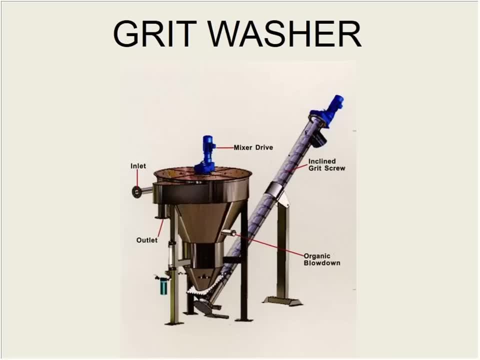 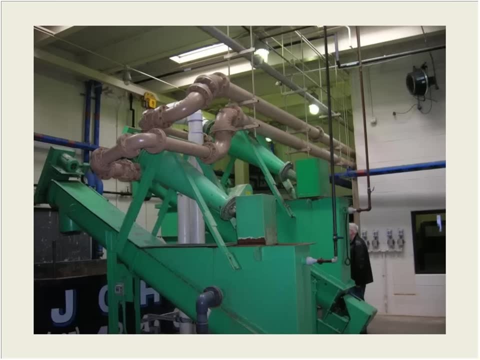 The water washes off the organics And then this screw conveyor will remove the grit. It de-waters very well The grit classifier. This is down in Wallingford, Connecticut. There's their cyclones right there And here's the grit washer. 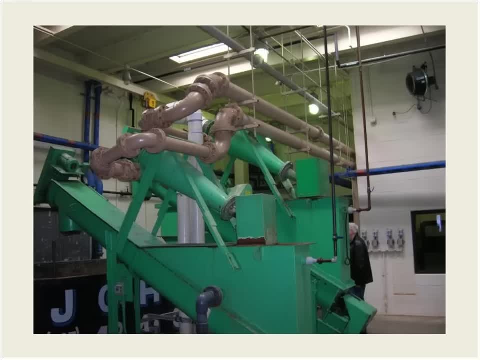 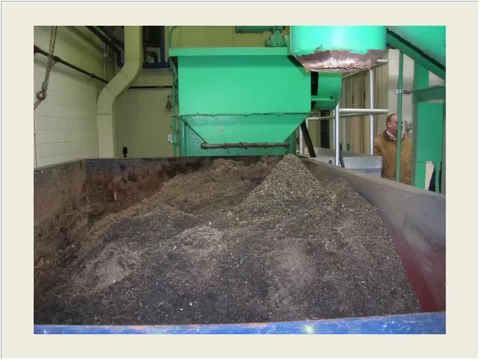 There's Chuck Conway's head back there And that's grit. It's just what it sounds like. It's grit. It de-waters very well. You don't have to worry about moisture content with these generally Off to a landfill. 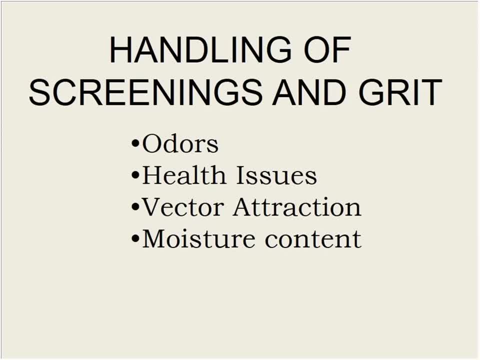 It's gone Again, things that we're concerned with, certainly odors. There's two smelly parts of a plant. It's going to be your headworks building. It's going to be your solids handling- Again headworks because of the nature of the old material coming in. 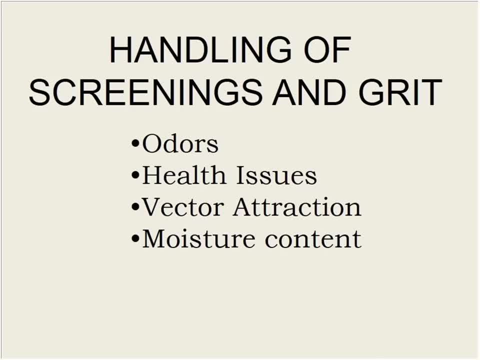 It needs some air, But we have to have odor control for that particular area and its operations. The health issues: This is raw wastewater- Good, bad, otherwise we don't know. We assume that it's just nasty stuff with bad bugs in it. 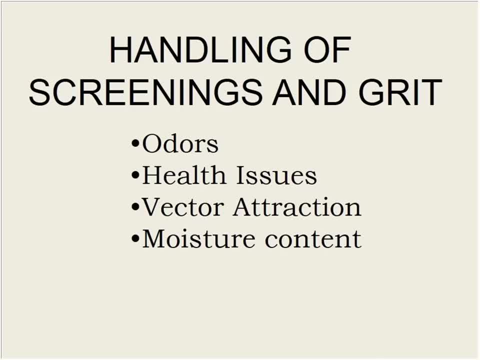 We have to deal with the vector attraction. Wash the organics off our stuff before we get rid of it so it can go to the landfill and they can't get after us And the moisture content. Total landfill: you typically have to have greater than 20% solids of whatever it is you're sending. 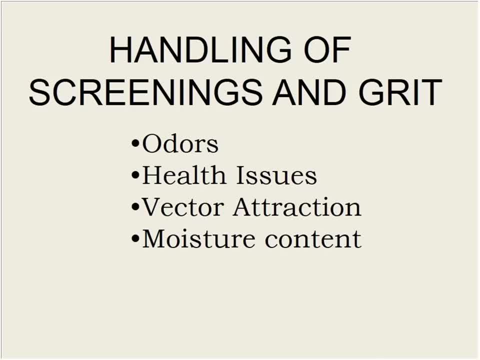 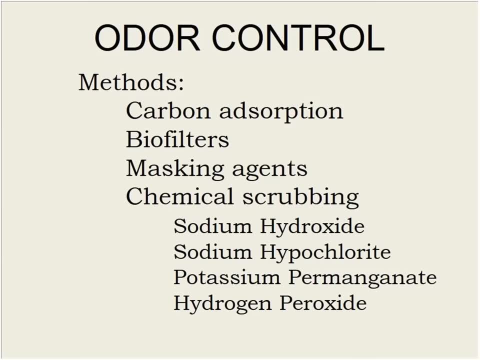 So we have to try to make sure that it's dry enough to be able to go without any problem. Again, odor control. These buildings tend to fall under an odor control situation as time goes on. A lot of different ways of dealing with the air. 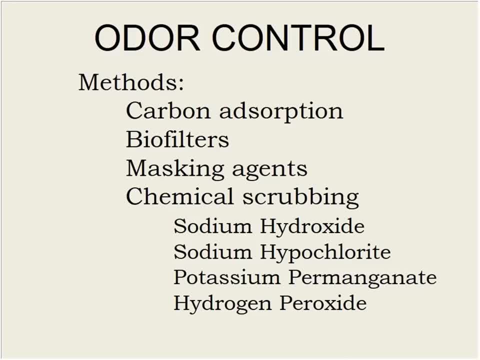 There's carbon absorption. There's biofilters. You can use chemical scrubbers with various chemicals in there. Worst comes to worst, Use a masking agent. It's just like spraying cheap perfume all around the building and it smells as bad as the building it did before. 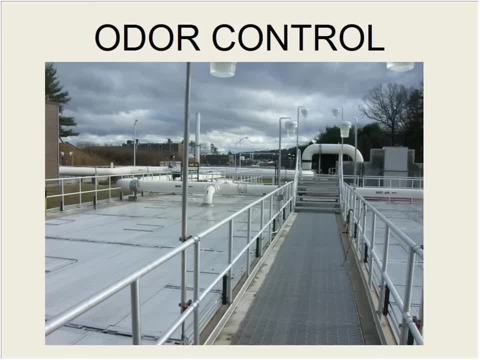 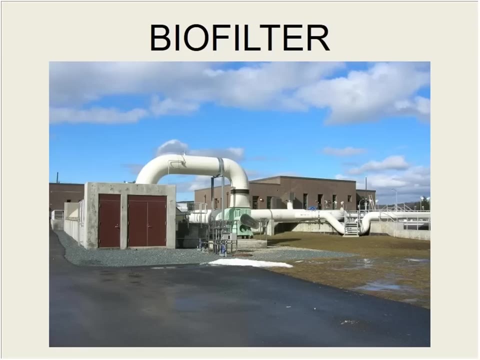 This is Upper Blackstone's new aerated grid chambers, Totally enclosed. All of this white piping is all fiberglass piping that goes off to a biofilter. They do a very, very good job. This is the biofilter here: All of the air from this building, from both buildings, from their aerated grid chambers. 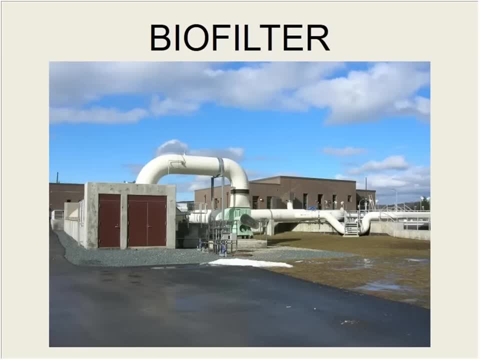 all come through this piping and pass through this Biofilter is really just the big tanks filled with a media. It could be wood chips. They actually have a foundation of lava rocks. Remember back in the 80s You'd get a grill. you had those funky little lava rocks. 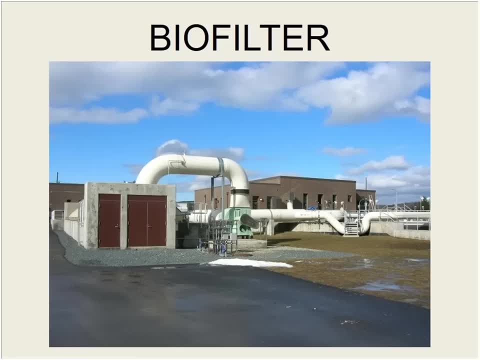 Loaded with that and then a bunch of wood chips And organisms actually live on that media and will consume the odorants as it goes through. So the block at the end of this where it discharges- You don't smell a thing. That's a very, very good job. 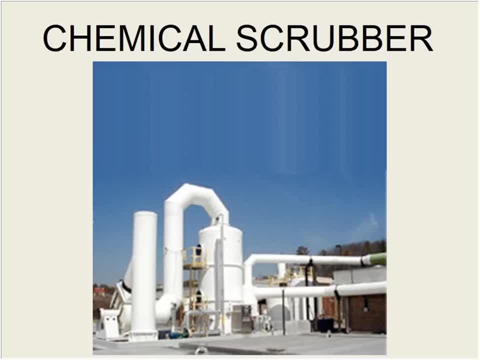 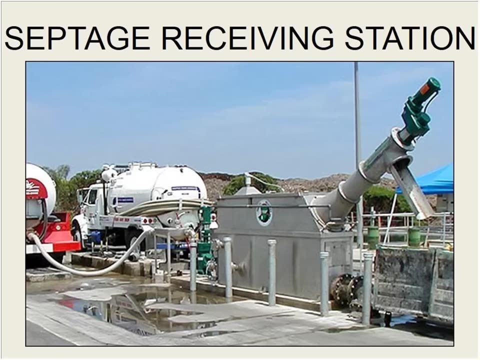 Some facilities will do chemical scrubbing. They'll run the air through a scrubber to knock it down. Sodium hydroxide, sodium hypochlorite- Very common methods of scrubbing A lot more complicated. So what you see here is a septage receiving station. 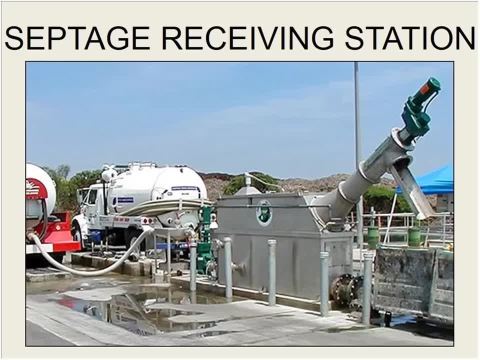 A very nice septage receiving station. Not everybody lives on a collection system and goes to a treatment plant. A whole lot of houses out there that have septic systems. There's other systems out there And all of that sludge from those things needs to go someplace on a regular basis. 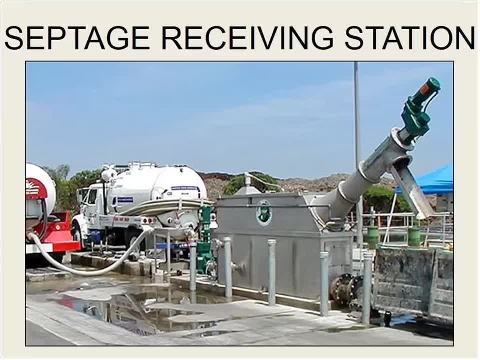 You can't be like my father and run your septic system until it finally pops up in the backyard, And so it's a good revenue source for a facility, But it has to be managed properly. Swallow flames in particular. This is concentrated wastewater. 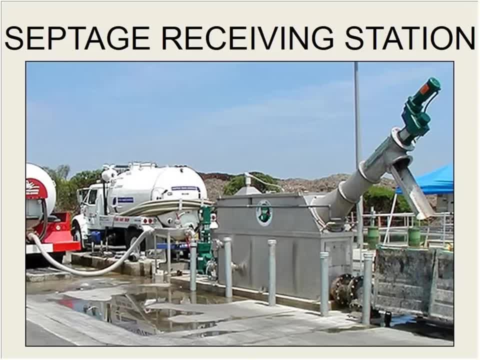 This to grow wastewater is like espresso to a latte. This is crack cocaine for bugs. So you've got to be careful with how you manage this stuff And also, you never know for sure what's going to be in those tanks. It's good stuff. 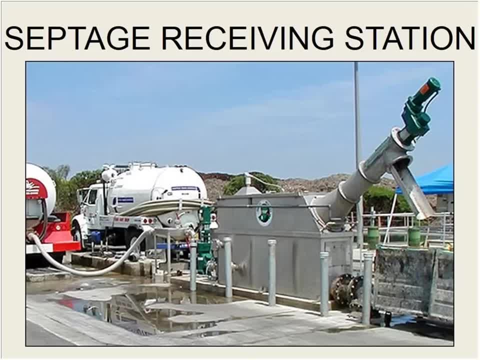 It's a screening device. It acts as a screening unit, Takes out all the Legos and the kids' toys that went down the toilet, WPH readings on those to make sure that they're within ranges and stuff. It's a good way to deal with things. 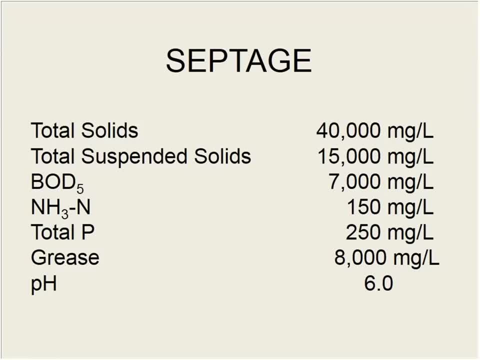 But if you look at it, if you remember our solids coming in, our raw wastewater is about 200.. This is what you're getting out of a septic BOD: 7,000 instead of 300.. It's rough stuff. 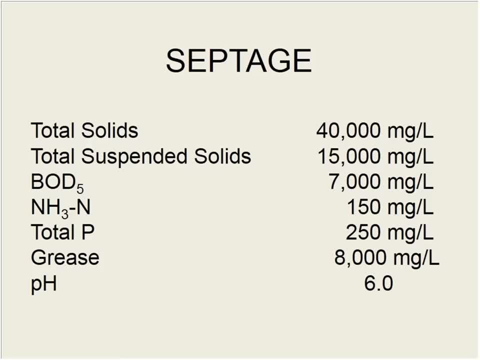 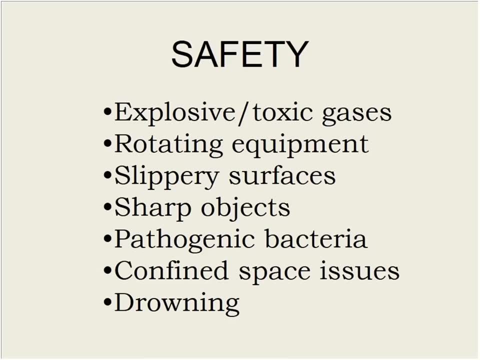 You've got to deal with it. You've got the whole ammonia phosphorus thing to deal with, So it's not one of the nicest places in the planet. And you've got the whole thing of Drowning- It's water. 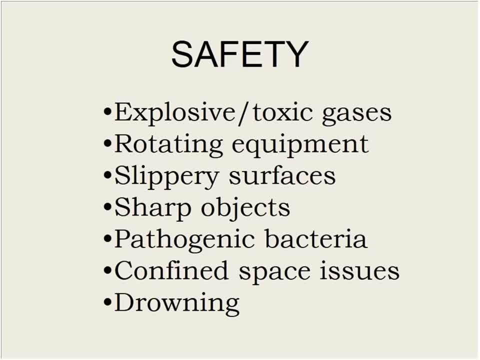 What's that? I'm sorry. I thought drowning That's a good method. What is that? What Drowning, You fall in. No, That's horrific. That's the kind of rule you do: Don't fall in. 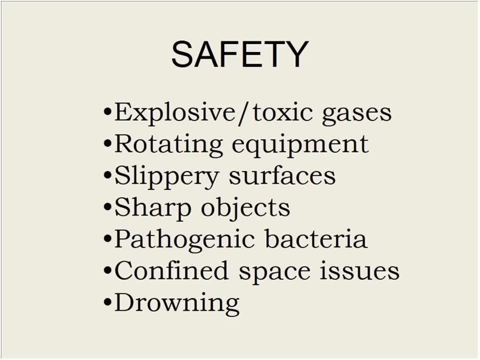 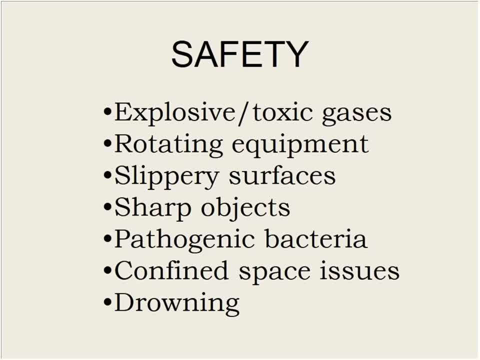 gases, So explosive toxic gases, when this stuff finally comes to light possible. You've got rotating equipment, those screens as sharp as all can be By the nature of the things going on. the floor is always wet in there. 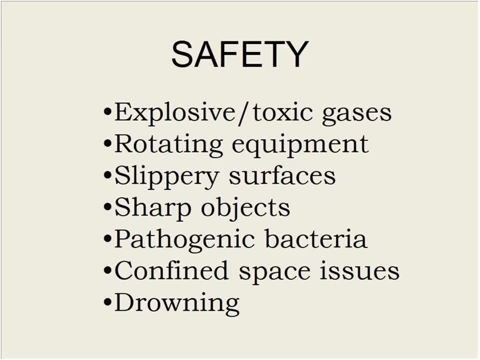 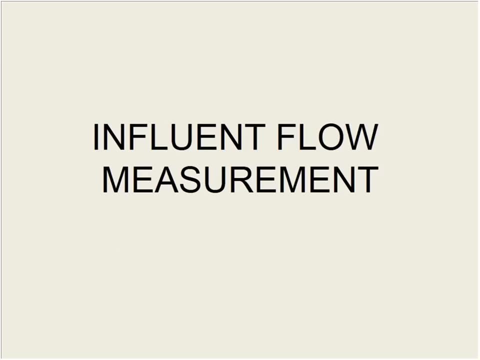 You never know what's going to come off. You've got hypodermics and what have you all out there. You want to be careful. Certainly we still deal with pathogenic bacteria. It's not a great place to be. I've worked at a lot of different companies, dealt with a lot of nasty chemicals and wastewater. 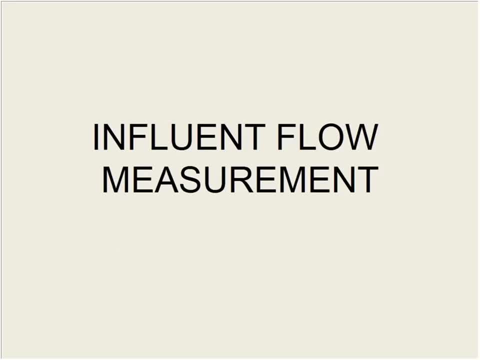 treatment can give you just as much danger as any of those places I've ever been Interesting. So we've taken out the stuff the bugs can't eat. We've taken out the two-by-fours and the pots and pans. We've taken out the grit. 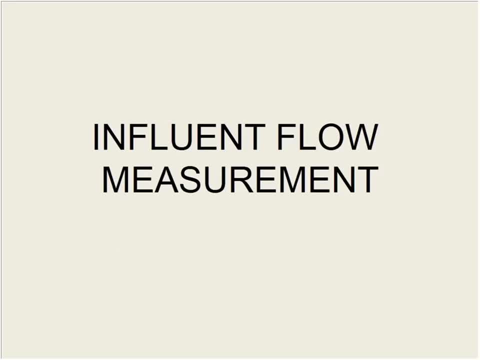 So it was relatively clean looking. but we need to now measure our flow. It's generally at this point that we measure the flow. I think Amherst mass is kind of an outlier. They measure before they get all of that stuff. 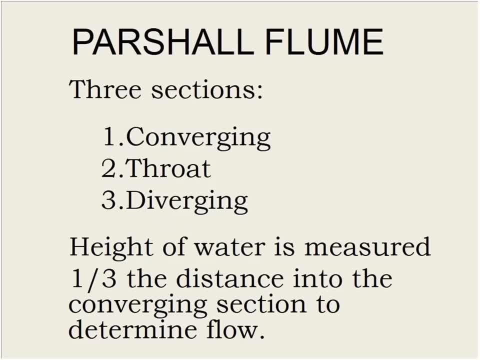 Most people will wait until that's done. We need to know it because we have to report that on our EMRs every month. We need to know it because we want to run our plant. We need it for process control. What's our flow? 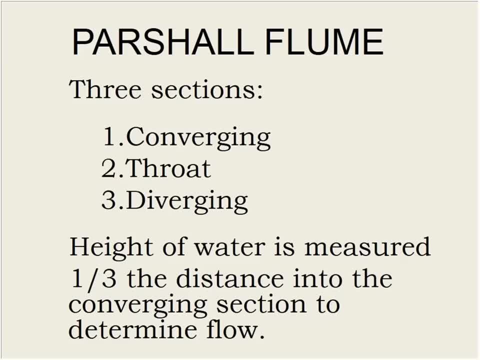 What's coming in, What's going on? Probably the most common method of measuring flow is a partial flume. A partial flume is an open-channel flow device. It has three sections: a converging section, a throat and then a diverging section. 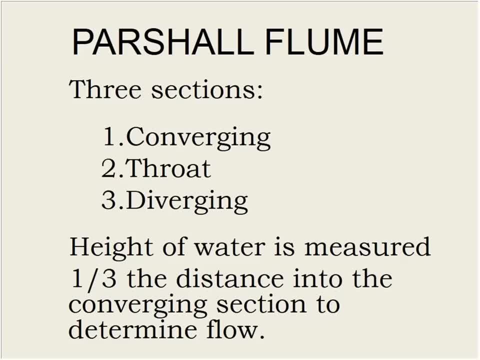 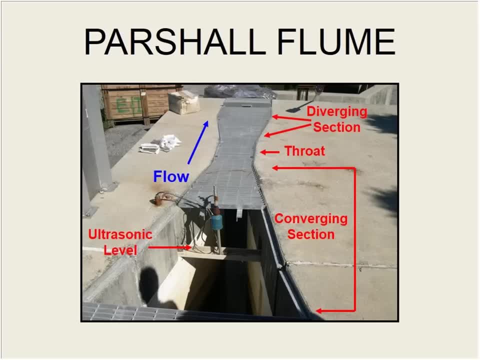 It's got a particular contour to the flora. also, It's set to give a certain velocity through the flume. We're going to measure the height of the water one-third the distance into that converging section. This is the Little Devil in Villarica. 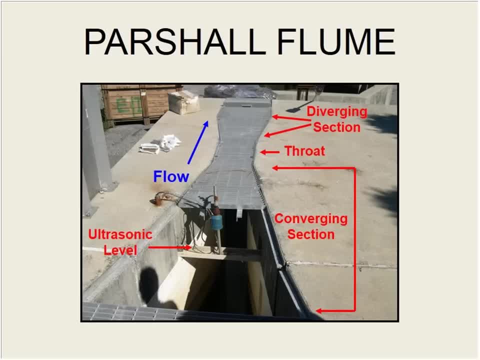 It's only a two-million gallon plant, so it's kind of small. You can see the converging section, There's that throat and then there's the diverging section. We measure it with an ultrasonic level device. It measures the height of that at this point. 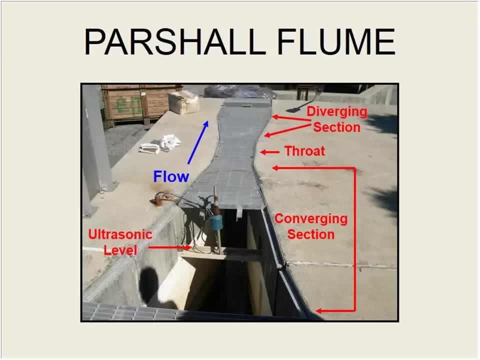 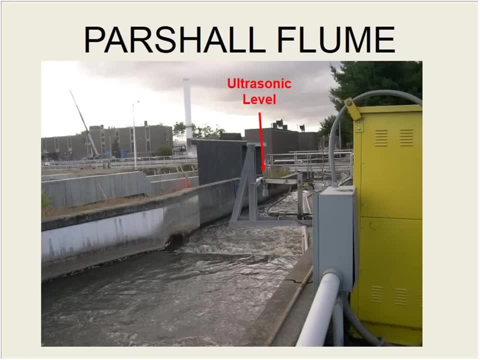 At that height, the area of flow changes, We can calculate what our flow rate is through the flume. This is Upper Blackstone, one of the biggest flumes around, probably the biggest one in the region. It has about 11 feet across its throat. 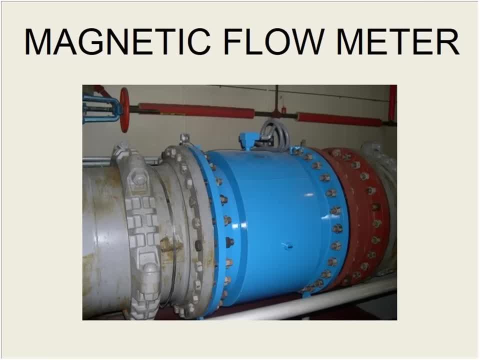 Again, it's our ultrasonic level device. There are other methods. This is up in Nashua. Nashua has a magnetic flow meter. As you see, it's a closed piece of pipe. What it does is it sends a signal across this flow. 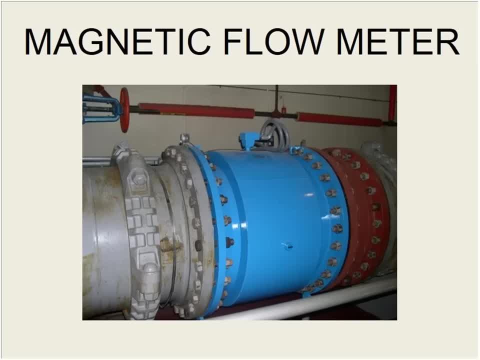 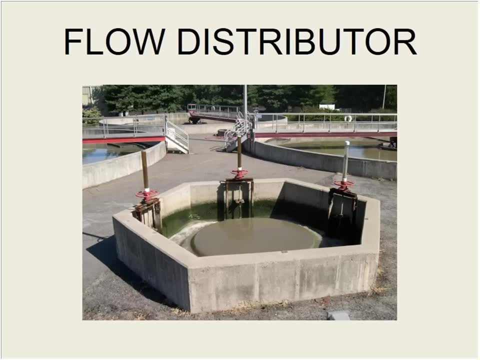 As it's deflected, it can determine the change in the velocity through that pipe. We can make the calculation Again at this point. we're going to go into primary treatment. We're probably going to have more than one clarifier for these operations. 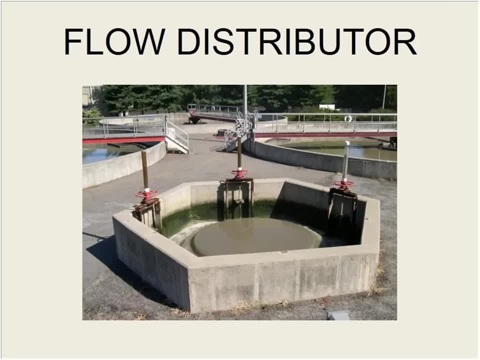 That's what you see: these three circular tanks behind us, The blossom here, The class we're heading next, and, depending on our flow rates, we may need all three, We may need one, We may need two. We have again some method of controlling the flow to whatever number of units we need. 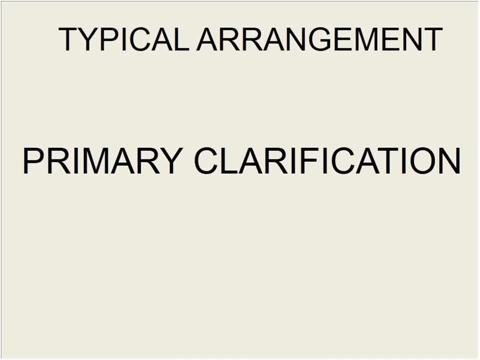 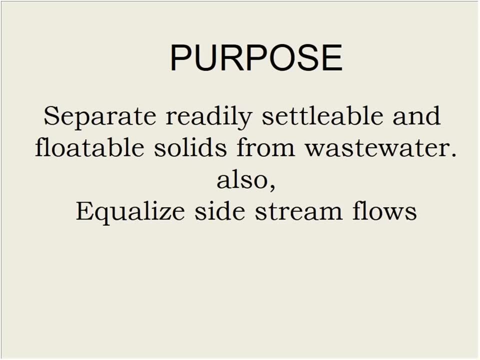 to have. We're going into primary treatment. Our next step It's a physical operation. We're going to separate readily settleable solids- the stuff we saw on the bottom of that iron half cone earlier- and any floatable materials. It's also where we equalize side streams. 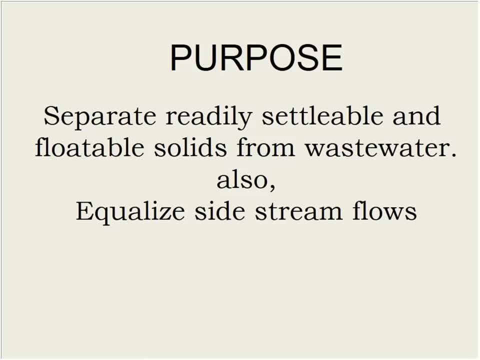 All of the operations that are associated with the solids handling part. Again, when it comes to solids handling, we're taking material that probably comes out to less than 1% solids and we have to get it to better than 20.. We've got to squeeze all that water out and that water has to come back at some point. 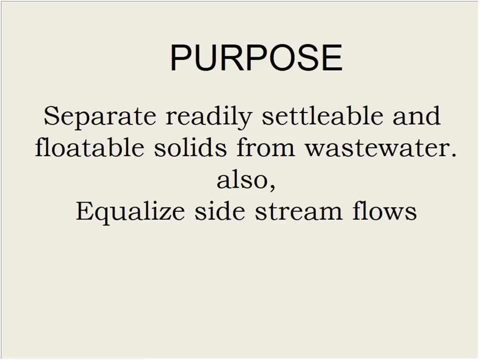 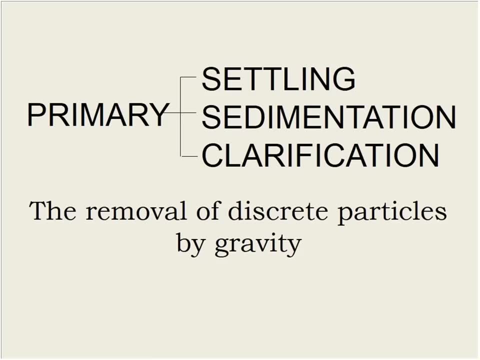 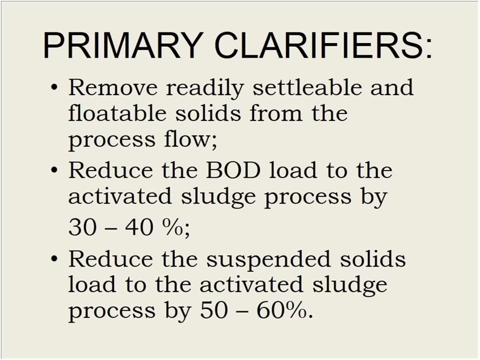 This is generally where it starts to come in. These terms all mean the same thing: Settling, sedimentation, clarification, Settling of discrete particles by graph. We're going to remove readily settleable solids. We're going to reduce our BOD by some percentage- 30-ish. 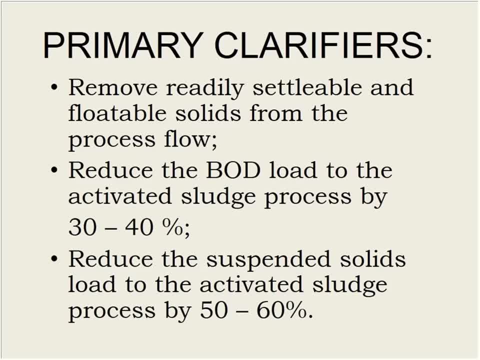 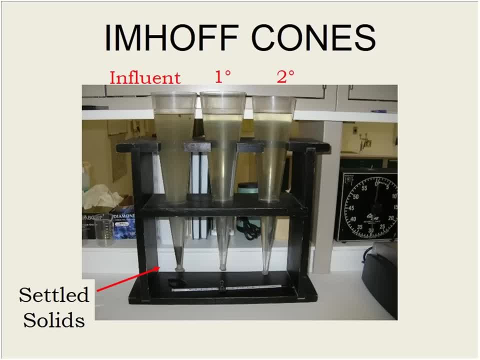 We're going to take some of our suspended solids out during this process too. That's what's going to happen on this step. We have talked about that settleable solids analysis. This is what's coming into our primary treatment. This is what it should look like afterwards. 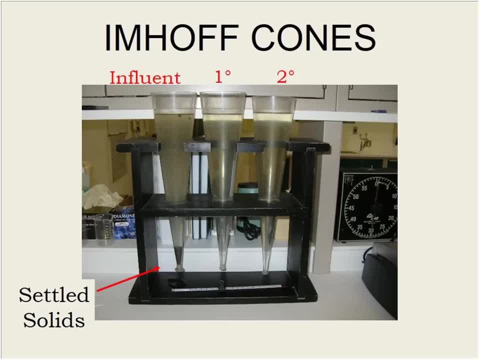 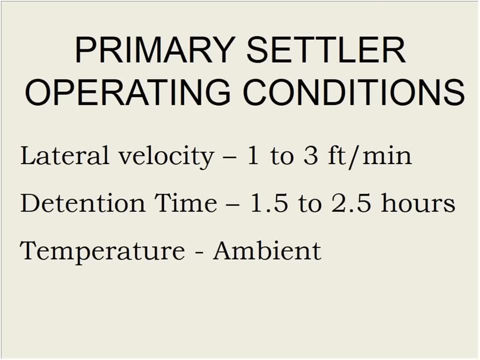 Nothing floating up here, Nothing settling in the bottom of the cone There to there. That's our whole job Again. what we're going to do is we're going to slow things down yet again. Now we're going from one foot per second to one foot per minute. 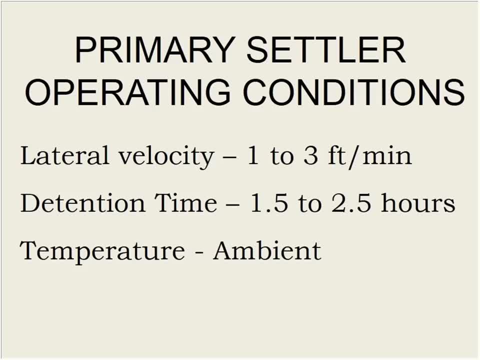 It should look like still water in these tanks One foot per minute. We'll go that far in a minute. That's pretty slow. Primary settling an hour and a half to two hours is sufficient. That's probably the summer time. This is probably winter time because water is denser in the colder temperatures. 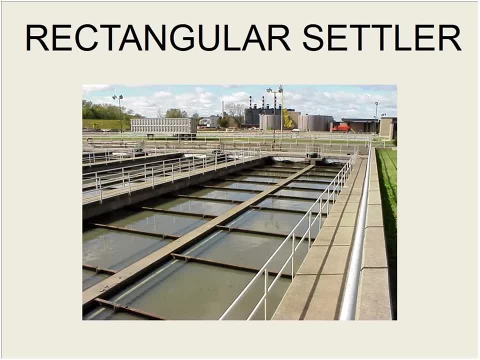 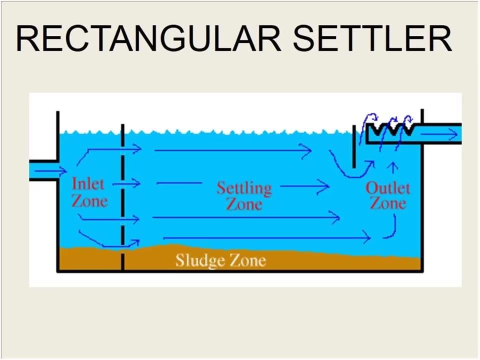 We have to deal with our expectations as a result of that. This is a rectangular settler. They're big tanks. This is a cross-sectional area. Those are rectangular tanks. We're going to come in here at the left And again we want to make sure that we're in the right place. 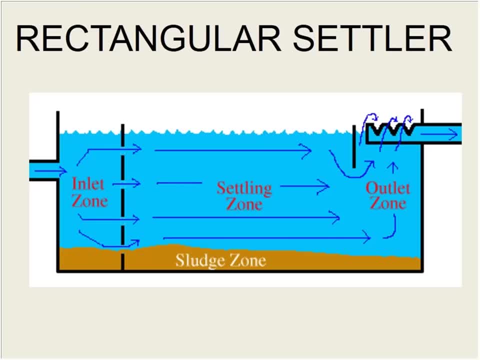 We want these to be as quiet as possible, So we just can't have this flow come charging into a tank. It will cause that, So we're going to have a baffle here to help slow that velocity down and spread it across the entire face of the tank. 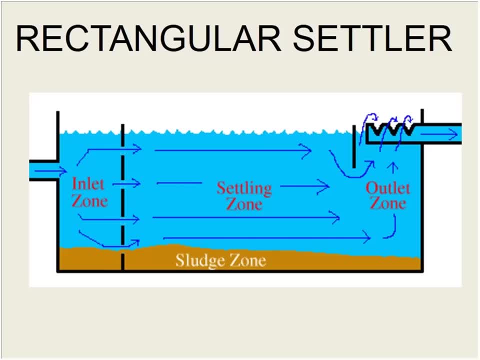 Water is going to move at one foot per minute. It doesn't discharge yet. As it does, solids will slowly drop down to the floor. Floatables will slowly rise to the surface. At the far end we've got a baffle layer. 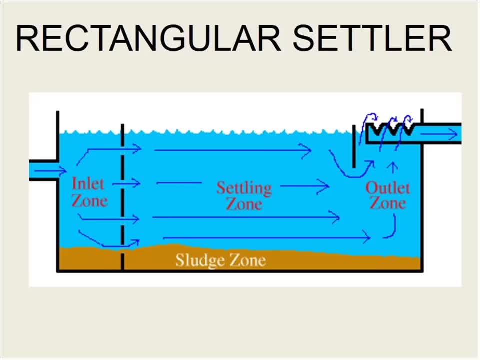 The floatables won't continue and come up with our effluent. We've got a baffle that goes some distance below the surface, Our solids we're going to drag out to another device And our settled water then overflows into a trough or launder to go away. 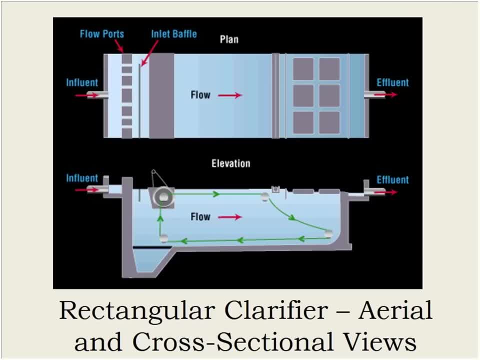 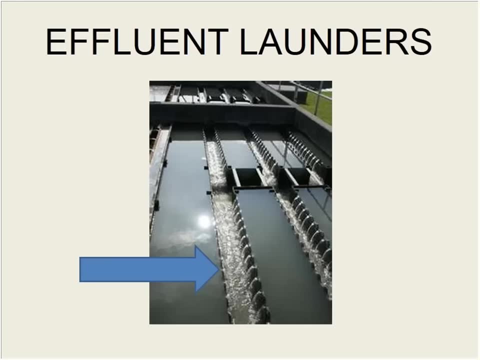 Here's another view of it. It shows the actual sludge scraping device. It pushes solids, floatables- in one direction and solids in the other. So our settled water at the end is going to overflow into, it's going to pass through a weir, into a trough that we call a launder. 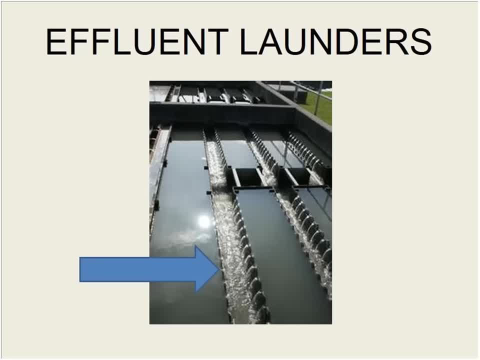 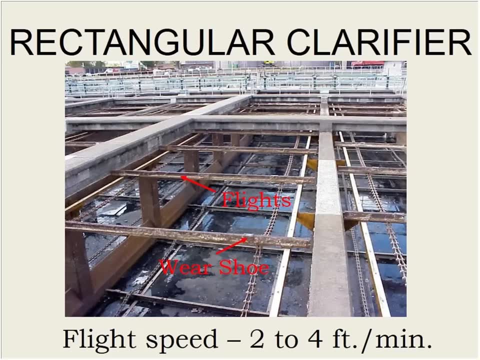 In that term we're talking about that trough that receives the cleaner water. So here's the chain and flight system. We have to have some method to keep the material moving out of the tank. These blades originally were made out of wood. Now they're made out of fiberglass. 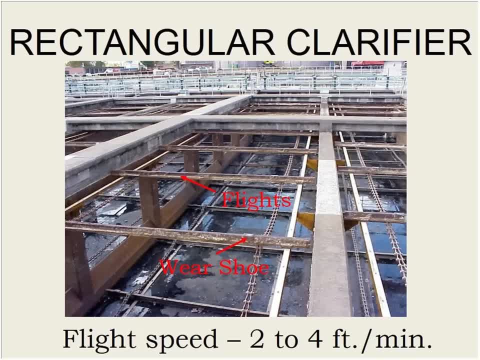 On the floor. they're pushing solids towards the discharge point. The ones at the surface are pushing the floatable material towards the receiving unit, And you've got some little units here Because this is dragging on the floor. you don't want to wear out this 60-foot hunk of. 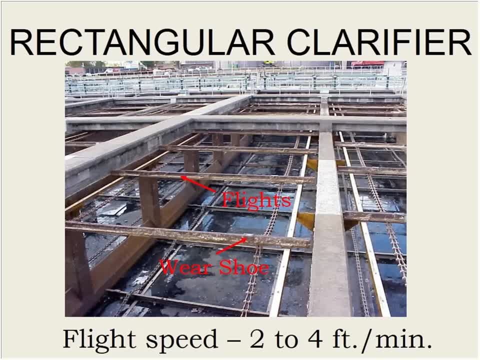 fiberglass. You've got all of these W&R replaced on, So we have sacrificial pieces of plastic on them called wear shoes. Those will wear out rather than the entire flight. It's a whole lot cheaper to replace. They travel very fast. 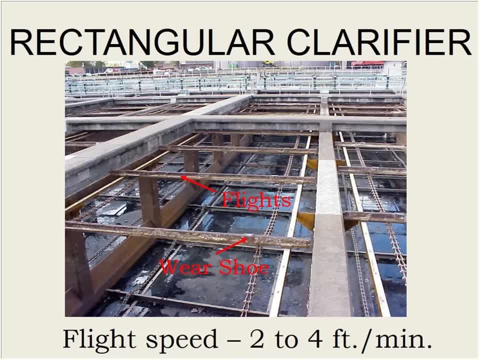 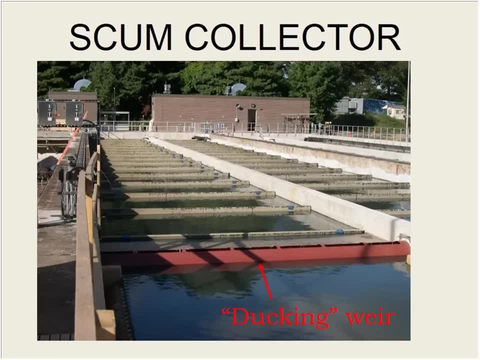 They move very slowly, Very slowly as they move And we don't want to generate any currents if possible. This is upper blackstone. You can see the flights at the surface. They're pushing the floatable material And, if you can just make it out right over this pipe, a change in the coloration of the 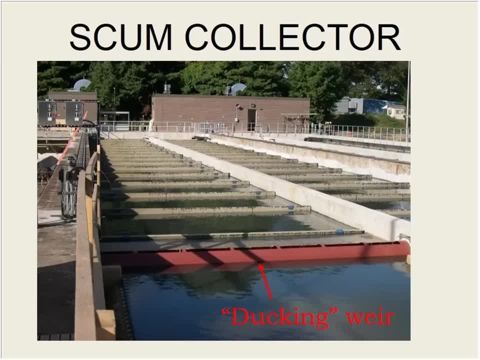 water surface. that's your accumulated floatables right there. This pipe here is what's called the ducking weir- Two purposes: It serves as the baffle. It's a good-sized diameter pipe so it goes well below the surface. Floatables can't get past it. 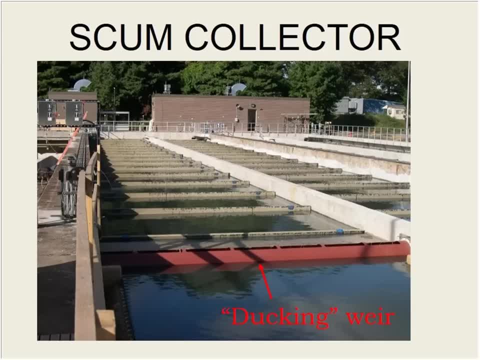 On a timer you can see the opening is cut into the top of the pipe. That pipe is going to rotate towards the inlet side so it goes just below the water. That floatable material will flow into that pipe and then go away to receiving tank. 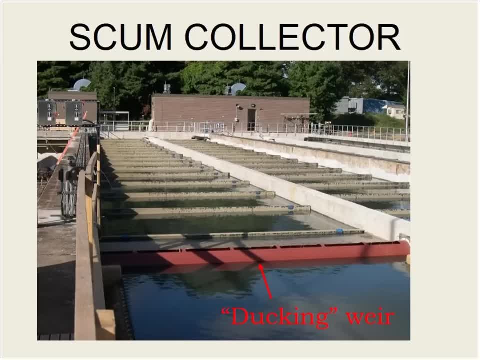 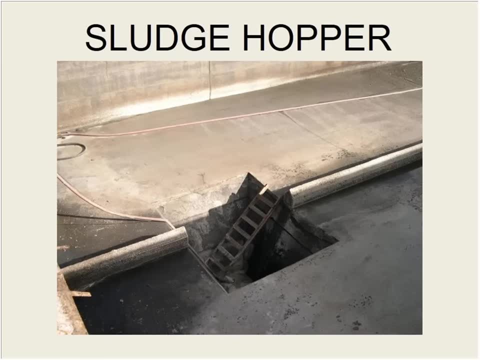 We've got nice clean water on this side of it. On the floor sludge is being pushed back, and that's generally the case. Sludge is generally pushed back towards the influent end of the tank. So push it down here, down into this sump, and then it gets pumped into the solids handling. 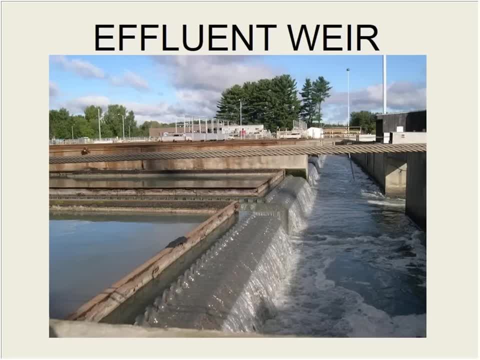 unit And what you have here is baffle, mold baffle on these units here. Relatively clean-looking water And for many years this was the treatment for most cities: Primary treatment. they disinfect, Boom. They left 30% of the BOD in there. 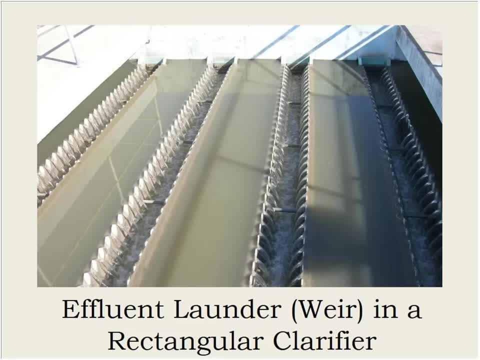 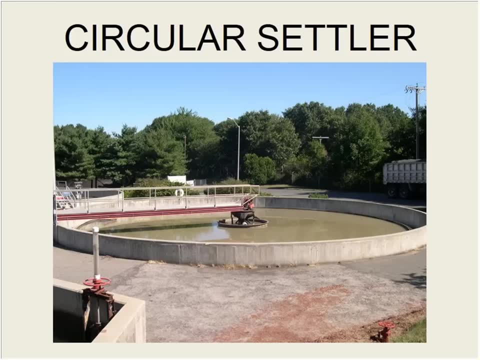 It's that water. Water flows up, flows into this trough and travels off. It can also be done with a circular settler. Rectangulars are much more common on the primary end because economy of construction: You've got common walls and civil engineers build these places and that's what they like. 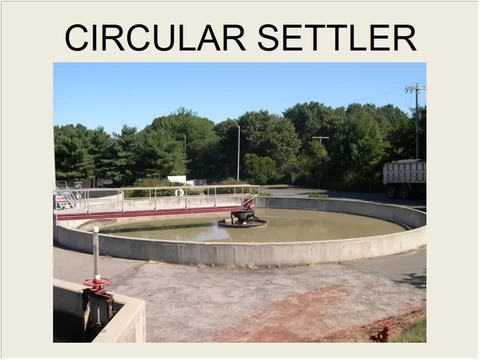 I haven't picked out a civil engineer yet, have I? I'm grateful to clarify. This is in Billerica, Same thing. Water's going to flow into a well here in the center. It's going to slowly work its way to an overflow weir on the outer circumference of the tank. 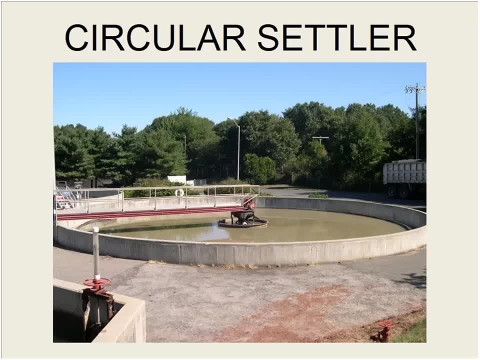 So let's go here There. we go Up in through here. What we've got is another baffle. It's a big circular wall. It's about three feet below the surface, So the water comes in The tank goes straight over to the effluent. 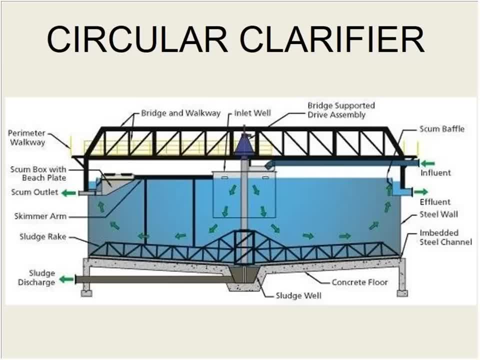 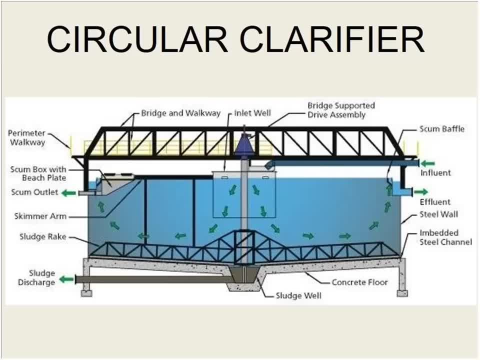 And then it's going to go down And then it's going to go down. It's a big circular wall. It goes about three feet below the surface. So the water comes in The tank goes straight over to the effluent. It has to hit that wall, come down and slowly work its way up. 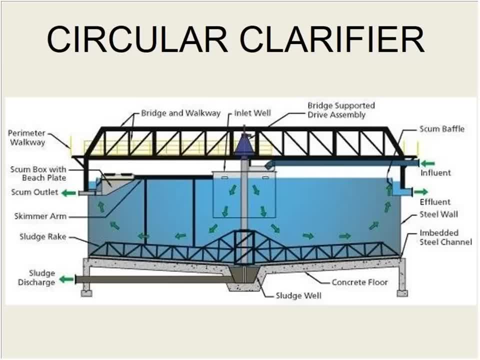 Again, one foot per minute. Solid's dropped to the bottom, Floatables go to the surface, hopefully. Well, it's good We've got a rake mechanism that's going to plow this into a well, And again that comes off to be pumped out later. 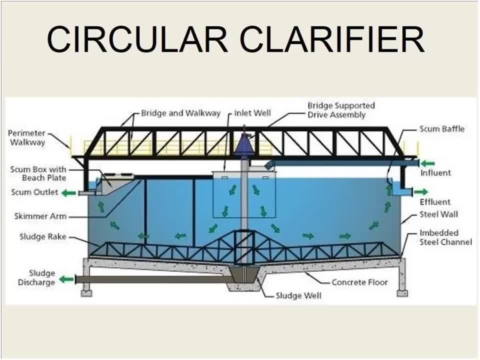 There's an arm there to pick up the floatable material, Skims it off into a receiving unit. at the surface It's a big circular wall. It's about three feet below the surface, So the water comes in, The tank goes straight over to the effluent. 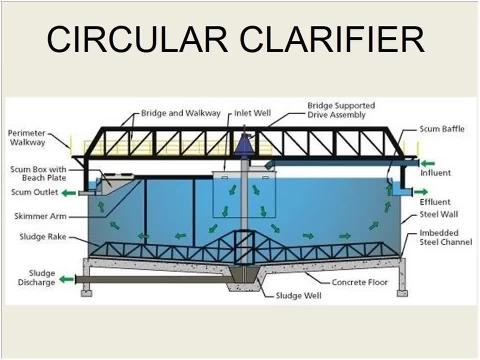 It has to hit that wall, come down, and then it's going to go down. We've got a rake mechanism that's going to plow this into a well And again that comes off to be pumped out later. There's an arm there to pick up the floatable material. 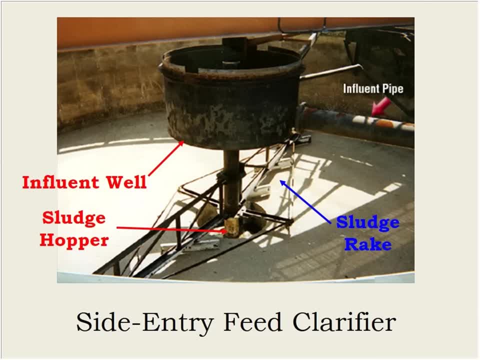 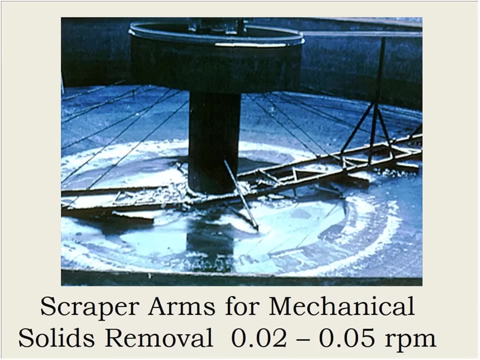 Skims it off into a receiving unit. at the surface You can see that baffle here, A big steel wall, And then there's a rake mechanism. There's that sludge. well, down at the bottom Again, it turns very, very slowly. 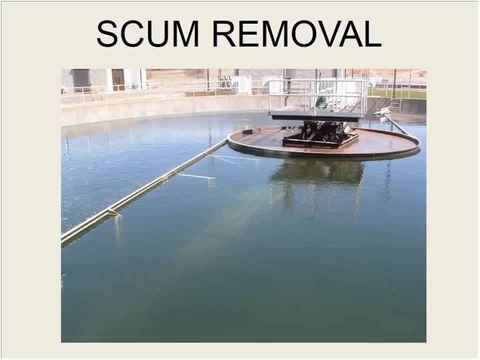 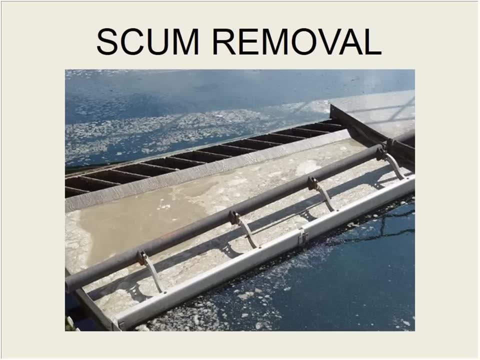 All right, So there's the For any floatable material. this arm's going to pick it up and push it around And it's going to come up with this wiper here that runs it up this little ramp. It'll drop down into this opening here to remove the floatables from the water. 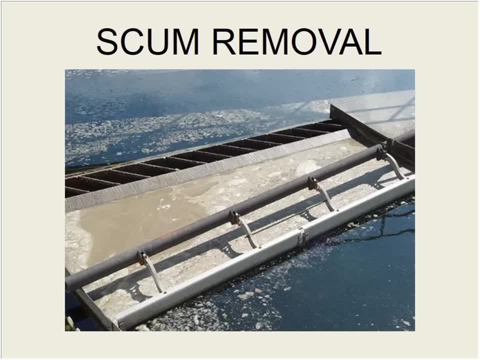 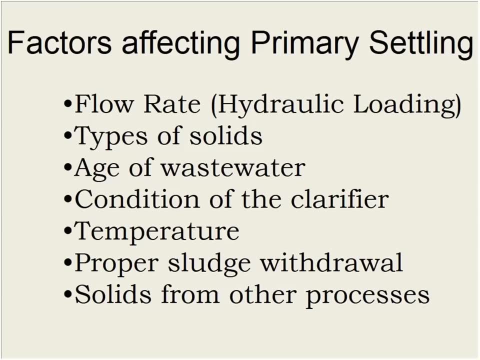 Sludge goes to the bottom and gets plowed into the stuff. It's pumped away. So things that we're considering is outflow rate. Again, we want to run within certain ranges. So if we've got a lot of water, we want to run within certain ranges. 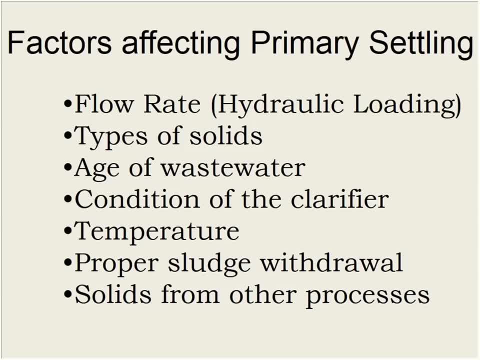 If we've got a lot of water coming in because of rain or what have you. we need more clarifiers. We've got a certain rate at which we want to run these in terms of hydraulic loading, The type of solids that are coming in. 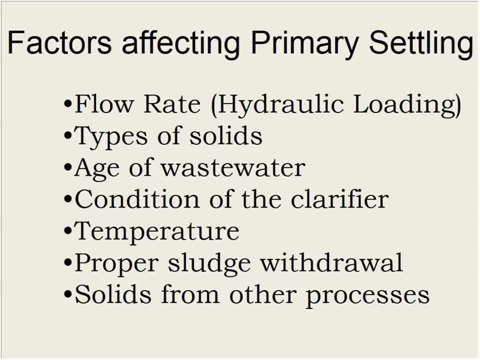 Old sludge doesn't settle as well The age of the wastewater Condition of your clarifier. obviously Temperatures are going to affect it. Things don't work as well this time of year as they will in August. How fast we take it out. 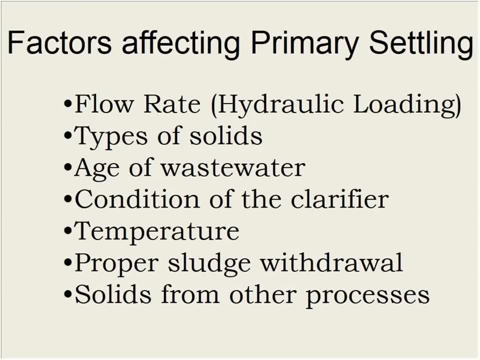 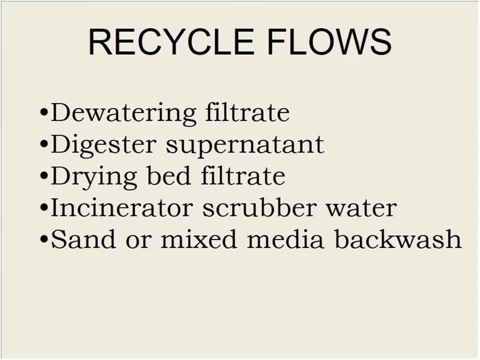 Again. another factor is: whatever's coming back in. Do we have thickeners, Do we have belt presses? Do we have incinerator water? All that stuff comes in at various times. It affects things, All of these materials Further down the road. 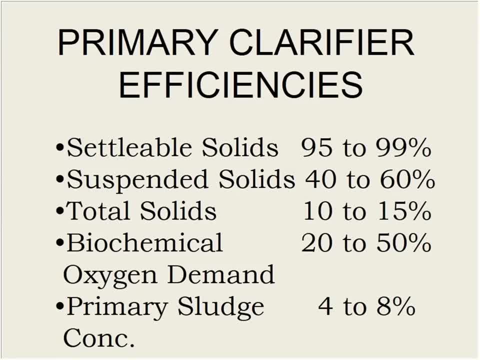 But at the end of the day, if all has gone well, we've removed 95 to 99% of settleable solids And all of the floatables. We've lost a little bit of total solids, Some of our suspended solids. 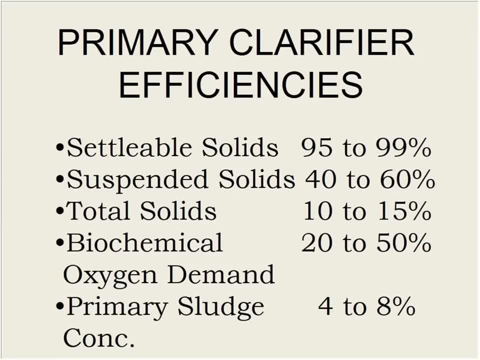 Our VOD has been reduced. I wouldn't go to 50%, 20 to 30, probably, And we've got a sludge that depends on how fast we withdraw. It might be 4% or so, Which is pretty decent. 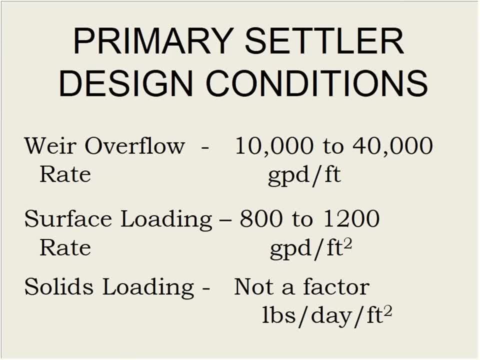 But it's not the highest volume We've got to talk about. we want to run these things in certain parameters, And this is what dictates how many units we're going to have at any particular point in time. The three things that we look at. 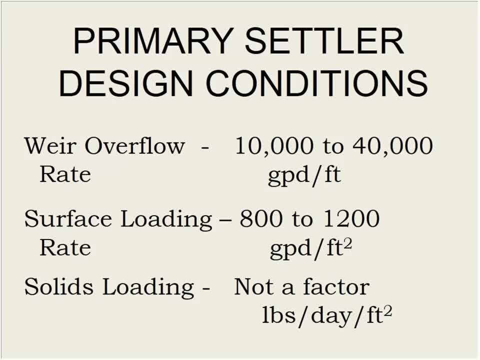 A wear overflow rate, A service loading rate, Solid loading doesn't really matter. A wear overflow rate is gallons per day per foot of wear. Again, you can see 10,000 to 40,000.. These things are pretty forgivable. 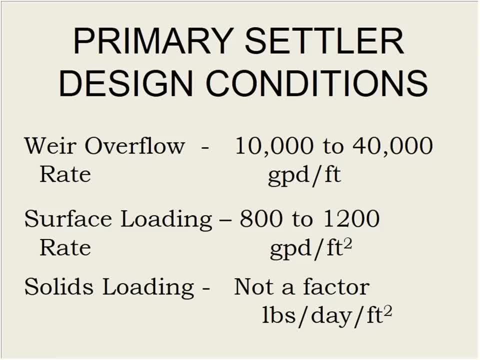 They can take quite a range of flow before they fail. Figure out how many feet of wear you have on your tank. however, it's designed And each foot should see something in that range. So if it's in August, I'm going to be down around here. 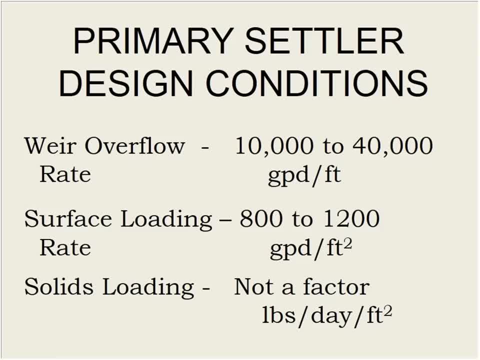 I'm going to be able to take some clarifiers off because I'm getting too low. I don't want it to be in there too long. Too long it'll start to decompose, It'll generate gases, Totally disrupt it. Surface loading rate is another one. 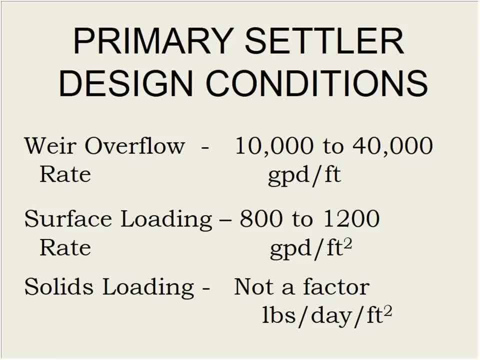 They're basically design factors. They're not anything a typical operator looks at on a daily basis. It's a design range, Tell you how many clarifiers you're going to have And it works back into your O&M manual. So when your flow is at this range, you want so many clarifiers. 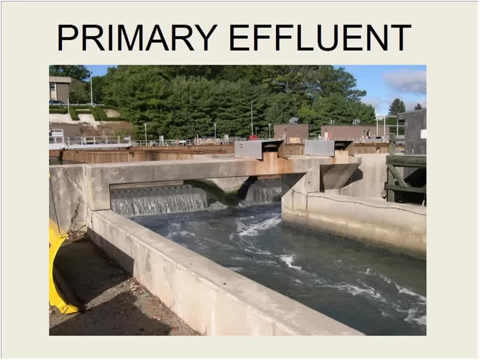 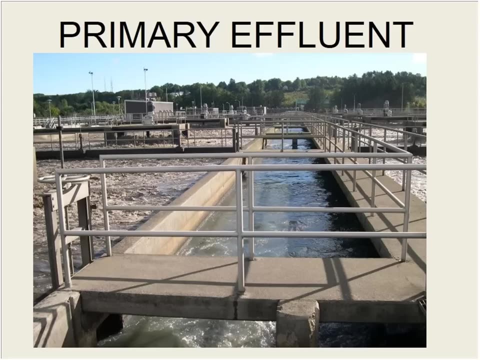 When it comes down here, you'll have fewer or whatever. This is our primary F4.. Relatively clean-looking water ready for secondary treatment- Blackstone- This is their old secondary treatment system on either side of this channel- Even their primary F4.. 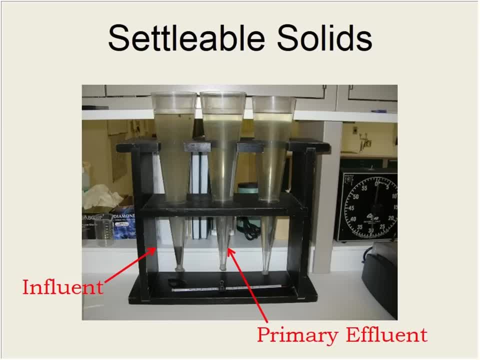 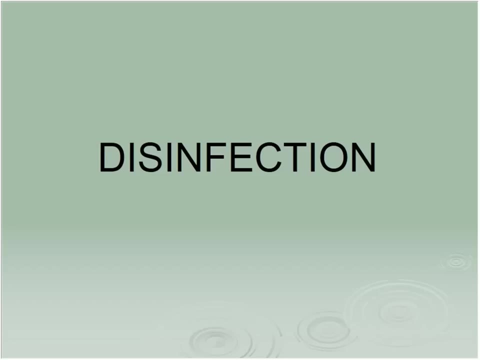 And again, this is what we've achieved. We've come in with this amount of settlables, a little bit of floatables, and we've got virtually nothing on either end after our primary treatment. Got anything in the question area? We don't. 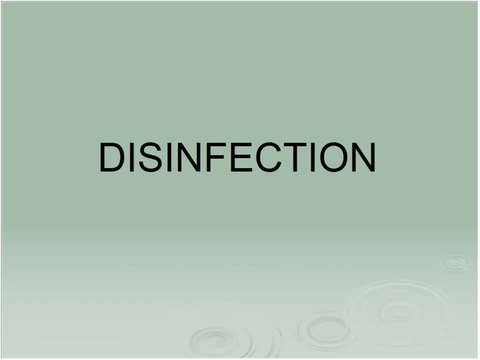 Online or calling in. I realize they haven't opened it up to our online audience. I'm either doing too well or they've fallen asleep. You all have questions. If they're calling in or if there's too much, we'll pass. There's a lot we've covered, so I'm sure you have questions. 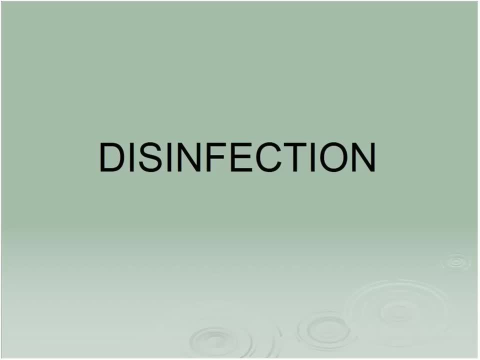 All right. Well, we're going to close this one here. Thank you, I'll see you next time. Thanks for listening, Thank you guys. Thank you, You're welcome. Bye-bye, I'm going to jump over the biological treatment, because that's going to take all of the next. 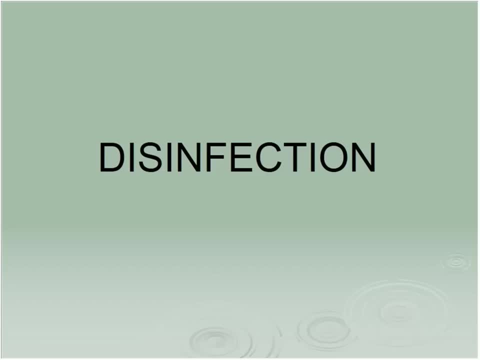 week to talk about. We'll go over the various aspects of that in more detail. We'll just jump over that and go into how we finish up the water before we continue. Alright, five minute break and we'll go back to disinfection. 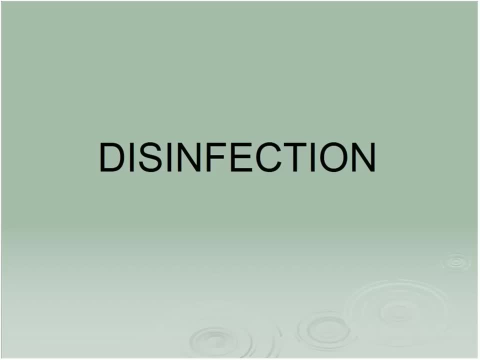 Alright, we'll go back to disinfection and we'll go back to disinfection. Alright, we'll go back to disinfection and we'll go back to disinfection. Alright, we'll go back to disinfection. Subtitles by the Amaraorg community. 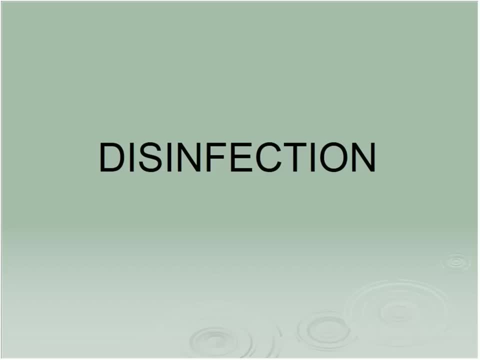 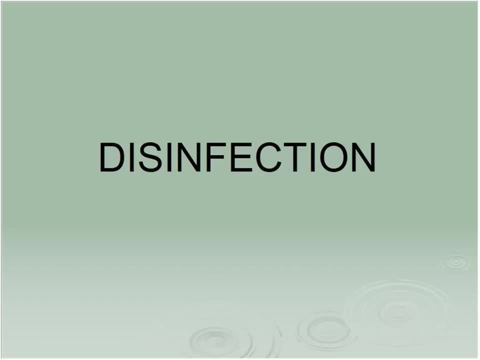 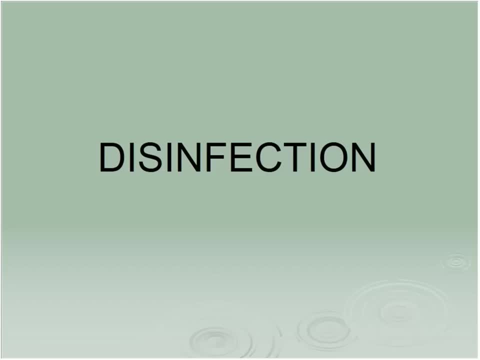 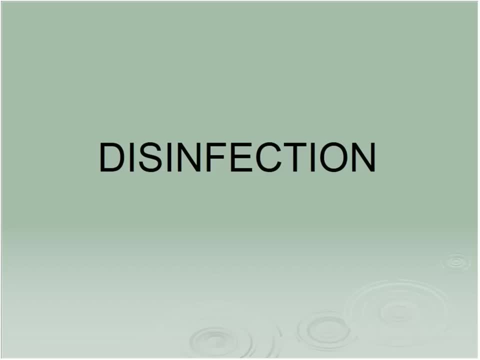 which can get very complicated depending on what we're trying to do. So we'll just jump right forward to disinfection. After the biological process, we go through starification once again. We have to take out all of those bugs that we generated during the process. 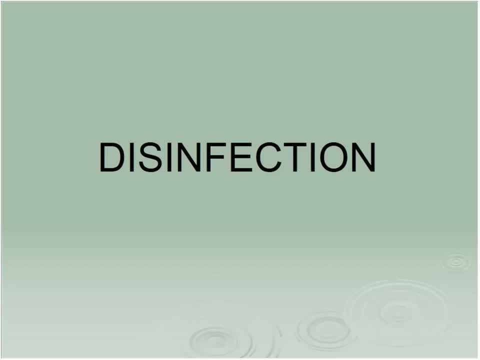 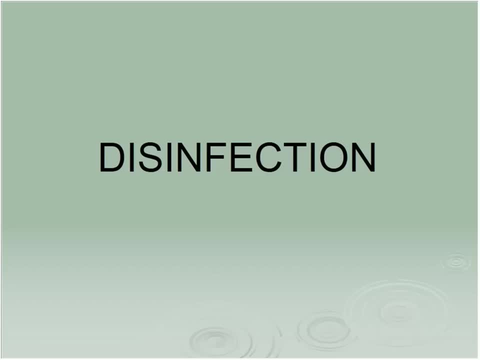 You're doing a good job. The one thing that we have not done anything about at this point is the pathogenic bacteria. To this point, we assume they're all pathogens and we treat them as such, but now we have to do something before we can throw this in the river. 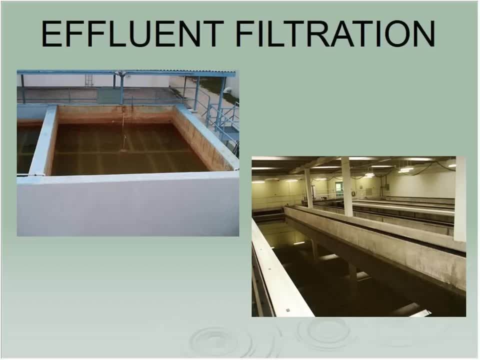 So we're going to go through disinfection Now quite frequently after a clarification step, particularly people who are dealing with phosphorus removal. phosphorus removal, particularly if you're using chemical, which is pretty much what you have to do to get down to the numbers they're looking at. 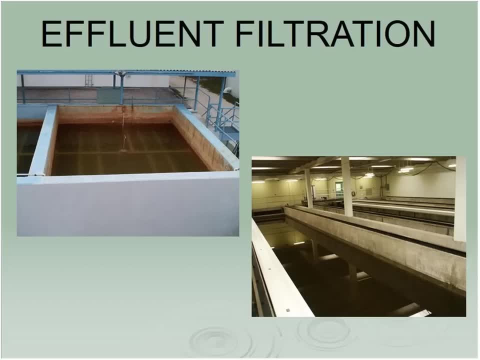 will leave you with a very, very fine clot that doesn't even settle out and have secondary clarifiers. So facilities generally are going to go through a filtration step before they discharge. in this situation, What you're seeing here are sand filters, A very common method. 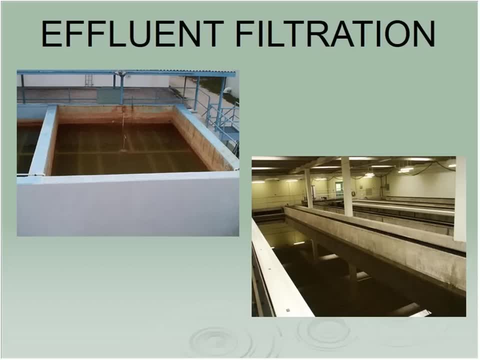 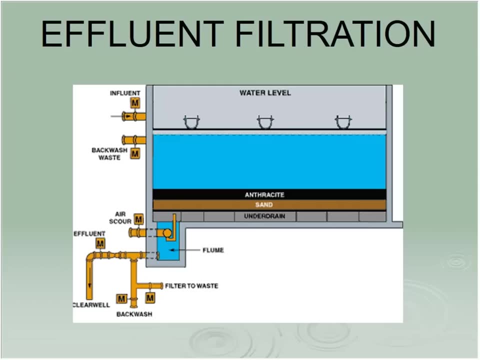 It's just a gravity filtration through a sand bed, But at some point that sand bed needs to be backwashed to remove the material that you're filtering out And that again goes back into the system Much like a drinking water plant. type of an operation: gravity sand filter. 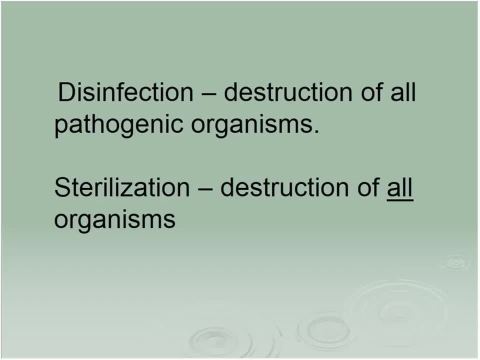 There are a lot of other. I thought I had a picture here of newer devices that are out there now: clot filters and that sort of thing. That has become a regular thing. It's just another step in phosphorus removal. So we're going through disinfection. 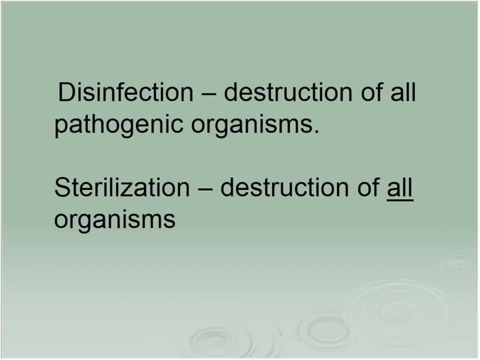 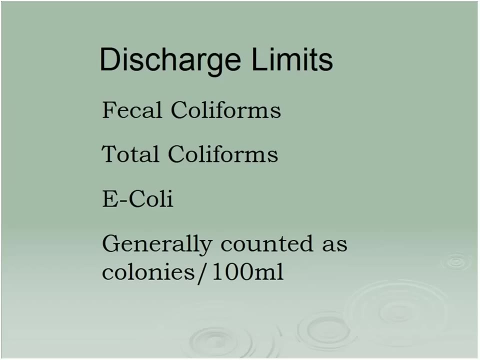 And we're not sterilizing, We're not killing all of the organisms in the system. We're just going to kill down to a certain point where we're comfortable that the water is safe to be dealt with. Now a little bit, we can be looking at various things. 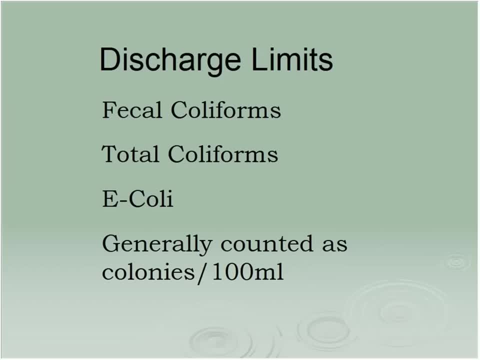 We can be looking at. there's going to be coliform bacteria of some sort. It could be fecal coliform, It could be total coliform. We can look at E coli. Some states are doing that. Again, we're generally looking at how many colonies we form in a 100-mil sample. 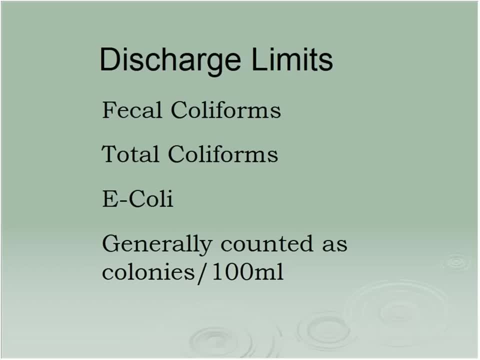 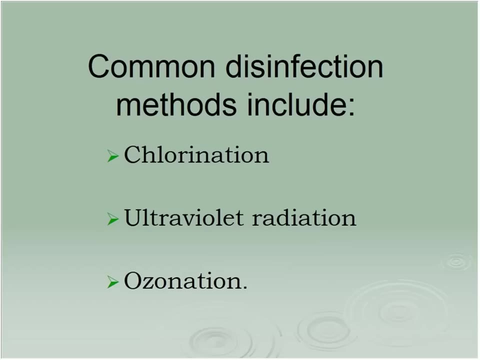 Coliforms again, are just indicator organisms. They're not necessarily pathogenic, But they're very stout. We know that if we kill them down to a certain point then we shouldn't have to worry about anything else. Common methods are chlorination. 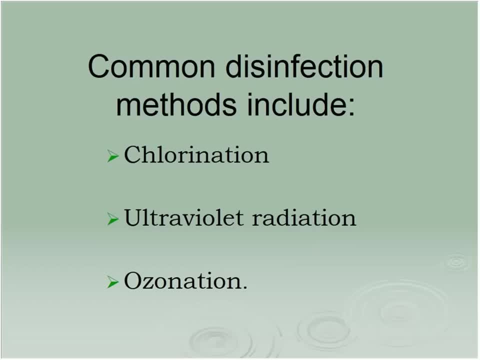 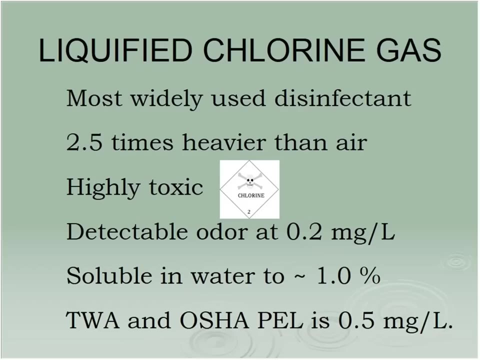 Chlorine has been a very common method for disinfection for a long time. We have ultraviolet radiation And ozone. while it's very specialized and difficult is starting to make some inroads into the process. Early days of disinfection: liquefied chlorine gas was the method to be chosen. 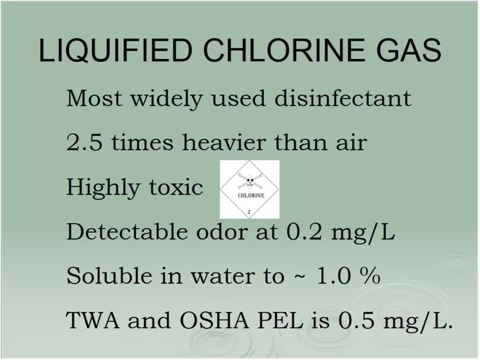 Chlorine was readily available. It was very inexpensive: $4.88.. You got a rail car. Why not use it? And it kills. It kills very well. It'll kill you if you let it Again. two and a half times heavier than air. 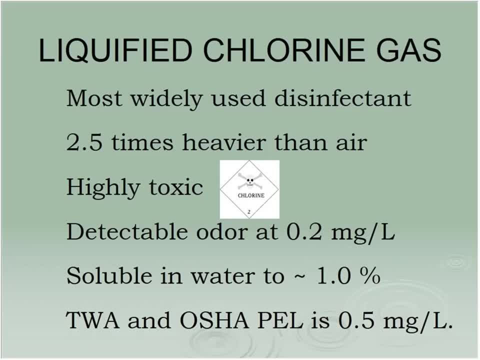 Any leaks then to pool distinctly at flow level. It's highly toxic. Smell it at very low concentrations. Just walked through our laundry area when my wife's doing white shirts. Smell it. Quite soluble in water. The O'Shapelle permissible exposure limit is half a pot per million. 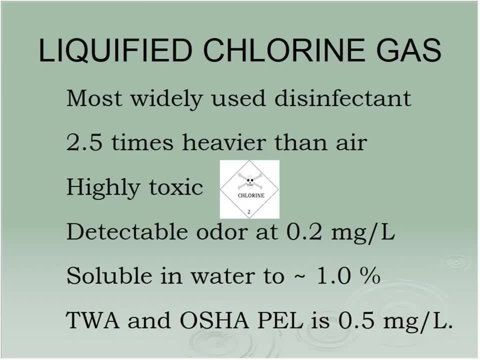 In air Half a pot per million, And if you read the regulation you'll also find out that OSHA states that nobody should be exposed to more than one pot per million. There's not a whole lot of buffer there. It shouldn't be smelly. 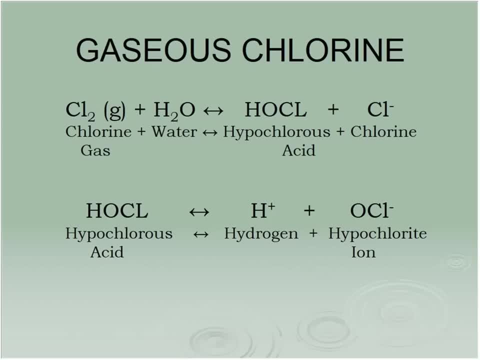 But this is what happens. Take chlorine gas, mix it with water and you form hypochlorous acid. Hypochlorous acid is the predominant disinfectant, So we want to make sure our pHs are in such that they're safe. 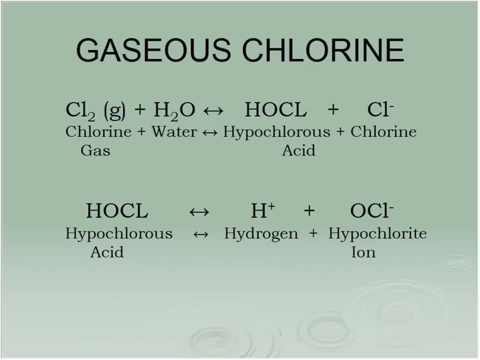 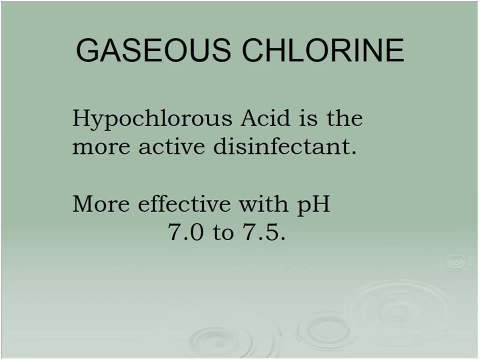 It's such that that is the ion that we're going to generate. So 7 to 7.5 is the optimum pH. That's where we're going to generate the most hypochlorous acid out of that solution. We can go above that and below that. 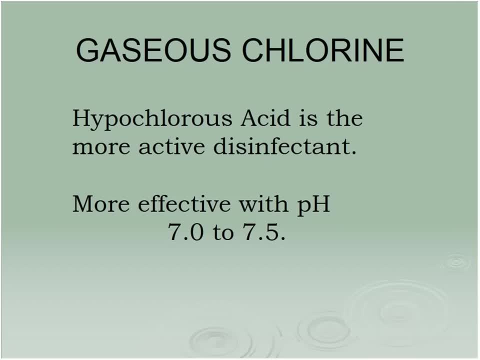 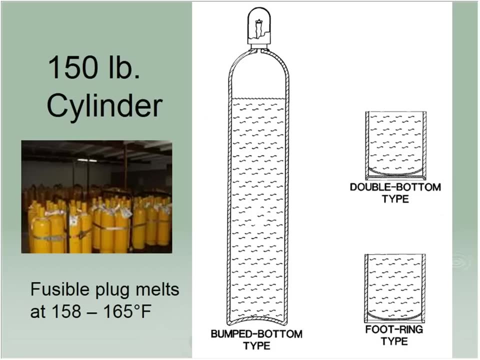 You tend to make more hypochlorite, which still works, but it's not quite so effective. We can purchase this material in three different containers. You've got a very small operation. You might buy it in 150-pound cylinders. It looks like your standard gas bottle. 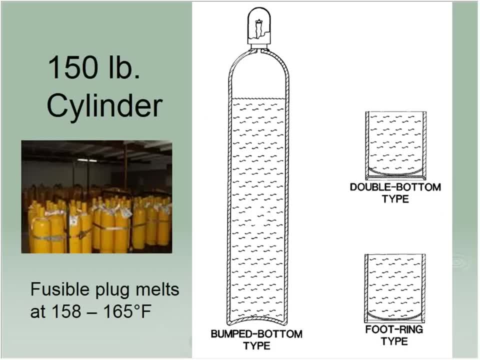 It's used in an upright position. It has a single valve at the top. That valve has a fusible plug in it that will melt at roughly 160 degrees Fahrenheit give or take, The idea being that we don't want this thing to explode. 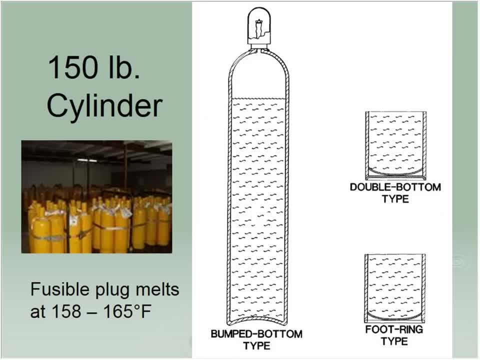 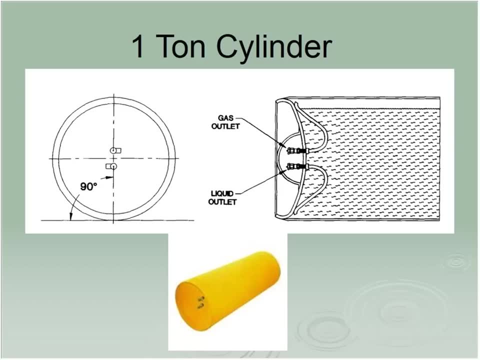 It's in a fire, It'll just release the gas and let the firemen do the work. I guess, More commonly, they're going to use one-ton cylinders. There are still a number of plants in Massachusetts that are using liquefied chlorine gas. 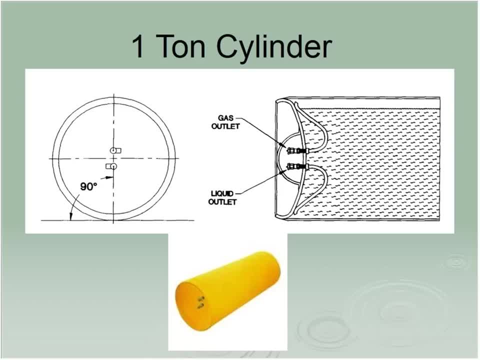 Amherst being one of them, Newburyport, I forget who else- A couple others. One-ton cylinder holds 2,000 pounds of liquid chlorine. It's used in a horizontal position. It has two valves. They sit on cradles that get the weight of the unit and also have rollers so that you can rotate it if you need to. 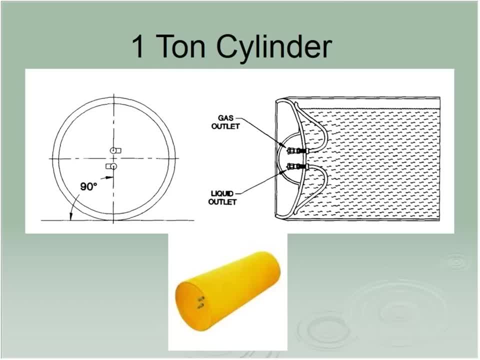 And you set it up so that the valves are. They are in a perpendicular situation one over the other And if you look internally, one of those valves will take liquid, The other will take vapor off the cylinder. If you've got a really big plant, you get one of these. 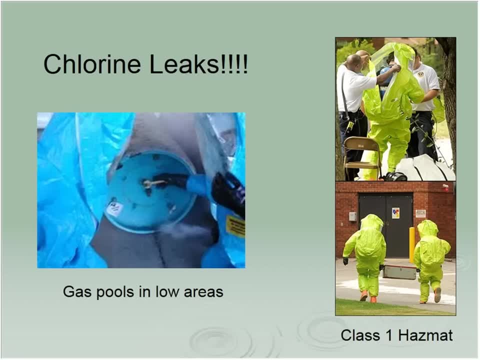 180,000 pounds, And this is why most plants don't use it anymore. Once you had this brownish-green cloud, go over the fence line, kill the neighbor's dog. somebody downtown says I heard about this hypochlorite stuff we might want to look at. 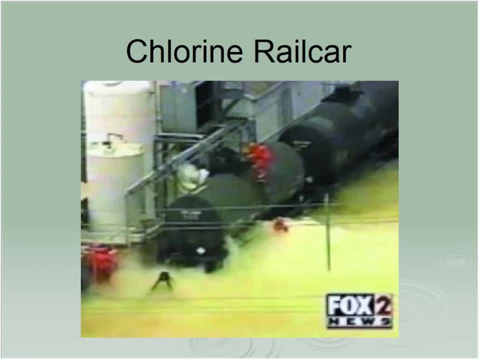 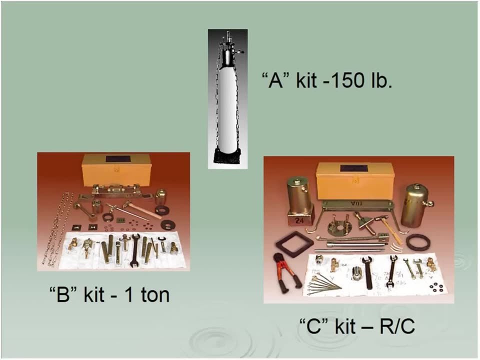 That is a bad day. That is a really bad day. There are kits for leaking valves. Typically, you're going to have a leak on the valve. American Chlorine Institute has devised these three kits for the different units. It's a very complex system. 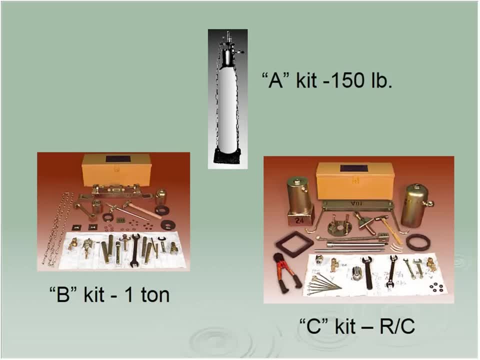 We've got the A kit for the 150-pound, the B kit for the 110, and the C kit for the rail cars. Hard to remember, isn't it? At Hampshire Chemical we'd bring in hydrogen cyanide cars of the exact same design as these rail cars. 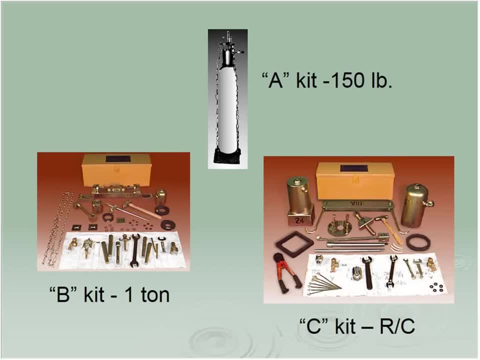 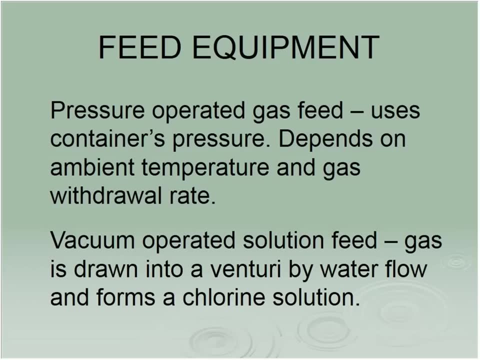 And we'd have to practice with these C kit units. A lot of fun. Two ways that we can feed. We can have a pressure system. We could have a vacuum system. The preferred method is the vacuum. If I have a pressure system and I have a leak, what's happening? 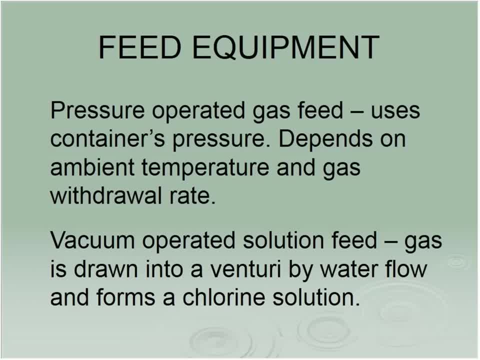 Chlorine gas is leaking out. right, It's under pressure. If I have a vacuum leak, what happens? I'm just going to suck it into my system. The worst I get is a bad bacterial sample. at the end of the day, 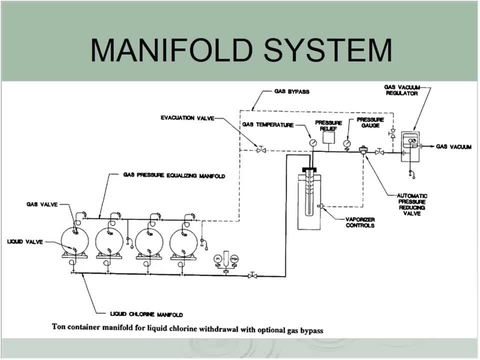 It's a lot safer. That's the important part. It's a one-ton cylinder. They're in a cradle, They're on scale so that you can see how much you're using. You can take liquid. If we take a liquid, we'll run it through an evaporator. 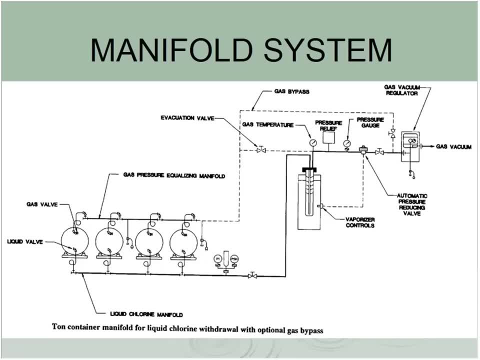 It evaporates quite readily. Just some warm water is all it takes there, Or I can take gas off the top of the cylinder and run it through Should there be a leak on one of these units. you never put water on the leak. 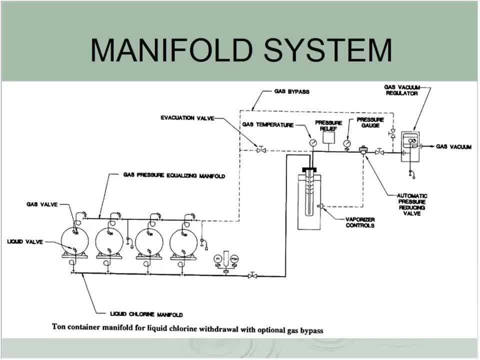 If you put water on the leak now, you're forming hydrochloric acid and a small leak is fast becoming a large leak. The reason that they're on rollers is if you have a leak on your liquid valve, you disconnect and you roll it so that it leaks gas. 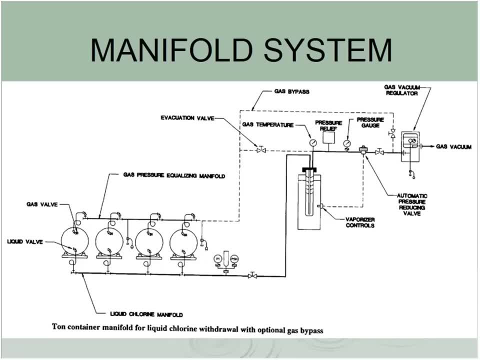 Any idea why. Just evaporates in the air. The liquid will spill to clean up and the gas just vanishes. That's not it, No, The liquid. when the liquid evaporates, it generates 479 times the volume, Whereas the gas comes out. it just is what the gas comes out. 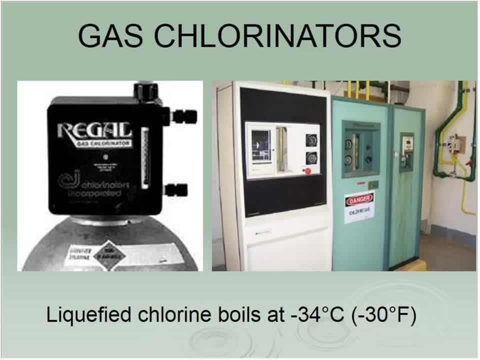 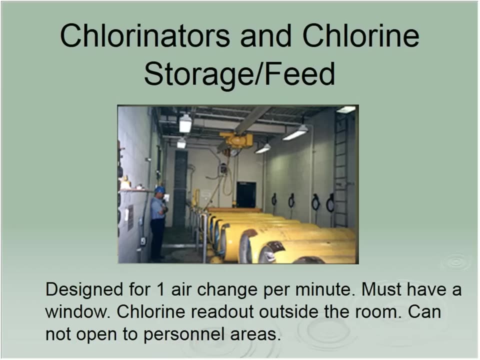 You don't want to fill up the room too fast. Gas chlorinators, Nothing to control it. It's basically just a little rotameter sitting on top of the 150-pounder. The one-ton units are much more complicated and stuff. 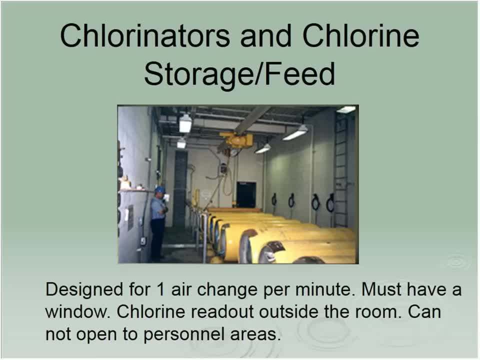 A chlorine feed room has to be completely isolated from any other employee area. You can't access it from the office, the warehouse, anyplace else. You come in from outside, you go outside, That's so. if there is a leak, it doesn't contaminate other areas. 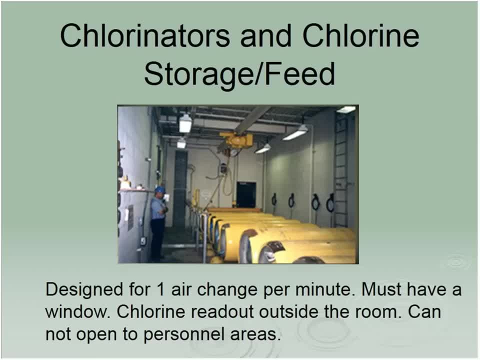 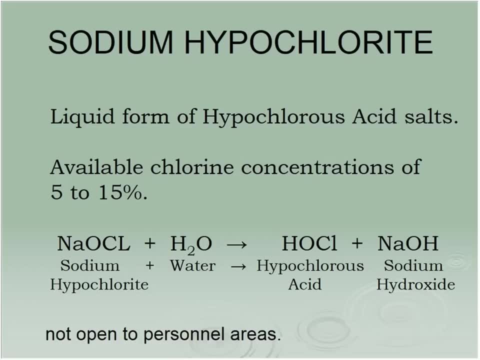 It leaks. It's two and a half times the density of the air, so it's going to leak on the floor. Ventilation will be at floor level to draw it away. Most people have abandoned liquefied chlorine gas in favor of sodium hypochlorite. 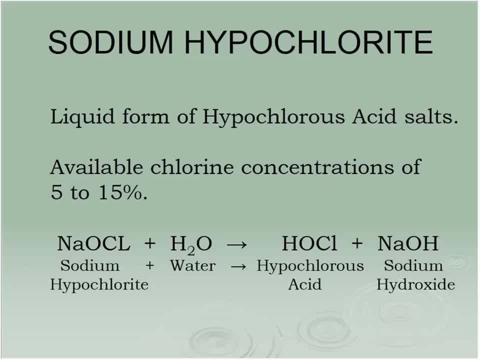 Sodium. hypo is just chlorine, bleached five times more concentrated. It's about 15% chlorine. Again, when you add it to the water you're going to form that hypochlorous acid, keeping in that same pH range, But you don't have any gas clouds going away. 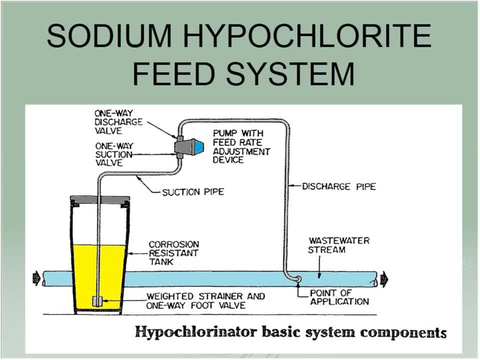 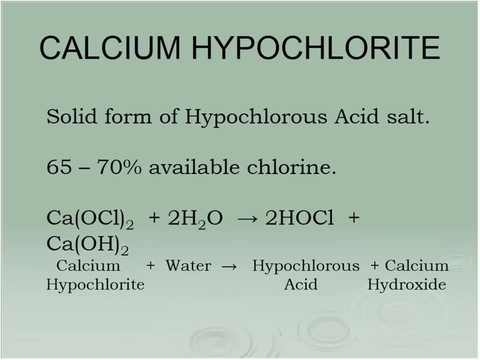 You just have tank trucks rolling over in your driveway or something like that. You've got a drum of material and a little metering pump. You can go and chlorinate anyplace you want. It works very well, easy to control. Now there are some systems. 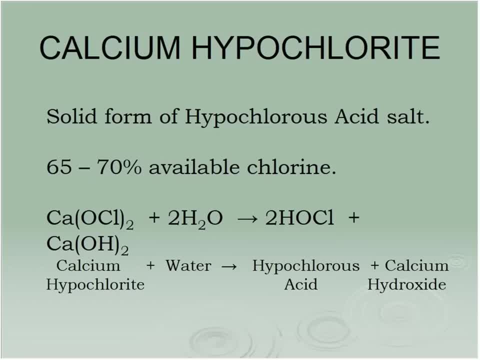 Very small systems. It might be an alternative system, or it might be a lagoon system that will use calcium hypochlorite. If you've ever had a pool and used HTH, that's what we're talking about: 70% chlorine in these tablets. 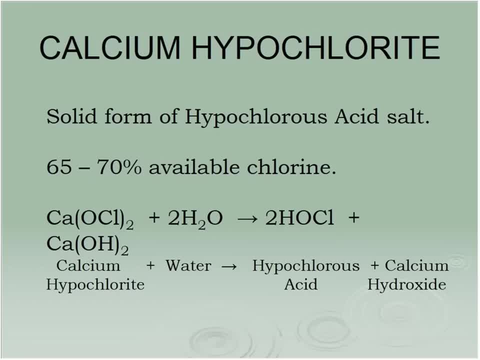 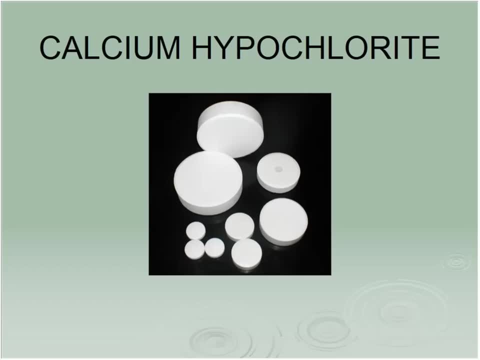 You've got to be very careful on how you store them. But again, once you add it to the water- hypochlorous acid- same deal. What you've got is these tablets inside of some unit, and then you just regulate how. 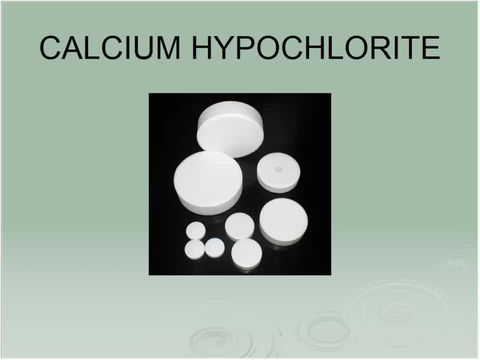 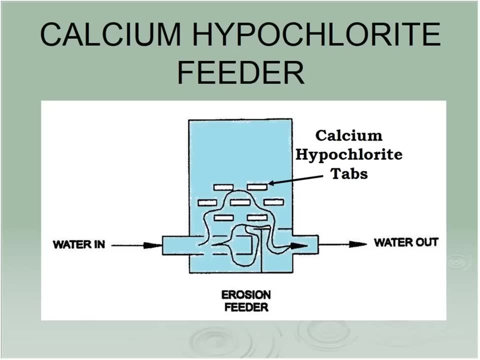 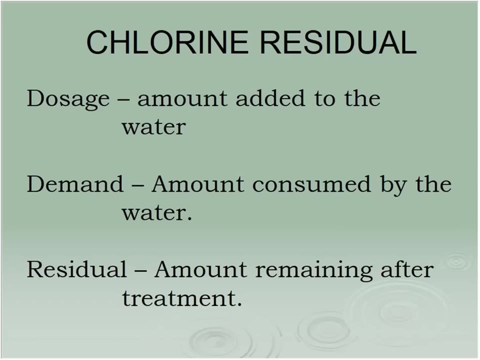 fast the water goes through and dissolves the tablets. Okay, That's very common with lagoon systems, where you don't have somebody hanging around all day long. So we have what's called a dosage. We're going to dose a certain amount of chlorine. 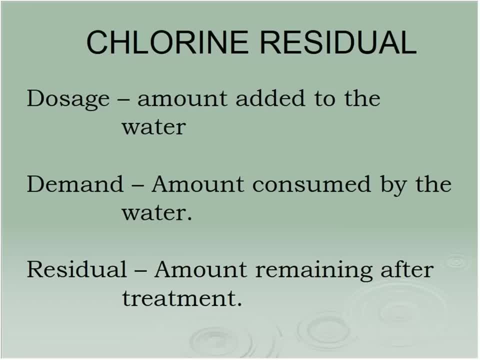 It's based on chlorate, generally in pounds, And what we do is we want to make sure we've got enough in there- Maybe we've got enough in there to get the kill that we're looking for- And we also want to have a safety factor that we call a residual. 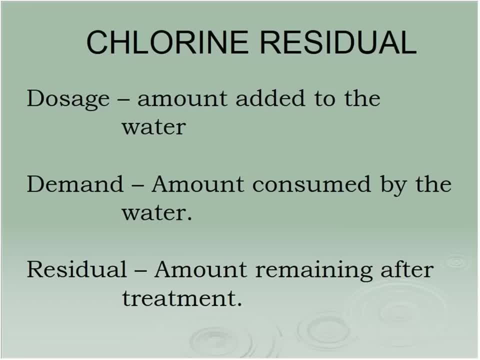 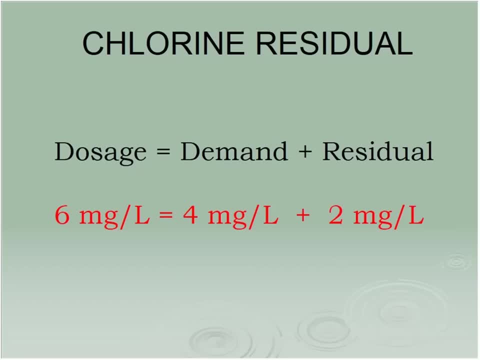 So our dose is our demand. We need to get the kill plus the residual. So if I need four to get the kill that I'm looking for, I'm going to have a residual of two as my safety factor in case things change as things go on. 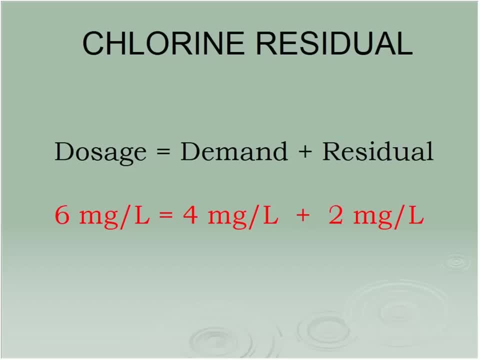 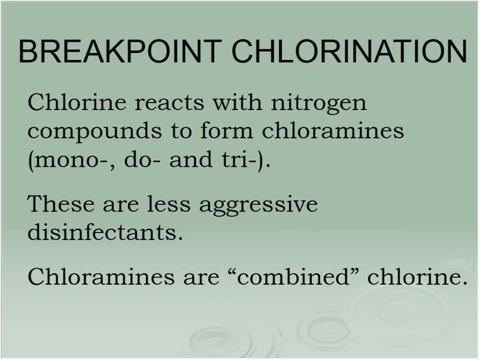 It may not be a lagoon system. I'm going to dose it six milligrams per liter. Very simple operation, Not hard. Here's one thing that may complicate it, though. It's what we call breakpoint chlorination. When treatment plants dose chlorine, they are generally looking for total chlorine residual. 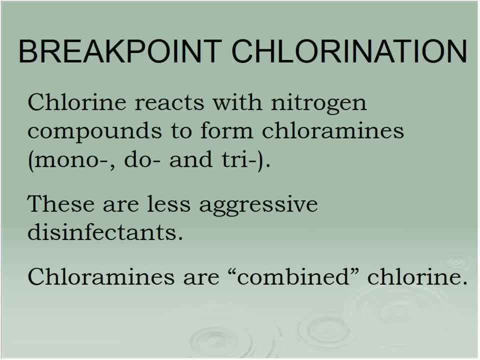 A drinking water plant in all probability will go for a free chlorine residual. It's a whole different thing, Because drinking water is generally dealing with pretty clean water, Nothing else around. We've got a lot of other different stuff, such as nitrogen compounds and various other. 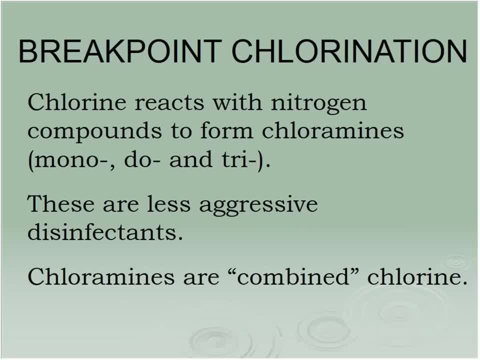 things that react with the chlorine. Chlorine is a very strong oxidizer, So if there's something around to react with, it'll do it, And if we have nitrogen compounds in there, they'll form chloramines, which will still. 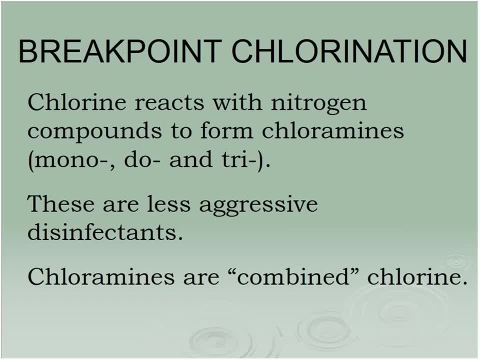 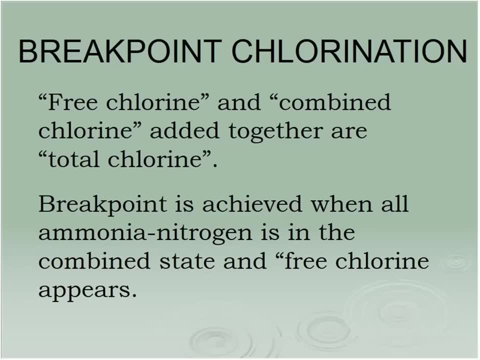 do some disinfection. It's not as effective. It's called combined chlorine, But this breakpoint idea is fixable. It takes a little while to kind of finally grasp the whole thing. It took me a couple years before I fully understood what the heck they were talking about. 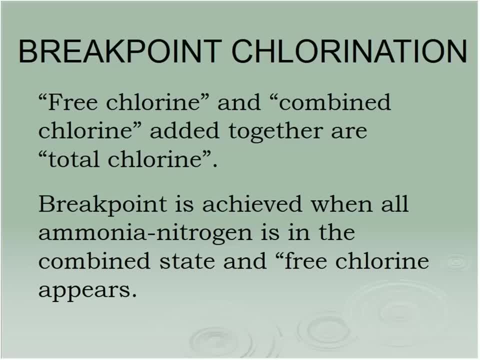 Okay, If you have free chlorine. that means I'm reading free chlorine. There's a chlorine ion floating around that water. It's a combined chlorine, which is a chloramine, ammonia and chlorine combined. Put them together and you've got total chlorine. 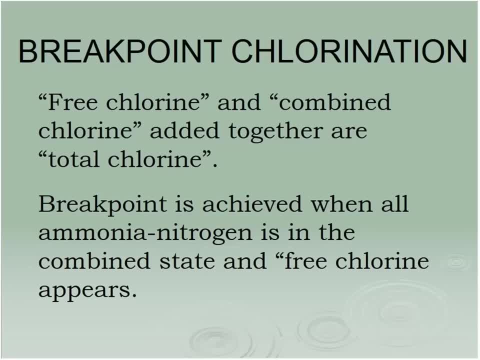 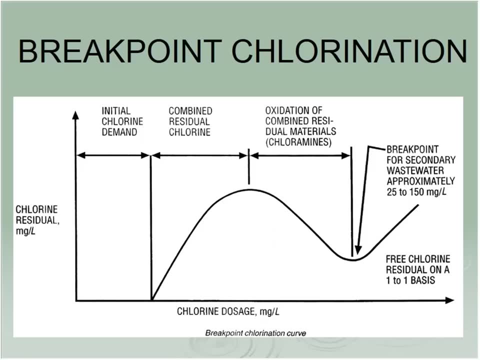 A breakpoint is when you've reacted every possible thing in there and for every little bit of chlorine you put in, you get that amount of free chlorine in your tank. So what's happening through here? I'm going to add chlorine. I've still got some bacteria in there. 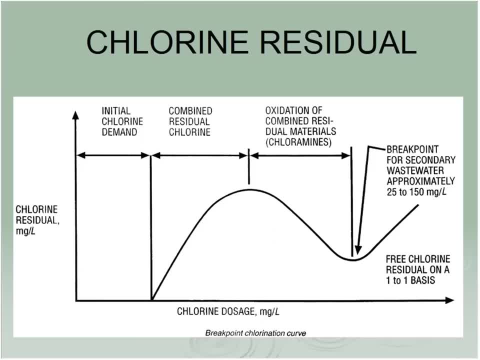 I haven't removed all of my solids. I've got some other components, maybe a little bit of metal or something like that. I put chlorine in and I see no chlorine at all. It's forming chlorides. It's breaking down other materials. 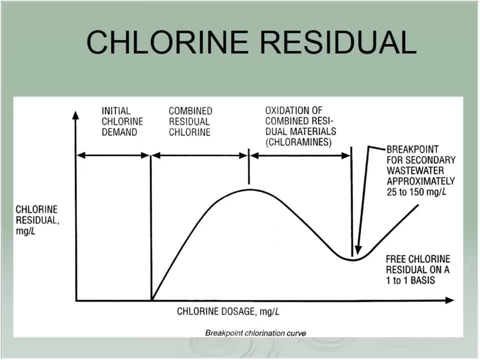 Once those are gone, I'm going to get some combined chlorine. It's going to start ammonia compounds forming chloramines which we're not going to get, any chloramines which would show up under a combined chlorine test. but I wouldn't have 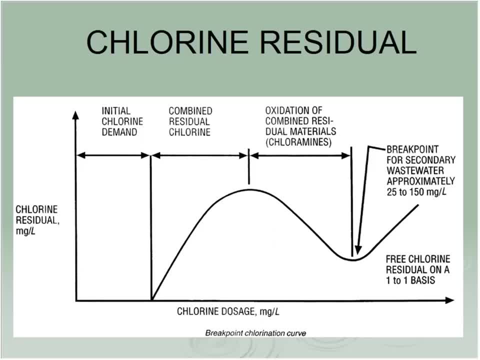 any free chlorine. I'm going to keep adding chlorine to the point where I now break down all of those chloramines And I get to a point called the breakpoint, where now, if I add one milligram per liter of chlorine, I get one milligram per liter of free chlorine in my test. 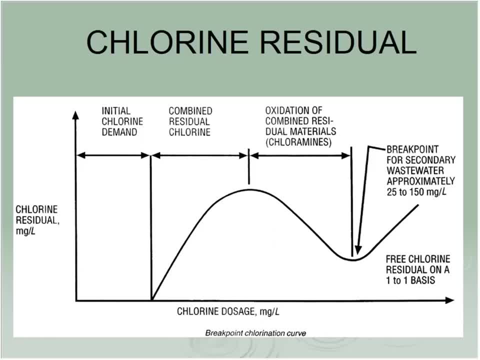 For drinking water. that's not hard For us out here. this is a huge amount of chlorine to get to a free chlorine, so we don't. We're going to put on a total chlorine Combined plus free. There's generally no free, so as long as we're getting the kill, we're good with that. 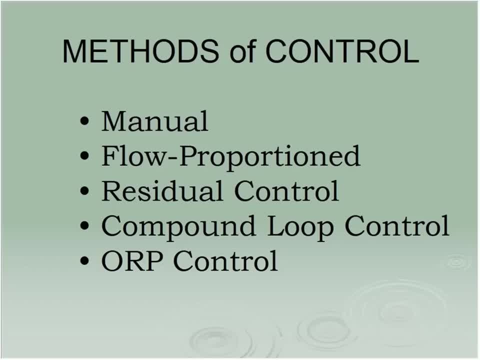 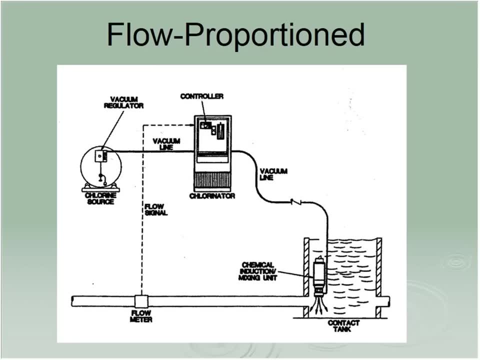 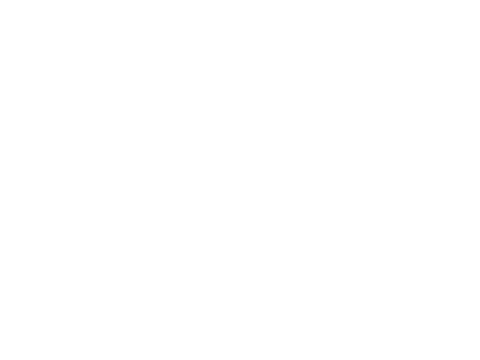 Control it manually: flow proportion, residual control, ORP- the various ways of controlling our dosages. Typically it's a flow proportion. We've got a flow meter that sends a signal to a controller that says: add this much chlorine. As the flow rate goes up, the chlorine goes up. 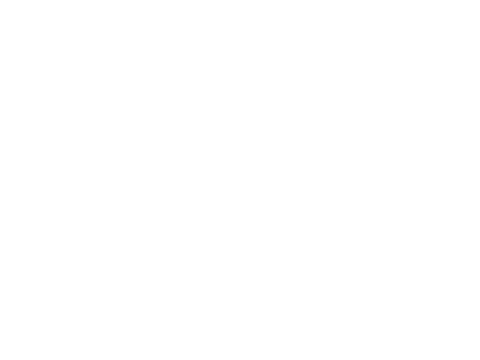 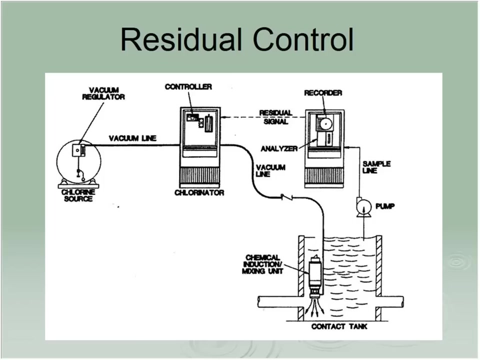 As the flow rate goes down, the chlorine goes down. Ideally everything works fine, But again things could happen. Maybe you get a little upset in your clarifier or something like that. Stuff could go by. Maybe you wouldn't have enough there. 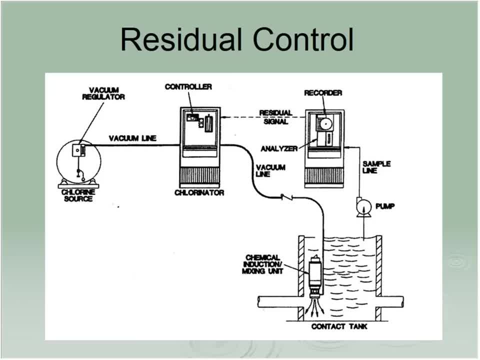 We do a residual chlorine. We're actually going to sample after our treatment with the chlorine- which is a 30-minute delay time- and say, okay, I want to have so much of a residual and that's going to tell us how much chlorine to add to the system. 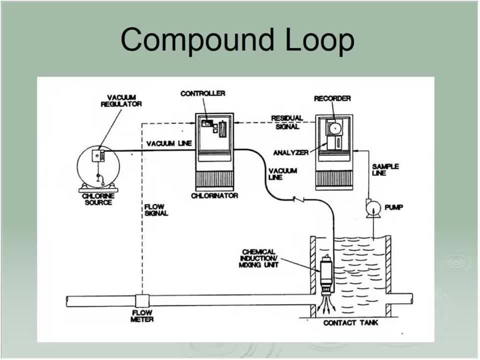 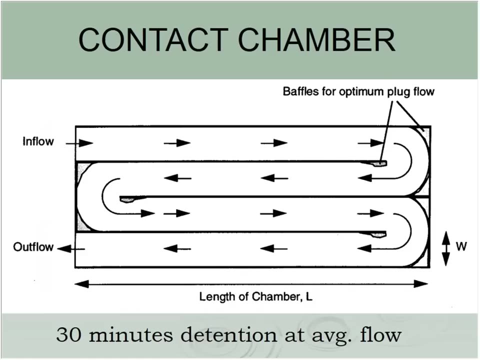 And then we get into more complicated instrumentation systems, systems, compound loops, where I've got going to feed based on a flow meter, plus I got a residual as a backup to override if I need to. and then there's cascade control, where controllers are talking to controllers. it's very complex, all to make sure you get the test that you're achieving. 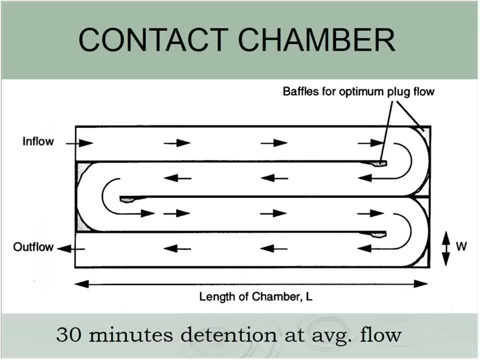 for chlorine disinfection work. ideally you've got three minutes detention time in your contact chamber and average flow. you need the time for it to be done. you need good mixing because all the organisms have to be exposed to the chlorine. good mixing and this is the prescribed design, the 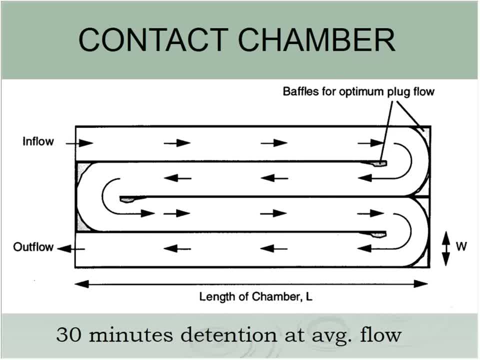 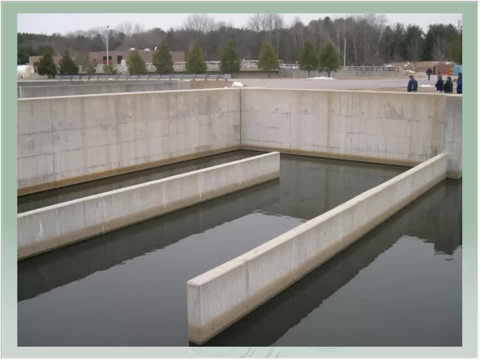 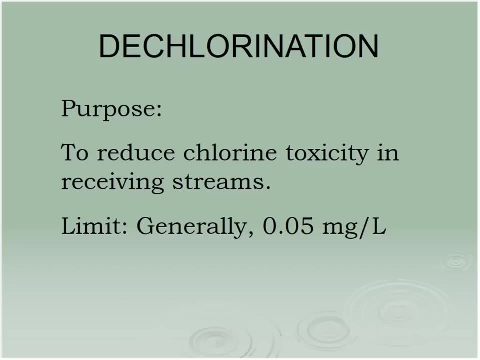 serpentine type of a tank. you find very few that look this nice, that's Nashua. not so nice deep, but not very nice. well, again, chlorine was cheap, so I'll say, okay, we'll disinfect. they just throw in chlorine like crazy. so they had this huge residual going to the river and the fish were turning white. so 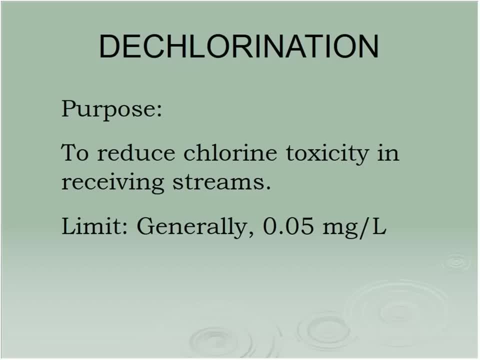 EPA said: oh, back off here, come on, you're going to have to dechlorinate. you can't have that much residual chlorine going into the waters, so now they limit, so we have to dechlorinate. you can have as much residual as you want be a safety factor, but you have to get rid of it before you. 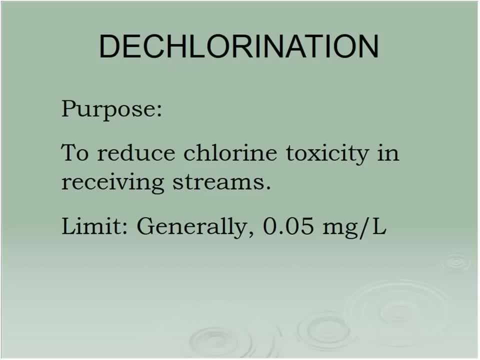 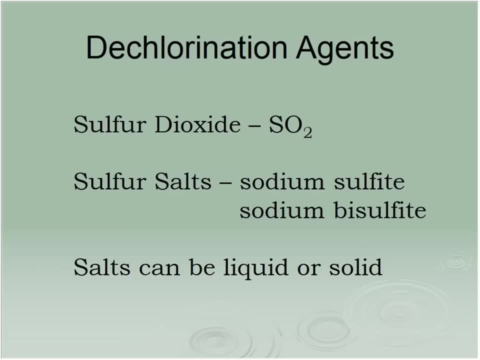 can discharge and they get pretty small numbers. I think the upper Blackstone's at 12 parts per billion. so originally, when licking gas was so popular, so was sulfur dioxide, a very nasty liquefied gas ugly- terrible. now I don't know anybody that's still using that. that's gone. 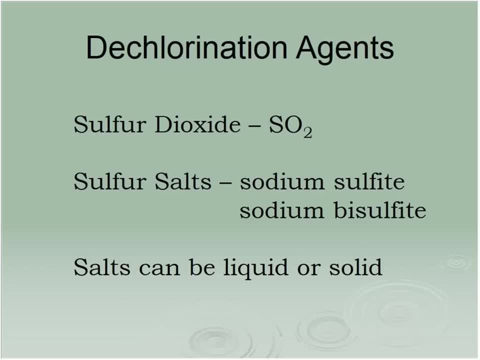 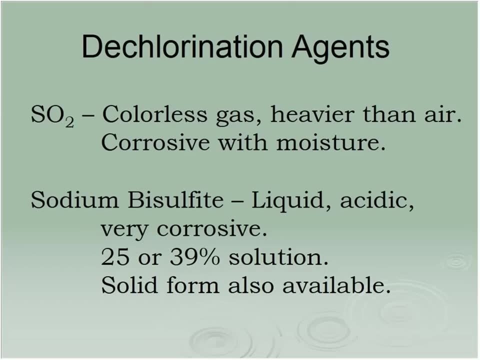 sulfur salt, sodium sulfide, sodium bisulfite, various solutions that you can buy. and so two: uh, colorless, heavier than air, very corrosive form, sulfuric acid. uh, the bisulfites work very well. the just another tank truck coming in a storage tank, but it is corrosive and you don't want. 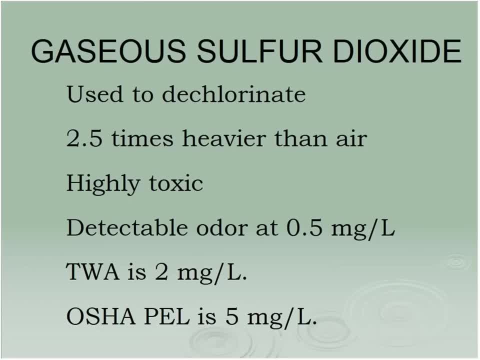 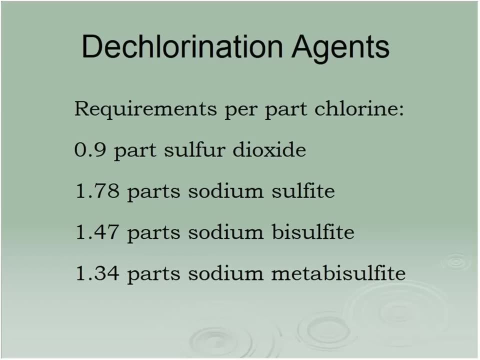 to bathe in it. They like this stuff because same vapor density, you can use the same regulator on your cylinders, very detectable. It's gone And it was also basically one pot for one. so if you had a two milligram per liter residual, you put in two milligrams per liter SO2, everybody. 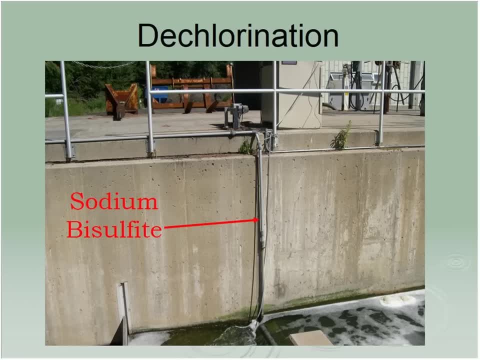 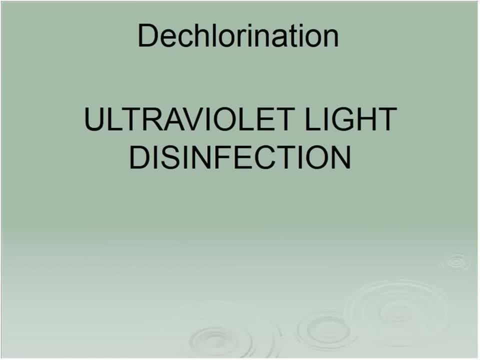 was happy. It's an instantaneous reaction. It forms a chloride. it's just a little salt now and nobody cares. Put it right at the end of your contact chamber. A lot of facilities said: we don't want to deal with chemicals. I don't want employee exposure, I don't want. 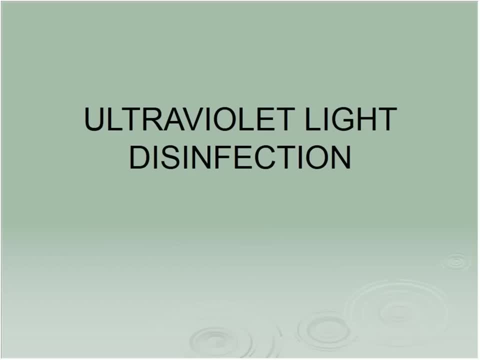 tank trucks. I don't want storage tanks and pumps and leaks and all of that stuff. I'm just going to write a check to National Grid and be done with it. So they've gone with ultraviolet rays Radiation. It's also very popular with small systems. What it is is light bulbs and water. 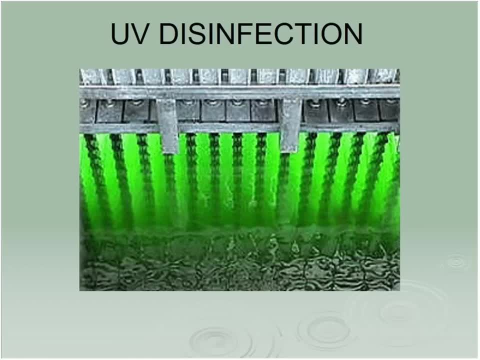 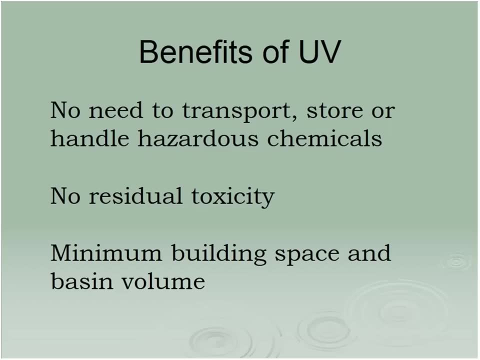 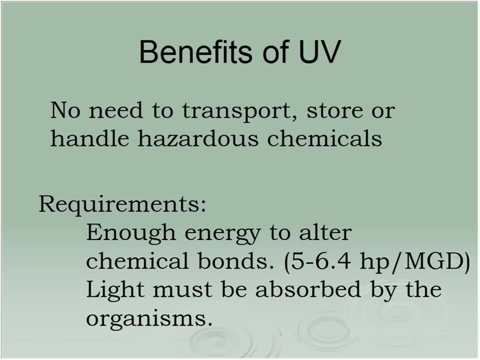 What's the worst that could happen? A lot of light bulbs, and water, as you can see, But again, no transport, no storage, no hazardous chemicals. there's no DUV, like there's D-chlor. There's some savings there, But here's the difference: Nobody dies. Nobody dies, Nobody. 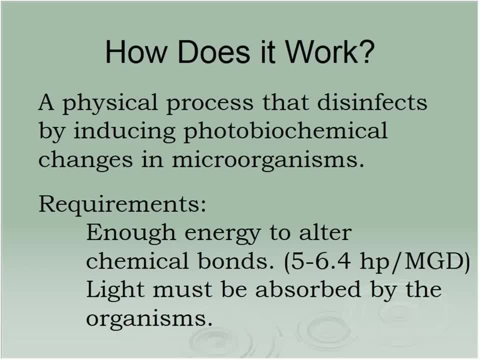 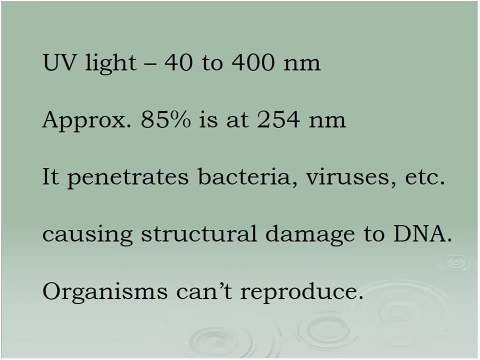 dies. Chlorine kills. UV doesn't kill anything. It's a physical process that inhibits the organism. You've got to have the right amount of energy to do it and the light has to be absorbed by the organism. That's why you see so many bulbs in that channel. We talked about UV. 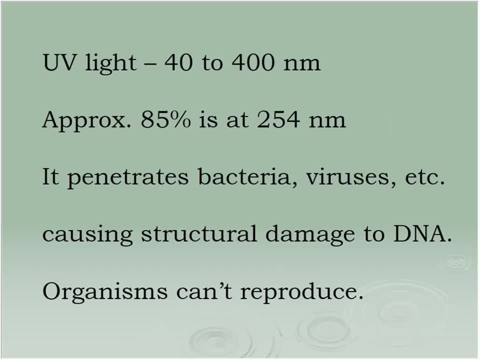 light. The range of ultraviolet light is 40 to 400 nanometers. The light that's effective for disinfection is about 254 nanometers, So the majority of the light is going to be the light emitted by these bulbs in that range And it messes up their DNA so that they can't. 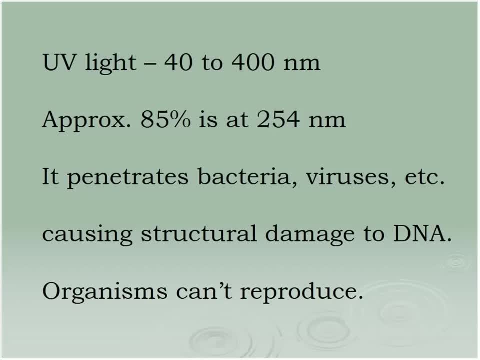 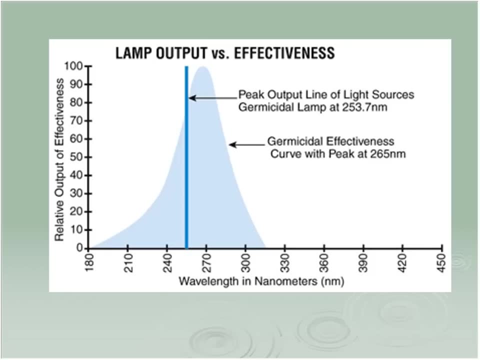 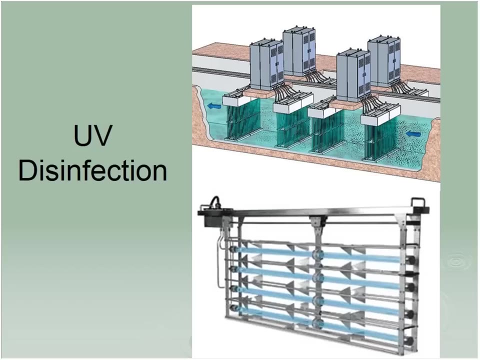 reproduce. They've got a lifespan of minutes, basically. So you throw them in the river. they die with no offspring, Nobody cares. But they don't die, Not from this anyway. The bulk of where the light comes out, 53.7.. And there's various types. There's types where 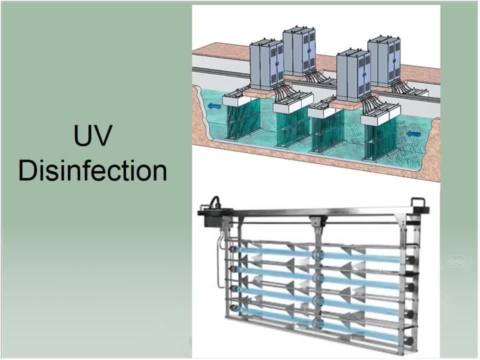 all the wiring is above the water, Some go down level, Some go down inside. The issue is again: the light has to hit the organism. So if you have turbid wastewater, you've got solids in there. that could be a problem. That's blocking the light A lot. 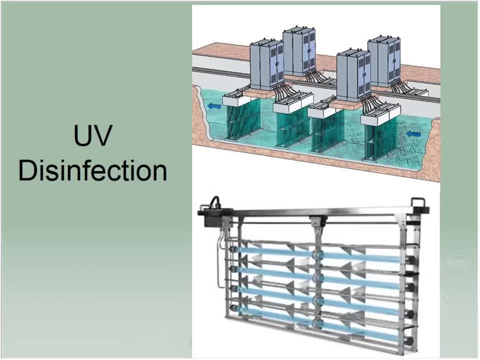 of them have wipes on them So the material collects. The bulb actually sits on a quartz sleeve for protection. The material can collect on that sleeve and block the light beam, so they'd have wipers that would go on it. A lot of trouble with the early versions. They were snapping the bulbs, which is not 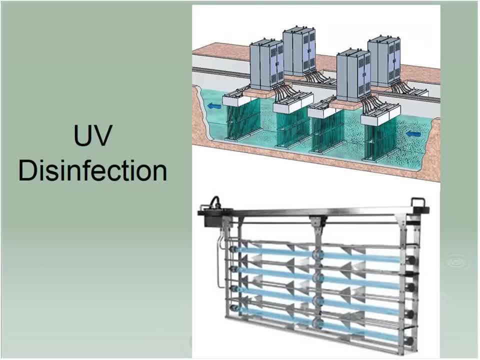 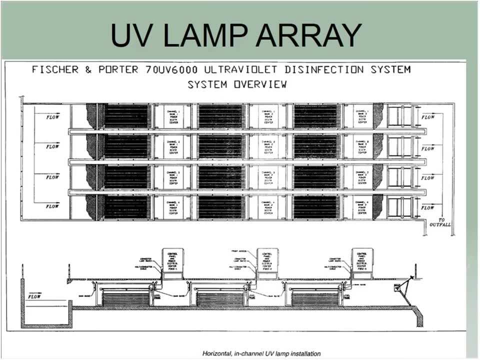 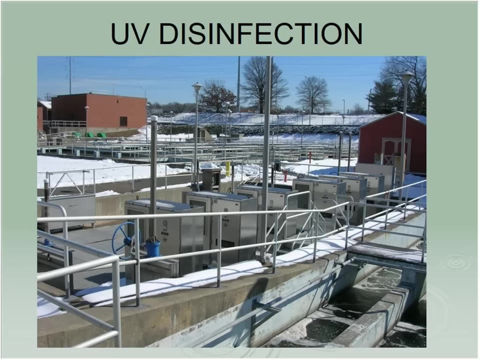 good because they contain mercury. You need a lot of them So if you have turbidity issues, it could be an issue. Lots and lots of lights. These are fairly old units down in Wallingford, Connecticut. Each one of these boxes indicates a set of lamps down inside that channel, Concerned. 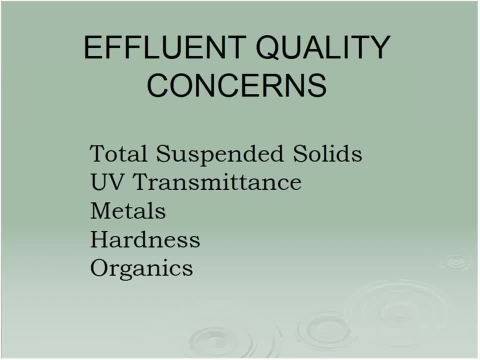 with high suspended solids You've got to make sure your bulbs are transmitting properly. Metals can be a problem: Hardness collecting on the sleeves in organics If. Do you go to fast food restaurants anymore? Inside, Look around, See if you can find the blue light on the wall. 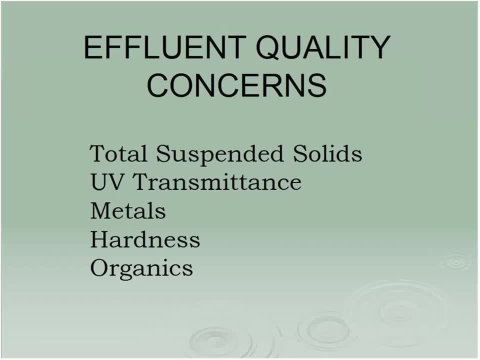 I get a kick out of this. I've seen it in restaurants. I've actually seen it down in Lahey Clinic Light up on the wall. It's an ultraviolet light Supposedly to disinfect. You know it's disinfecting About four square feet of wall where it's shining because you can't see it. 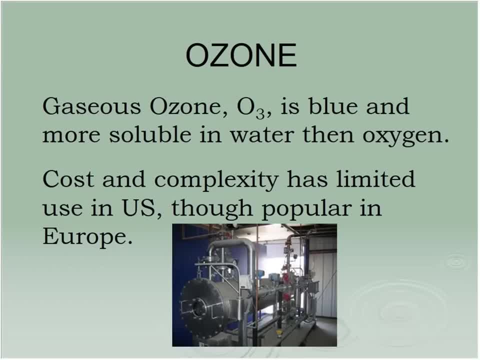 in the rest of the room Ozone. Ozone is an extremely strong oxidizing agent, Very strong. It has to be done on site. It's very complex and difficult to deal with. Okay, In the case here, Europe, they do all sorts of crazy things over there. They've been pretty. 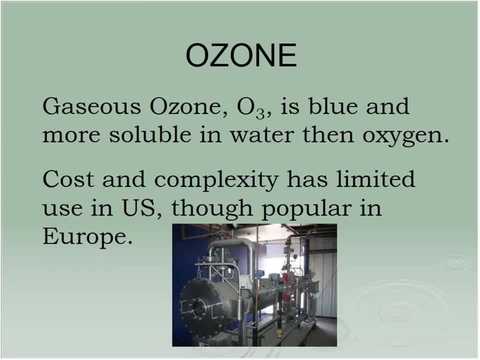 good with it And I'm starting to see some inroads here in the United States where we use an ozone as a disinfecting agent, But it's not a popular thing. We tried it at Hampshire for a while on a different process. It's more trouble than it's worth. 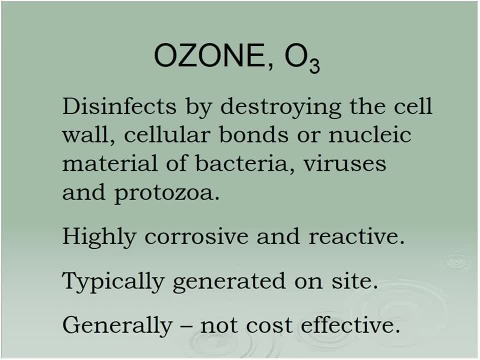 Alley corrosive reactive. There's actually, and to talk about chemical pretreatment, there's a. There's a T-shirt manufacturer up in Keene, New Hampshire, Three Dog Moon. I don't know if you've ever heard of those guys And they were giving the Keene treatment plant fits. 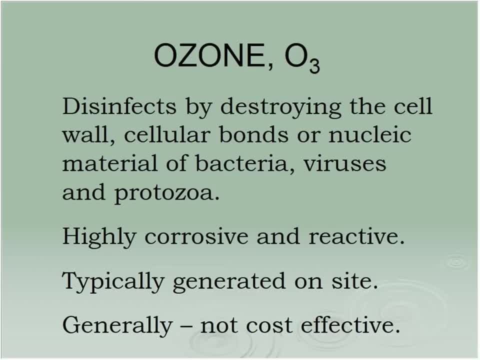 Because when they did the red and the blue dyes for their shirts, color would travel right through to the plant and drive them nuts. So they actually installed an ozone system to knock that color down. Chlorine wasn't working, so they had to go to ozone. 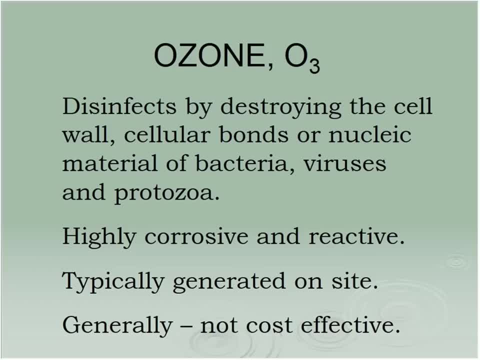 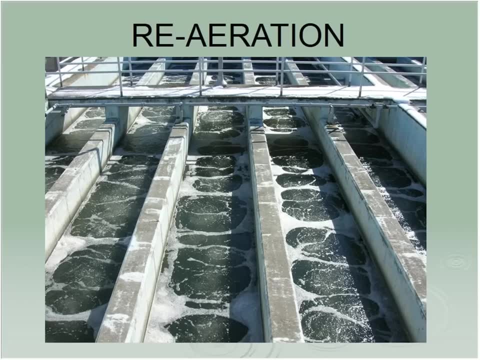 Very expensive system, but it's keeping them out of trouble with the treatment plant. So So BOD's down, Suspended solids down. Maybe our nutrients are down where they should be. We've got nice clean water. We've killed off the pathogens. 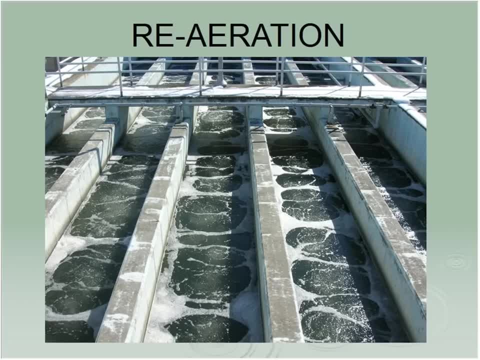 Everybody to a point where we may have to One final thing to do before we let this go. The last time this water saw any air was back in our biological process. We have to pump a lot of air in there to keep the bugs out. 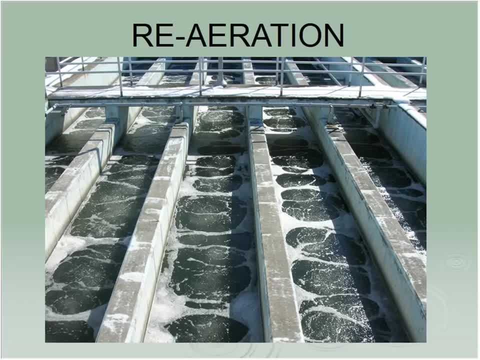 So we went through a clarifier, which is probably two to three hours. We went through a contact tank, which is half an hour, So there's still a little bit of food, a little bit of bugs and no oxygen. So what we have to do is reaerate. 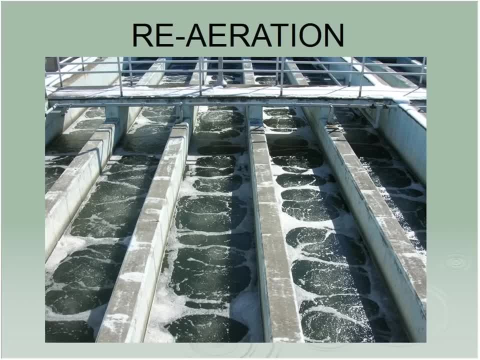 Because now this is going into the stream and all this is part of is going down to what we refer to as the assimilative capacity of the river. Our water is now going to go into this receiving stream and we want it to disappear in that. 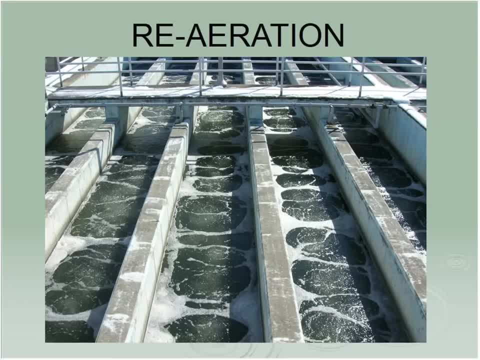 stream as quickly as possible. We don't want you to go and sample a mile downstream and say, oh geez, The DO is down to probably three because the treatment plant's got no oxygen in their water when they throw it in. 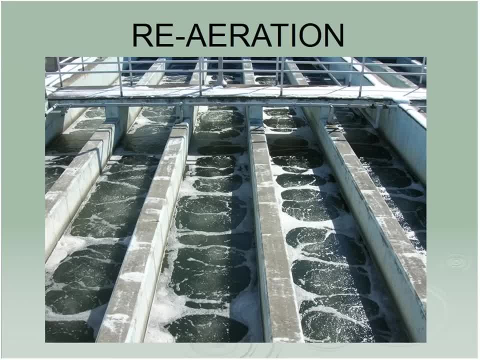 We want it to go away. So permits invariably will say that you must have a dissolved oxygen content in your effluent of a minimum of six milligrams per liter. We've got to get that in there, And again it depends on how things go. 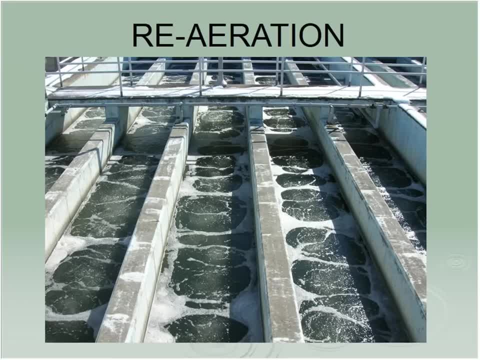 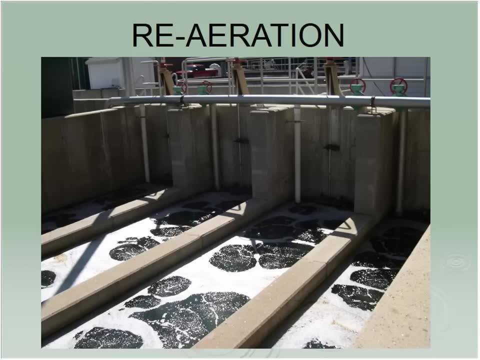 This is Wallingford, Connecticut. They actually have to pump aerate based on the way their system works, So these aerate it Just like we would a water pump. It would have made me in our grid chamber, Bill Ricker, the same deal. 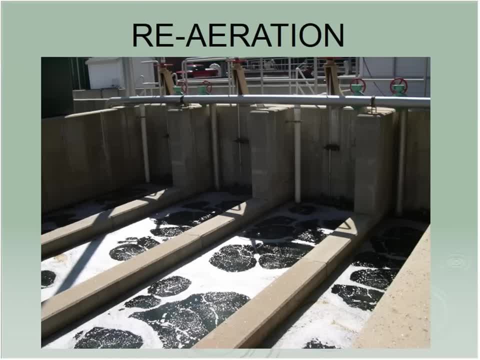 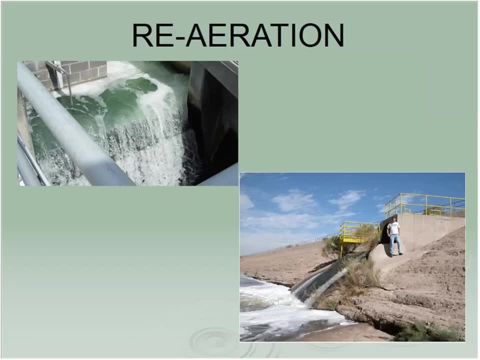 This is the way it works. They have to pump air in to get that dissolved oxygen. up Upper Blackstone is very fortunate, and their water all flows downhill. When it comes out of their contact chamber, it goes over a weir similar to this and: 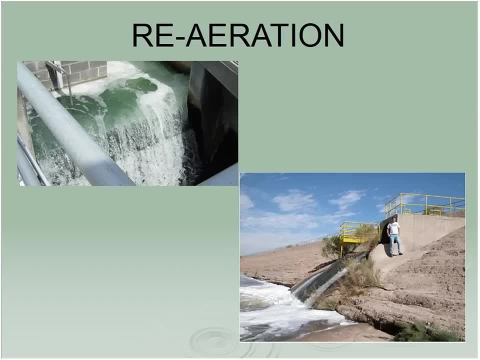 then drops about eight feet, You've got six and a heartbeat. by doing that Some other places. You go to Brockton. It cascades, somewhat similar to this, down a series of steps. All that, just that little bit of activity is enough to get that oxygen for free. 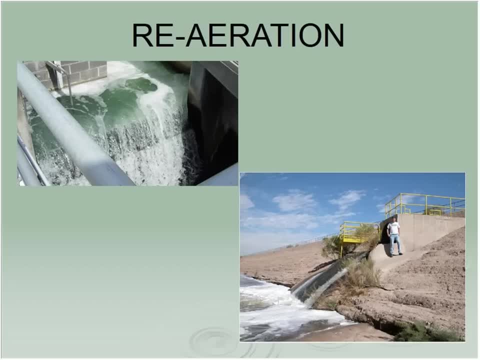 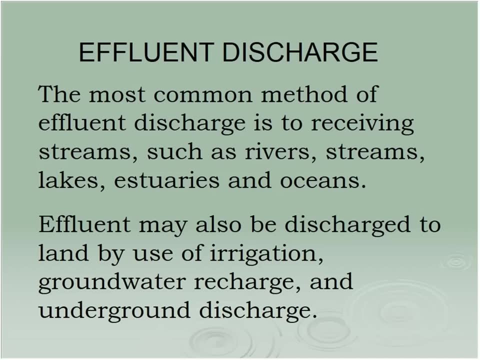 So now, when it goes in, it doesn't kill off the oxygen in the stream, It just kind of blends right in and hopefully you never see anything. This is something that we may see one of these days, particularly out west, where a lot of 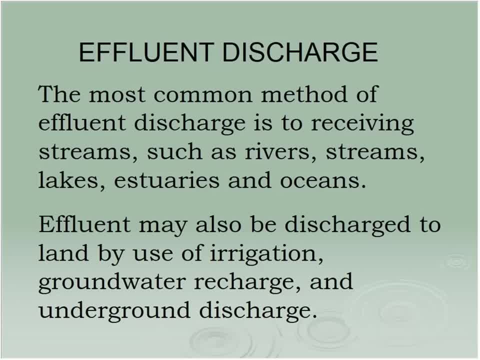 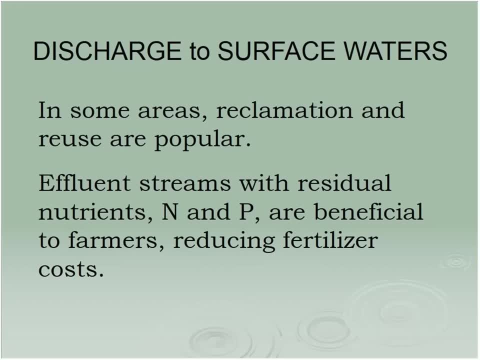 this water could be used for irrigation. Stop taking the nitrogen and phosphorus out. We like that stuff, Wouldn't that be nice? Blah, blah, blah. Where's my thing? The receiving stream. Yeah, They test your waters upstream and downstream to see what the effect of your wastewater 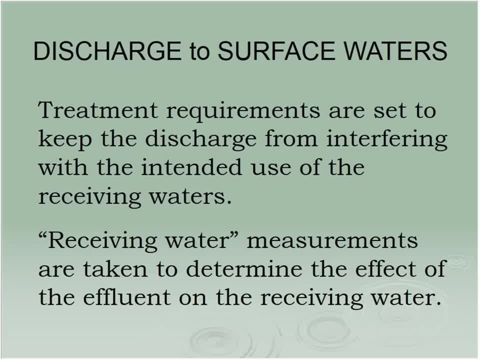 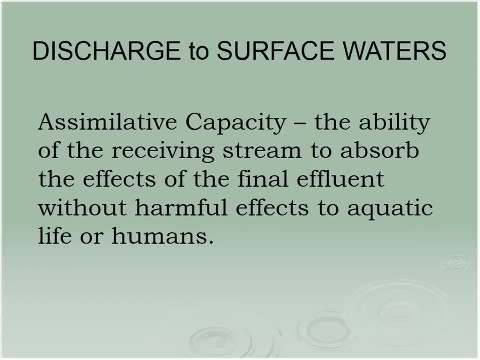 is on the receiving stream. how fast it blends in. It's that assimilative capacity? How fast does your material disappear? Temperature-wise, dissolved oxygen pH. Our discharge went into the Merrimack River. We had a pipe that extended out to the midpoint of the river. 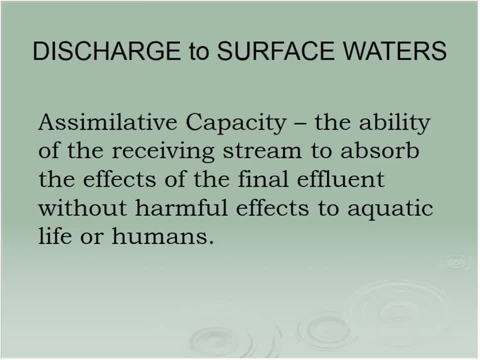 It had 14.9.. It had 14 nozzles to help blend that stuff out. They call it mixing zones. What you got to do to mix that into the river as quickly as possible so that there's no actual detriment to the whole thing. 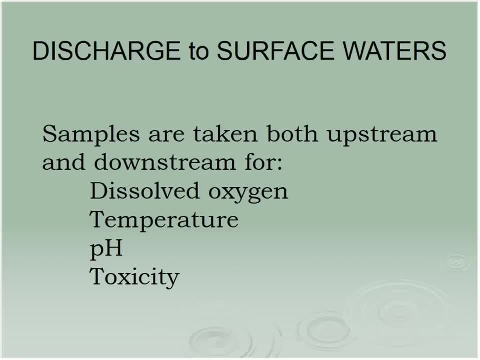 The other thing that occurs is what they call whole effluent toxicity test. Are you familiar with that? It's a strange thing. We would do it quarterly, and what we would do is we would take water from upstream, from the river, and when we take our water we'd send it off to a lab and they would 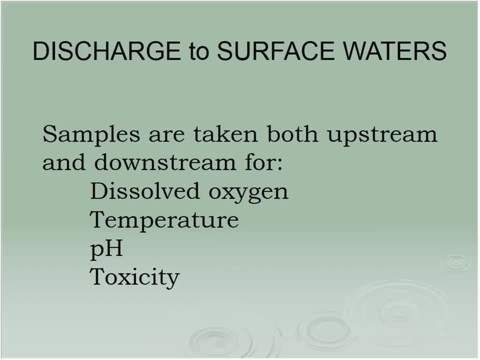 test it. What they'd do is they'd keep making increasing concentrations of our wastewater into the river water and they would test for seriodaphnia, which is water flea and fathead minnows, and they'd go until our wastewater would kill 50% of them. 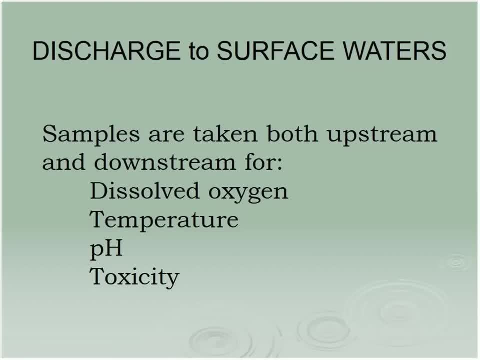 It's a fun job, huh? Oh my God, I'm counting fathead minnows And the question always is: what do you do? And the question always is- in fact, somebody asked me this in my classes last fall- is: 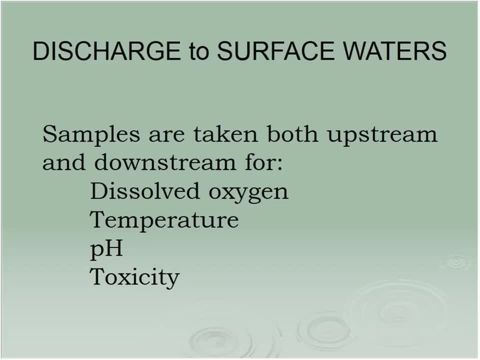 what happens when you fail. I have no idea, But the test is so accurate that it could take more than 100%. That's another thing that they test for. What is your effect on the river streams? All of those, And that, I believe, must be that. 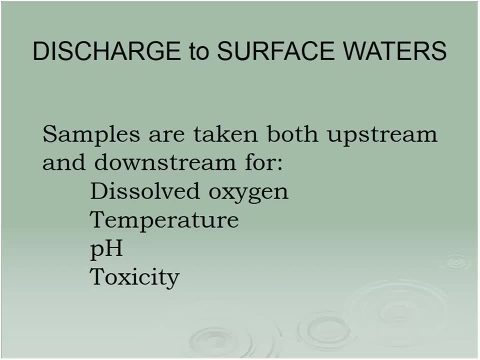 All right, Any questions? I did get a question. Oh, Excuse me, It's pretty specific to do you have any experience, Jim, with paracetic acid? No, I don't, and I've only recently heard of that. 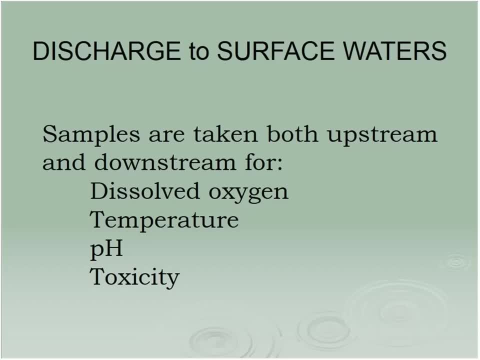 Apparently there is some work being done in that area. paracetic acid for disinfection, But I have none myself Any questions. A new concept. Folks in the room, other folks on the line? feel free to use the chat. 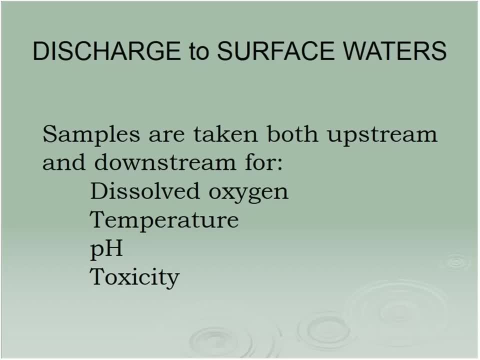 Thanks, Dan, for answering my question. I know this is going to vary. The answer to this question is going to vary a lot depending on the plant, But I'm just trying to grasp the concept of how long it takes for water to get from. 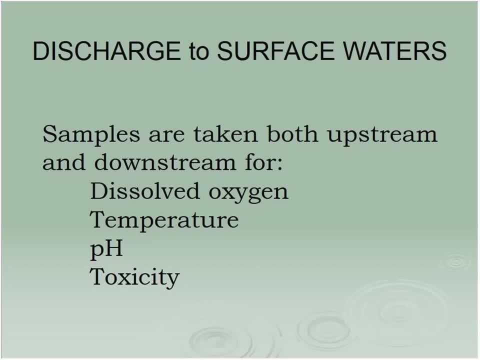 the beginning of the plant to the end. Is it hours, minutes, days, Eight to 12 hours generally? Oh okay, Those go pretty fast And the bugs are extremely quick in what they do. Do treatment plants run 24 hours. 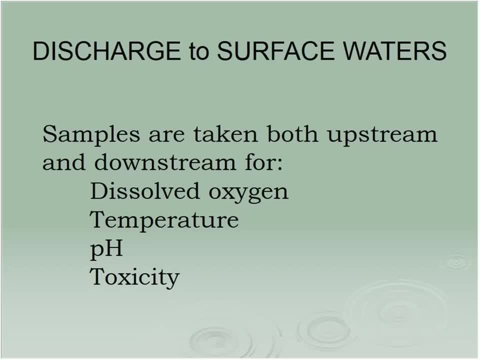 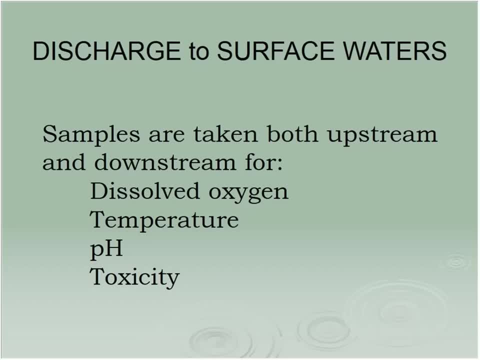 They can't get people to stop flushing at 8 pm and hold up until tomorrow morning. Again, that's one of the challenges. Whatever is going badly in your plant, you can't stop the water. It's just going to keep on coming, no matter what's going on. 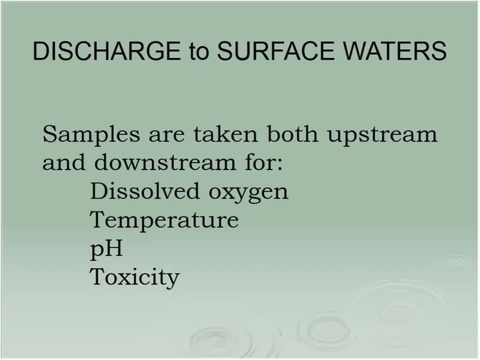 When you're looking at treatment plants. in order to facilitate that operation, no matter what happens, all the lights go out every place else. there's going to be generators in two locations of the plant. You're going to have a generator at your head, where it's. 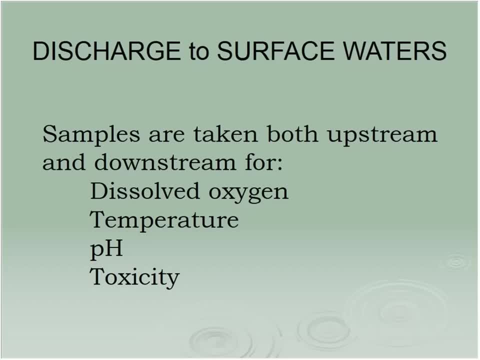 built Because, no matter what happens, if you can't keep those screens clean, then it's coming out the doors and windows and running all over the place. And the second one is down at disinfection. No matter what happens to your plant, you're going to disinfect that. 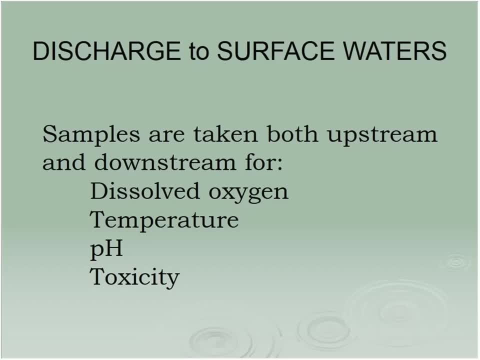 water before it goes, because it's going to keep coming. It doesn't matter if the power's out in everybody's house, because the drinking water plant is in all probability still running. I don't mind that. I've got water. if nothing else, If that water keeps coming, they've got. 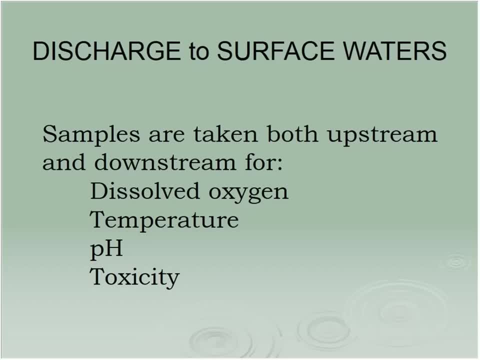 to disinfect it before it goes out. So that's a regulation, that's in the books that they have to have. I might just run around like crazy trying to straighten that out. So those are the only contingency plans in terms of any kind of scale, just basically. 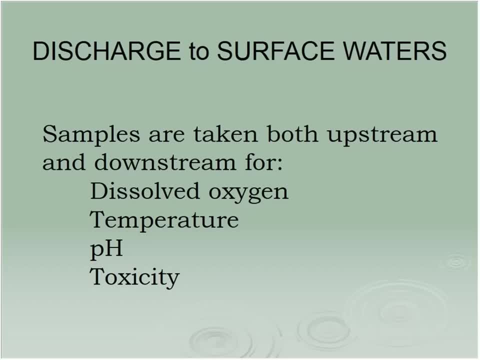 keeping things running as opposed to any other kind of alternative system, you know, because you can't shut down. Well, when you say, like if things are going badly, there's got to be some measures that you can take while things are going badly, you know. 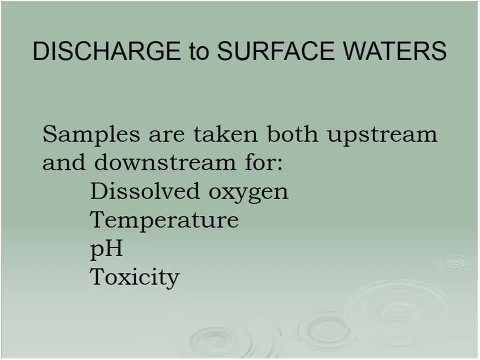 You have multiple units. It's not just one pump running everything. You have other ones you can switch to and do what you've got to do to get by Again for the most part. once you bring that water up to ground level, it generally tends to run on gravity, the water. 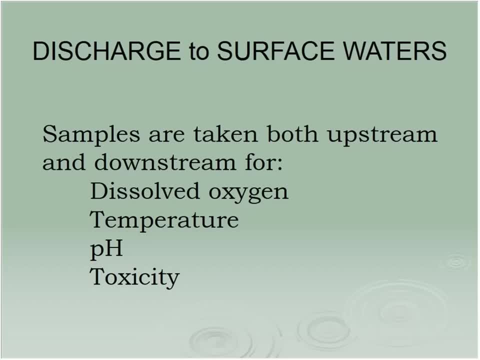 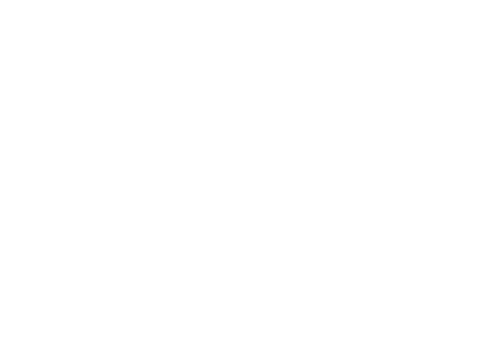 side of things. Anyway, one of the reasons that we need to keep, you know, the I&I down to a minimum is because, again, we talked about big tanks full of bugs, that if your flow is too high that goes, And that's one of the things that is a common operation If you get you know. 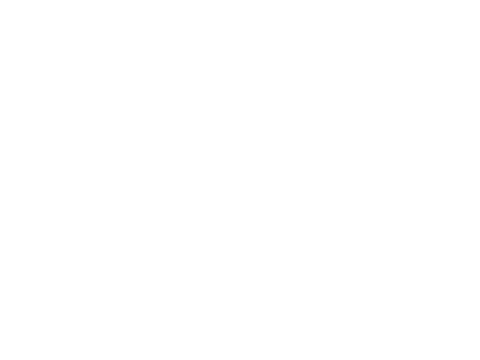 that three inches of rain in an afternoon type of a depot. it's amazing how that flow changes up when you consider the area that you're covering. You can just kill your aeration, let your bugs go sit on the floor And let the water just pass on through, as long as you're disinfecting. at the end You. 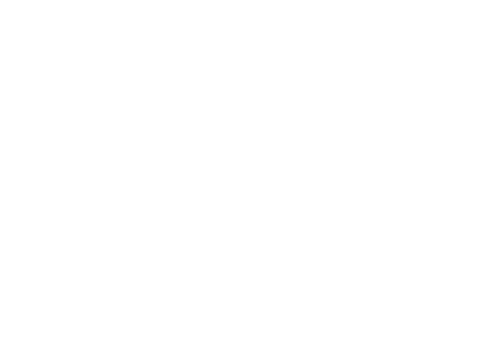 can actually bypass under certain conditions- And bypass is the naughty word in this business- But under certain conditions. you've got to save your plant Because you know, if all your bugs are on the way to Narragansett Bay, then what are you going to do tomorrow? So 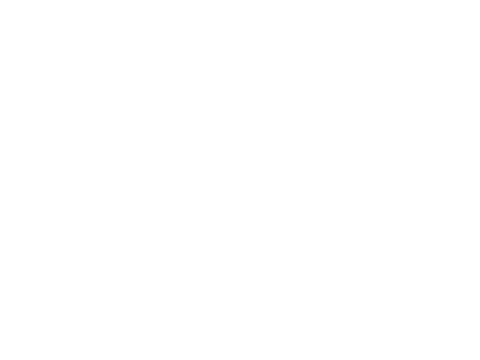 things like that, But it can be a challenge sometimes. My particular operation was strange in that, you know, I didn't have multiple units, I had one clarifier And when that broke down once, we all went into a panic because we didn't know what the heck we were. 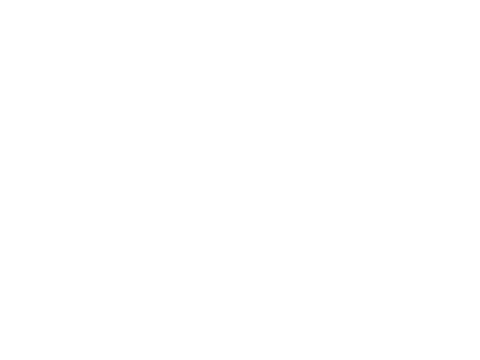 going to do So. it varies from plant to plant. What happens when maybe somebody discharges something that kills all the bugs, or something like that? How do they replenish that supply of bacteria? Again, you like the situation up in Plymouth and some others. you have multiple trains. 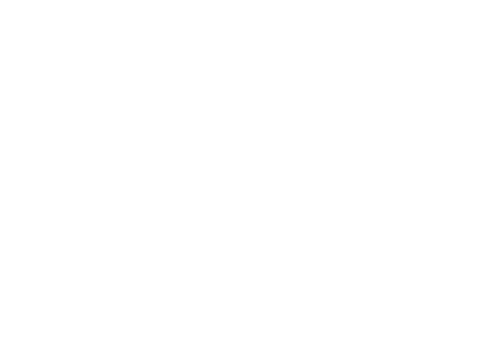 Okay, So, depending on how bad it is, maybe you just wiped out one train and you can bring the other one back. online. Worst comes to worst, you're going to have multiple trains. So, depending on how bad it is, maybe you just wiped out one train and you can bring the other one back. 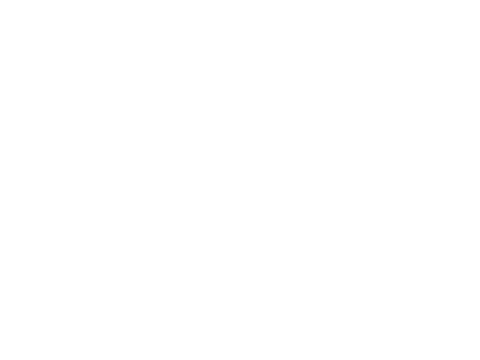 online. So, depending on how bad it is, maybe you just wiped out one train and you can bring the other one back online. So, depending on how bad it is, maybe you just wiped out one train and you can bring the other one back online. 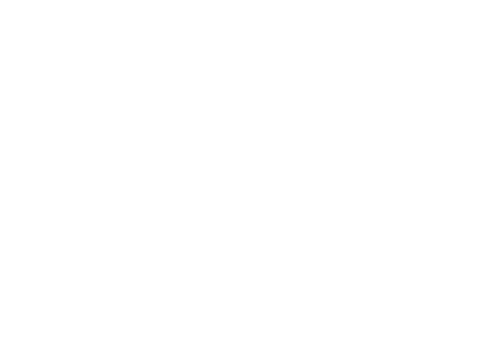 And some of the things I learned is: you have to bring in sludge from somebody down the road and reseed the whole system. You still are going to be in violation, probably for a week or so, before you get things back to normal, And that's why it's very critical to have that pretreatment operation to do it. 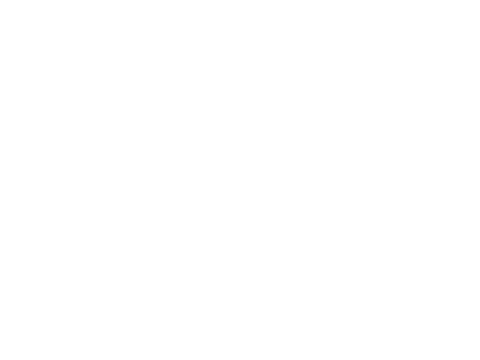 And that's the thing. Generally things don't happen that quick. you know, Somebody nukes your plant like that. you know they just dumped a whole ton of cadmium into you. Nothing you can do. Most things change very slowly. 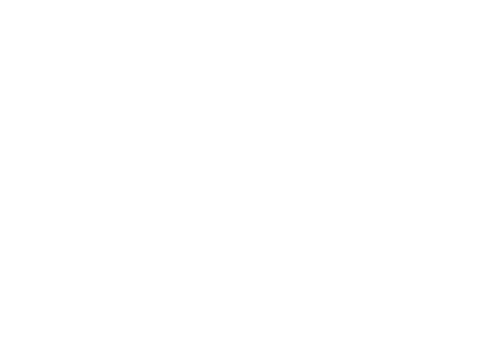 slowly and that's where process monitoring and the process control is really important. The microscope exams: I guess we're going to be doing it again for the commission. We'll have little bugs out there. To me that's a very critical thing because these systems change very slowly and again. 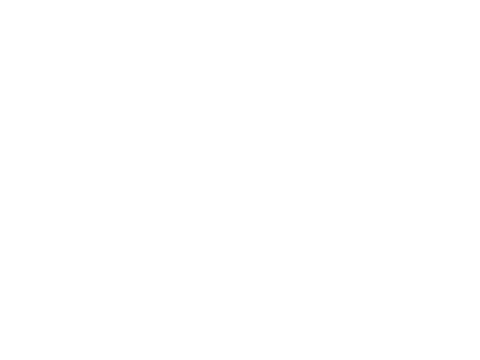 you're relying on five-day data, like BOD's, five days old, so you've got to monitor and see what's going on. It's very crucial. I'll be honest, I've not run a municipal plant, but to me it does seem kind of boring to some. 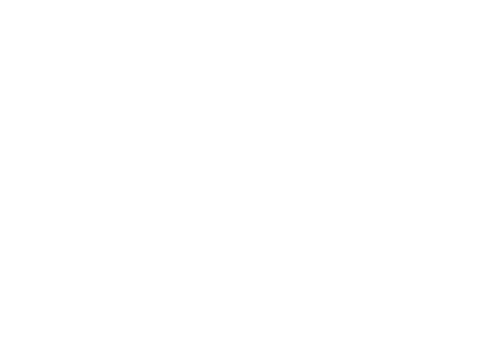 degree. My place was just all over the place because it was an industrial situation with different things. These things are very consistent in what their influence is like. It doesn't change a whole lot unless somebody messes up it, whatever. but 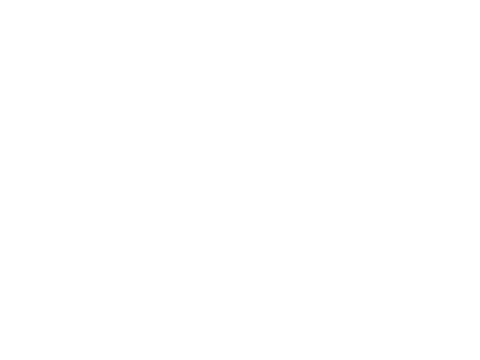 I have a question about the coordination. Why would you, Do you know the demand before you try to keep that as low as possible? On the chlorine demand, Yeah, You set up with. You kind of know how things go Again. things at that end shouldn't be varying a whole heck of a lot and you're going to 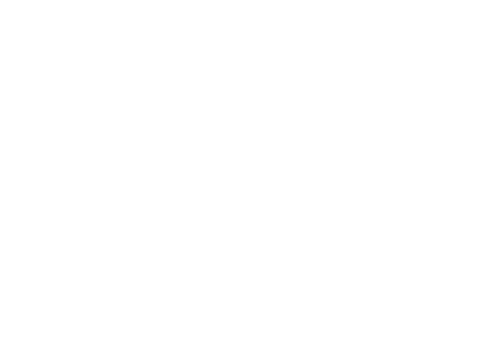 know. anyways, You're going to take a look at your clarifiers, You're going to take a look at your raffle window and interpret it as all get-up. so you know you're going to be losing a lot of stuff. 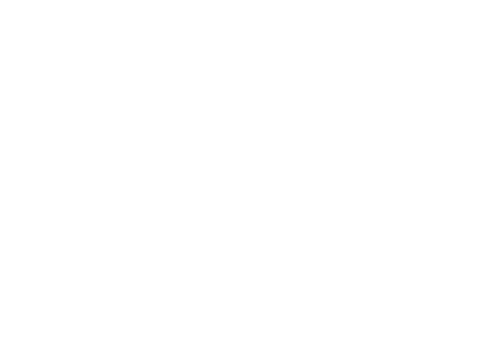 When we talk about nutrient removal on the last day. that's one of the places where plants kind of get caught with their pants down, because if you don't want to nitrify, if you don't have to do nutrient removal, you kind of slip into it by accident your chlorine. 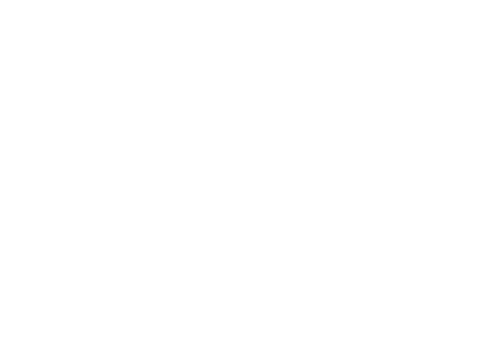 demand is going to go crazy. You're going to get caught by the eight ball. I actually got a call from Lowell Drinking Water one day. They wanted to know what the heck we were doing because he was using chlorine. I said I don't know. 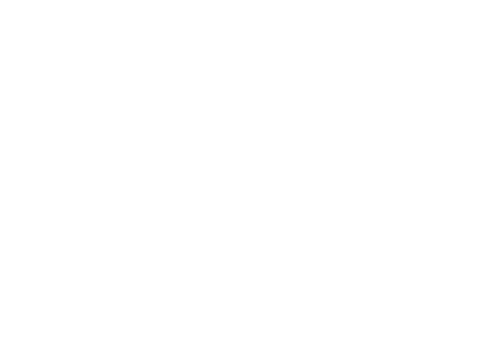 What the heck we were doing. because he was using chlorine like it was going out of style. He was accusing us of dumping excessive ammonia into the river. I'll tell you the amount of ammonia we were allowed to put in in those days, compared to: 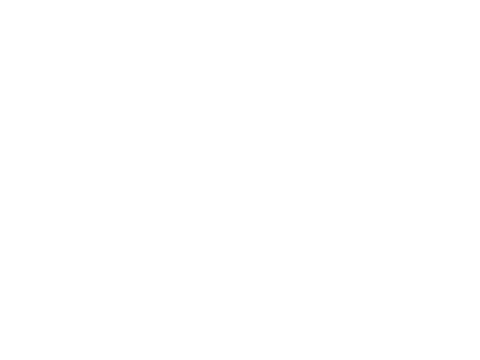 what you can do now is astronomical. We had nothing wrong with that. He apparently had a lot of ammonia compound coming in from someplace and it just eats up that chlorine like crazy. and again when they're trying to go for a free chlorine residual. 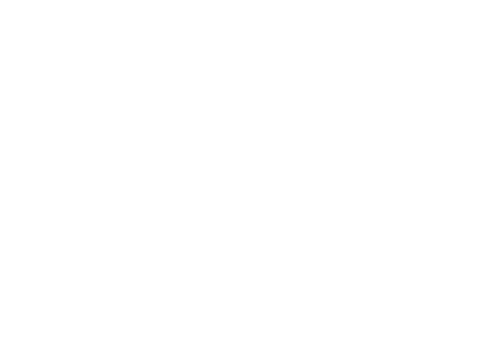 unlike us, this whole plant I have a question about. I know it's a topic that NUWIPEC is exploring and maybe training on in the future- but for plants like Deer Island or maybe anything on the Arrogant Bay or anything that's coastal and coastally influenced, maybe if you could just speak briefly to what? 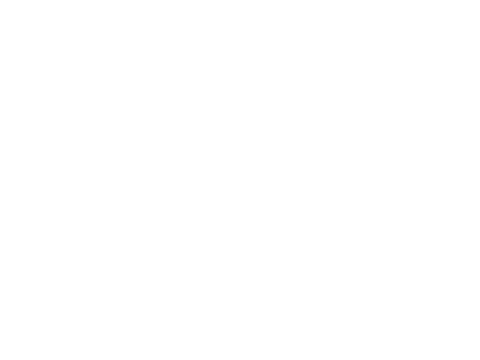 planners and construction folks are looking at with resiliency to coastally influence. That's a big topic. Well, I'm really not totally in tune with that whole thing, but one reference point I have. they're looking at the 100-year flood, plus five feet now, which is all well, and 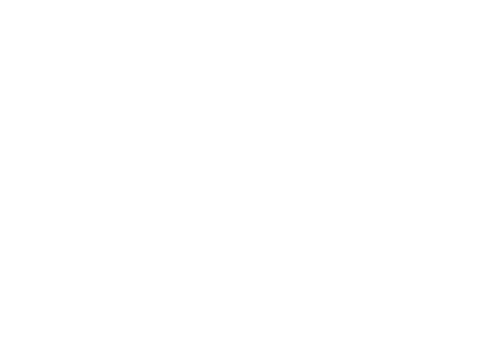 good if you're going to build a new plant but nobody's building a new plant and how do you deal with the old plant? You can't just jack the whole thing up 10 feet. You can't get it across. There are things that can be done and that's what we're addressing this spring in our training. 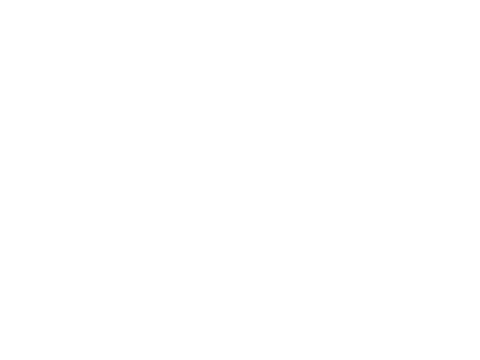 We've got three training courses scheduled, one in Portsmouth, New Bedford and somewhere in Rhode Island, Connecticut, I think, to address those issues. There's a lot of planning and how you're going to deal with it, All right.